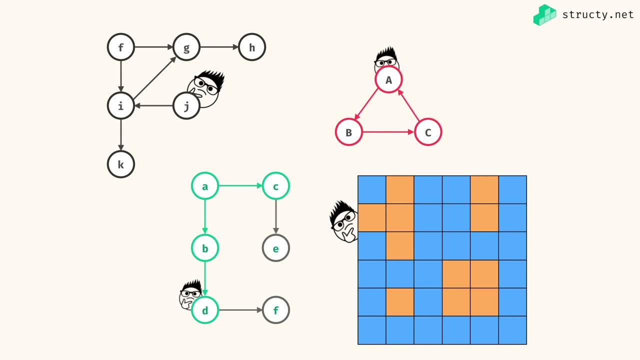 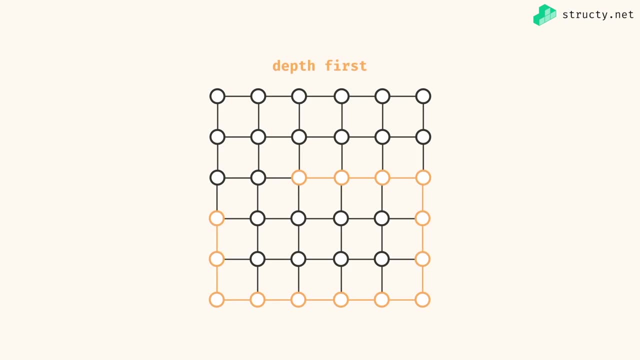 classic interview problems about graphs. Right, and I'm going to give you plenty of opportunity to practice these patterns and different problems. that way, you'll be ready whenever you have them on a technical interview. What I love about the topic of graphs is just using a handful. 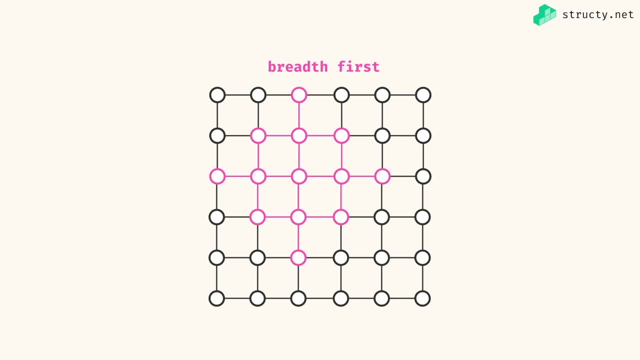 of different algorithms, you can cover the majority of graph problems right. For every graph problem that we cover, we're going to split it up into two sections. section one is going to be about the approach for the video, So we're going to go over the strategy and overall theory. 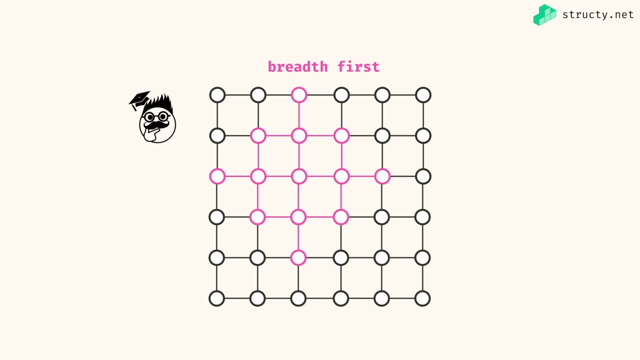 And be sure to sketch out a nice, meaningful picture. We're also going to talk about the complexity of the algorithm in the approach video. We're also going to talk about the complexity of the algorithm in the approach video. We're also going to talk about the complexity of the algorithm in the 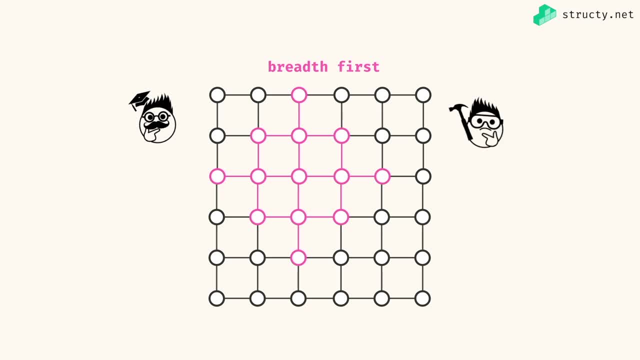 approach video Following every approach. we're also going to implement the code. of course I'm going to be writing all of my code in JavaScript. you'll be able to follow along in any language that you like. So that means occasionally I'll be switching to my. 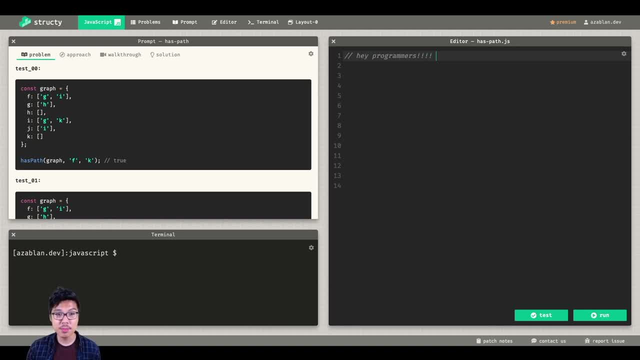 code editor, where you, of course, can follow along. We're also going to be sure to provide links in description as well as links on screen. That way, you can formally read the prompt for every problem as well as look at the different test cases. Alright, I think that's enough. 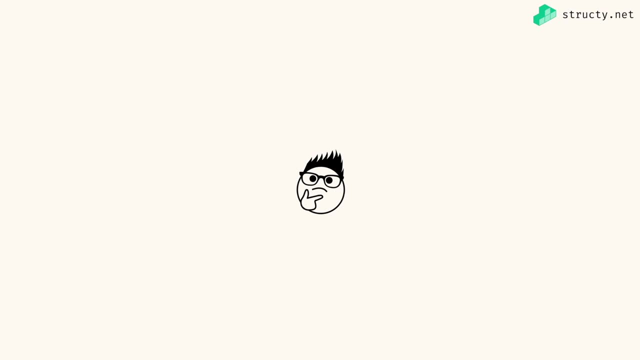 introduction. for now, Let's hop right into the course. Alright, programmers, let's jump right into the course. I want to start by giving you some background about your graphs. we're going to go over the graph basics that you need to start attacking problems in a 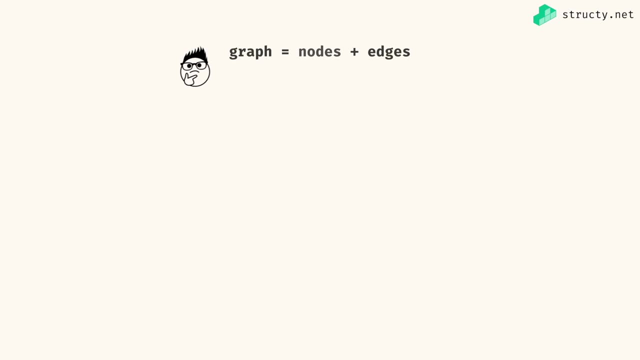 technical interview. So, first off, what is a graph? a graph is really just a collection of nodes and edges. So with respect to nodes, you can visualize them as typically just some circles with some data inside of them. So I'll put some letter values in my nodes over. 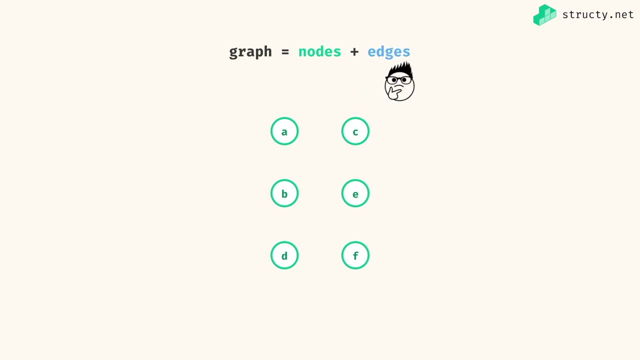 here And when we refer to edges, that would be just any connections between nodes. So, for example, if there was a connection between A and C, it would look something like this: right, What I can formally say is: there's an edge between A and C. I can create many. 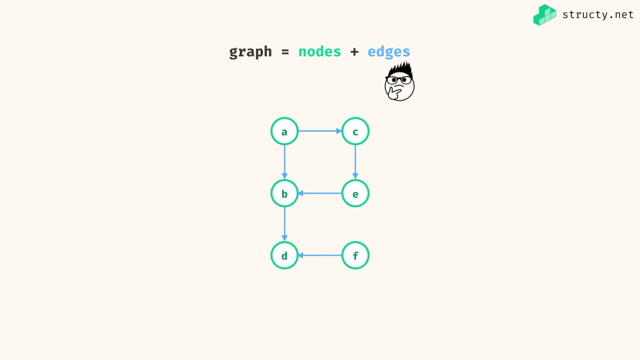 edges between any nodes I want within this graph. Another word you might hear out in the wild when it comes to describing nodes is you might hear the word vertex being used. right, They're really the same thing. In this course, I'll stick to the word node And an. 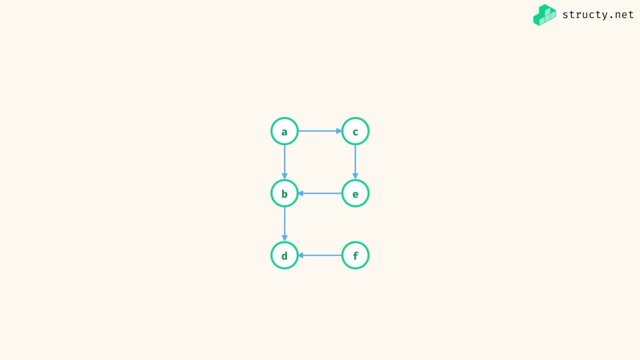 edge is just a connection between a pair of nodes And that's really all. the graph is at a high level. where things get interesting is how we can use this graph framework to actually solve a problem, right? So if you think of these nodes as just things and the 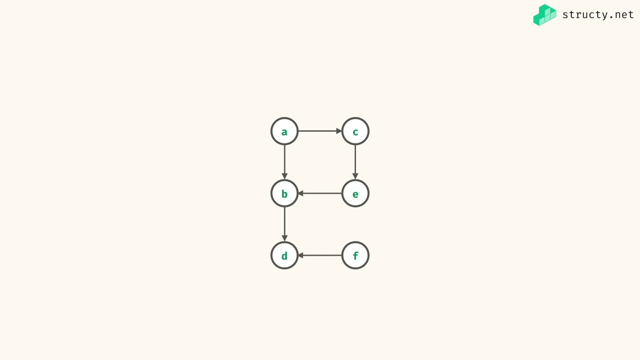 edges as relationships. a graph is great at describing the relationship between things. For example, we can say that the nodes here are cities and edges would be roads connecting cities. or in a similar way, maybe our nodes here are courses and then the edges represent. 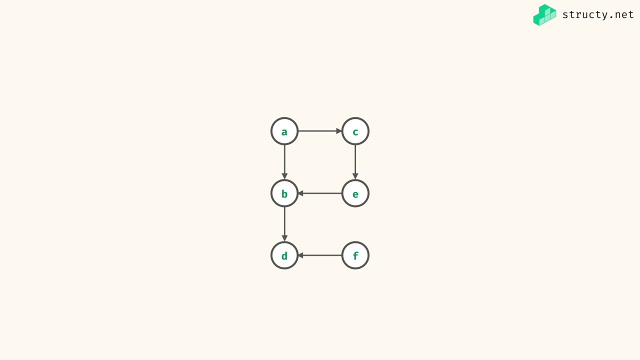 prerequisites, And so in the future we're going to use graphs as a way to illustrate and frame some narrative problem. Let's talk about this graph in particular. here I really have drawn a directed graph And that's because I have some arrowheads along the edges that 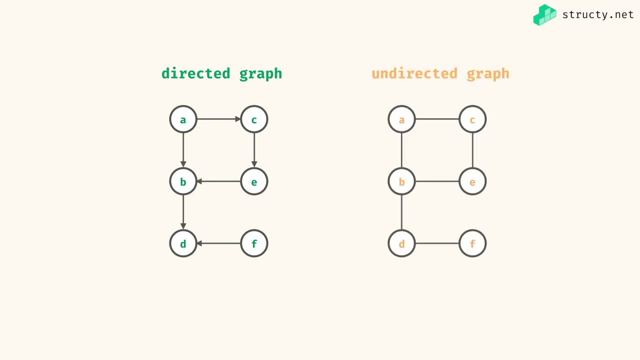 would be a comparison to an undirected graph. So I have really the same structure, except I don't have any arrowheads on the edges. So I'm going to use the same structure, except I don't have any arrowheads on the edges, And that's because I have some arrowheads. 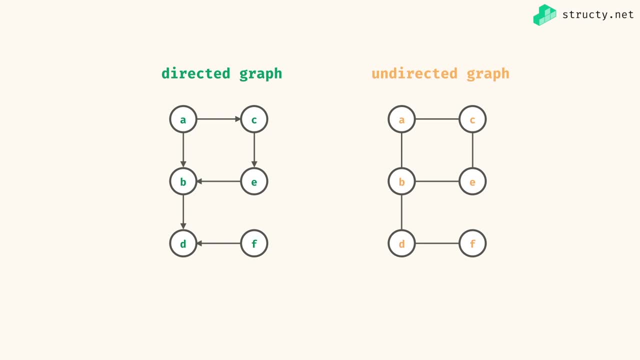 along the edges here, And that means that there is no directionality to it. right, If I look at the directed graph, let's say I was at the node A. well then I can travel to B or C. let's say I move to C. However, once I'm at C, I cannot travel to A. I can. 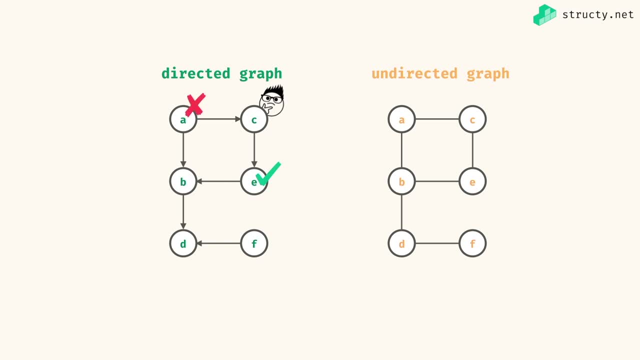 only travel to E right. That's because I have to obey the direction of the arrowheads here. If I take a look at my undirected graph- let's say I was currently situated at the C node over here- then I do have the option of traveling to either A or E right. So if 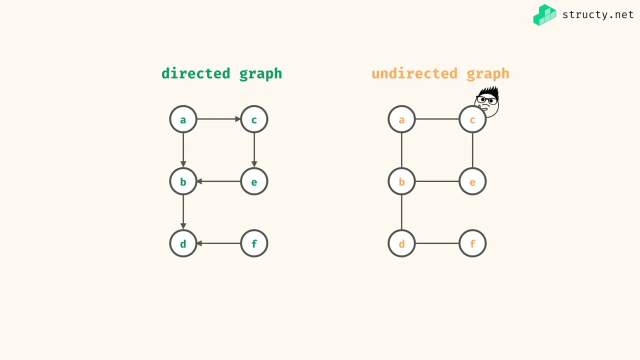 I travel to A, that's all good. I can even travel back to C, So think of a undirected graph as a two way street. For now, we'll just continue on with our directed version. Let me also introduce some useful terminology we can use when talking. 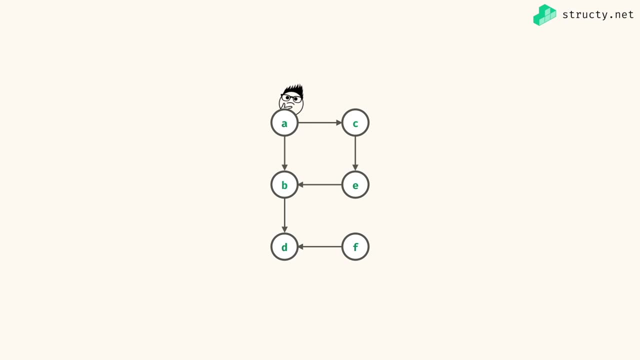 about the nodes in our graph. If I was currently situated at this a node, I can refer to B and C as neighbor nodes, right? So a neighbor node is really any node that's accessible through an edge, of course obeying the direction of the edge. In other words, if I was currently 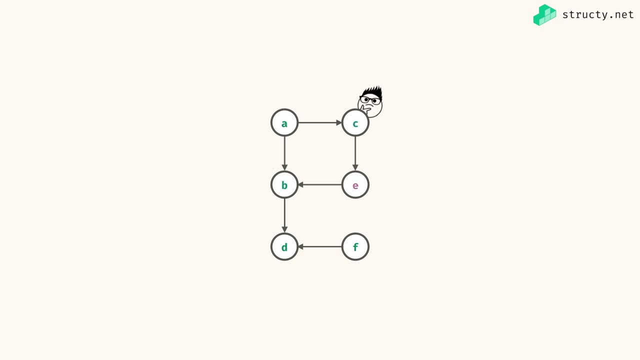 situated at the C node, that I only have one neighbor of E right. If I'm at the C node then I won't be able to travel to the C node right. So if I'm at the C node then I won't. 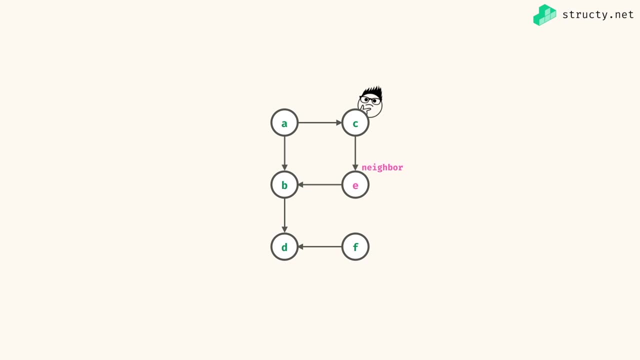 consider a neighbor. Awesome. When you visualize graph algorithms, you should really sketch a picture that looks just like this. right literally draw nodes of circles and arrows as your edges here. However, when it comes to how we implement this algorithm, in some 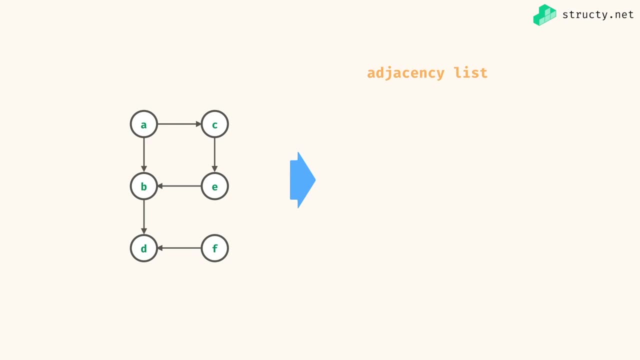 code, we're gonna have to represent it in a more programmatic way, right? So in my brain I think of this image of like nodes and arrows between them. However, in my program I'm going to use typically an adjacency list. it's probably a preferred way to represent. 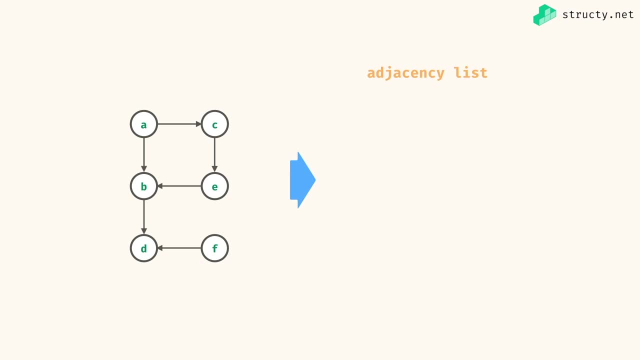 graph information Right. So, depending on the programming language of choice you're going to use, typically we would use some hash map data structure to represent an adjacency list. Really, you're looking forward to using some constant time lookup data structure. that has a key value. 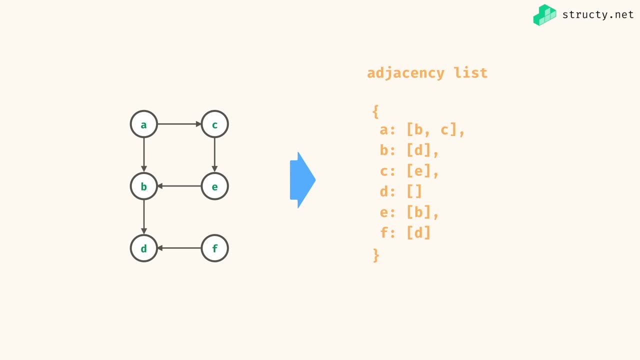 pair mapping right. So if you're in JavaScript, there'll be an object. if you're in Python, there'll be a dictionary. If you're in a language like Java or C, you'll be using an unordered map. Looking at this hash map I have drawn, or this adjacency list: the keys of this adjacency: 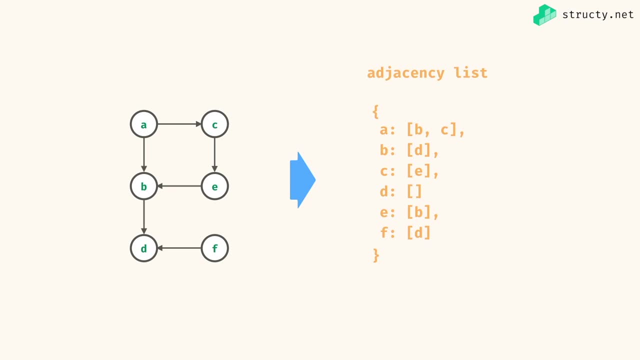 list are going to be every node in my code. Okay, so I can take this node in my graph, right? So I just have all of the node values A through F laid out as the keys. However, if you look at the corresponding values, the 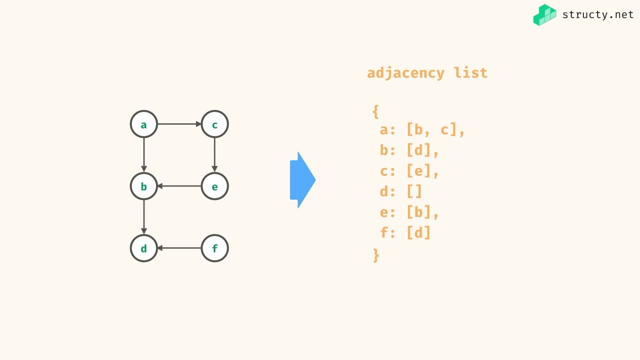 values are actually going to be in array, right? So if I look at this very first entry, it says that I have a node of A And then in the array I've populated all of the neighbors of A. that is, A has two neighbors of B and C. That's why I have this correspondence within. 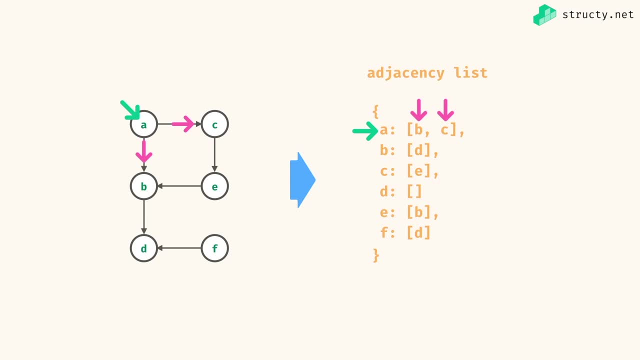 my adjacency list. That holds true for every entry within my adjacency list. So, for example, example: let's say I look at the entry for E, So I go to the spot in my JC list where the key is E. it only has one outgoing edge to be And that's why the array for E only. 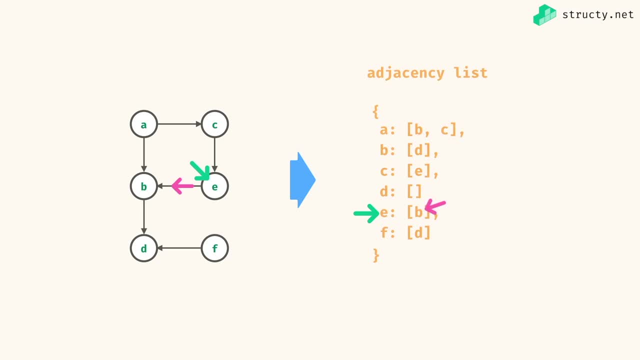 has B inside of it. One thing to also notice: even if a node has no neighbors, it should still appear as a key within my adjacency list, For example, if you look at the D node, D has no outgoing edges. that's why its neighbor array is empty. However, it should still at 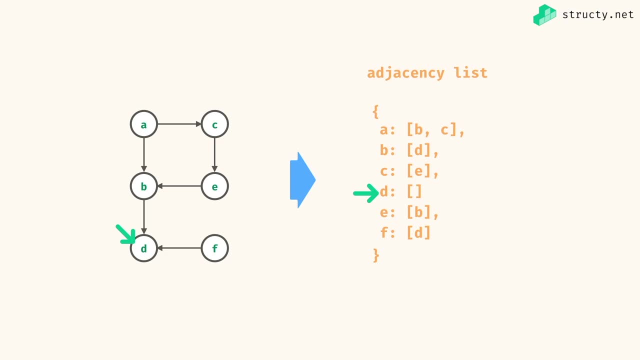 least appear as a key within my adjacency list, right? That way I can still know that the D node exists. So at the start of the course we'll usually be taking in adjacency list as the information to represent a graph, right? But as we sketch through things on, 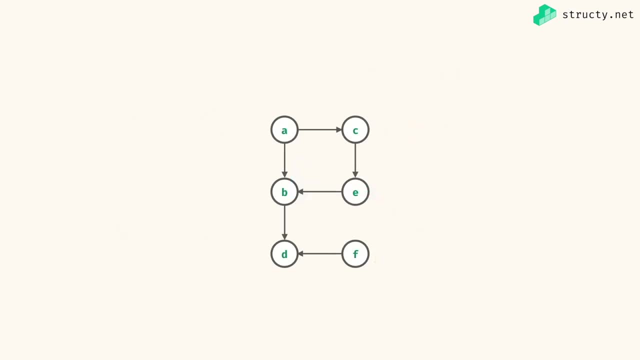 the whiteboard. we should be visualizing them using a nice picture like this. Awesome. So let's actually jump into our first pair of algorithms. To me, the must know algorithm for a graph is really going to be to do some sort of traversal on it. Why don't we start? 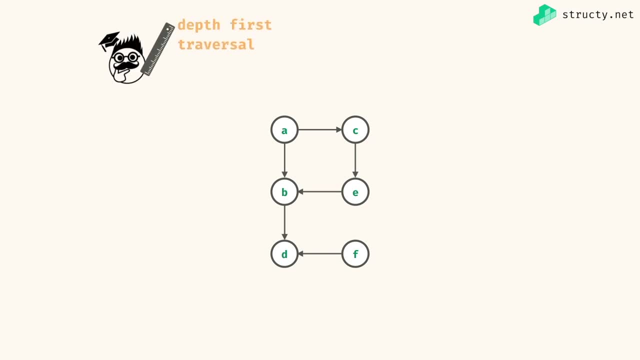 by talking about a depth first traversal, something you may have heard of before. Right now we're going to talk about the depth first traversal reversal algorithm that operates on a graph. So let's start by understanding at a high level what order a depth first reversal would give you. So let's say I had some starting. 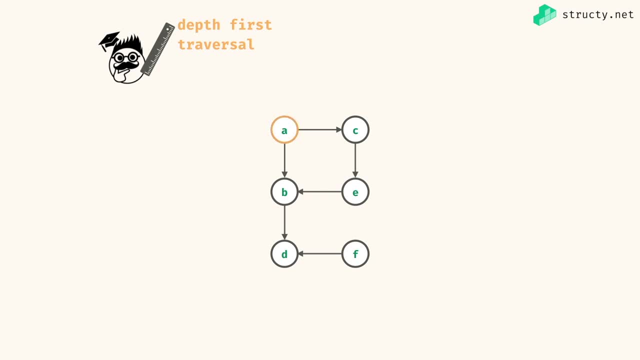 node and I'm going to choose a as my starting node, right? so I'm going to color it here in yellow if I was following a depth first reversal. now that I've chosen a as my starting point, I can either hit B or C next. I'm just going to commit to using B. So let's say I: 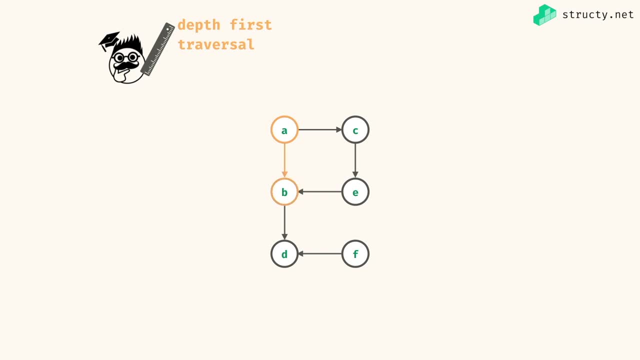 had the sequence so far of a, comma, B, And at this point, if I was truly following a depth first reversal, I must go deeper, to the D node. In other words, I don't go to the C node yet. Cool, that would be a true depth first reversal, right. And at this point, 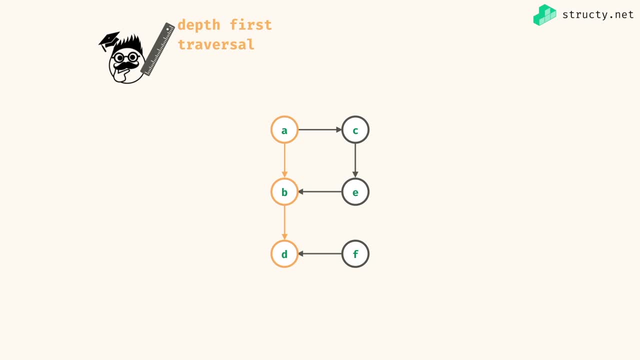 now that I've bottomed out at D, D is a dead end, right. I can't travel to F from D because that would be disobeying the arrowhead, And so now I can move to that other neighbor of C, And from here the algorithm would continue. right, I go from C to E and then E to B. 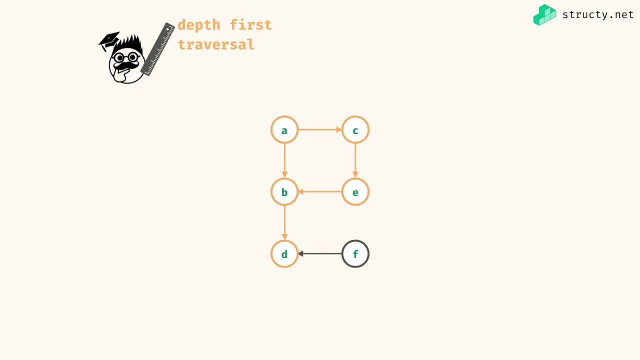 And technically I would have to double traverse some nodes like B and D over here. So overall in this yellow coloring I have colored the full region that a depth first reversal would explore, starting at a notice that if you started at a it would be impossible. 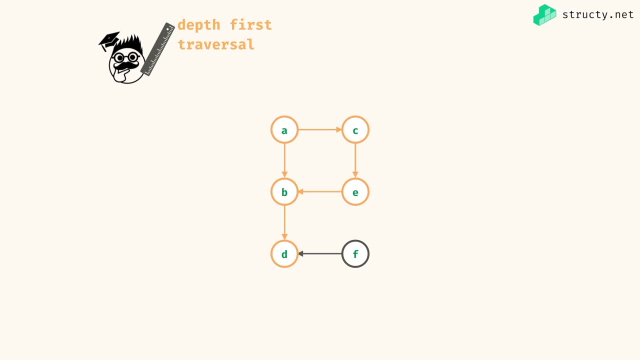 to reach F And that's kind of normal, right? That's kind of why we use these traversal algorithms that can tell you whether or not you can travel between some nodes, And we'll see that literal problem later on, right? So you're probably wondering, you know exactly. 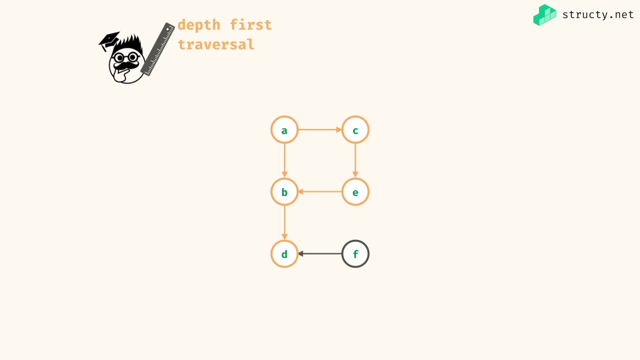 how to implement this, But for now I just want to stay focused on the order that we got right. So, just regarding our depth, first traversal, if we remember the first three, you know- iterations of the algorithm, we hit the sequence. 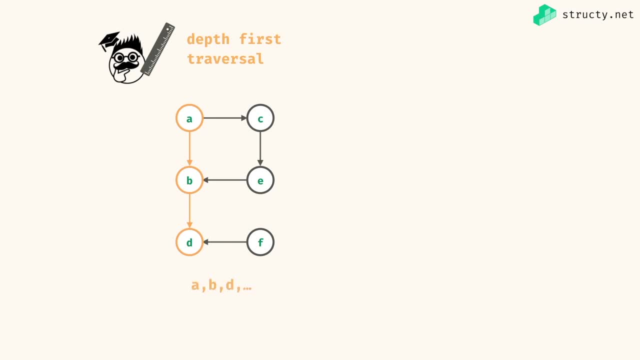 of ABD. right, that's indicative of a depth first reversal. Now let's compare that to the breadth first variant. So I'm going to lay down the same exact graph. we're also going to start a traversal at the A node, but this time follow a breadth first order. 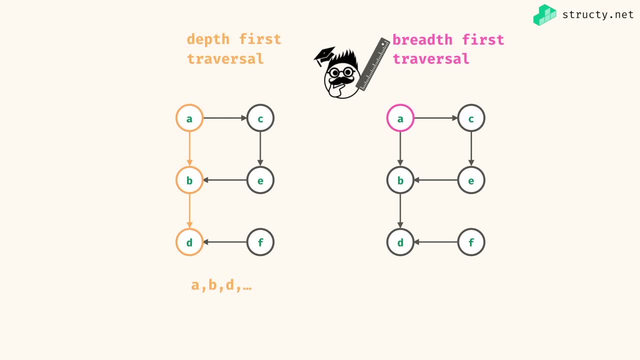 So I have a first and let's say, you know, I chose B as my next node. when it comes to a breadth, first reversal, it doesn't matter like which you know initial neighbor you choose. So I'm just going to choose B. 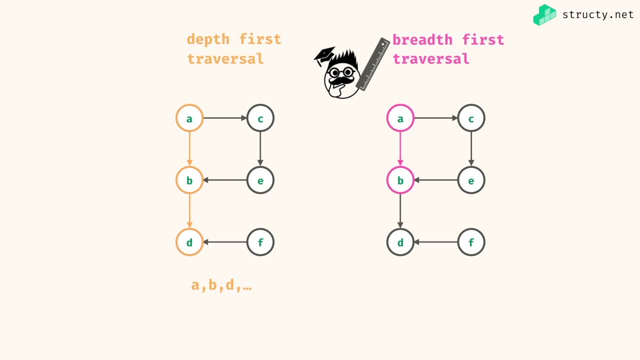 But now that I've chosen B, if I was following a true breadth first traversal, I must hit C next right. And that's the main difference between our depth first and breadth first reversals For the same graph: my depth first would start ABD, whereas my breadth first. 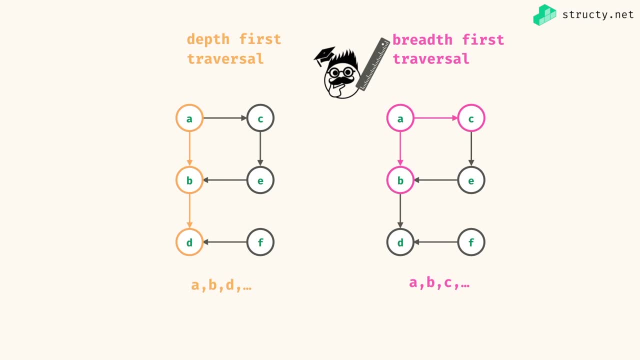 would start ABC, And so you're probably wondering is: is there any importance between this nuance, right? When would I prefer depth first over breadth first, or vice versa? Either a depth first or a breadth first traversal would explore the same exact nodes within a graph, However. 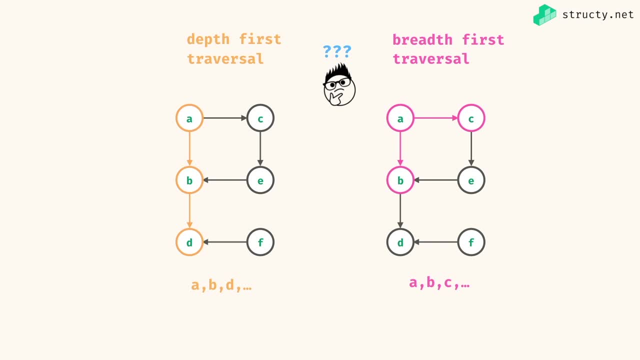 it would explore them in a different order, right, And this is more obvious to see when we have a larger graph with way more edges. And so let's look at how a depth first traversal explores again, but this time on a much larger graph. let's take a look at this one. So I'm 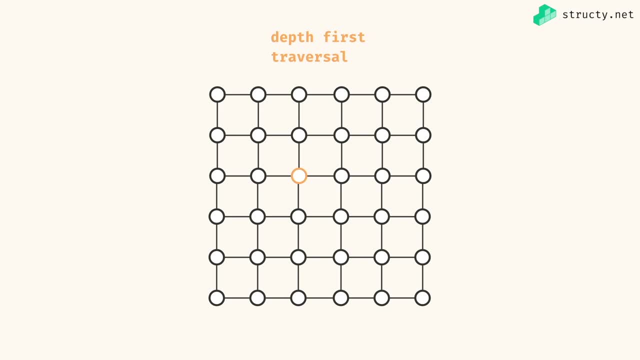 going to choose some random node as a starting point. let's say, I chose this node in yellow. that was doing a depth first reversal. what I'm going to do is, you know, pick a direction and travel in that same direction as far as possible before switching directions. So let's. 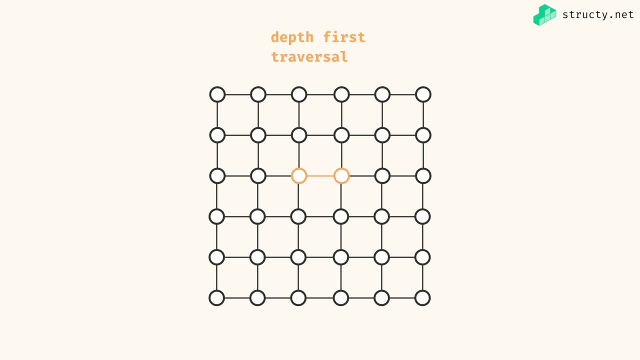 say I move to the right, At this point I would have to continue moving toward the right until I can't move to the right any longer, at which point I have to choose some new direction. So let's say it was downward, or keep doing that until. 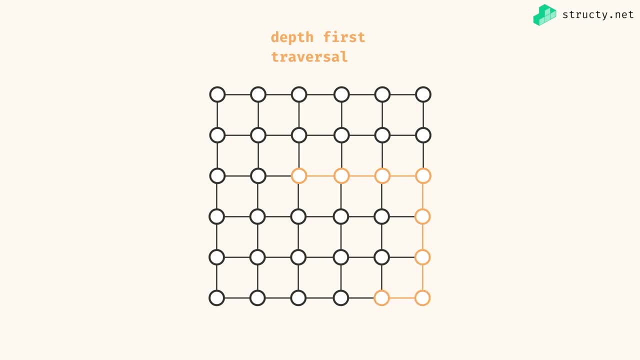 I can't move downward anymore, And so I'd have to move to the left now. Now I'd keep chasing this single path in a very deep direction. So that's behavior indicative of a depth first traversal. right, You're exploring one direction as far as possible before switching directions. 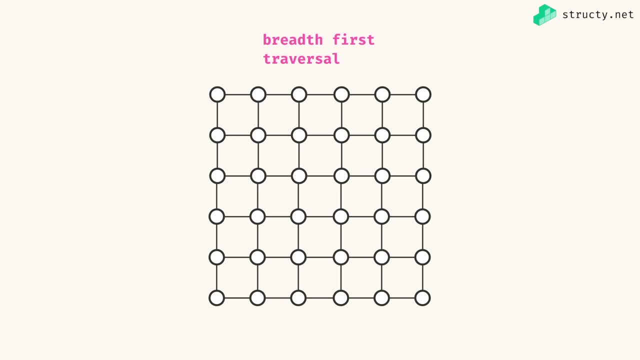 Let's compare that to a breadth first traversal. So let's say I started at the same node in pink. If I was following a breadth first traversal it would look something like this: From the starting point I would explore all of the immediate neighbors of this node, kind of. 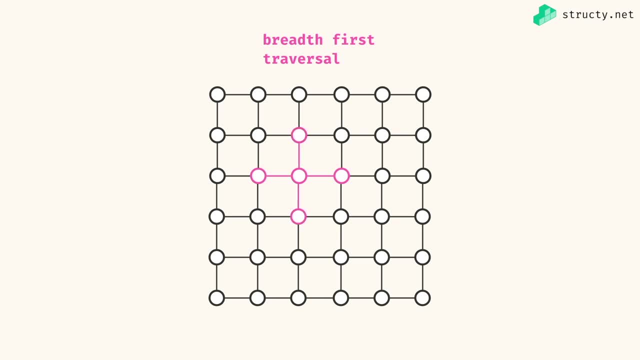 in a circle like this. And now I just keep applying that behavior. So what she noticed about the breadth first traversal is it'll tend to explore, you know, all directions evenly right, instead of just favoring one direction all the way through. That's really the only. 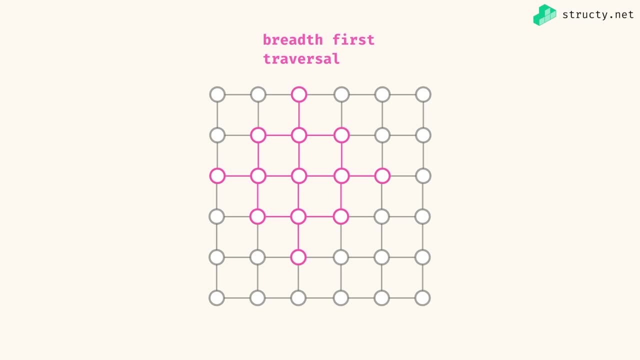 difference between a depth first and a breadth first. When you do a depth first, traversal, traversal. Later on the course I'll bring up explicit problems where you might prefer one over the other. Alright, but for now what I want to do is give you all the background. 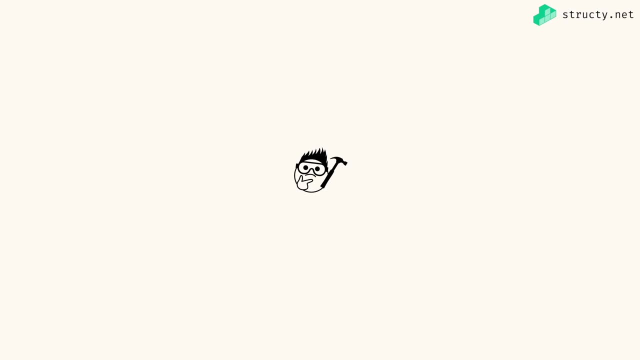 you need So you can actually build this algorithm. we'll kind of talk about things at a high level. consider this the pseudocode. then, of course, we'll express it in some JavaScript code later on. So when it comes to actually implementing in code these two algorithms, 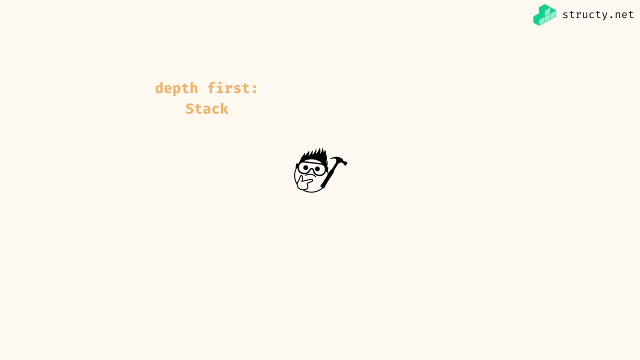 the key is to understand that a depth first traversal uses a stack and a breadth first traversal uses a queue. Recall that a stack is something where you add to the top and remove from the top as well, Whereas a queue is something where you add to the back and 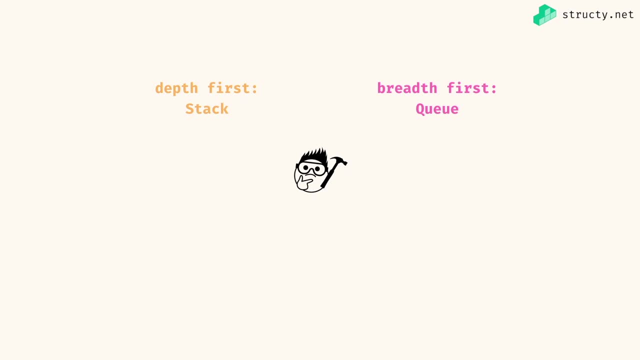 remove from the front And it gives you two very different orderings. That's really the only difference between these two algorithms. So let's start by tracing through our depth. first traversal, of course using a stack, So I'm going to use a slightly different graph. 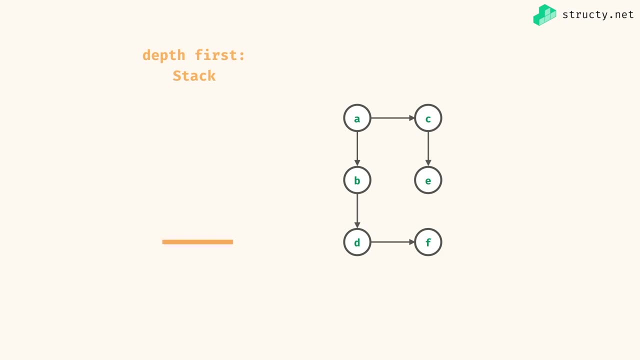 And to visualize my stack, I'm going to use this bar to represent the bottom of my stack. Obviously, for me at least, I think of a stack as some vertical data structure, So I'm going to use a stack here. Cool. So let's say I just arbitrarily chose a as my starting node. 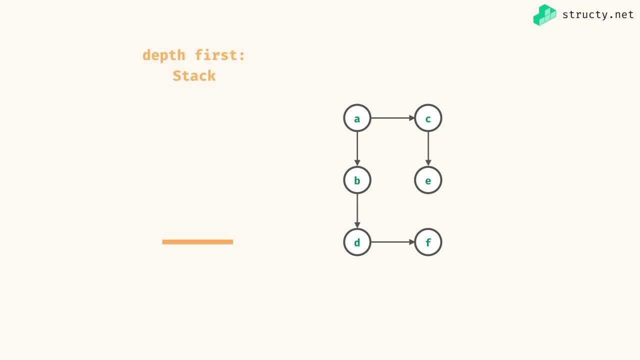 to perform my depth first traversal right In the long run. I'm just want to print out all different node values within this graph. So what I'm going to do is I'm going to take my starting node of a. I'm just going to immediately initialize it onto my stack. So right now, 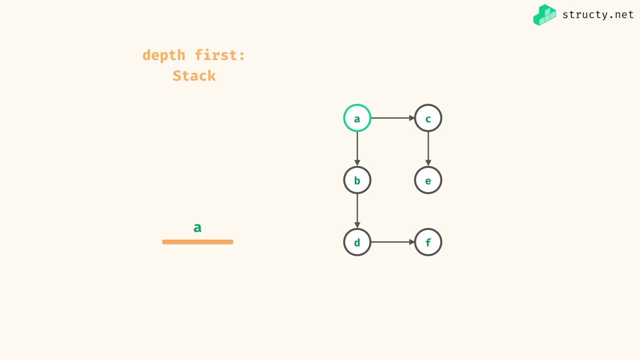 a is the only thing on my stack. It's also at the top of my stack And now I can enter the flow of the main algorithm here, Because I have a stack. what I can only do is remove the top of my stack. 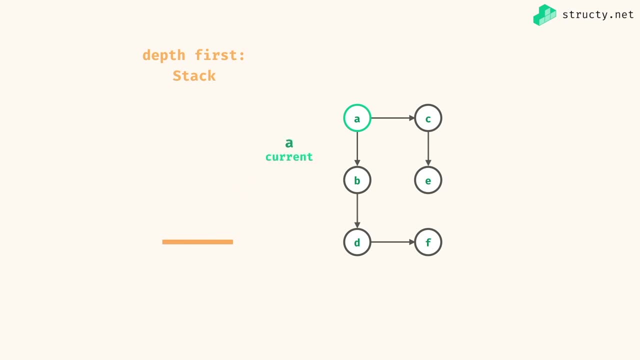 So that means I pop off a from the stack and consider the a node, my current node, being looked at right At this point. let's say I print out a to my console And from here what I want to do is consider A's neighbors right. So if I look at the C node, what I should do is 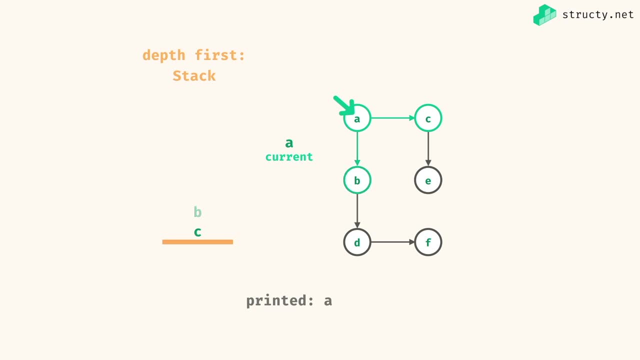 just push C to the stack, then also push B to the stack, right, And it doesn't matter like in which order you push these neighbors. If I wanted to hit B first, then I'm going to push them second right. Awesome. Now it ends like my first iteration of this depth. 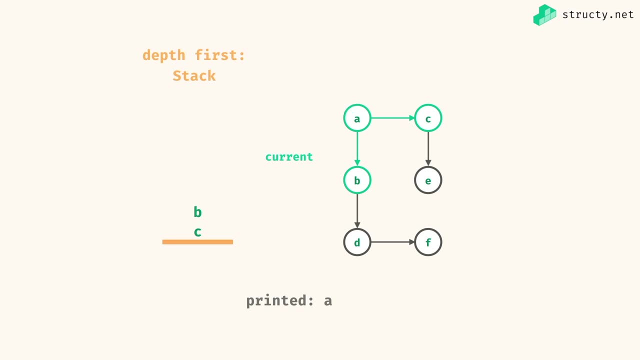 first traversal. Cool, So at this point I can look at my stack and my stack still has some data on it. So what I should do is again pop the top of my stack. So I'm going to pop and be off my stack And now becomes my current. I'm also going to print it out At this point. 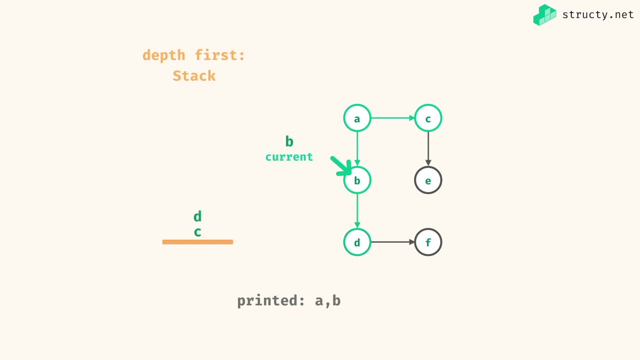 I look at B's neighbors. B has one neighbor of D And so I push D to the top of the stack. Notice that, because I have a stack, D ends up on top of the C right. And so now, when I get to another iteration, when I pop the top of my stack, I look at the D node and 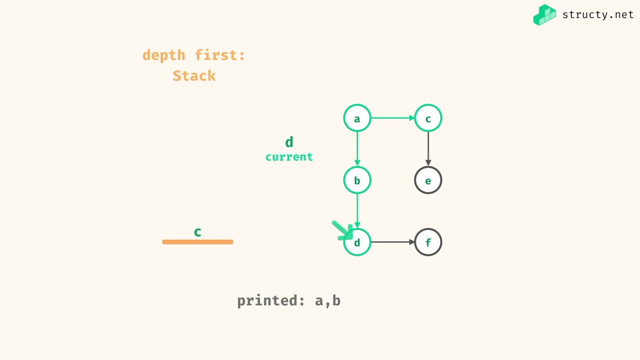 I can print out D And this feels good because so far my print order would be a B D. notice that I kind of pursued that single path deeply following a B D. But I have to look at these neighbors. I can take F and just push F to the top of my stack. Next iteration: my stack. 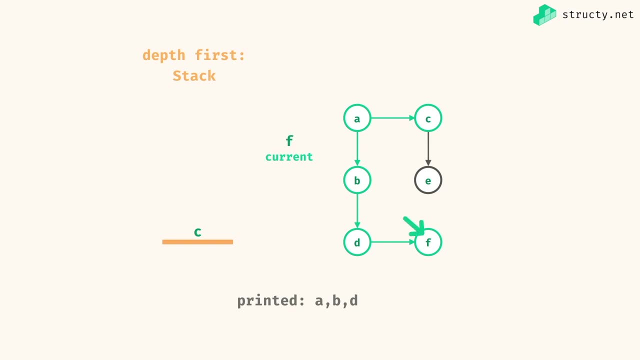 is still on empty. So I should do is pop the top. F is now my current. I can print out F, But F has no neighbors, So F isn't going to push anything else to the top of the stack Right At this point. I get to this next pass And I pop the top of my stack And that 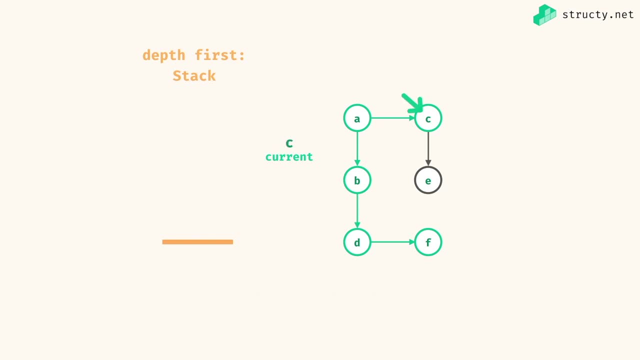 means C is now my current. I can print out C's value And then I can look at C's neighbors And I just push E to the top of my stack. On this last iteration, I pop the top of my stack. he is now my current. I print out E. since he has no neighbors, I don't push anything. 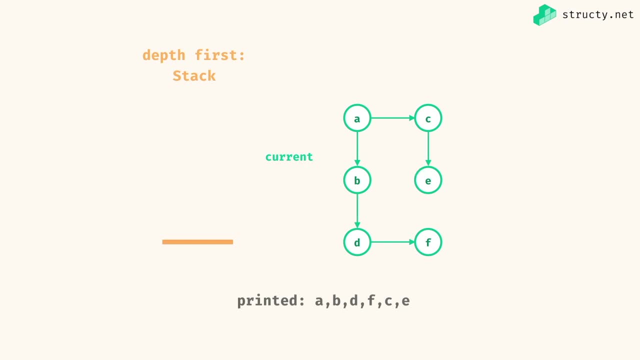 else to the top of my stack, And at this point I've reached the state where my stack is empty And that means my algorithm is done right. That means you explore it. you can see that it's stored as far as possible within your graph. Notice that might not necessarily be. 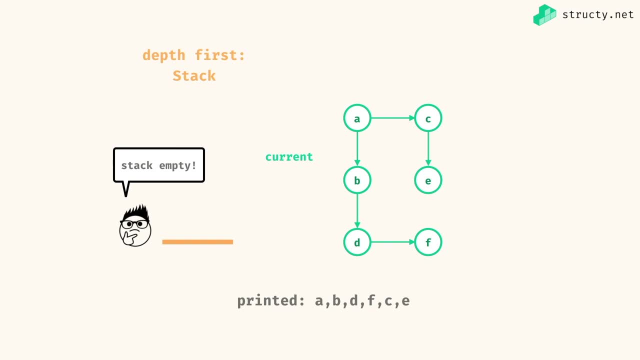 the case that you're able to hit every node of the graph. In this particular example, it was possible, though Awesome. So let's redo that trace using our breadth first algorithm, which means we just adjust things slightly And we use a queue order, right, Remember. 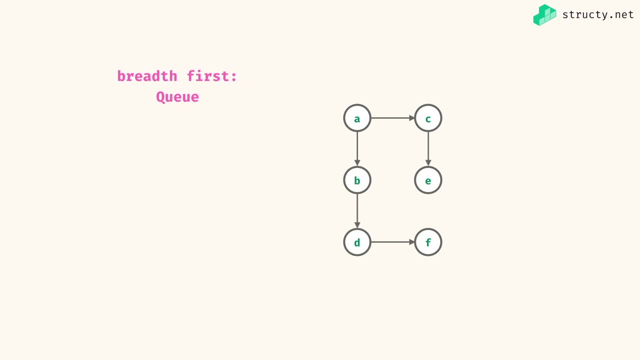 that a queue is a first in, first out data structure, meaning things enter to the back and then they leave from the front. And so let's say I use this arrow to represent the directionality of my queue Right And I start the algorithm in the same way for my breadth, first reversal. Let's say: 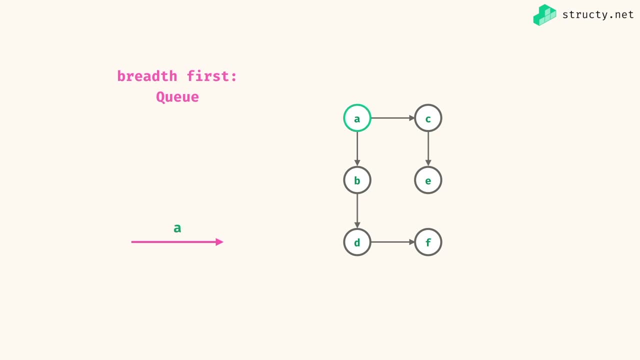 I wanted to begin at node A, So I just initialize my queue with a cool. So I start by removing the front of my queue, So A becomes my current node. I can print out a as well, And now I consider A's neighbors right, So I consider B and C if I wanted to travel to B before. 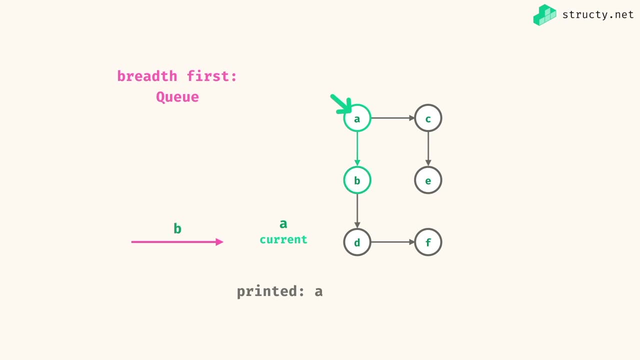 C, then I should push B to my queue first, right. So I add B to the back of my queue Right And I should also add C to the back of my queue Right, And that would actually end my first iteration. So now I look at my queue, it still has some stuff on it, So I removed. 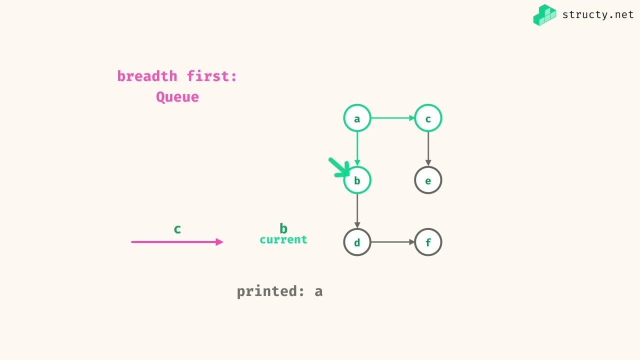 the front of my queue. That means B becomes my current. Of course I print out B Now I consider B's neighbors. So I just look at the D node and I push D to the back of the queue. Since D enters through the back, it ends up behind the C And that's really important. 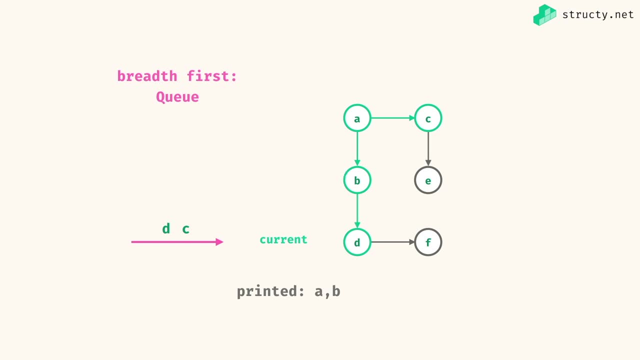 behavior. Next iteration: I remove the front of my queue, So my current is now C. right, I can print out C and then look at C's neighbors of just E, and I add E to the back of the queue, which means that in the order of my queue, E ends. 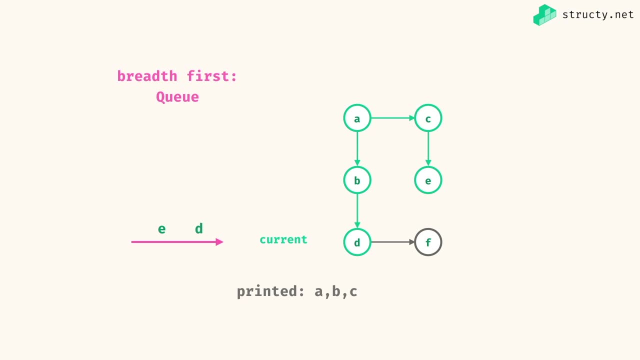 up behind D. On my next iteration I removed D from the queue And I print out D and add its neighbor of F to the back of my queue. Next iteration: I remove E from the front of my queue printed out. Since E has no neighbors, he's not going to add anything else to the 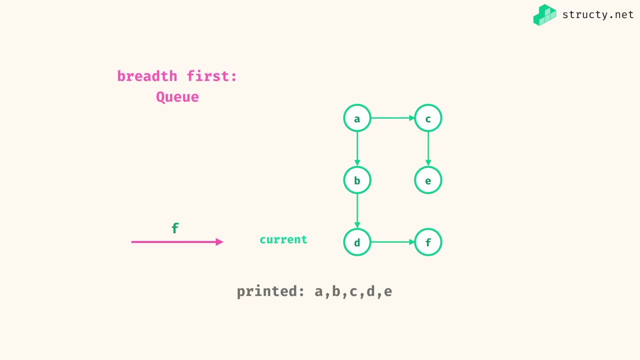 back of the queue And, of course, finally, F leaves the front of my queue. I print out F. F has no neighbors, at which point now, my queue is totally empty. And since our queue is empty, that would be the end of our algorithm. All right, and that's all there is to our depth, first and breadth. 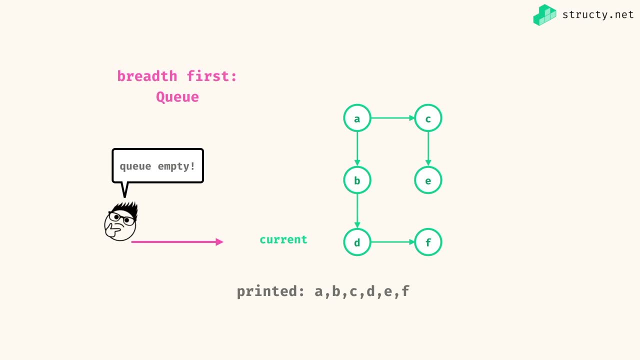 first algorithms. they're going to be the nice baseline code that we use to solve many different graph problems. I think that's enough theory For now. what I want to do is now switch to my code editor, where we can actually implement these in JavaScript. Hey programmers. 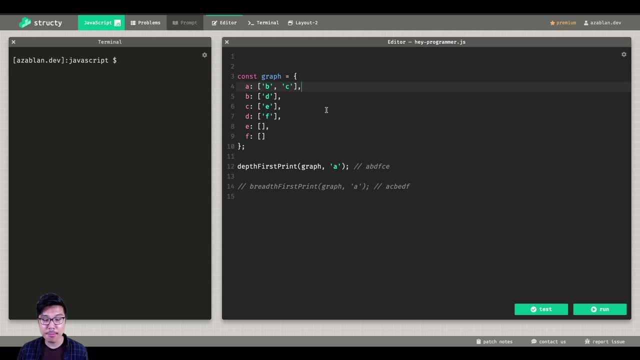 here I am in my editor. what I want to do is now show you how to implement, For example, those depth first and breadth first algorithms. So we'll start with the depth first, And my goal is really just to build a function that will print out all of my values in the graph. 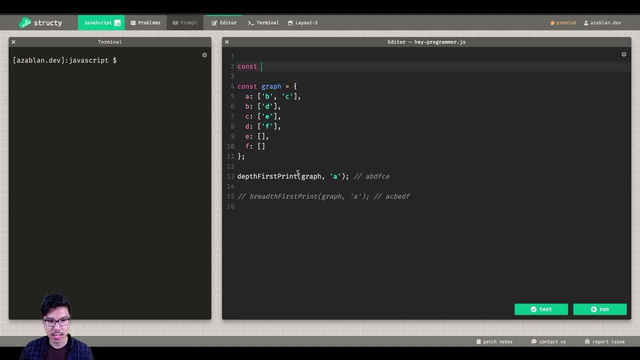 according to a depth first traversal right. So I'm going to define this function: depth first print, make it an arrow function JavaScript it's going to take in the graph which is going to be given as a nice adjacency list, And this is actually the same graph in that. 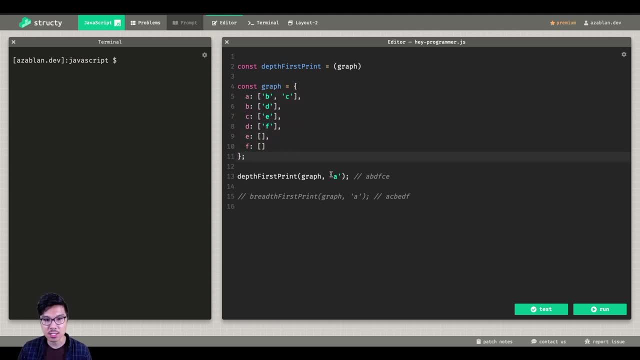 last example we traced out. I'm also going to need to specify some starting node here. I'll call it a source node. I'm going to begin the traversal starting at that node. Cool, And so we know, inherent to a depth. first traversal is going: 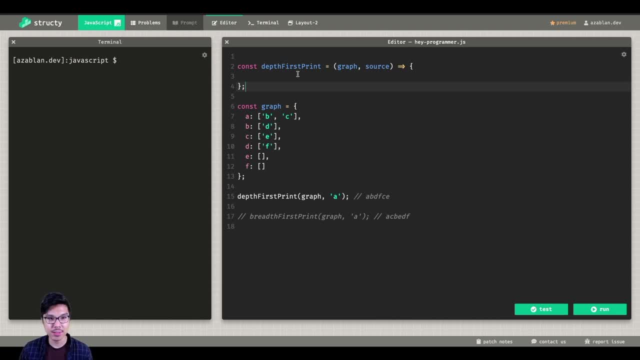 to be a stack, So I'll show you how to implement this iteratively, which means you need an explicit stack. For me, in JavaScript, that's as simple as just using a JavaScript array. right, I'll make it empty at the start And I can use this array as a stack, if I just 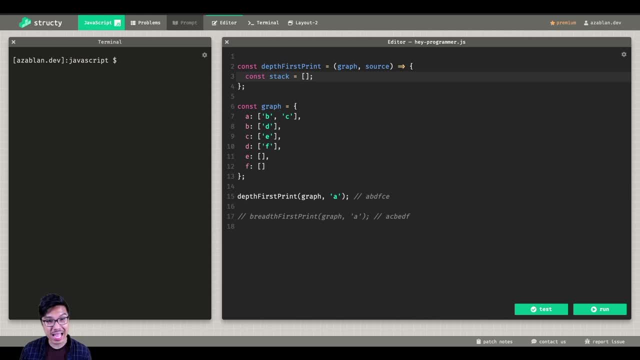 commit to using operations that manipulate the same end of the array. In other words, if I just use push and pop, that will always manipulate the end of the array, right? So I'm going to use this array as a stack And I'm going to commit to using operations that. manipulate the same end of the array. In other words, if I just use push and pop, that will always manipulate the end of the array. right, I'm going to use this array as a stack And I'm going to use this array as a stack And I'm going to use this array as a stack. In other words, 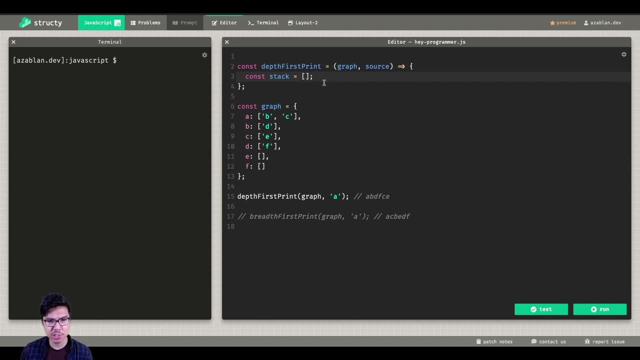 removing and adding to the end of that array. What I want to actually be sure to do is I want to initialize the stack with my starting node, that is, with my source node. remember that, like a node here is really just designated by some character, Cool. And when it comes to designing like the main, 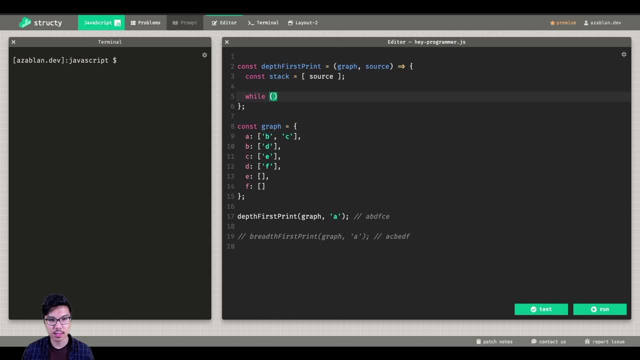 loop for the algorithm here. do you want to keep running the algorithm while the stack is not empty, In other words, while stack dot length is bigger than zero, then I have to keep running, And that's very reminiscent to what we expressed on the whiteboard. So, when it comes to performing, 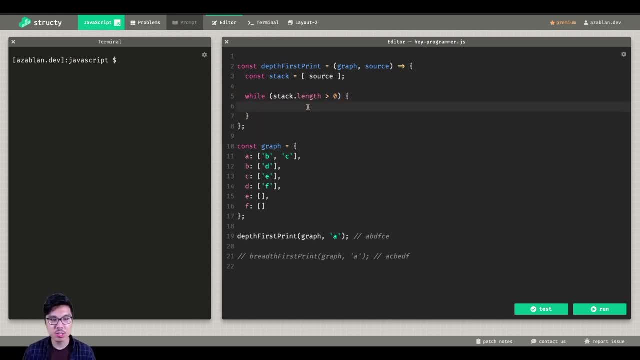 forming like a single iteration of this depth. first, what I want to do is remove the top of my stack. So if I do stack dot pop, that will remove the last item of an array, in this case like the top of my stack, and also return it to me. So I'm going to say that. 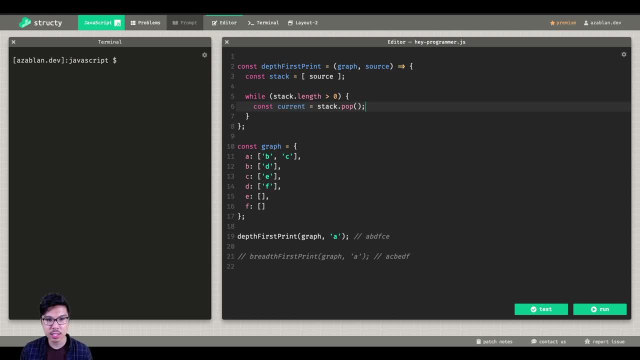 to a variable, I'll call it my current, And so this point would actually be a great opportunity to just print out that current. So I'll console: dot log current, Right. So looking at you know this example over here, since I initialize a stack to contain just the source node of 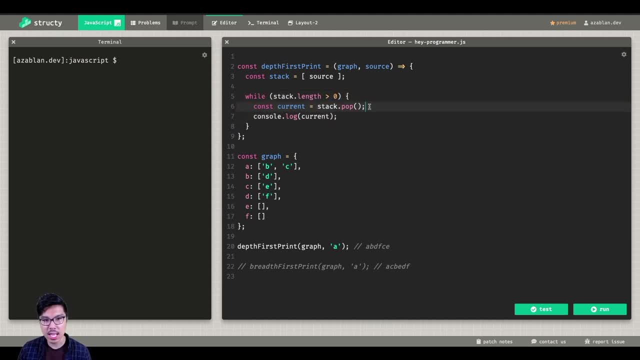 a. on the very first iteration of this while loop I would of course pop out a, then I would print it out Right And from that point what I want to do is consider as neighbors of B and C. So if I want to look at like the array associated with a, I can just key into: 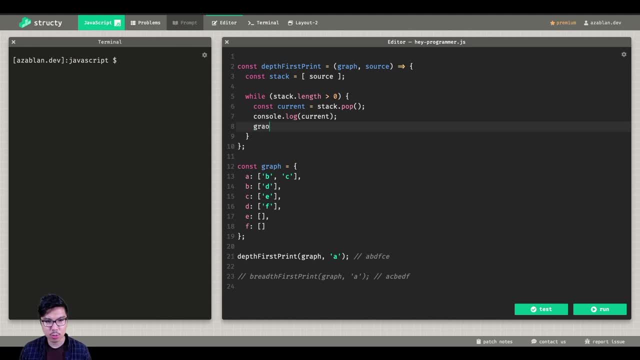 my graph right because my graph is an object right now. So if I say graph square bracket current, right. if current is a, that means graph square bracket current would give me back this array. I want to iterate through every node or every neighbor in that array. 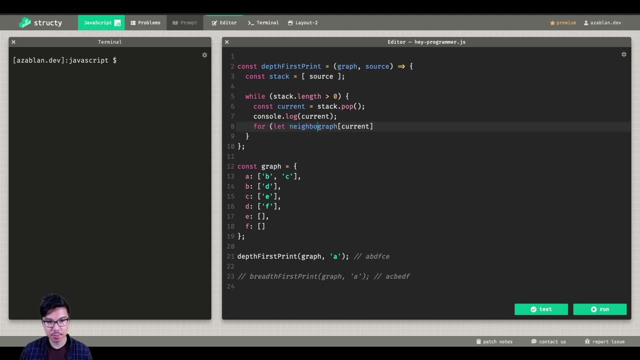 So I'm going to nest a loop here. I'm going to say for let neighbor of that array. So if you're unfamiliar in JavaScript, if you just use a for of loop, that will iterate in order through an array. So now I'm hitting neighbor as B and neighbor as C, What I want. 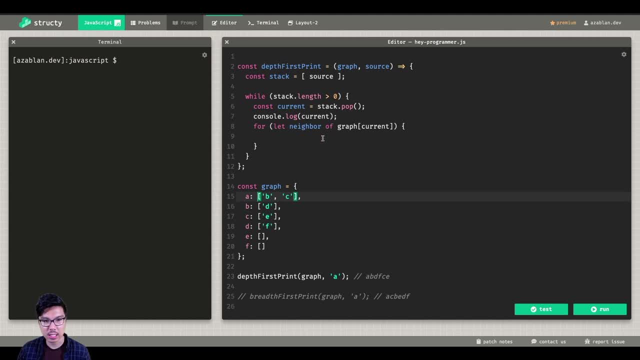 to do with those neighbors is simply push them to the top of my stack, So that will just be stacked up. push and push this neighbor. Awesome, I'm going to be sure to push every single neighbor that it has. So sometimes I'll have two neighbors, Other times I have. 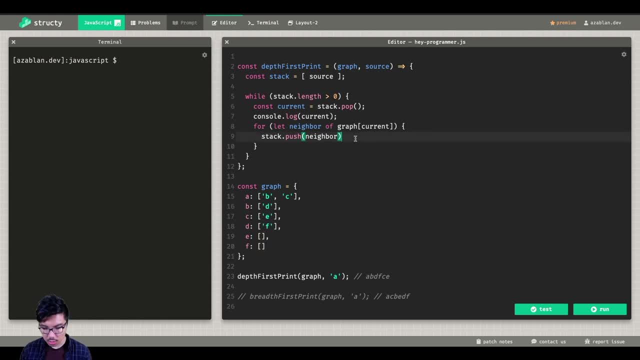 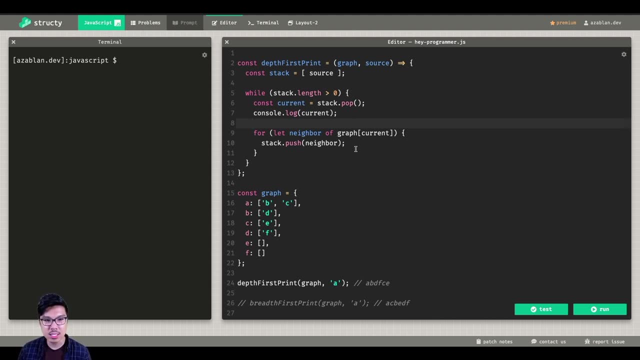 one neighbor, Or even no neighbors. That's really all there is to implementing a nice baseline depth first print. something that I do want to point out: My favorite way to implement this algorithm is to consider like processing your node when it leaves the stack, not when it enters the 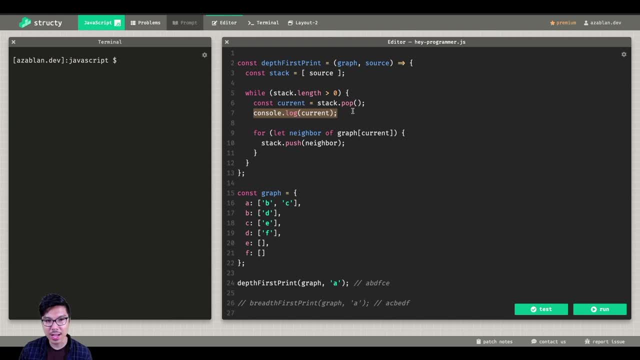 stack. In other words, I usually write, like my print statement, right after something is popped, And the thing that I pop is exactly what I print, right? So let's go ahead and give this a run. see what we get. It looks like in my terminal. I got the order of a. 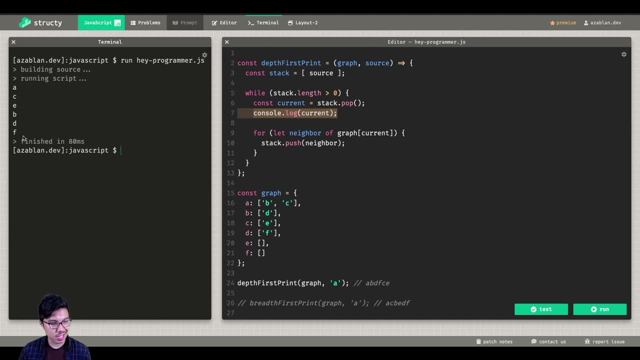 C, e, BDF, which you'll notice is slightly different from what I expected from over here. However, this would be also a valid depth first traversal we have to bear in mind is, you know, depending on like the arbitrary order of values within the same neighbors. 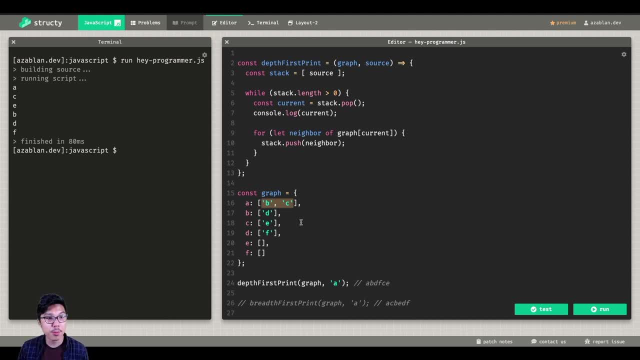 array, you could tend a different direction at first. right? Most important thing I look for when it comes to verifying a depth first is to make sure that I, you know, chase the same direction before switching directions. right? So, since I started out with a C, so 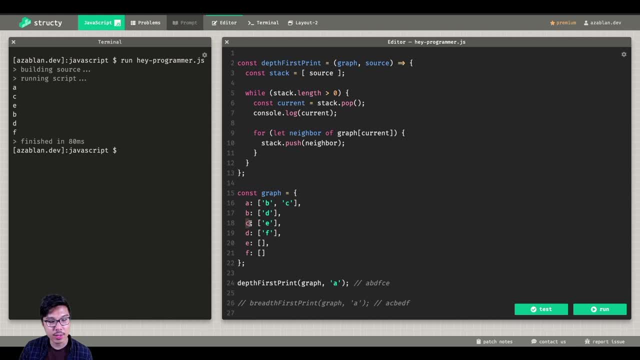 let's say, I'm going from a and then to a C over here. the next move would be going to E, And that's exactly what happened in my code, right, And then, once I hit, E is actually a dead end. So then I can go on to my other lateral neighbor, like B, right, And so I 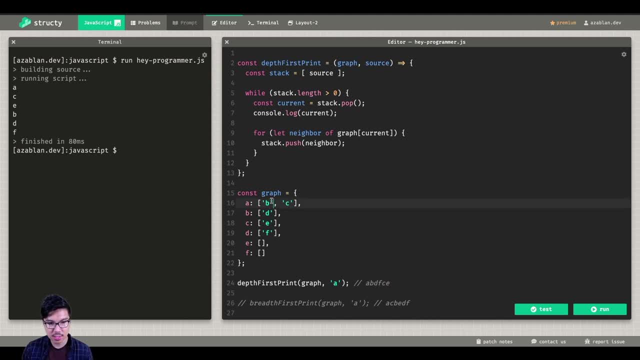 can contrive the same order I expected here. if I just flipped this right. so I put C followed by B, we'll give that a run. they're both valid depth first reversals. See what we got now. So let's say that I just popped out a from my stack, So I printed out a, that's nothing. 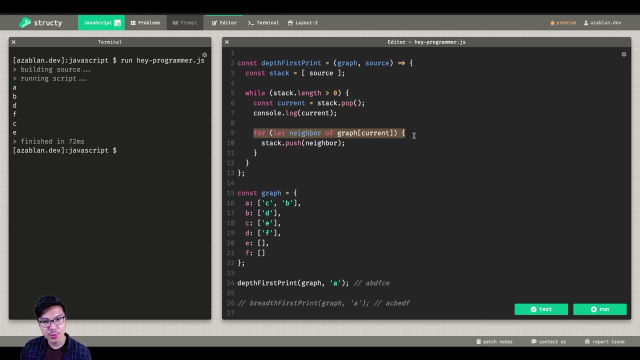 fancy right, And then from there I start iterating through the array that's associated with a right. So on the first iteration I iterate through C- right. If I push C on the stack, let's say this is the bottom of my stack. If I push C on the stack, it's right. 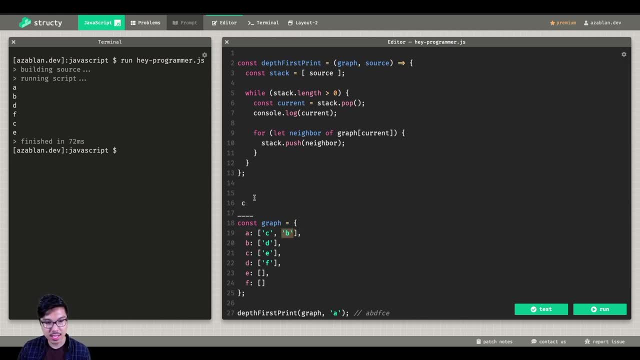 here. Then, followed by that, I push B on the stack. Now B is on top. Since B is on top, we already have the second iteration where B is on top. Because B is in the first iteration, we already have B on the stack. So we're gonna come back to the top of the array. So for 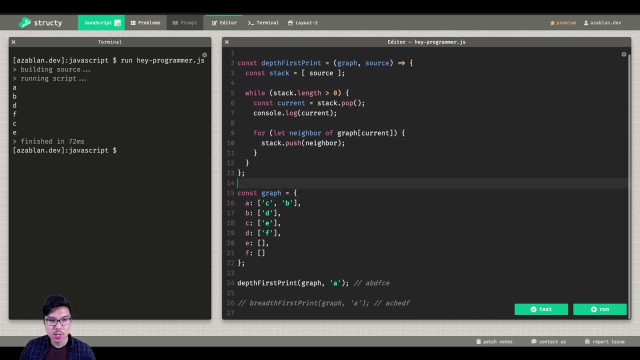 the next iteration. we're gonna go ahead and trigger B, So we're gonna click on the first iteration And then we're gonna take the iteration we created When you log in. it's a super important step, So it's gonna give you a little bit of a sense of where your current version. 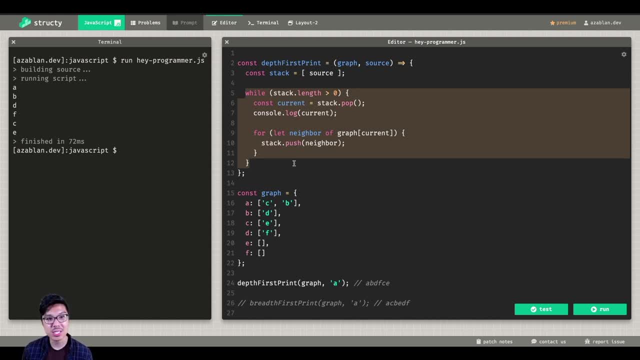 is going to be in a few seconds, So let me jump in here. Number one: I'm going to go into this region And I'm going to create this region first, Because now I'm going to have an array of values right, And let's call it just a little bit. 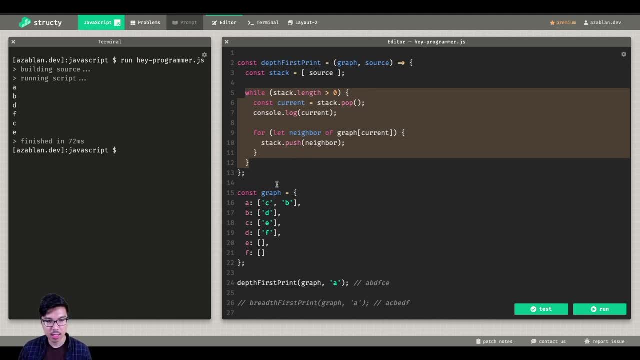 All right, let's click on this region And you can see that this region is under the first iteration stack. So let me show you how to implement that as well. And when it comes to you know, having all these different tools in your arsenal, I would definitely practice both the iterative. 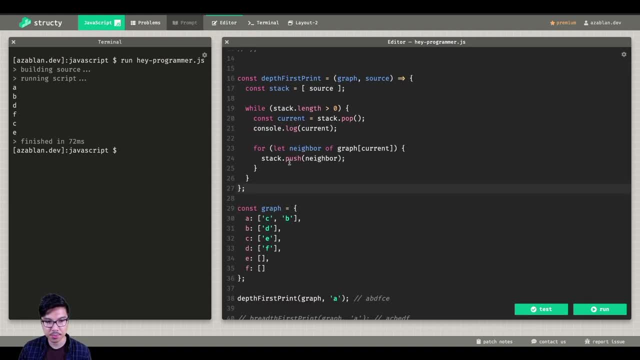 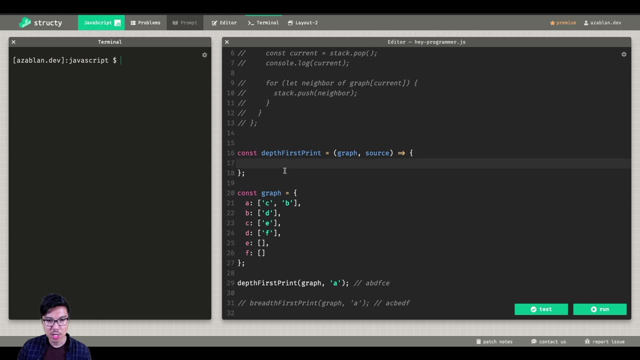 and recursive flavors. We'll see that later on this course. So let's say I wanted to solve the same problem, But now recursively it's actually going to be less code. So I'm going to have the same sort of arguments. I'm going to have the graph which is the adjacency. 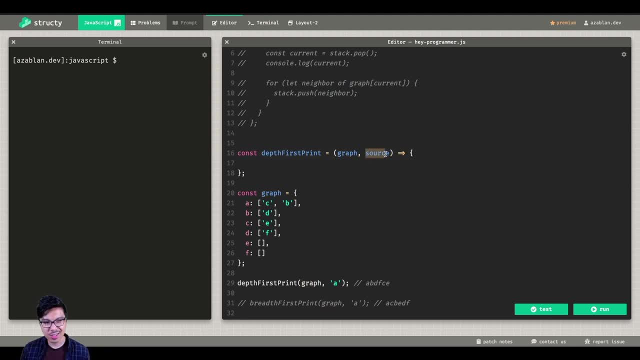 list as well as a source node. consider like the source node as like your current location. So if I'm at some node, maybe the first thing I should do is just print out myself. right, print out this node. So I'll do is console dot log this source node And that feels. 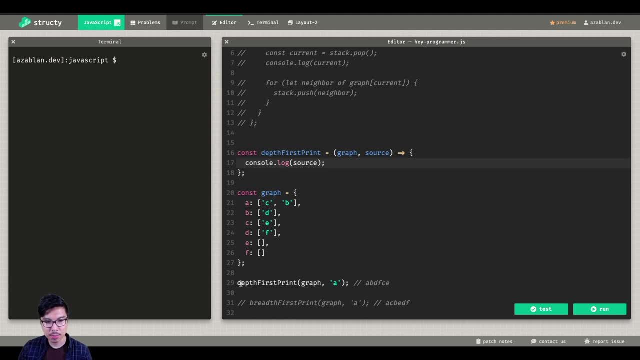 good just from the get, because when we actually do a top level call to this recursive function, they're passing in a as the source node. So I do want to begin a as the first node in my print And then from there I need to look at a's neighbors. Well, if you want to look, 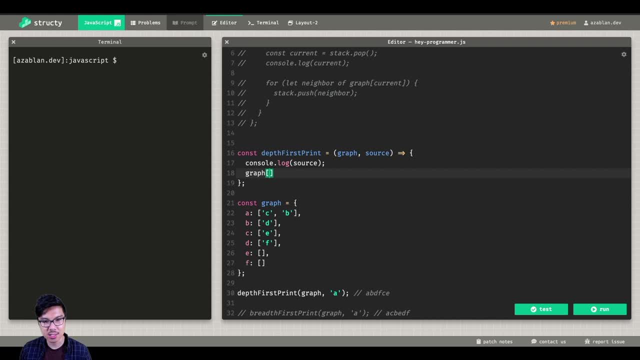 at a's neighbors, like before. just key into the graph adjacency list using that node, right? So I'm going to give me an array of C and B. Now I just iterate through that array. So I'll say: for let neighbor of that array. And at this point what I want to do is now: 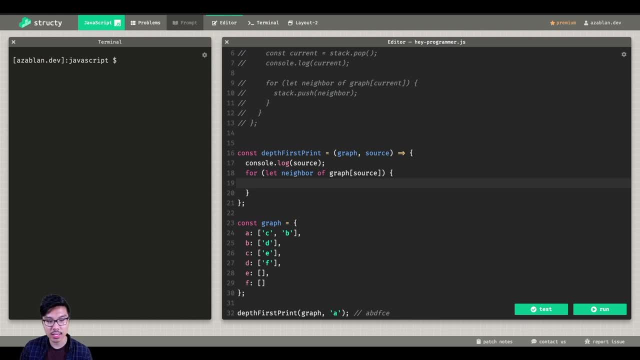 do the recursion right. so I make a recursive call on each of these neighbors. So for me that means just called depth, first print. you give the same graph right, the graph object doesn't change. but you should change like the source node. Now you want to pass. 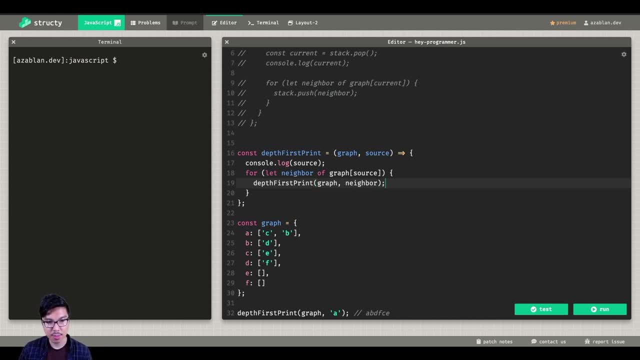 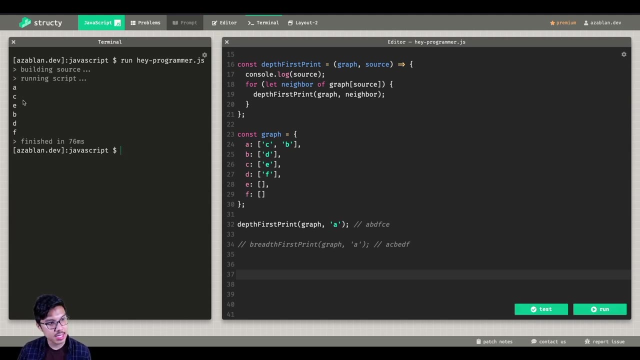 in that neighbor as the source node. you're going to make a recursive call for every neighbor in that array, And this would actually be all we need. Let's go ahead and just run this version. Give that a run over here. Looks like now we get the order AC, BDF And that's really again another. 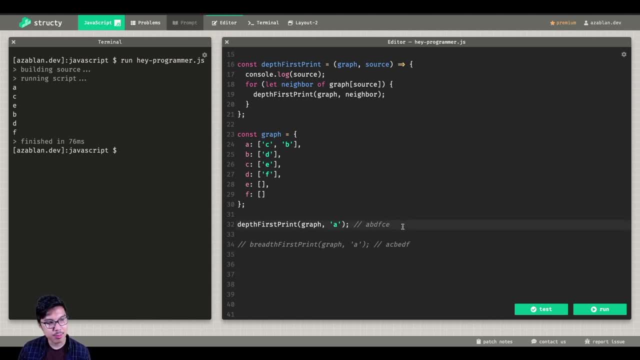 type of depth, first print, right. It's not exactly this order, Because this time we chased C first, right, we went a C. if I want to get exactly this ordering in my recursion, then I would have to put B first, right. Really same sort of pattern, though let's give that. 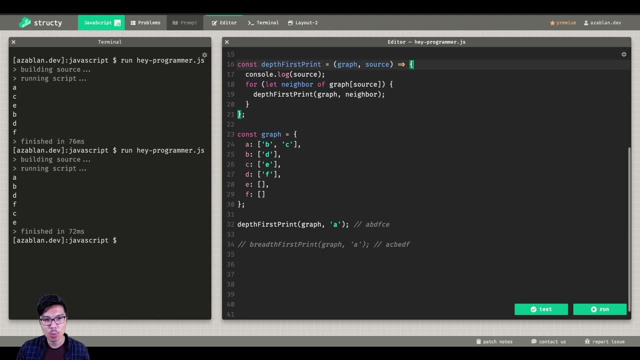 another run. Good ABD FC. One thing I want to bring up about this recursive depth first is it has no explicit base case, meaning there's no obvious like if statement that just like returns, like you typically see in most recursion. That's because in this problem I have an implicit base case. 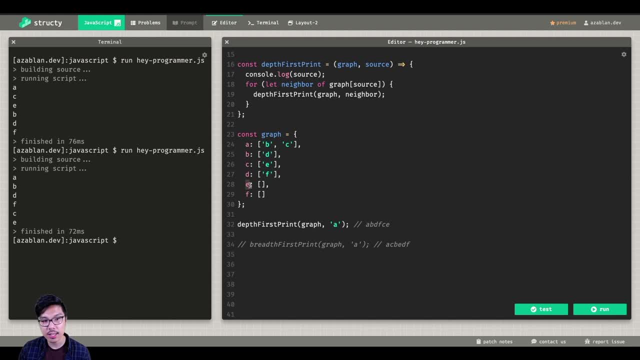 when a node like E is a dead end, right? Let's say, my current source coming in is E. well then, when I iterate in this for loop, I'm iterating through this empty array. I mean they have zero iterations. if you have zero iterations then you never make a recursive. 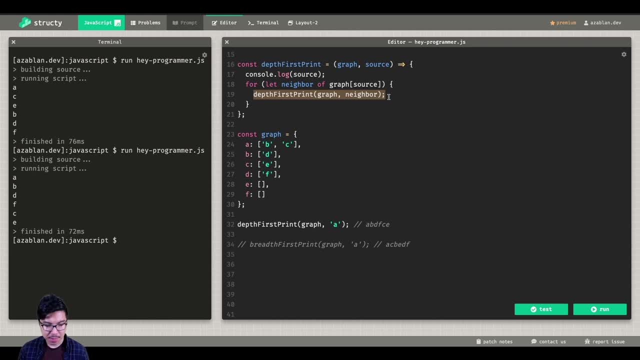 call. Right. So that's the same thing as having a base case, right. A base case is really just a scenario where we don't have a recursive call, So that's how this code still works. Alright. so now you know how to implement depth. first, in two ways: right: iterative and 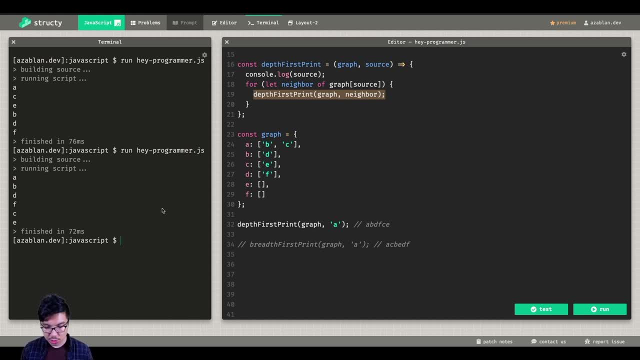 recursively, and they both use definitely a stack. Let me now show you how to implement your breath first. right, So we'll comment out some of this code Now. we'll do a nice breath first. give myself some room over here, So for a breath first. we'll want to solve. 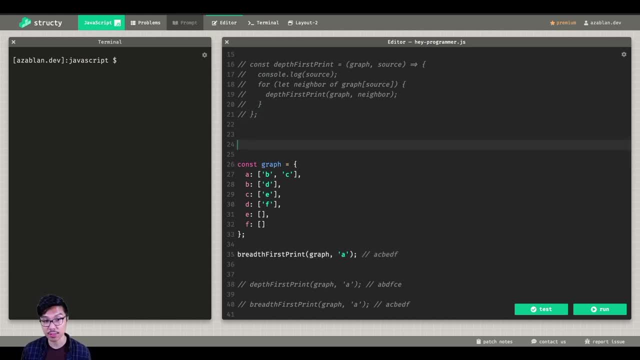 this one iteratively, And it's really only possible iteratively, right? So I know a breath first reversal demands a queue. If you try to like implement a breath first reversal using some recursion, and under the hood there's some stack data structure that's going to fight against the queue order. 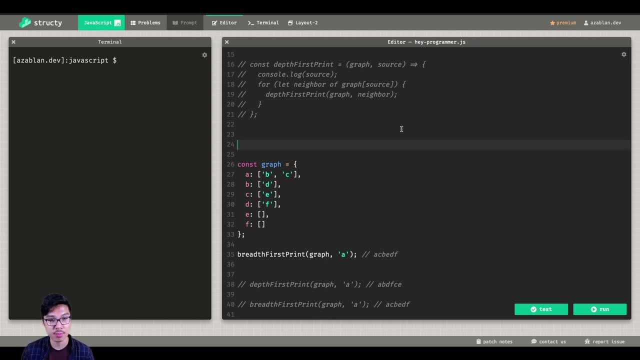 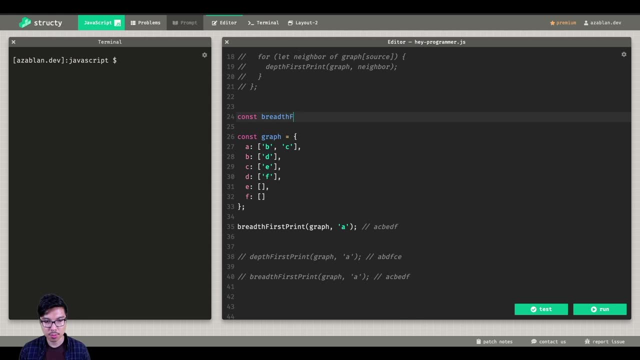 that you want, right? So for breath first reversal, you're always typically going to be writing some iterative code, So some loops, right? So we define this. I'll say: breath first print. take in the full graph adjacency list as well as the source node. So I'm going. 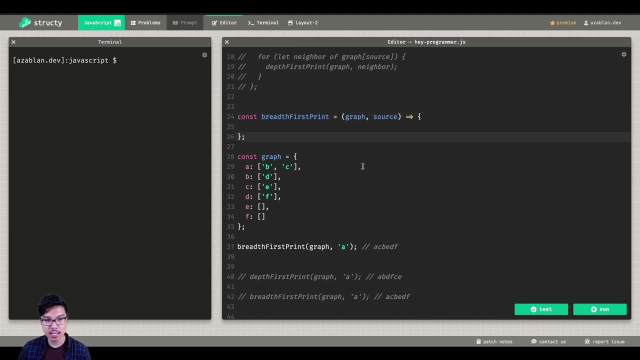 to write a new array And I want to initialize my queue with that source node. Again, the queue here is just going to be an array in JavaScript, So I'll say: const q equals an array that begins with just the source node- Awesome, And I'm going to use this queue by 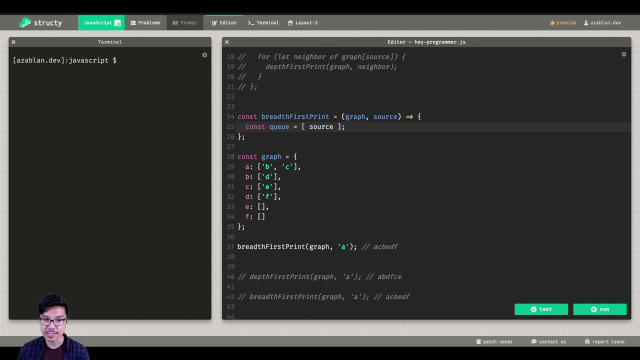 just committing to two specific methods on my arrays in JavaScript. So if I use array dot shift that removes the first element of an array, If I do array dot push that adds to the last position of an array, And using those two methods in combination, we're going. 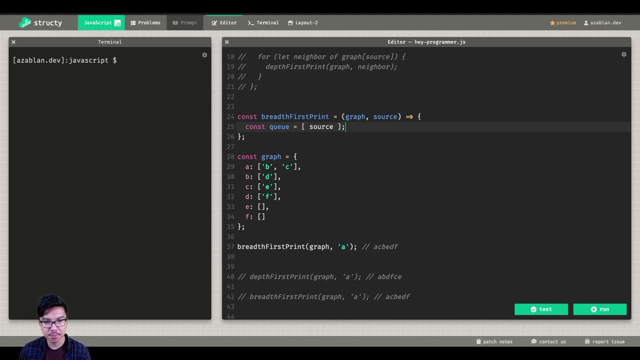 to have a nice queue where I add to one end and remove from the other end. So, like before, we're gonna have a while loop, we're going to iterate while our queue is not empty, And so while q dot length is bigger than zero, nice and same thing as our iterative you. 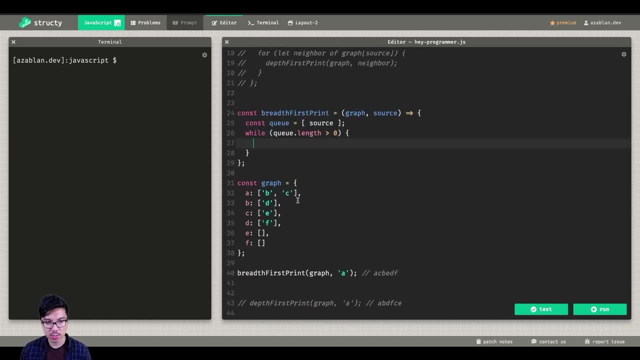 know depth. first, you want to start by just removing the front of your queue. So I'll say q dot shift. that will remove the first element as well as return it to me So I can save in a variable, like to call it current, just like the whiteboard right, And then 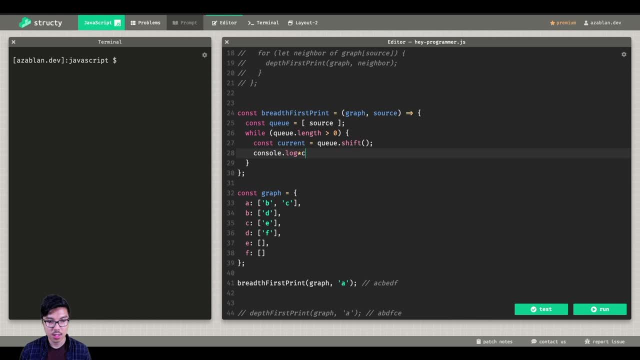 from there. maybe I'll print it out, So I'll console dot log this current node And then from here, just consider your neighbors, right? So if I key into my graph using this current node, that would give me an array of its neighbors. I want to loop through each of those neighbors. 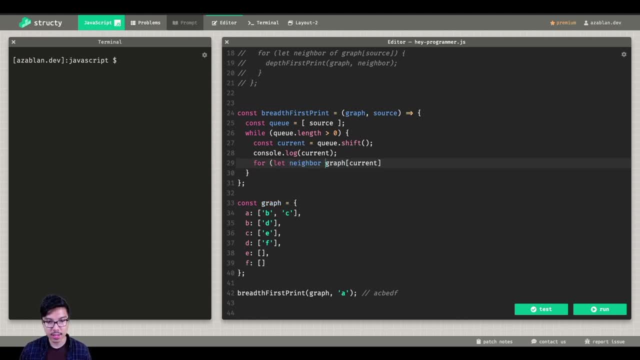 So I can say for we'll say let neighbor of that array, And for that neighbor I want to add them to the back of my queue. So for me that would mean simply q dot, push. I'm going to go ahead and push that neighbor, Awesome. So I remove from the front and I 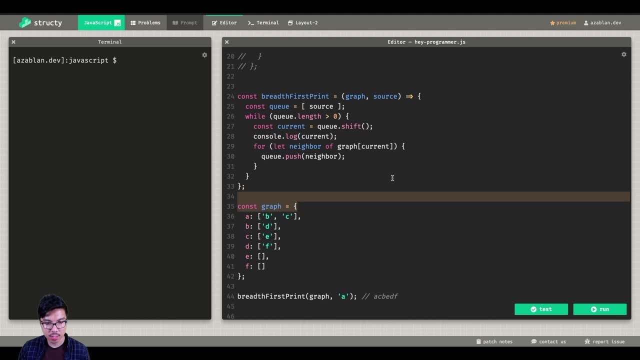 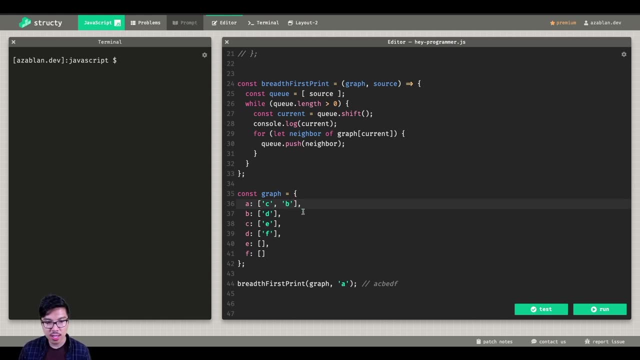 add to the back, So that looks pretty good. Let's go ahead And give it a run And actually before I do that I'm going to change the order of this. I put the C and B again. doesn't really matter the relative order for neighbors I. 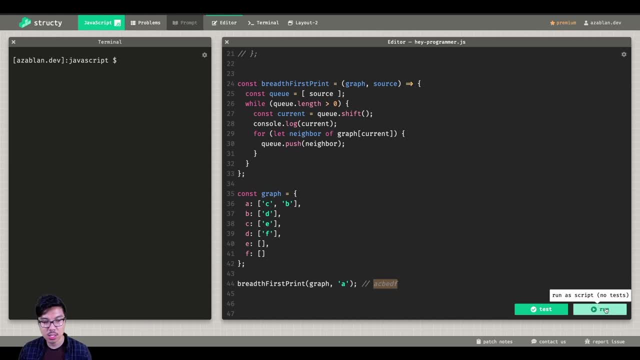 just want this exact output. we'll talk about why that is right. give that a run. So I get a CB EDF, just like I expected, a CB EDF, Right. So let's say we're on the first iteration of this breadth, first print. I know that I would have just removed a because I initialized 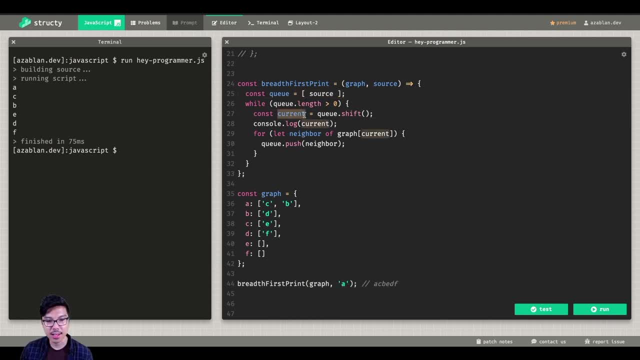 a on the queue right. So my current is a and I print out a and then from there I start iterating through this array right. So in the first iteration I have C. I have C. that means I put C into my queue right And then afterwards I put B. if you put C. 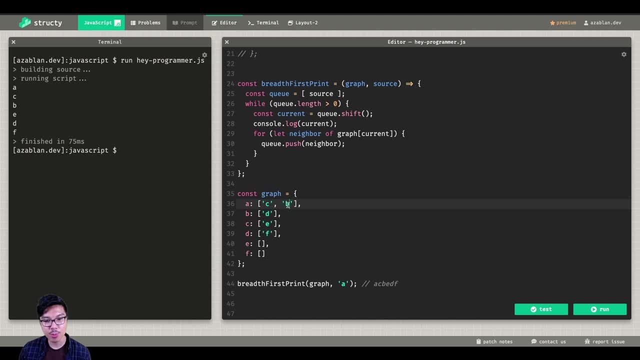 and then B. that means C is at the front of the queue, which is why on the second iteration I have C first Right. So that's how you can manipulate potentially the lateral order of a breadth first print. Awesome, And that's all there is to this traversal algorithm. 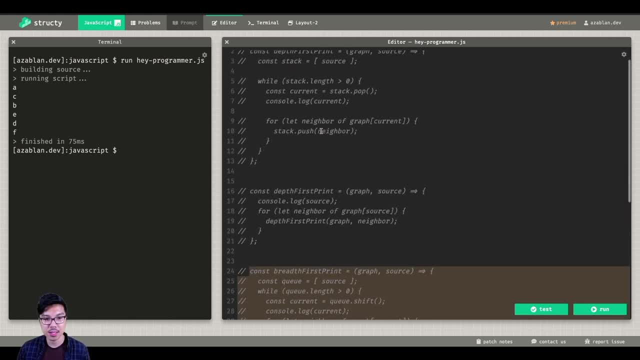 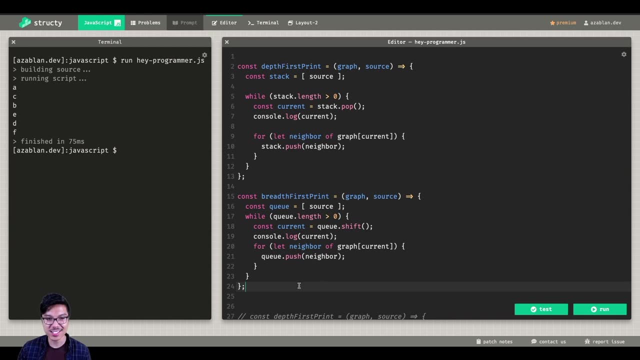 What I really want to emphasize is, especially if you look at the apples to apples iterative code. you compare your depth first First, your breadth first. it's almost identical code. you're really just changing how you access items in your array right. You either pop or push, or you shift and push, Other than. 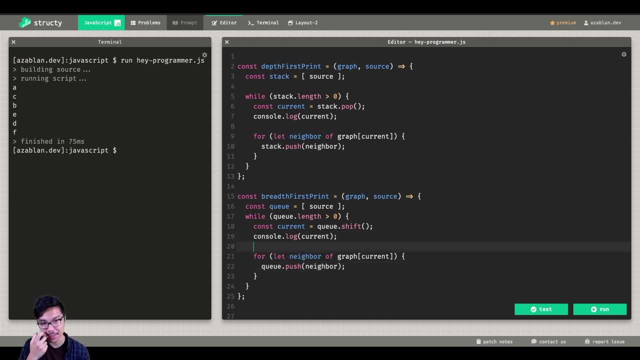 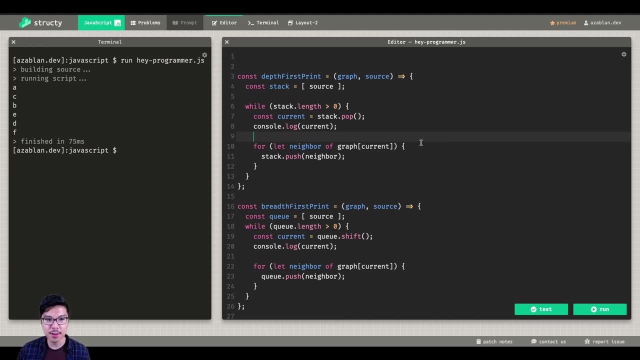 that the whole like structure of this code is identical, right? Alright, so that's our introduction on depth first and breadth first for our graphs. In the next section we're going to start to solve a problem, right, which will be really fun. I just utilizing 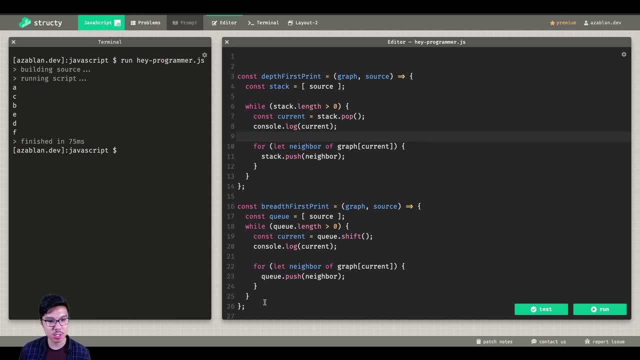 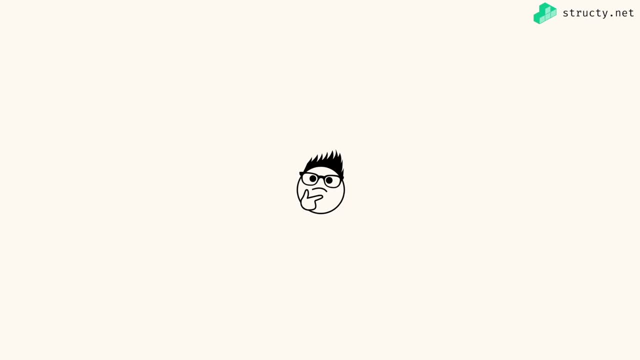 this code as our baseline tool, And in that section I also promised to start doing the analysis for big O of these algorithms. So let's jump back to that whiteboard. Hey programmers, welcome back. right, let's go over the approach, for this has path problem. So in this problem we're going to take in 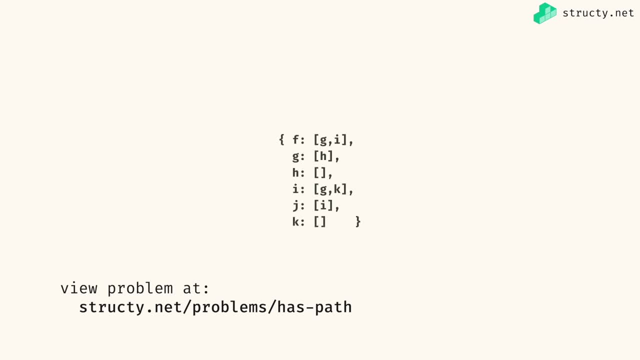 an adjacency list representing a graph For this problem and really all graph problems. you definitely want to visualize this one with a picture, And so what we'll do is we'll interpret each key of this adjacency list as representing a distinct node And, if I 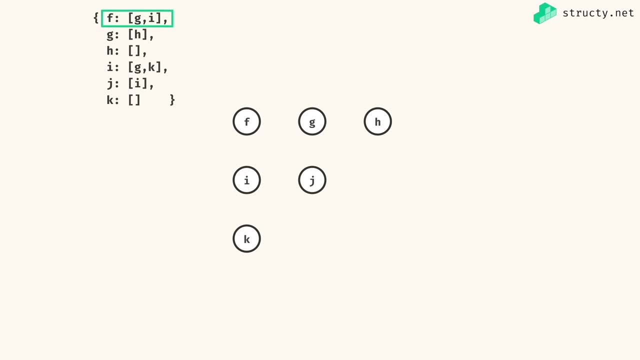 look at any particular list, I can see that this F node should point to G and I. and they do tell us in this problem that I have a directed graph, So I'm going to draw arrowheads on these edges here. So f points to G as well as f. 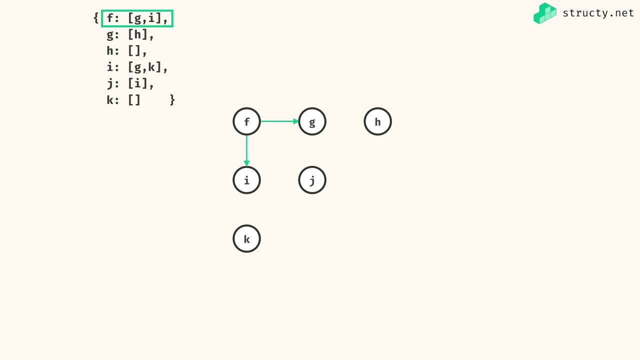 points die And I'll create similar edges based on the information in the given graph. So I end up with an image like this, And so they tell us that this is a directed graph that explains the arrowheads, But they also tell us that this graph is a cyclic. So if 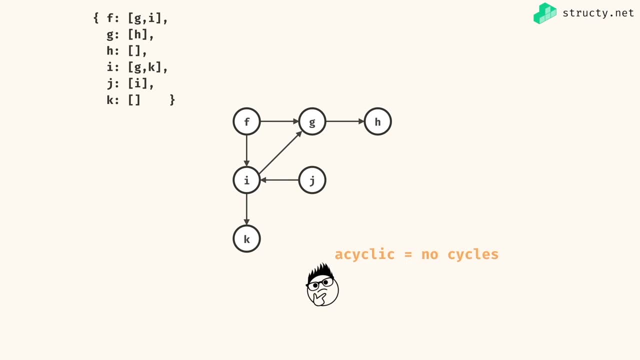 you're unfamiliar. a cyclic just means no cycles. that kind of begs the question: what is a cycle in a graph? So a cycle would be a some path through nodes where I can end up where I want started. In other words, if I started at the A node over here that I can go to B then from there. 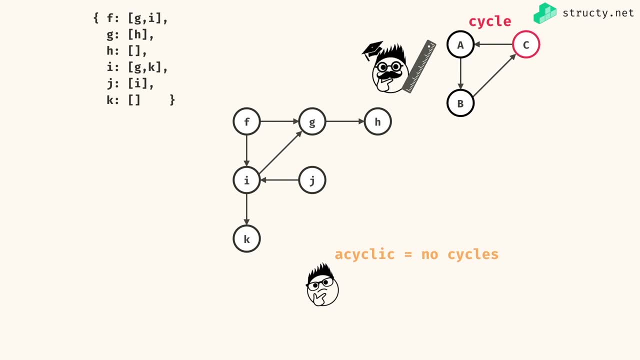 I can go to C, then back to A, and so on and so forth. So if I did a traversal on the cyclic graph I would get an infinite loop. And what they're saying is: our graph input is guaranteed to be directed, So it has arrowheads but also a cyclic, So we won't have to consider. 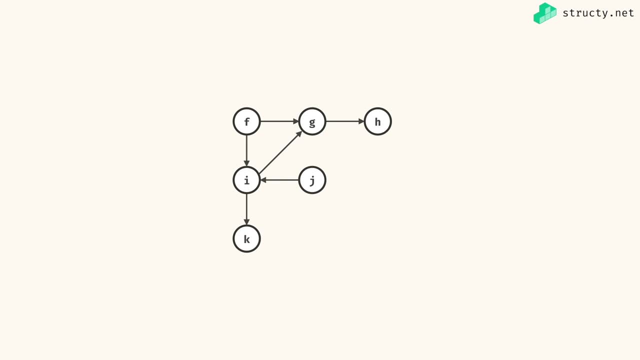 any infinite cycles here. That being said, in this problem we also want to take in not only the graph information, but also a source and destination node. What we want to do is return true or false And whether or not we can travel from the source node to the destination node, In other. 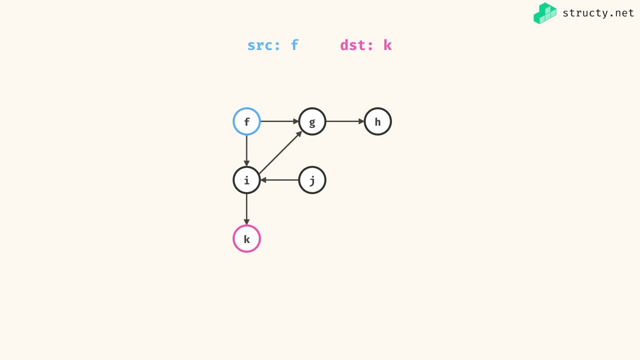 words. is there a path that exists between those two nodes For this problem? we can use either a depth first or a breadth first search actually solve the problem here. I'll trace through in this approach video just the depth first search, but in the walkthrough 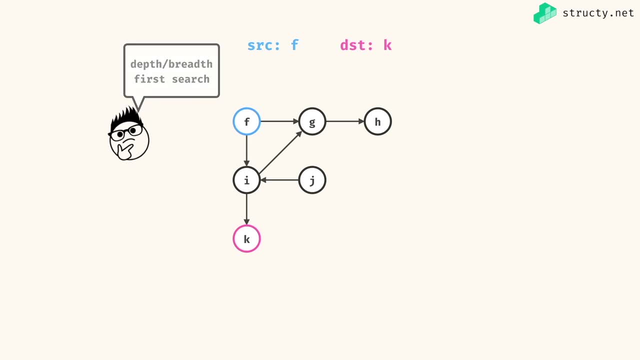 I'll be sure to code it up both ways. So let's say I started at my source node. I know that if I was doing a depth first reversal, I can either choose the IRG- let's say I happen to choose the G necks. 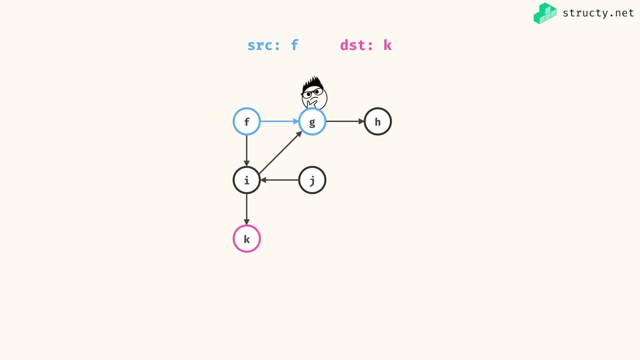 Now I have no choice, right? If I'm doing truly a depth first, I should go deeper to the H. So then I hit this H, And as I traverse through these different nodes, I need to ask myself if my current node is equal to my destination. So far, that hasn't been true At this point. 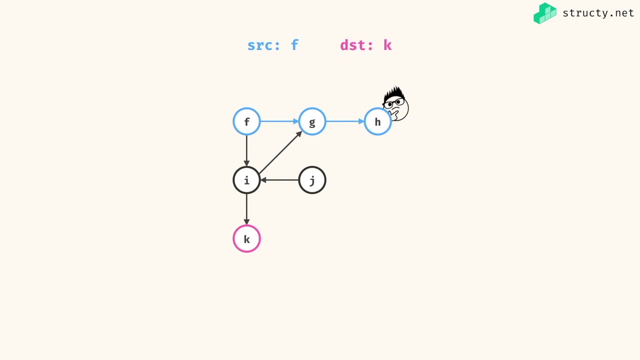 I've bottomed out with my H node. I can't travel any deeper, So now I can move laterally to a node like I. at this point from I can either move to a K or a G, let's say by luck. 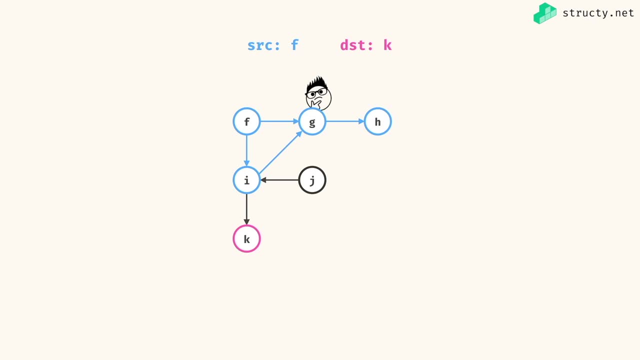 I just happen to go to the G. this would actually bring me down a path I've explored previously, which we can optimize later on. be too much of a big deal. Eventually, if I continue this depth first search through the graph, I would end up at a node that matches my destination, at which point I can return. 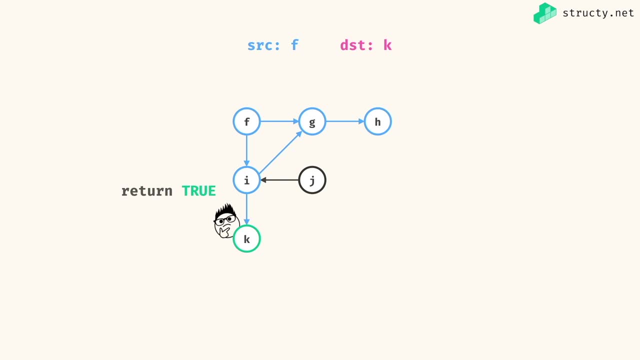 true, signifying that there must be some path from f to k, just doing a depth first search. And as we do this depth first search, it's really important that you obey other directions of your arrows, So I should never try to travel upstream. So that was a scenario where we 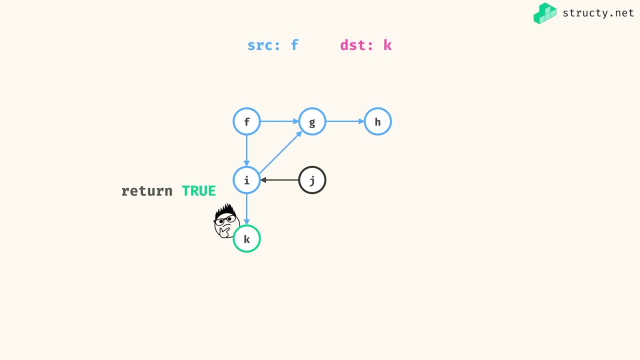 were able to find a path from source to destination. That's why we return true. Let's reset and say that now I should return false, right? So let's say my source was j. So I start at j And I'm trying to get to my destination of f. If I started a depth first reversal. 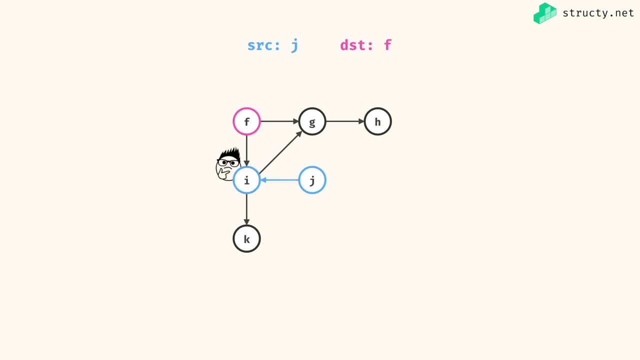 here- sorry, my J node- travel to the I node. At this point I can hit either the G or K. let's say happens to hit the K, this point of bottom now. So now I can move to the G. 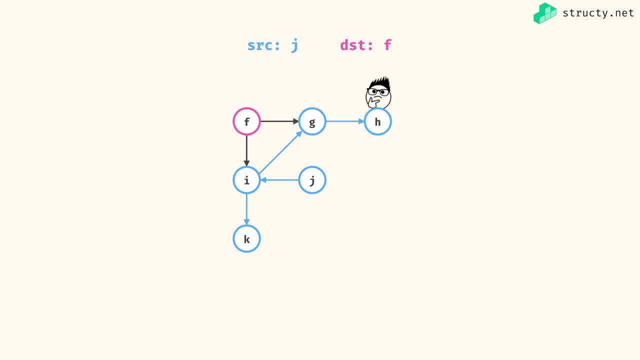 then from there to the H, And at this point there's actually nowhere else I can go right. So if I finish my traversal through the graph using either a depth first or a breadth first and I never hit my destination and I can just return false, right, it must be the case. 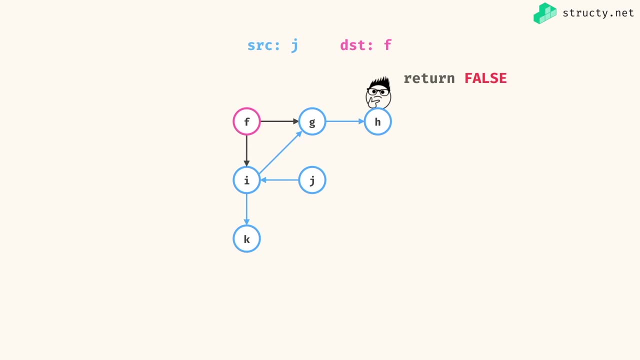 that there is no such path from my source to my destination. And when it comes to implementing the depth first and breadth first reversals on this graph, it's going to be exactly what we're used to: can either use a stack and solve it recursively, Or you can do it iteratively. 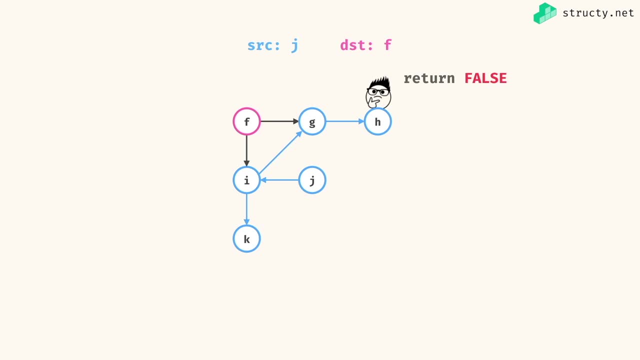 and use a queue, in which case you'd be doing the breadth first traversal. We talked about the complexity of this. let's say that n is the number of nodes of our graph. A common thing that you can also do with these graph problems is: 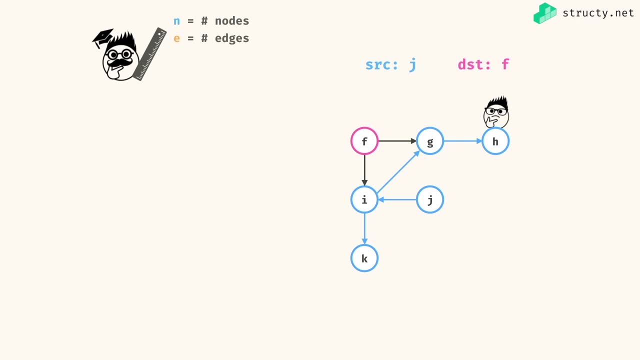 define E as the number of edges here, and edges refers to a connection between two nodes, basically just the arrows. So if we use these two terms of number nodes and number edges, we would have a time complexity of O, of E, O of the number of edges, as, because we would 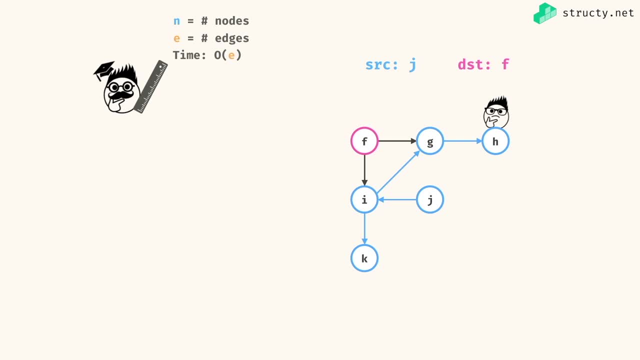 have to travel through every single edge of our graph. Here the space complexity would be based on the number of nodes, right? If I solved it recursively or even iteratively with some sort of a depth first stack, then the worst case I would have to have every 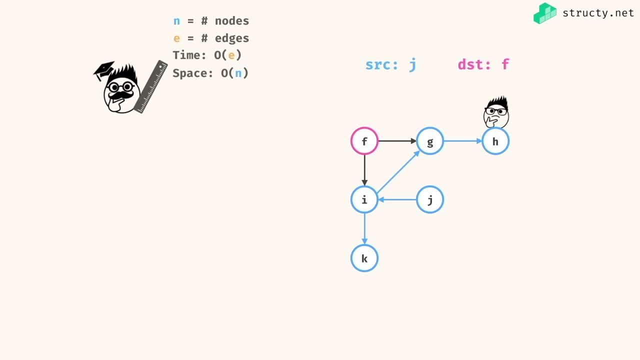 node on the stack right. Likewise, if I saw the iteratively with a breadth first, I would have every single node on the queue. So that's just one way we can define the terms for analyzing the time and space of this graph, Typically for graph problems. another acceptable way. 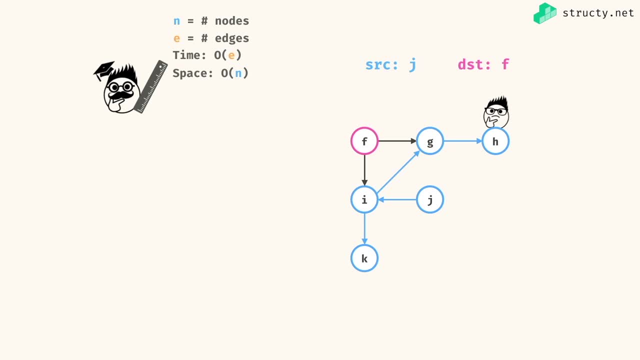 to analyze the time and space of your algorithm is to just use a single variable and just define n as the number of nodes. And that's because if you say n is the number of nodes, then we can also say that n squared would be the number of edges. Remember that big. 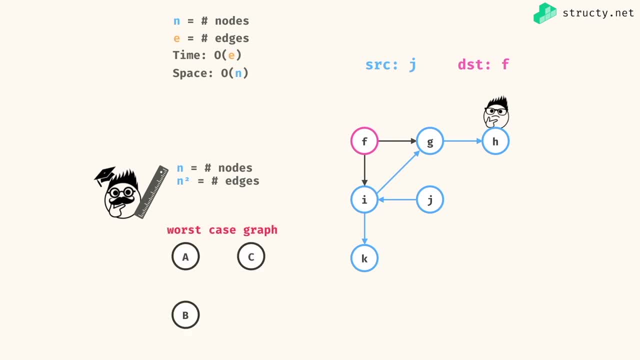 O, it's about the worst case. So let's imagine the worst case graph. let's say I just had these nodes of ABC. Well, if I wanted to create as many edges as possible, how would I just create a single edge? Well, 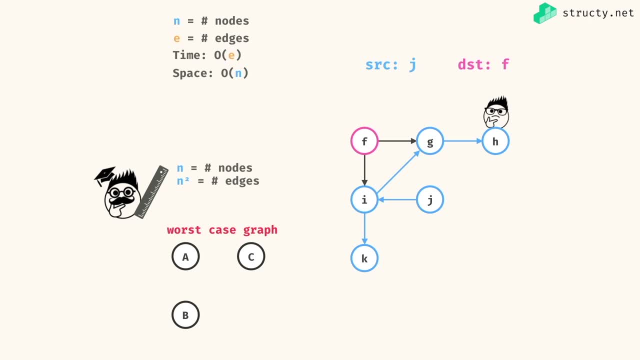 an edge is just a connection between two nodes, So you could just really draw an edge for every pair of nodes in your graph, something like this: And that's why we can say that n squared is the number of edges of any particular graph. And so if you just wanted to use n, 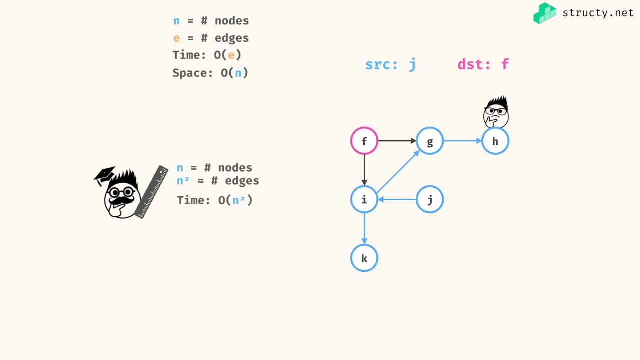 to define the complexity here. then you could say that your time is going to be O of n squared And your space complexity would still be O of n. do note that these are both two valid ways of for defining the complexity for a very typical graph problems. That being said, 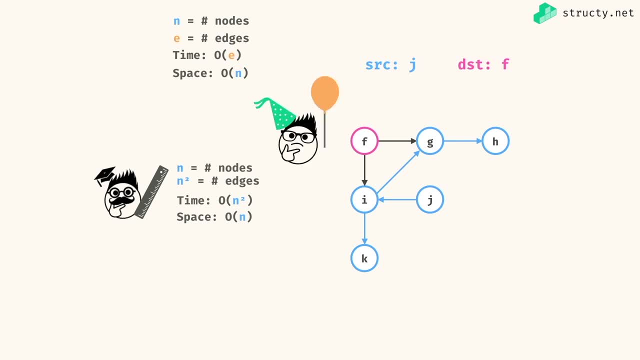 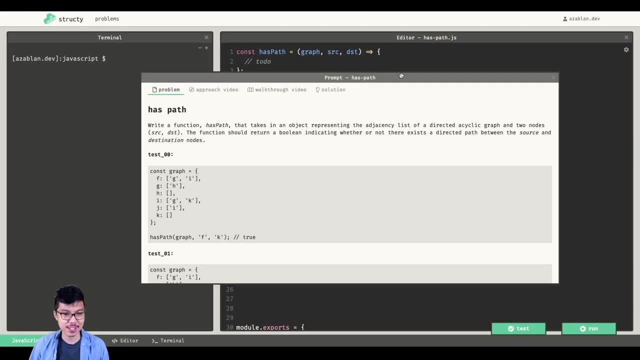 I think this is pretty straightforward. Let's hop into the walkthrough video where we're actually implement both: a depth first, any breadth first. solution for these. I'll see you there. Hey, programmers, Alvin, here Right now, let's go over a JavaScript solution, for this has. 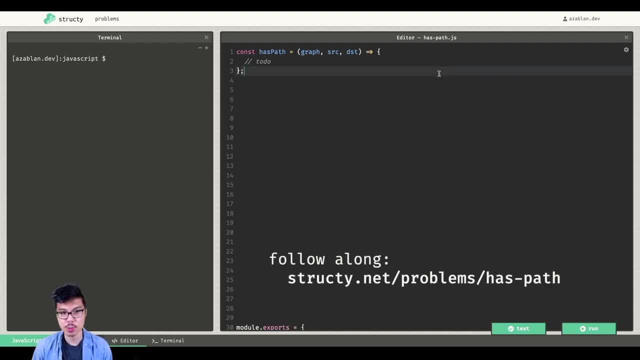 path problem, And so we'll jump right in. we're going to start by solving this one using a depth first reversal, which I know requires some time, But there's a lot of things that require some time right, So I'm going to show you a little bit of it, But what you should 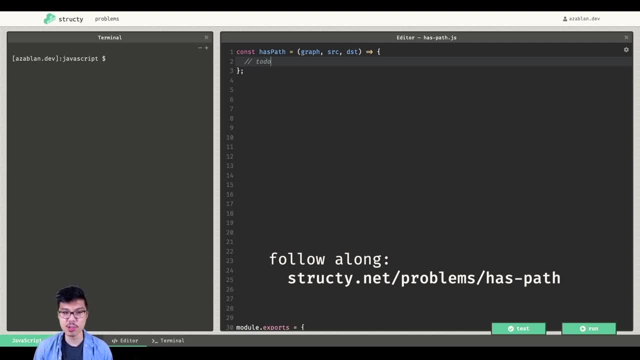 require some underlying stack data structure. I'll just implement it using recursion So I can leverage the call stack to get my ordering, And so I'm going to solve this recursively. I'm going to consider my source argument as like my current position during the traversal. 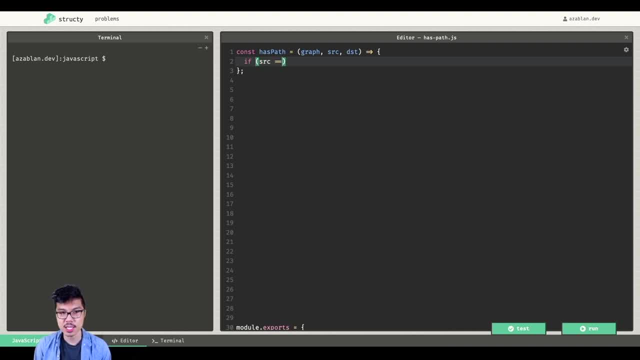 And so I can have a base case in check. alright, if my source is equal to my destination, that I must have found the thing I'm looking for, So just return true. this base case signifies that I found my destination, So there must exist a path, And so I return true always. 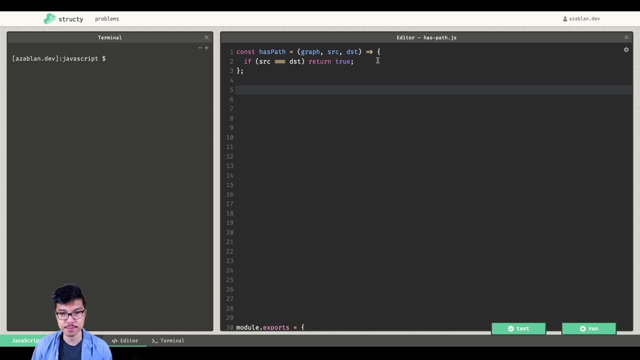 paying attention to the type that they want us to return for this function. Let's say it's not true. well then, I need to keep looking. So what I should do is consider my current node, which is source, consider its neighbors. If I key into my adjacency list, I know that 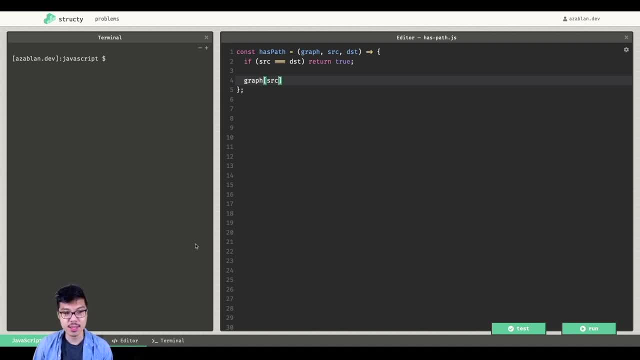 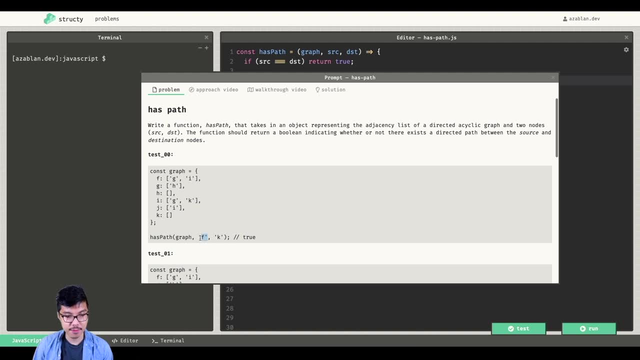 this is going to be an object. So if I key into it using my source, that would give me an array of all of its neighbors. So for example- let's say I was staring at this one- if my current source was F and I say graph square, bracket F, I would get back an array of G. 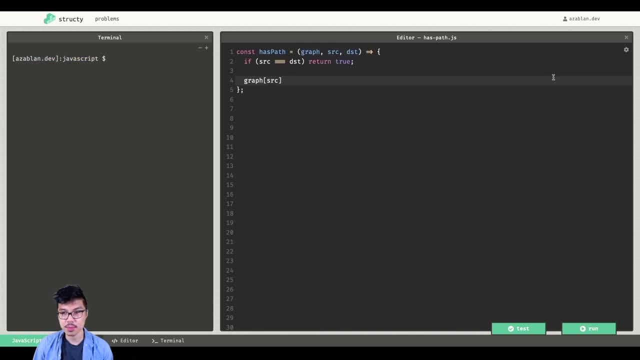 and I. So now I want to look through the neighbors right, So I can say over here is turn this into a loop and say, for let neighbor of those neighbors I want to traverse to them, which means I call recursively or I call has path. keep your graph the same, but update your current position. 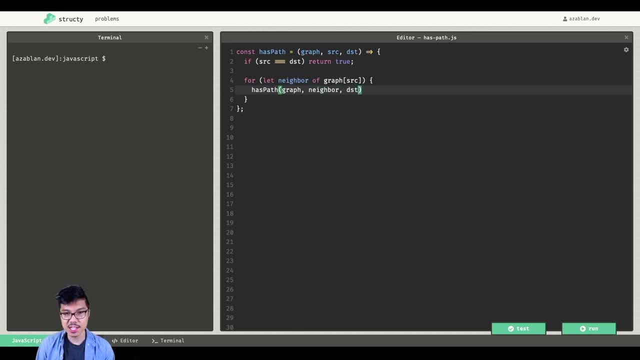 Now I'm going to be situated at the neighbor And the destination stays the same. I always have the same goal: to get to solving this one recursively. So think about what type this is going to return. I know it's going to give back boolean right. It's going to tell me whether or not there is some path between. 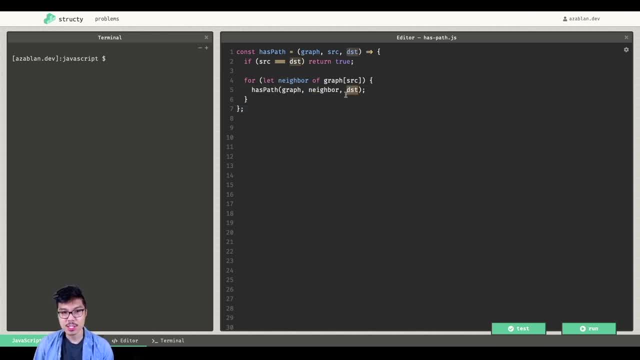 my neighbor and the destination, right? So if there's some connecting point or some connecting path between my neighbor and the destination, then I know that there must be some path from my source to the destination, because your source is definitely next to your neighbor, right? So there would be a path between all of us, And so what I'll do? 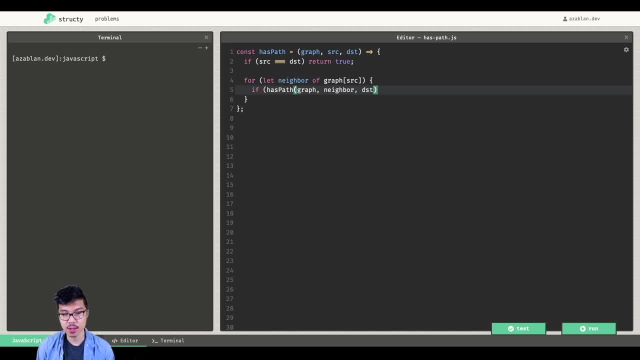 is check. if this recursive call returns true. I'll make it explicit here. maybe it's clear. And so if there is some path through my neighbor to the destination, then I can return true. just pass that true upward, Because once I find a path you can just exit out and return. 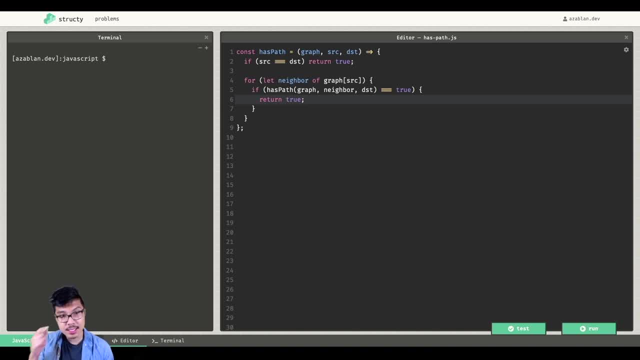 that true, all the way back to the top level caller. But let's say that this call returned false. that means that there is no path through my neighbor to the destination. But it could be the case that some other neighbor is actually going to work out, And so what? I don't want. 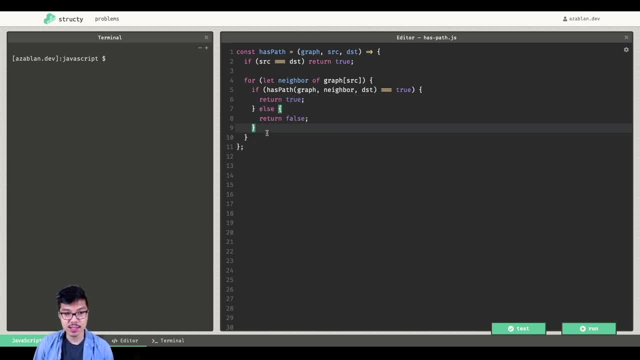 to do is just say like: else, return false. you should be able to immediately catch that code like this is suspect, because there's no point of having a for loop, then right, If in either case you're always going to return, then you're never going to have a. 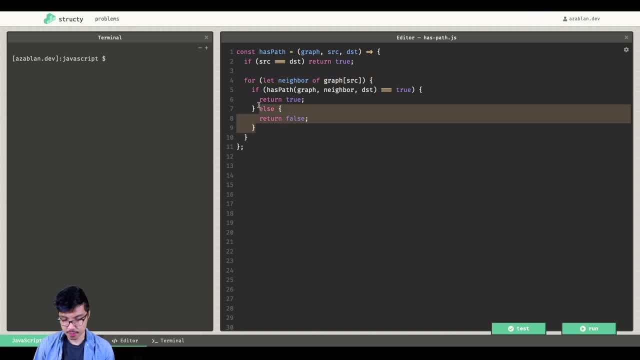 second iteration of this for loop right. So if I don't find a path through my neighbor, so if this call returns false, then that's okay, just continue on to the next iteration and search through your other neighbor. That begs the question: where should we return? 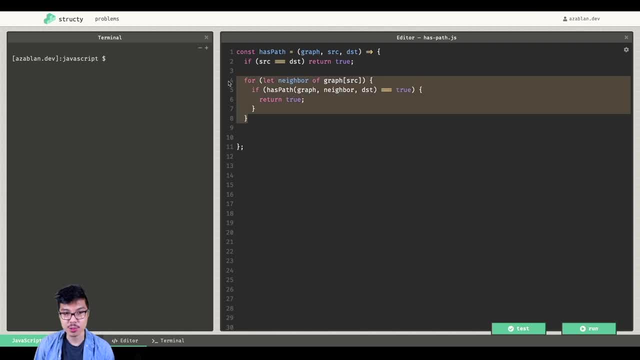 false needs to be after the for loop. So only after I searched through all of my neighbors and I never find a winning path, Should I return false. that would be our nice depth first reversal. Let's give that a test run, Awesome. 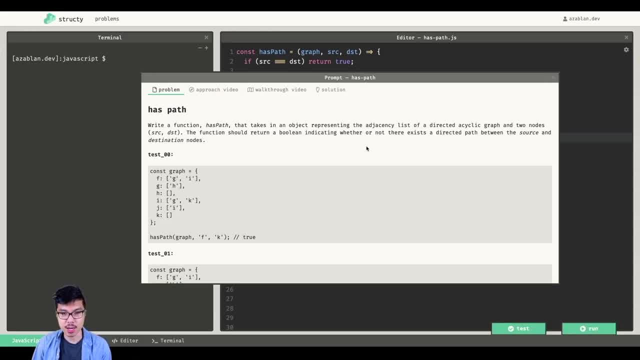 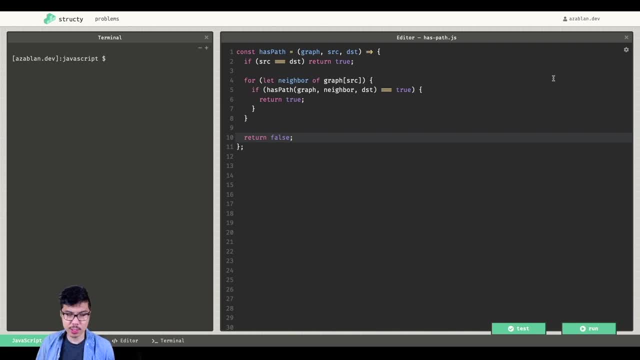 There we have it. One thing to bear in mind: here we are leveraging the assumptions in the problem right to tell us straight up that the graph you're going to be given is a cyclic, So there are no cycles. So that's why in our code, we didn't really worry about. 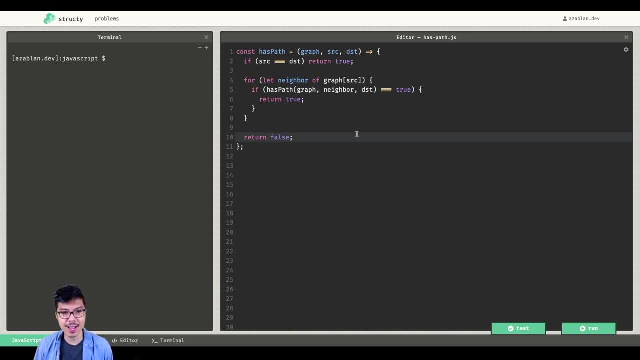 getting trapped in an infinite loop. In our upcoming problems we'll have harder graphs that actually deal with that cyclic case, But for now this is a good baseline solution. While we're here, let's also do a breadth first solution, which you know we're going. to call itotojadadamn right, because it's a really good way to do that nearest to everything. And so what I'm going to do here is I'm going to call it to the library strong index And, as you can tell, it's going to be a no by now should be iterative right. there's no way. 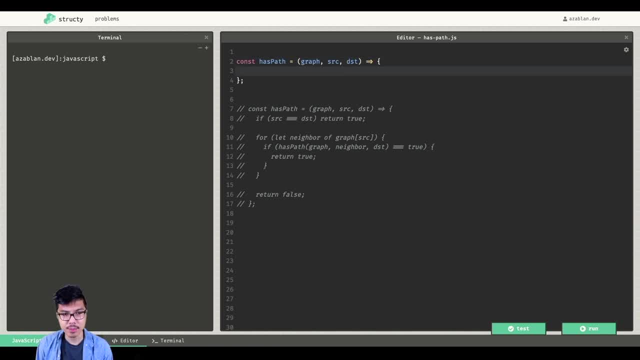 to do like a breath first recursively, And so I need to create my own queue. So I can create a queue kind of in a pinch, I always just use an array in JavaScript. we're going to initialize that queue with my source on it, So I'm going to refer to like source and 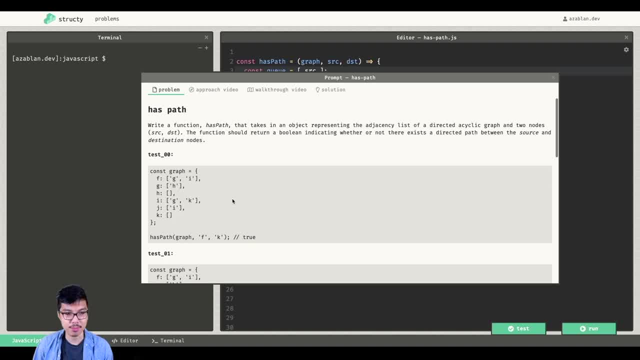 destination. they're really nodes, But in the context of, like our problem, they really just given us strings, but they represent nodes, right? So think about the information they represent. I'm going to iterate while my queue is non-analogical, right, so I'm going. 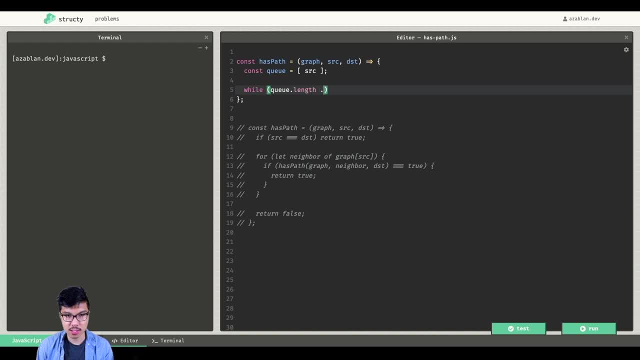 going to iterate while my queue is not empty. So while q dot length is bigger than zero should be familiar code, very similar to our tree algorithms. And I start a single iteration of breath first by removing the front of my queue So I can say q dot shift, so move the. 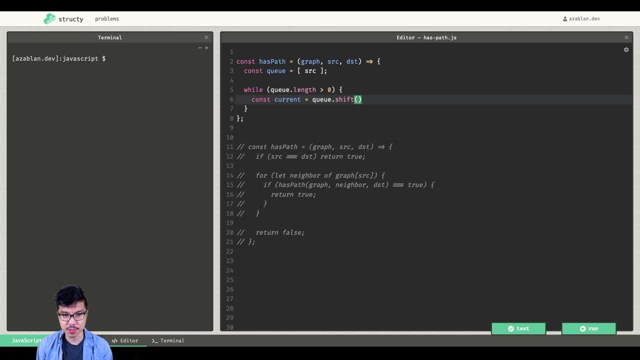 front. I can call that my current node that I'm traversing through And now that something has left the queue- typically here is where I check- I can check. alright, if that thing I just visited, if that is my destination, then I can just return. true, right, I found. 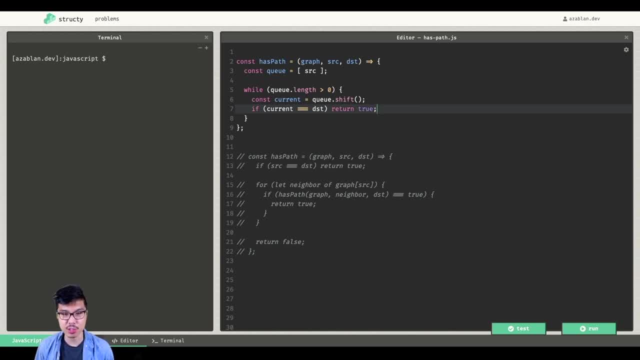 the thing I'm looking for. So there must be a path that connects my original source and my destination, Nice, But let's say this was not true. well then, I need to consider its neighbors. So, like before, it's like at the neighbors. just key into your graph using 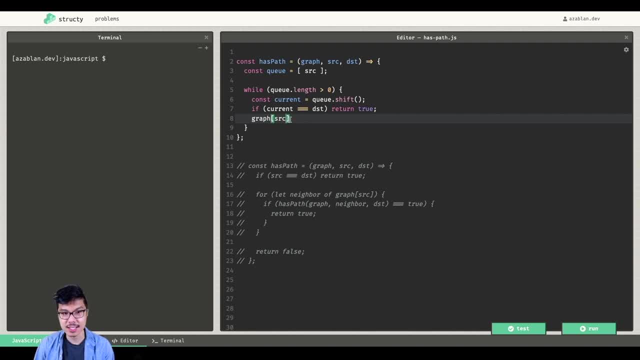 the source. I can say graph, square, bracket, source. that gives me an array of all of the neighbors, all the neighboring nodes. So what I want to do here is iterate through every neighbor over there And then I can just add them into my queue. So q dot push. 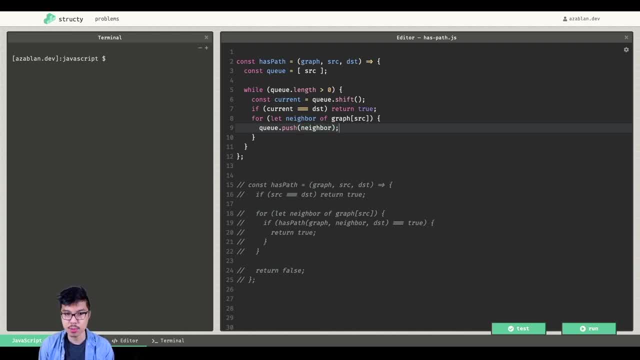 that single neighbor and do be sure to implement your true breadth first. So you need to make things: leave from one end of your queue and you add to the other end So this codes looking good. So you should realize how similar this is to our old, like binary tree breadth first. 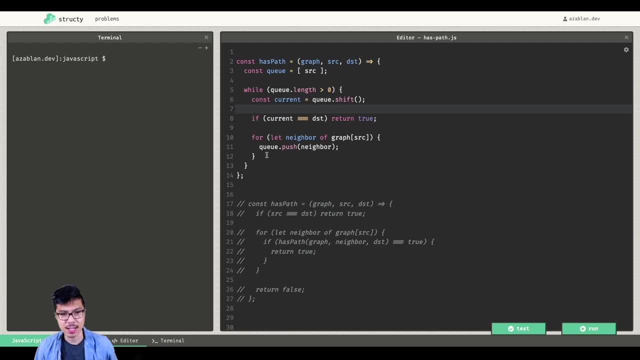 except now we have to account for the fact that we could have like a dynamic amount of nodes. So I'm just iterating through all those neighbors and adding them. I need a way to return false. and you guessed it. the move is after you finish this entire while loop. if your queue 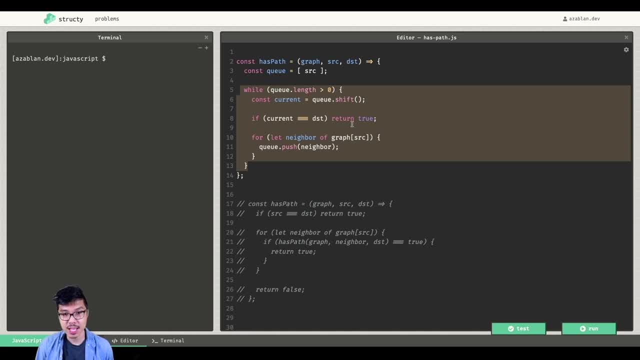 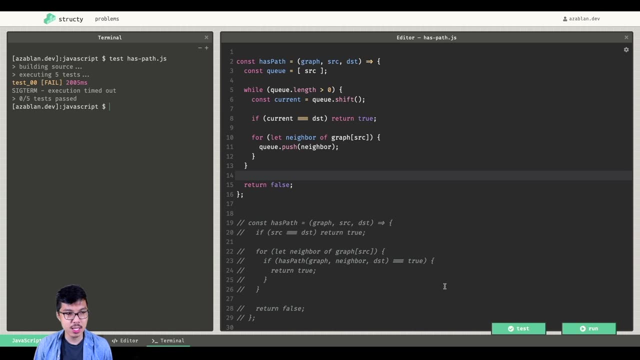 becomes empty, then you must have explored as far as you could, And if you never returned true, then now you can return false, because it must be the case that there is no path between the original source and your target. So let's give this a test run. We'll have a very similar time and space complexity. 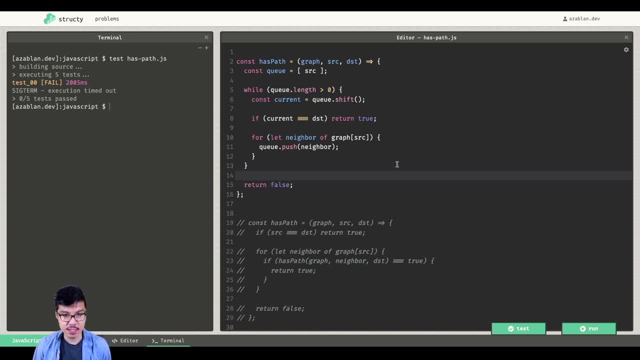 This would be the code for all of my iterative fans, So you're getting a little error. Let's see what we did wrong here. So it looks like I timed out here. Let's debug this one together. If I had to guess, that means I did something wrong, getting trapped in an infinite loop. This: 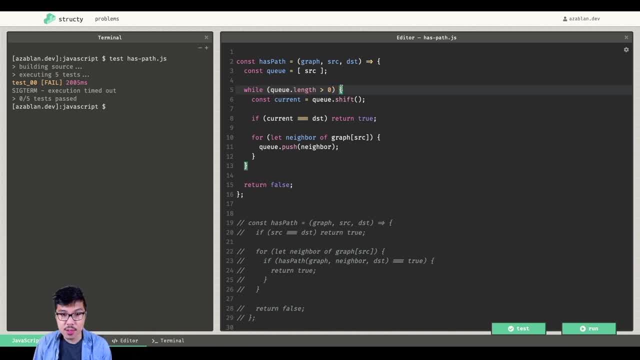 condition looks okay, right. q dot length greater than zero. And so here it is. must be the case that I'm not correctly iterating through the neighbors here. I just wrote source. Instead I need to say current, because now I'm doing this iteratively, right. 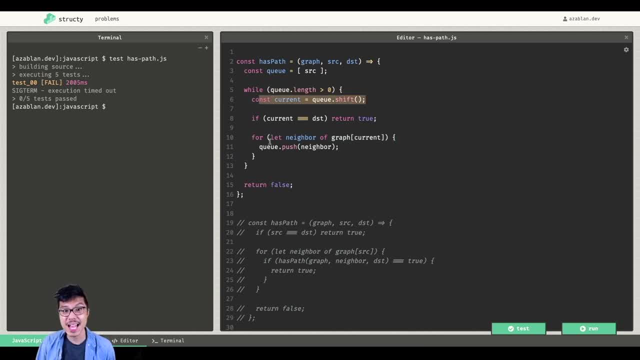 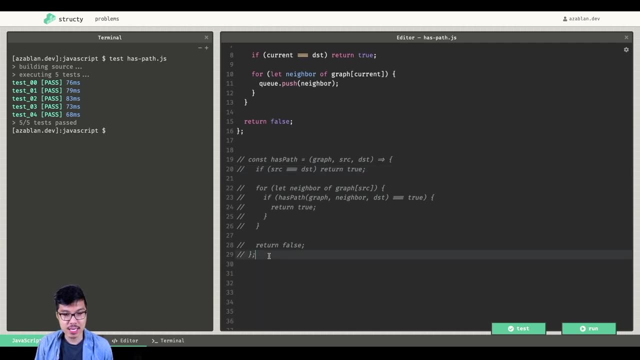 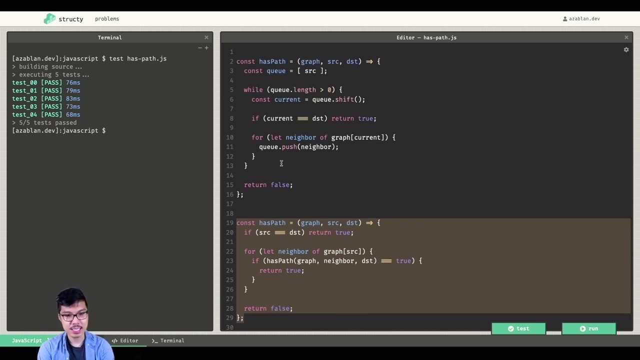 So whatever node has just left my queue, I consider that nodes neighbors and add them to be visited next through my queue. So let's give that test run algorithms now, while the problems are relatively easy. So practice this, give it a shot on. 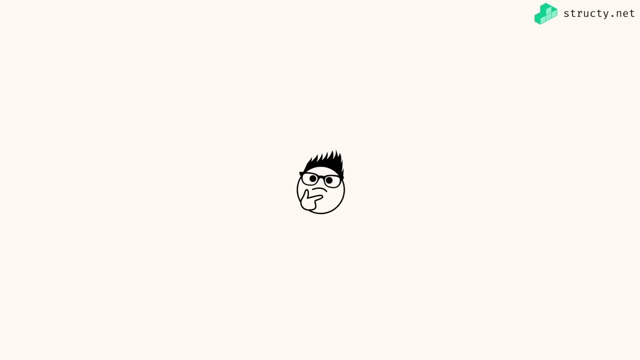 your own And I'll catch you in the next problem. See you there. Hey programmers, Alvin here right now let's go over the approach for this undirected path problem. So we'll jump right in In this problem. we're going to be given an edge list for a undirected graph. So if 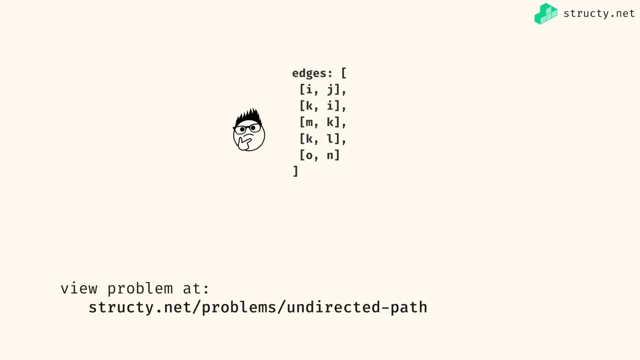 you're unfamiliar with the terminology here. really, what we're saying is, every pair in this edge list represents a connection between two nodes. For example, if I look at the first edge in the edge list, I see i comma j. that means that there's a edge or connection between. 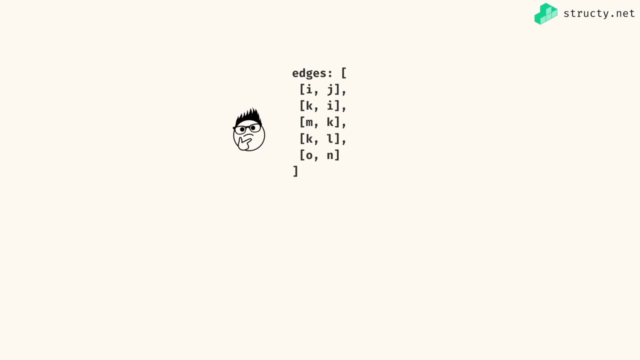 i and j, And since this is an undirected graph, not only can I directly travel from i to j, but I can of course move from j to i, So it really represents a connection in both directions. And so, as we start to attack this problem, I want to do is actually convert this edge. 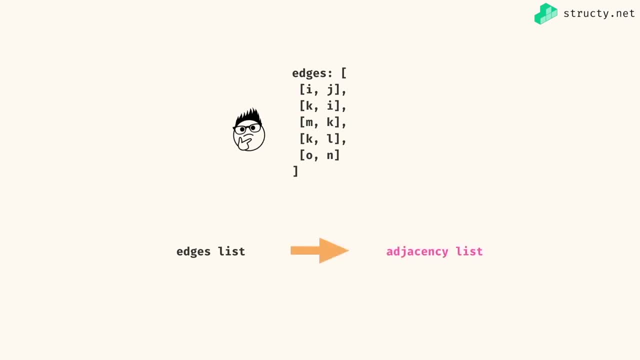 list into a more favorable format like an adjacency list. That's because typically, when we perform our traversal algorithms, they work best on an adjacency list form. So let's start by doing that conversion Here. I'll actually be pretty easy to code up, So I want to basically generate a graph. 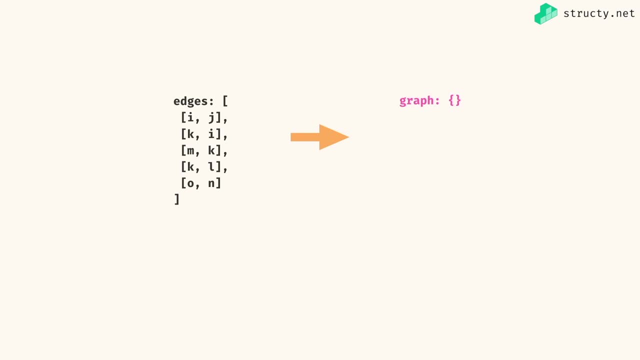 where I have nodes as keys and I want them to point to an array of their neighbors. For example, if I wanted to convert the first edge into an adjacency list form, what I can do is create keys for i and j. I know that i is a neighbor of j and also j is a neighbor. 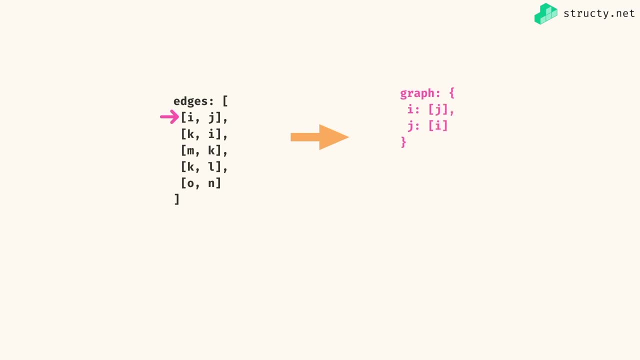 of i, So I'm going to populate those neighbors respectively. Now just follow this process for another edge. So if I look at the edge k, comma i, I'm going to populate those neighbors respectively. I need to create a new key for k and I'm going to populate that with. 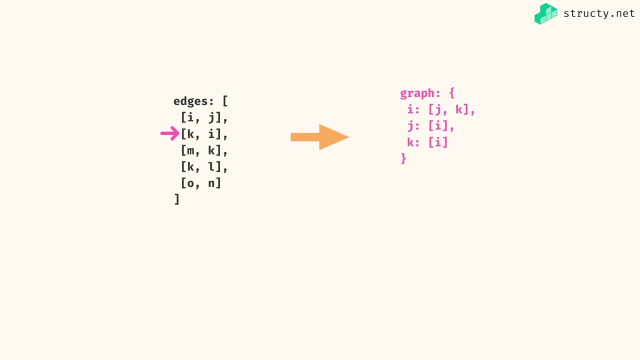 i and then for the existing key of i, I just add k into that collection. So do bear in mind: the most important thing about this conversion is because we know that the graph is going to be undirected whenever you put a connection within your graph. make sure. 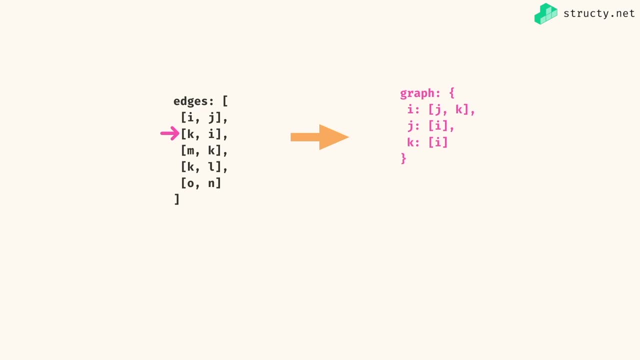 that you have the inverse connection. So if I have an edge from k to i, they also need to have information for i to k, And this process would just continue for the entire list of edges. So at the end of this conversion we'll end up with an adjacency list, just like this. 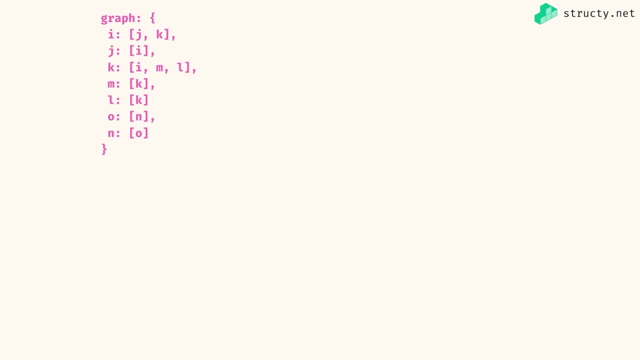 And now we're ready to perform our main algorithm. When we go through the code walkthrough for this, I'll show you in depth how you can actually create this adjacency list. And so when we want to actually come up with a traversal algorithm to solve a graph problem, it really 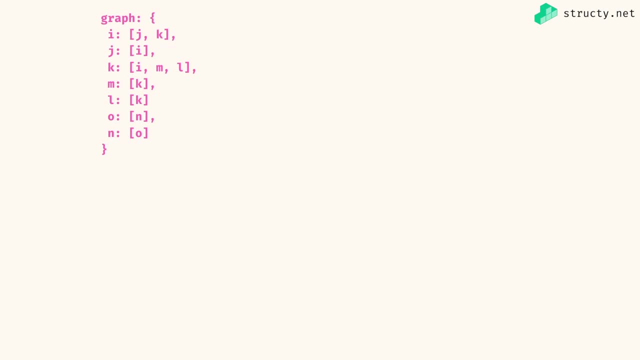 helps if you actually visualize the shape of your graph. So I actually want to visualize this in terms of nodes and edges, So that means a bunch of circles and lines between them. So if you drew out a nice picture for this graph information you would end up with. 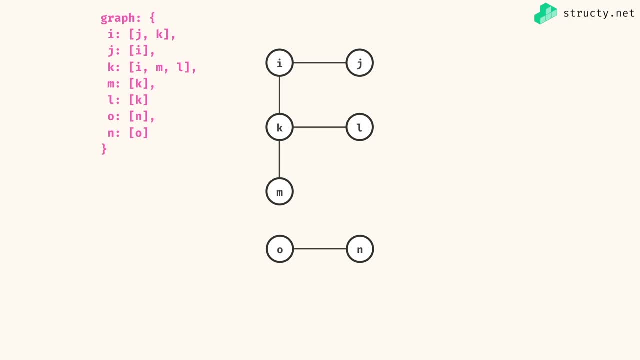 a diagram. So I'm going to go ahead and create a graph with this graph And I'm going to create a diagram like so, And so we'll go through the rest of this approach video just referencing this diagram. Something important I want to bring up at this point is for this: 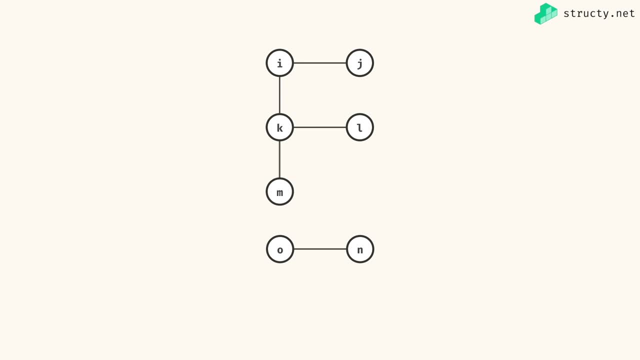 graph. a very common case you'll have to handle is what if your graph has a cycle, And that's especially true for your undirected graphs. And so, just for the purposes of this approach video, I'm going to add an additional edge, just so we can talk about an explicit cycle. 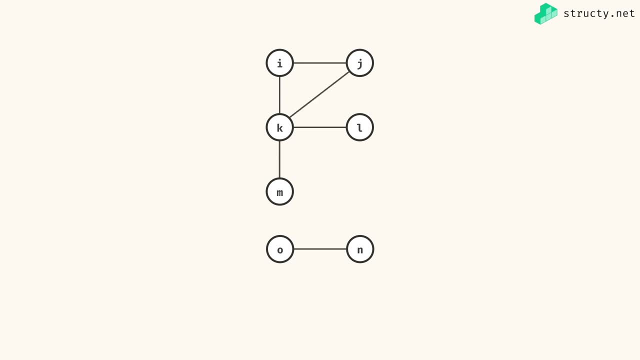 So I'm going to add one new edge from k to j. Cool. The reason is now there's a nice big cycle of length. So let's just say I have a cycle of length three, highlighting in red right now, And this cycle is important to watch out for Because if we don't do any special handling, 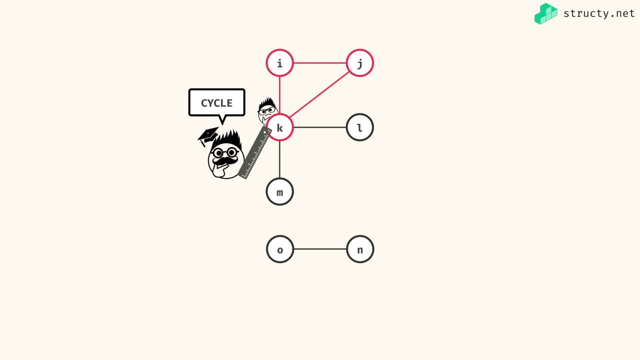 we may get trapped in an infinite traversal. So imagine I started at this k node And next I moved to j, then I would move to i and then back to k, and then back to j, and then i, and so on. So that would give me a cycle. we'll have to guard against that, And so I can have. 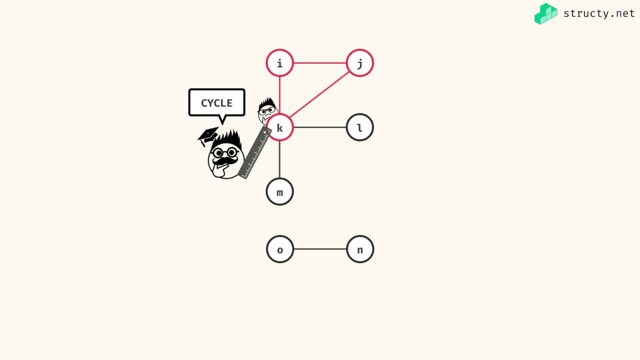 a cycle of three nodes here, right, And you can really have a cycle of basically almost any size as long as it's more than one. So, for example, if I took a look down here, I'd still look down here. notice that my graph actually contains, technically, like two separate. 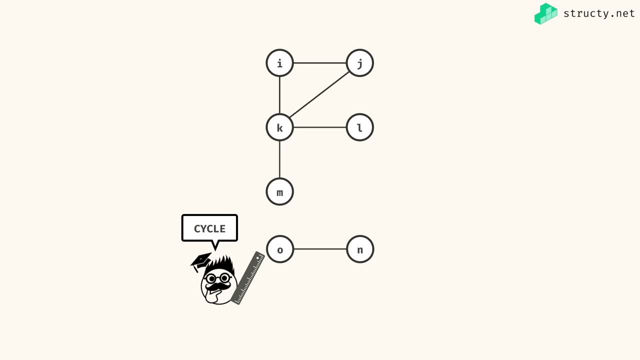 islands, But we would consider them as just one giant graph, right? So if I look at the small island of o and n, they actually form a trivial cycle, right? If I start a traversal at O, from there I can move to n. And because I know that the edge between o and n is bi, 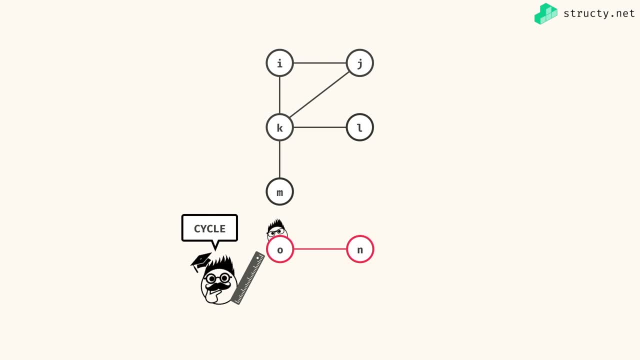 directional right. It's an undirected graph. That means I can travel back to O and then back to n, And this would give me cyclic behavior. So I have to watch out for all types of cycles In this problem. So in the context of this problem, not only are we given a graph, we're 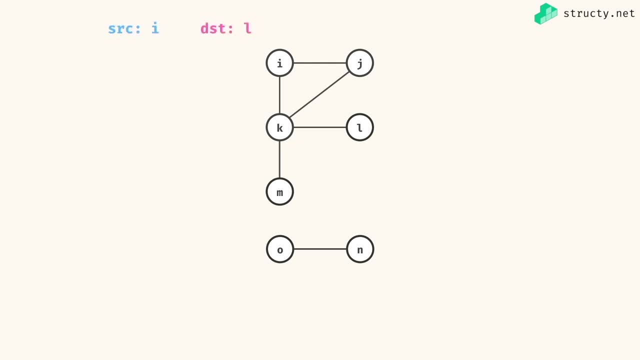 also going to take in a two nodes. So let's step through an example where I want to return true or false. is there a path between i and l? So I'm going to mark those in my graph visual. So I'm going to start at the node of i And to solve this one you can use any. 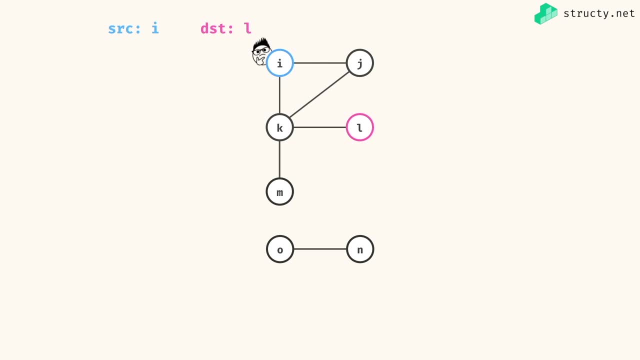 type of traversal. So either depth first or breadth first. I'll step through explicitly the depth first reversal right now, in order to avoid any infinite traversals. I want to mark my nodes as visited as I travel through them. So not only do I situate myself at this source node of i, but I'm going to mark it as visited. 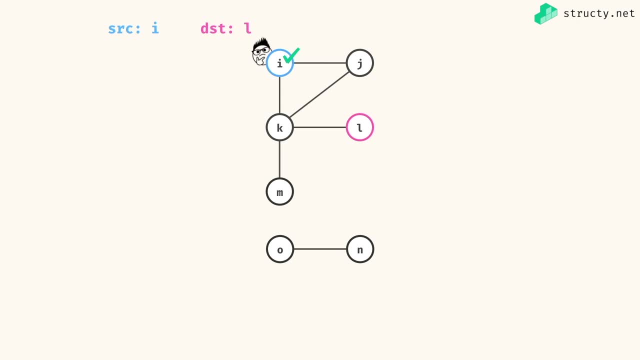 And you can implement this, like marking a visited pattern, in a few different ways. When we code this up later on, we're probably going to use a set to represent what we have visited, But for now I'll just check them off in my diagram. And so in my diagram, if you see. 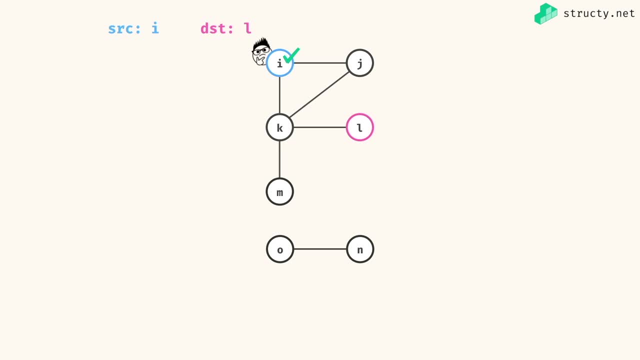 a checkmark next to a node, that means that I already have visited it. So since I'm at this node of i, I want to move to its neighbors. So I'm going to move to the neighbor of j And I'll also be sure to check it off as visited. At the end, I'm going to move to the neighbor of j And I'll also be sure to check it off as visited. At the end, I'm going to move to the neighbor of j And I'll also be sure to check. 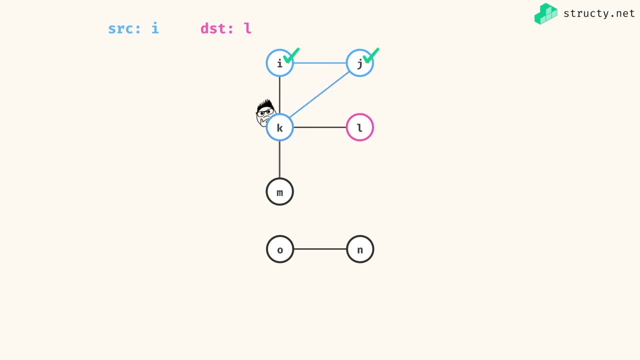 it off as visited. At this point I can move to one of Jay's neighbors. let's say I moved to K and I'm also going to mark it as visited. Now that my K, I can move to a few different neighbors. I could either move to I, L or M. let's say by chance I chose I And once I 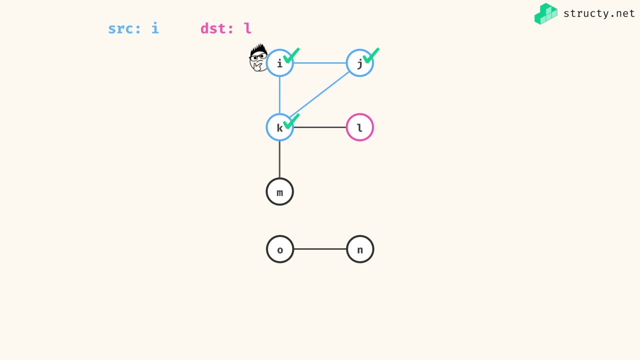 get to this I node, I'm immediately going to be able to see that, oh, I visited this node previously, So what I should do is not travel through I again. instead, I should go back to the K right, because this I node is already visited And that's where I actually 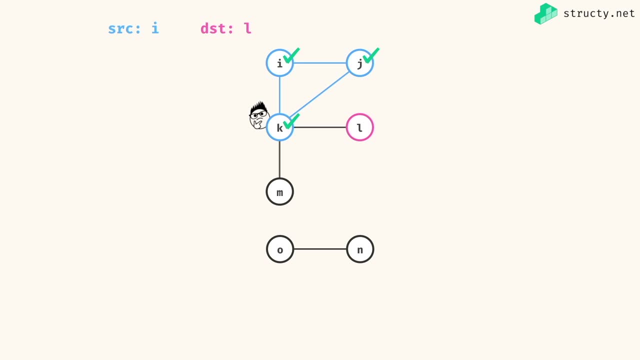 avoid the infinite loop. So instead I move to some of K's other neighbors. let's say I chose the L At this point I would mark it as visited. If I do a quick check I can see that this node- I'm at L is. 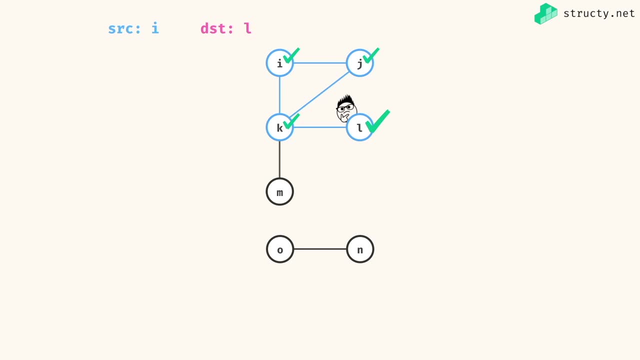 also my destination node. So I must have just found a path between my source and the destination. So at this point, if I find my destination, I can just return true, which is a pattern we spoke about in a previous problem. The only additional criteria we need is to mark: 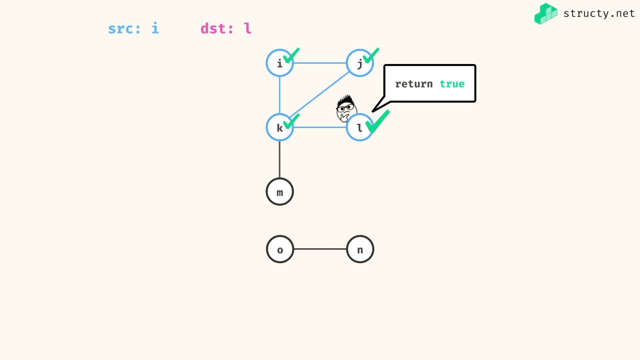 nodes as visited. That way we don't get trapped in an infinite loop, And that's only going to be needed if we have cycles in our graph which, if they don't give us any assumptions, we should always guard against. So let's take a look at another example. Let's say I had 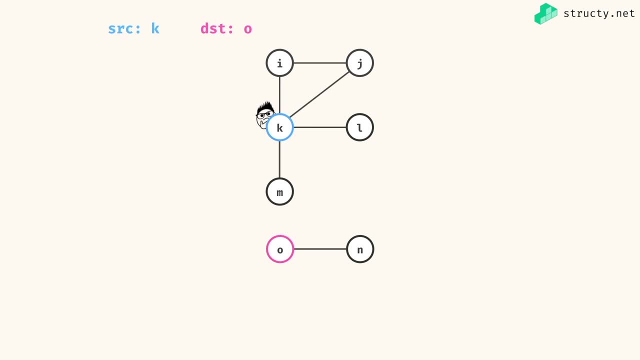 a source node of K and my destination was. oh, just looking visually in the graph, you can already see that there's no way to get from K to O because they're disconnected. right, They're on separate islands, But let's step through the algorithm regardless. So 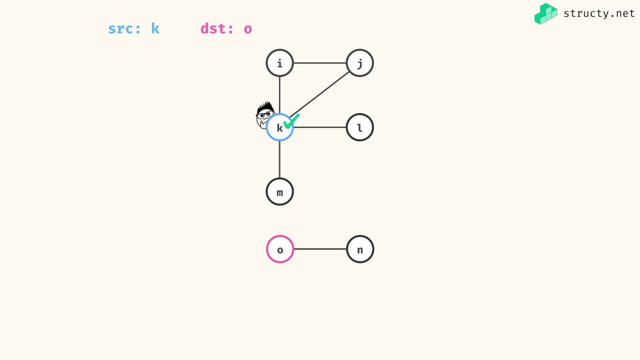 I'm going to start at K. I'm going to mark it as visited. I'm going to visit some of K's neighbors, So I can move to I, then I can move to J And then, at this point, I would move back to K. So I'm going to move to I, then I can move to J And then, at this point, 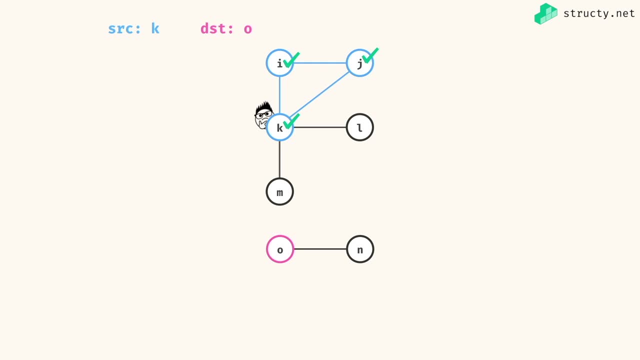 I can move back to K and really make sure that I don't explore any of K's visited neighbors. So I don't move back to I right. instead I should move to an unvisited neighbor. like L market is visited, then I only have one other node to visit, which would be this M. 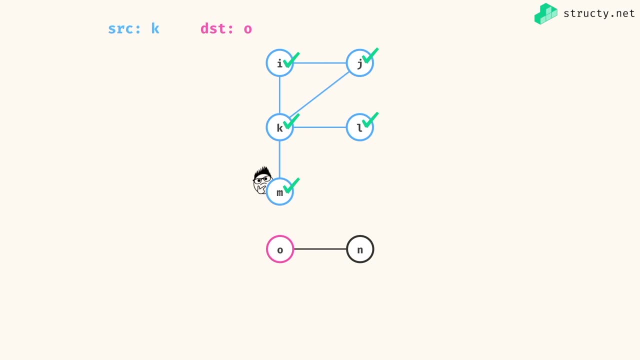 node, And at this point I've actually exhausted this full graph region. right, there's nowhere else I can go, And once I finish my traversal, if I never find my destination node, then I can just return false right. It must be the case that there is no path that it goes. 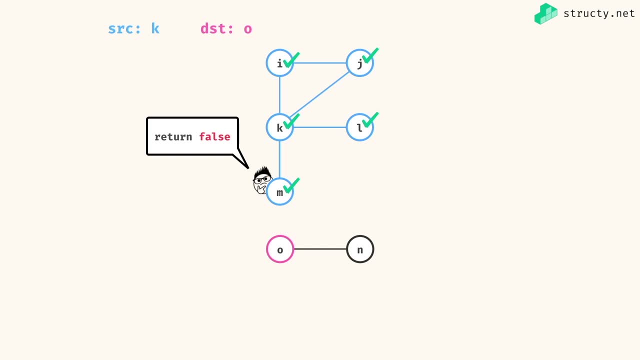 back to. So I'm going to go back to the destination node and I'm going to go back to the destination node And that's really all there is to this algorithm. Let's talk about the complexity. If we say that n is a number of nodes, let's also define that e is a number of edges, Like 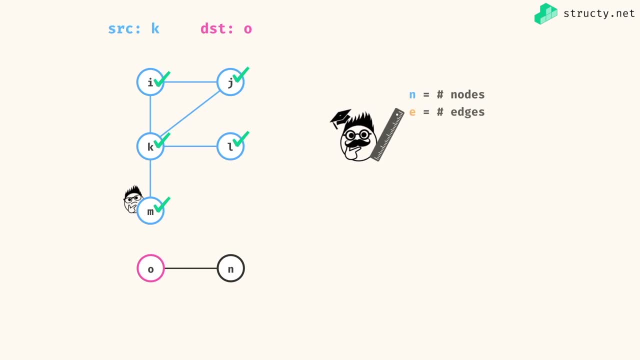 we said previously, this is something typically acceptable to do for our graph problems. I know that the time complexity is going to be roughly the number of edges and my space complexity is going to be O of n, that is, the number of nodes. I think it's worth stepping. 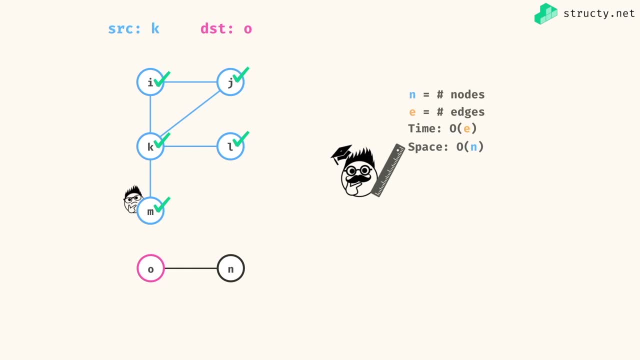 through. you know what this complexity actually is. Actually means we know big O refers to the worst case. So let's think about a worst case graph that we can have, And there are a few different graphs that you can kind of design and think of. I'll just show you one example. So let's say I was given a graph like this: 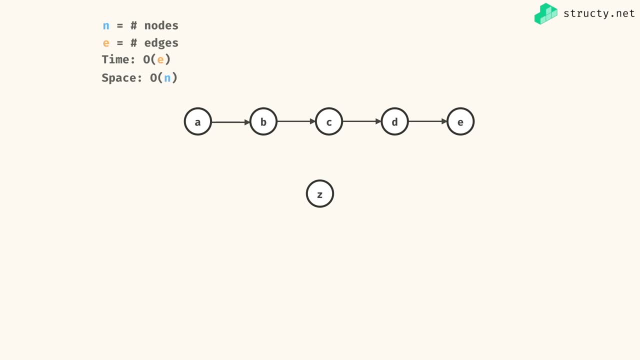 right. Notice that, although z is kind of on its own island, all of these nodes, that is, a three as well as the Zeno, they're all members of the same graph. So let's say I wanted to figure out, is there a path between a and z? So if I did my traversal algorithm from 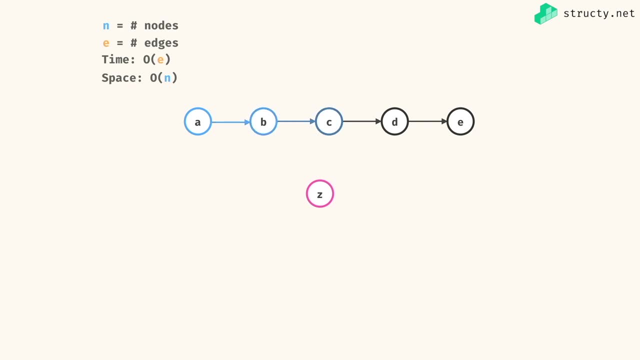 here. I'll start at a, then move to B, and then to C, and then to D and then to E. At this point I've covered all of the edges in the graph. remember that the edges are the arrowheads here, because I had to travel through every edge of this graph. That's why. 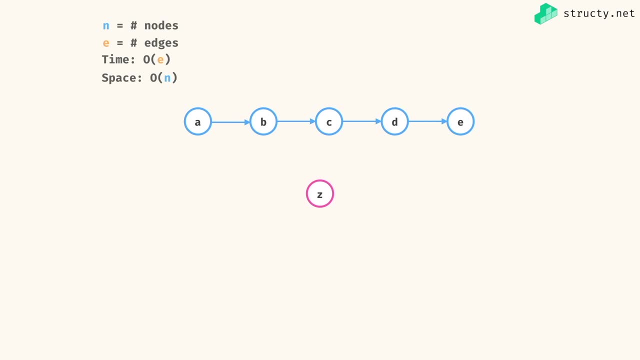 we said, the time complexity in the worst case is going to be O of E right, O of the number of edges. And here we can say the space complexity is O of n, because if you're doing this with either a depth first stack or a breadth first queue, in the worst case you would have to 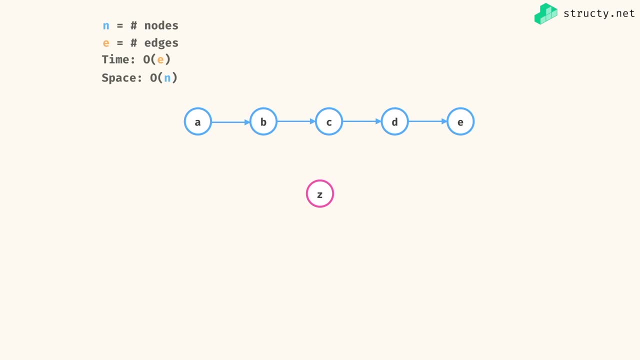 add every number of edges. So let's say, we have a graph like this and we're going to add everything you visited, or that is, all of the nodes, onto your stack or queue. That's why we say for regular graph traversal algorithms, we have a time, complexity of O, of E and a. 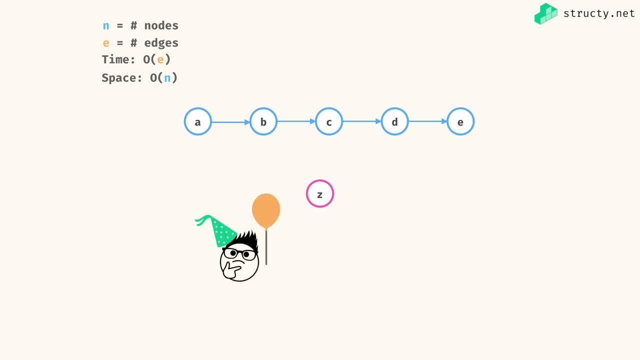 space. complexity of O of n. All right, I think we have the approach for this algorithm down pat At this point. you'll want to join me in the walkthrough videos where we can actually see how to implement these visited patterns in some code. I'll see you there, Hey programmers. 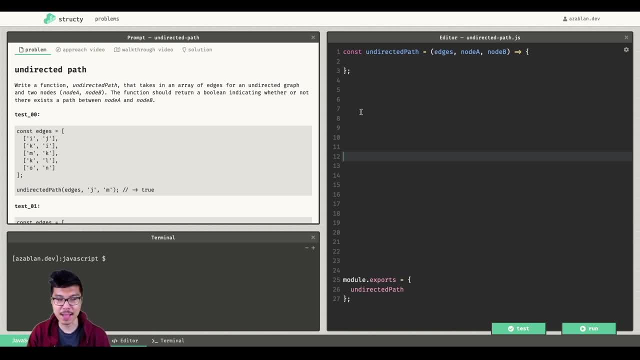 Alvin here Right now let's go over a JavaScript solution for this undirected path problem, So we'll jump right in. So, just like we said in the approach video, this is going to be like a two parter. First 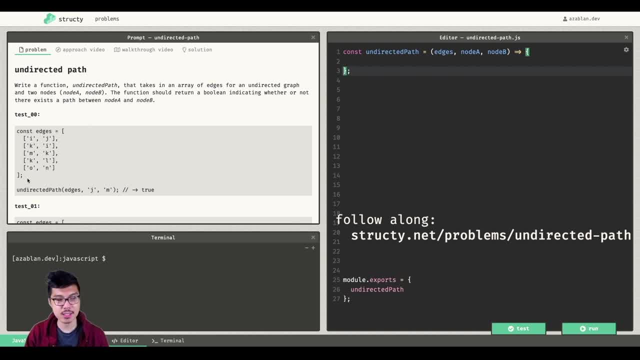 we're going to convert our edge list into an adjacency list. That way it's easier to do a classic traversal through it. So I'm going to pretend I had a helper function here That gives me back an adjacency list. I'll call it graph And I'm going to call this. 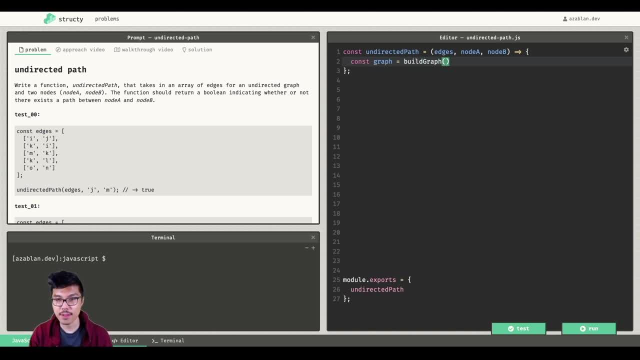 helper function will say: build graph. If I pass it, just all of my edges wanted to do that conversion for me. So let's work on that helper function right now And then we'll jump back to undirected path. So we'll go ahead and create my build graph function, just going to take in the edges. 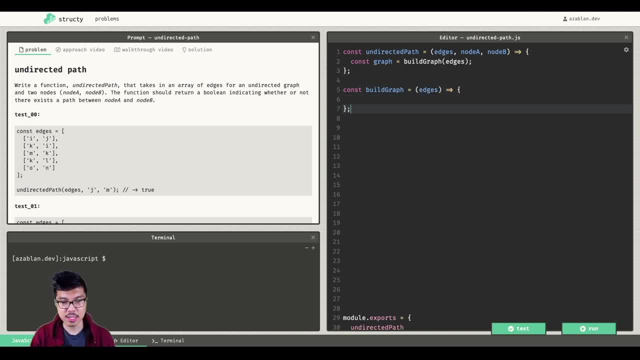 right, And I know I want my adjacent list to be in the form of a plain old JavaScript object. So create that graph object here And I'm going to return it by the end, just like this, And what I want to do is fill up this graph with information from the edges. I'm going 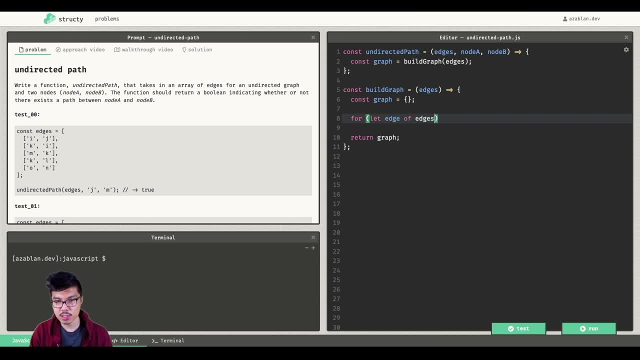 to iterate through every edge. So for let edge of edges, so iterating through every single edge, I'm going to set up an new edge object And I'm going to create an edge object. I know a single edge would be a pair, So I'm just going to destructure out of that. Maybe. 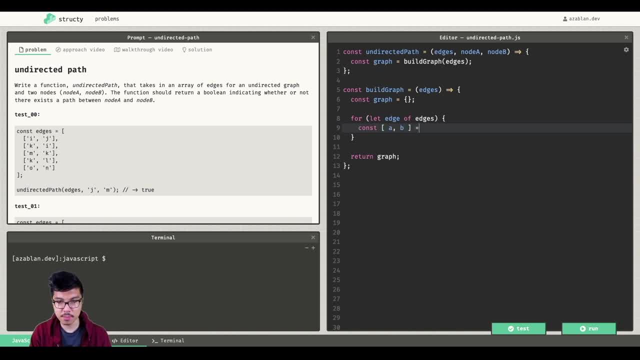 just my two node identifiers. we'll call them A and B from the edge, Nice. What I want to do is now initialize these nodes as keys of this graph object. So a would be something like this I node, or this K node, right? So what I'll do is check if a is in my graph. 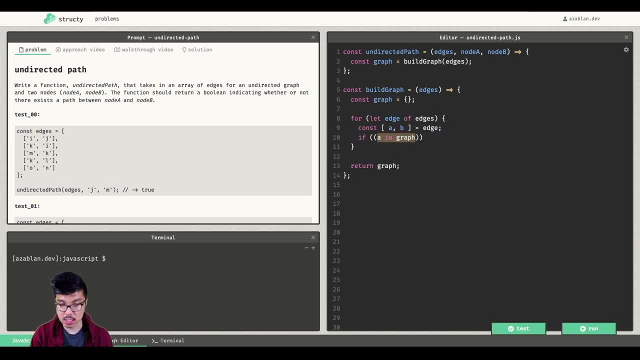 I think really to clean up this code, we better if I check if it's not in the graph. So if the A node is not in the graph, then what I can do is initialize it in the graph. So use it as a key and assign it to be an empty array, And I'll do the same for B over. 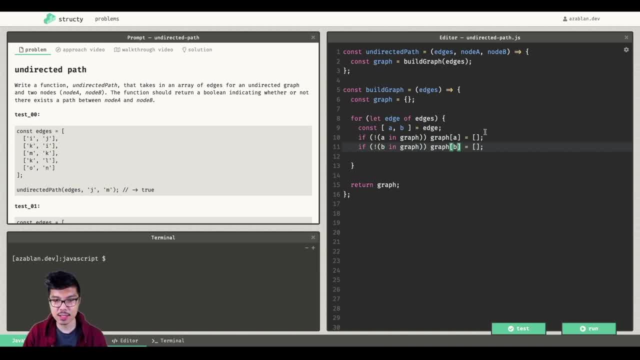 here. Alright, so I'm initializing A and B in the graph if they don't exist, And once I do that, then I can safely just add neighbors into their their edges. right, So I can say: graph, square, bracket a dot. 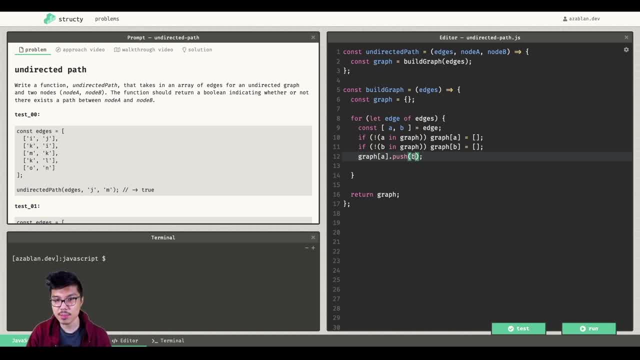 push B. So now I'm saying that, alright, B should be a neighbor of A, but I know that this is an undirected graph, right? So that should be symmetric. In other words, then make sure you push a into the neighbors of B. So it's really important that you notice. 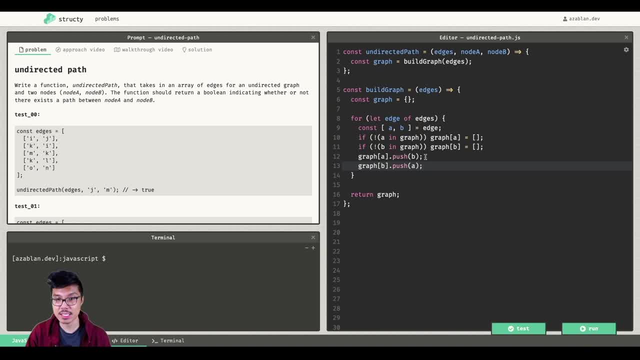 that this is an undirected graph, So your adjacency list needs to be symmetric in that way. So if A is in B's neighbors, B should also be an A's neighbors. So that's looking pretty good. Let's go ahead and see how. 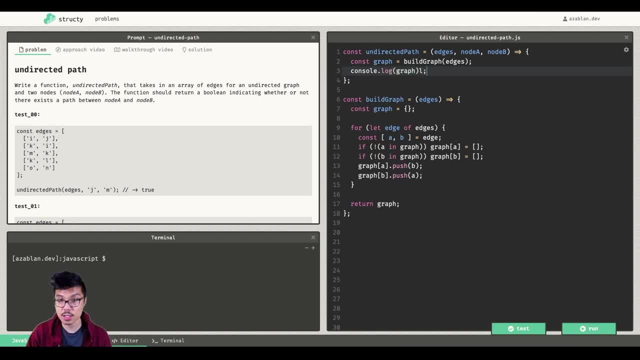 that graph looks just with a little little side test here. So I must steal maybe this snippet. Look at that full snippet here. I can just run it manually. I love to make sure I can test these little helper functions before I use them. So we'll give this a run. we should. 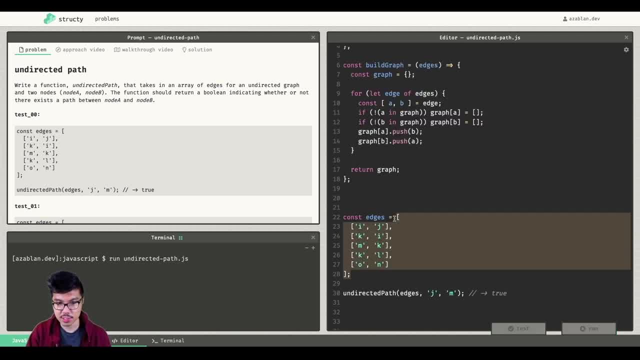 just see the adjacency list form of these edges here. See how it looks. So that looks pretty good. So I'm seeing that. all right, I is connected to J and K And that looks correct based on these edges- Awesome. And I'm also want to make sure that. 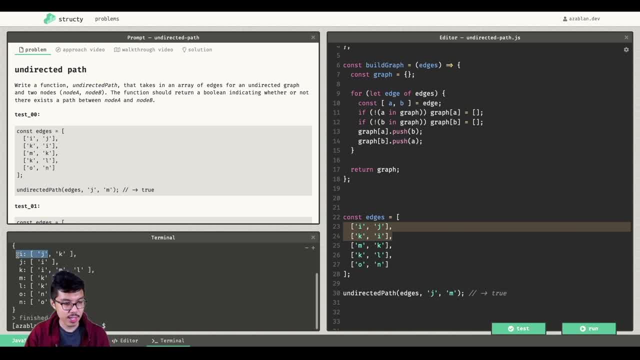 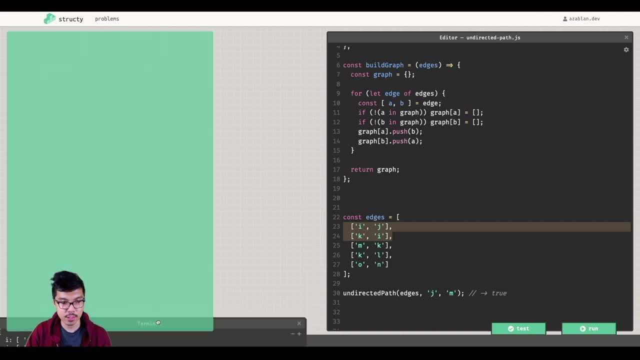 symmetric, right. So if I and J are over here, then I should have J and I over here as well. right, it should be a two way street. All right, now let's work in our real algorithm here, which would be some sort of a traversal. Now that you have a nice adjacency list, you. 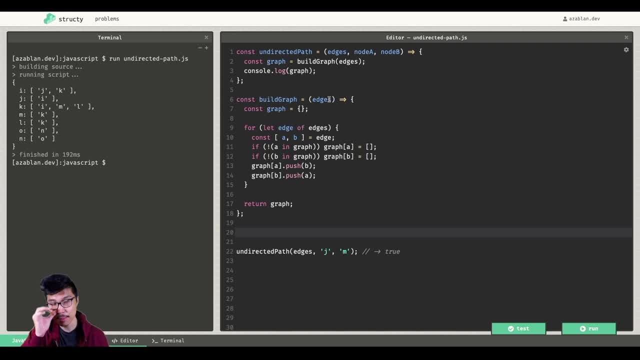 can do either a breadth first or a depth first reversal. I'm going to implement, I think, a depth first. Typically for me, it's just easier to write, especially if I do it recursively, And so I'm going to pretend I had a function. 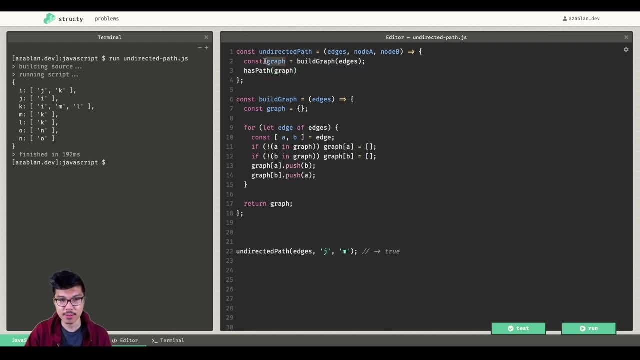 called has path it's going to take in my graph now and also a start node and an end node. So I want to find a path from node A to node B. of course I'm going to assume that this function returns a Boolean, But of course I have to write that function for. 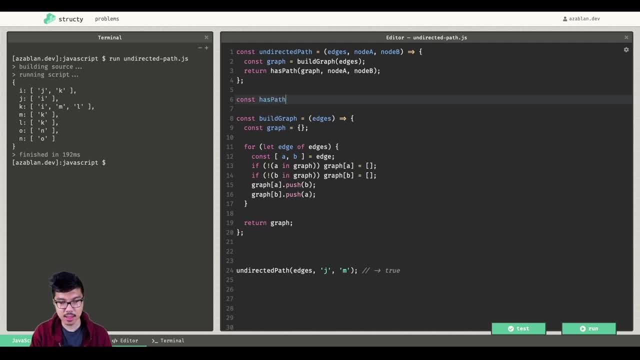 myself. So let's say, organizing our code, we'll say: has path. I'm going to take in the graph as well as node A and node B, And I think a better way to do that is we're going to take in a path from node A to node B And then we can take in the graph as well as. 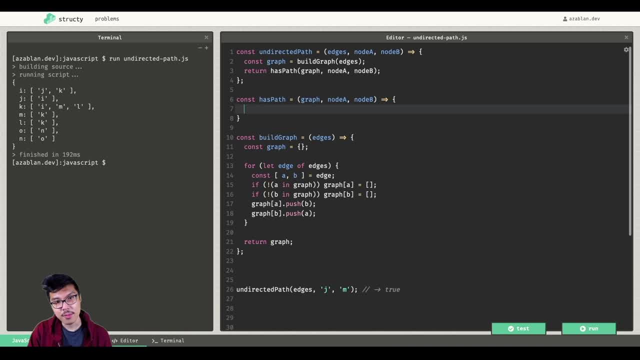 node A and node B. So we're going to take in the graph as well as node A and node B And I think about that better name for these arguments. I'm doing this recursively. let's call this one source and this one destination. So over time we're going to call recursively and update this. 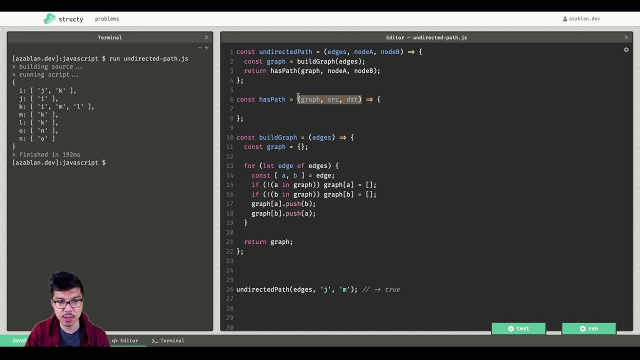 source node, And that should be a familiar pattern to some other problems we solved recently. So I think about my base case. Alright, I know that I have successfully found a path when my source is equal to my destination node. If that's the case and return true. 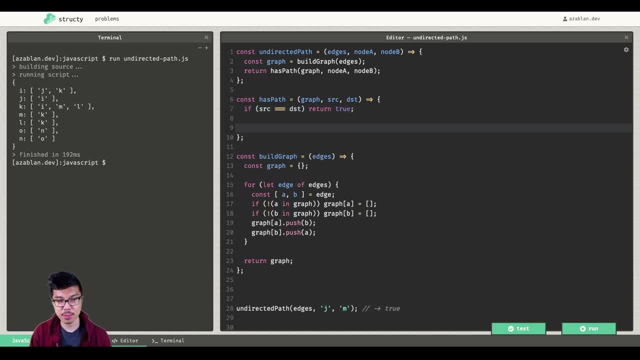 because I just found a path. Otherwise I have to keep looking. So I should be able to look through the neighbors of my source node. So I could say: graph, square, bracket, source, right, Remember that at any point through this recursion source represents my 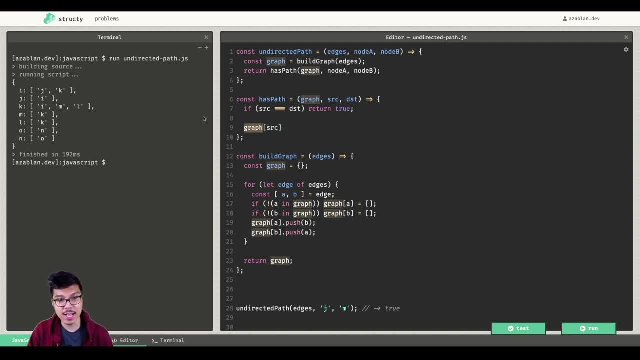 current position. If I say graph, square bracket, source, let's say source was I, I'd be accessing all of eyes, neighbors, right? So what I want to do is really iterate for let neighbor in, or rather of graph of source. So if sources I, on the first iteration, neighbor would be. 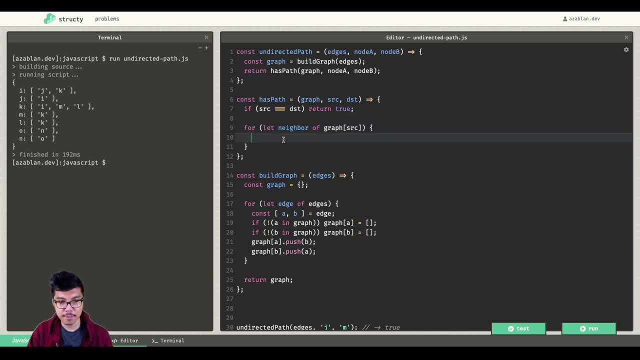 J. Second iteration: neighbor might be K, And for each of my neighbors I want to travel to them. So call has path. you can keep your graph argument the same. needs to change your source, though. Now you're situated at your neighbor and your destination is fixed, or? 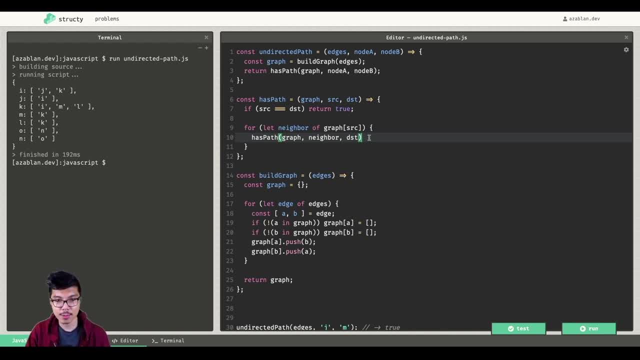 you're always trying to get to the same exact node. I'm going to think about what type this returns. I know this is going to tell me Boolean right, True or false. Is there some path from my neighbor to the destination? I'm going to check. Alright, if that call returns true. 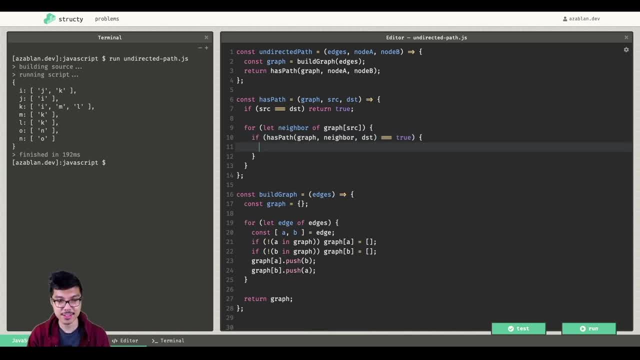 I'll be explicit here. So my neighbor is taking the path from my destination, right, So let's take the path from the destination. Also, if your neighbor is noiseinski, so this is� ku I'm going to say, pouring in too much material here, close to 0, so that we can just çalış the. 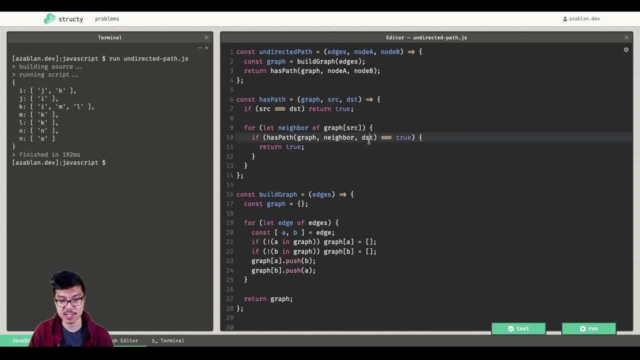 last Mm, and this will get managed by the behavior in the wallet. This should be perfect. So let's see if we can get it to 0 without pressing anything, because Awesome never find that any of our neighbors make a winning path. then it means I finished this. 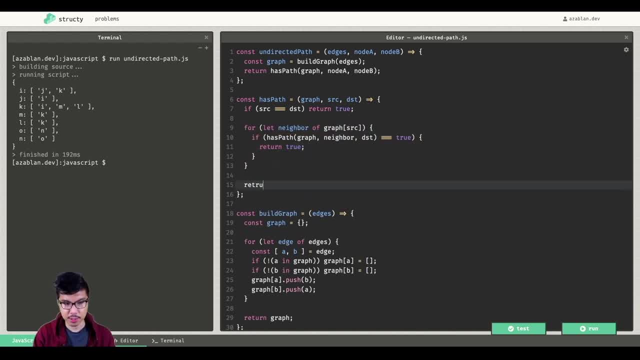 for loop without ever returning true, which means that I can return false. right must be the case that this source node does not have some path to the destination, So I think we can go ahead and give this code a test run. If you watch the approach video, you'll. 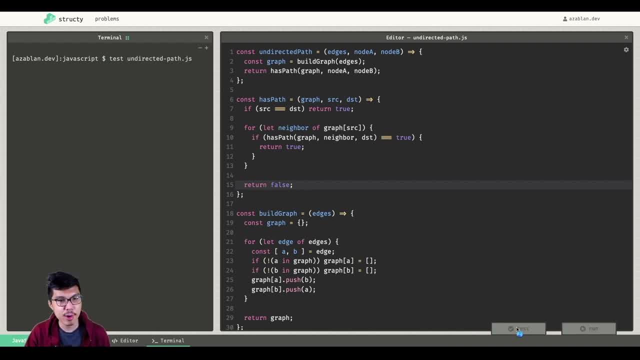 notice that there's something important missing from this code, But we'll just run. it can show you how to fish here. So here I'm getting an error. edges is not defined, what I do horribly wrong Line 34.. Let's look at line 34 over here. So gotta take out this call, Don't need. 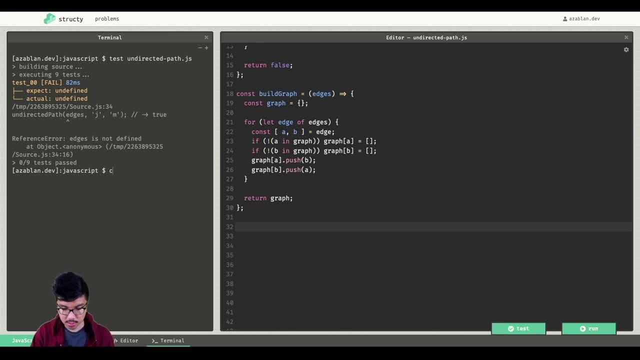 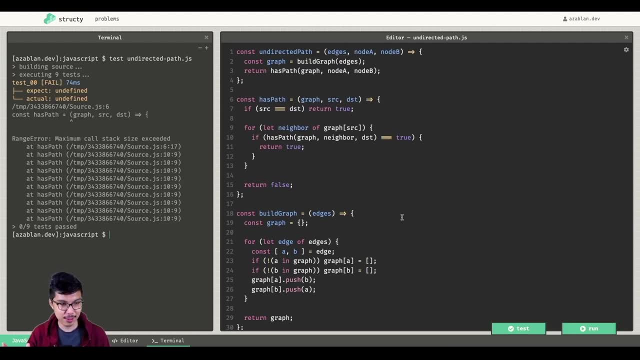 that anymore. That's on me, Let's get that test run. So that was not the error I was expecting. I am expecting some sort of an infinite loop. though Perfect, I'm getting maximum call stack size exceeded, So I got like an infinite recursion really, And that's. 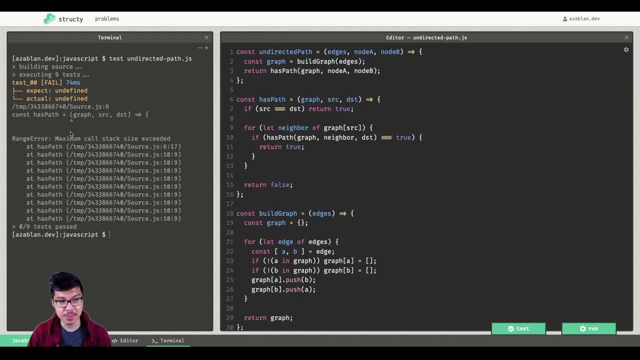 going to be the end of this video. If you liked this video, make sure to hit the like subscribe button And I'll see you in the next one. Bye, bye. So this has path. I know that that is the actual function that does the traversal. I'm 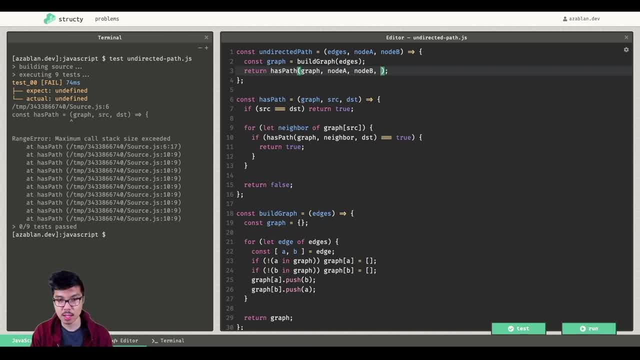 going to pass along a new argument here And I'll make it a new JavaScript set. So if you're unfamiliar with sets in JavaScript, they're really just a collection of items, And what's really great about a set is in O of one time I can add something into the set And I can 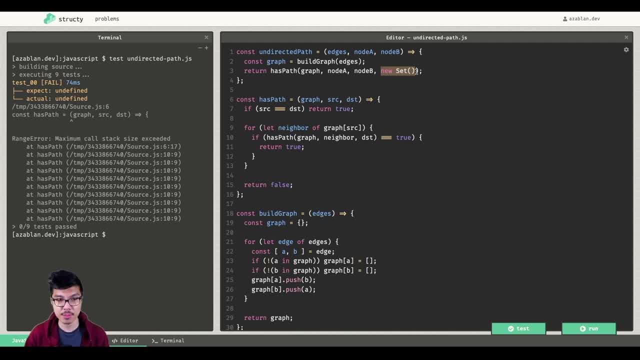 also check for something within the set which is going to be very, very quick for our traverse. So I don't want to use something slow like an array, because to do a lookup or a check within an array that would actually be O of n time, whereas for a set it's O of one. 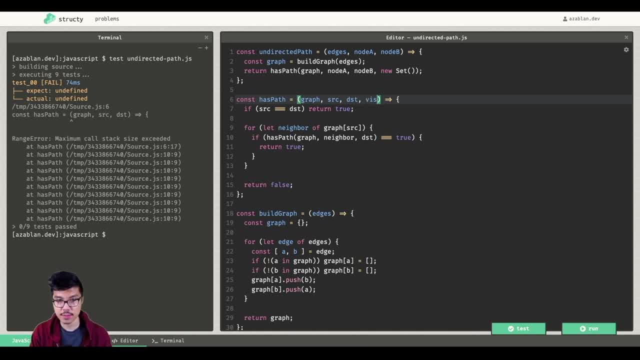 So I'm going to make a new argument here to receive- I'll call it visited- And what I want to do is: all right, check If my source node is already in the visited- set to do that in JavaScript, I can check visited dot has. So if the source node is inside of the visited 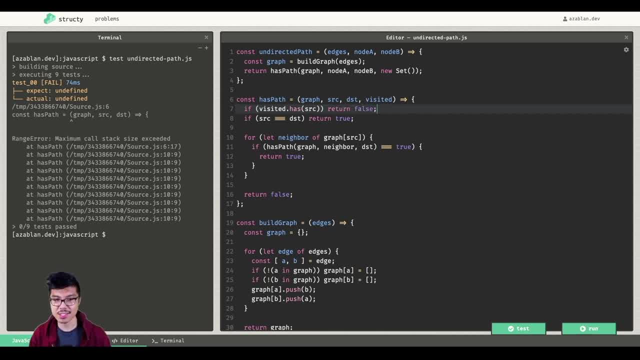 set. then I could return false here, right? There's no reason to travel through this note anymore, Because if it's in visited, then I must have traveled It previously. this is how I can avoid any infinite recursion And I can also move this. 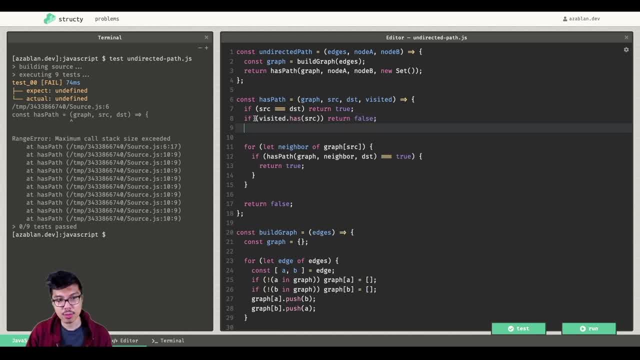 line downward if I wanted to, And let's say that I make it through this if statement. So that means that, all right, this node source has not been visited, but I'm visiting it right now, So I need to do visited dot add source. So this expression checks if source. 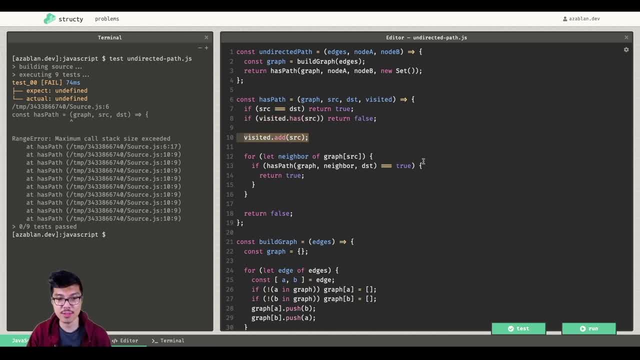 is in visited and this expression adds source to the visited set. I want to change a few other details here. Make sure that you pass the along the same visited set through all of your recursive calls over here, Because you want this visited set to be like global for the entire traversal right. I need to know. 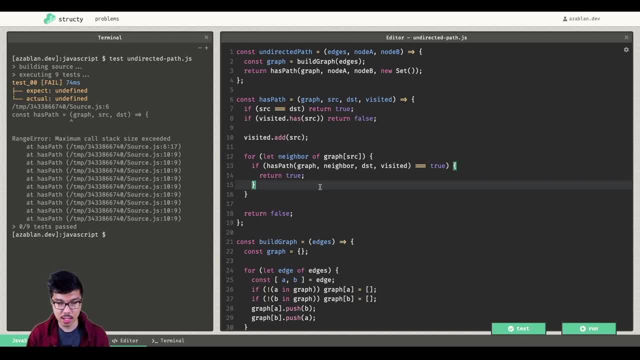 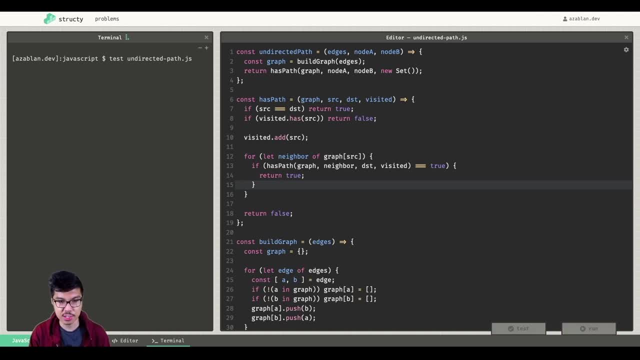 exactly where I've been in the past, And once we have that in place, that should be everything we need to prevent any, any cycles from giving us infinite recursion here. Let's give it a test run. Awesome, There's a solution for our undirected path problem, So important. 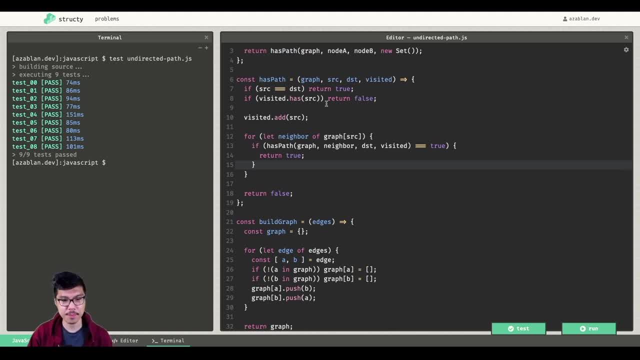 things to take away here. do consider this problem a two part problem. So let's say we have a problem, a two parter right. Phase one is really straightforward: just converting an edge list into an adjacency list, which is actually an important skill to practice. 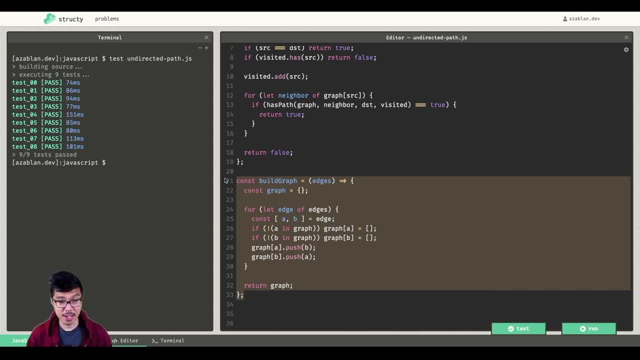 Because when it comes to you know some problems you'll face in the wild, they are all going to be basically graph problems, But sometimes they'll give you the graph in like a different format And you can always convert into a format that you're comfortable with. Then 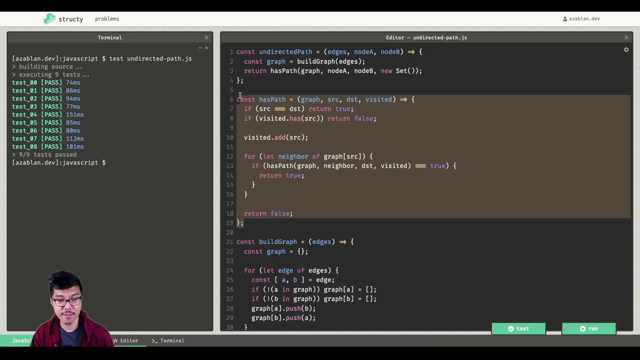 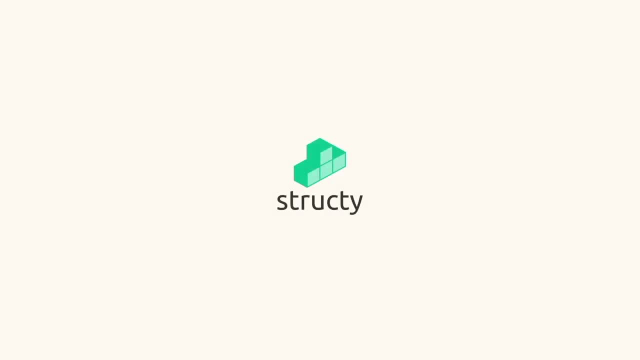 from there we have a really core pattern of just doing a traversal through a graph, but also guarding against infinite loops, right, And to do that we just use some sort of a visited set. Hey, programmers, welcome back. Right now I want to go over the approach for this connected. 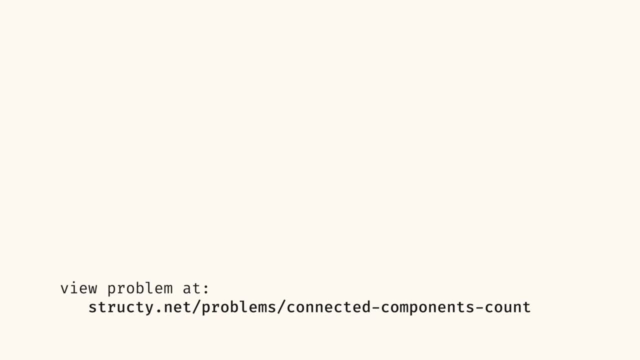 components count problem. So in this problem we want to do is take an adjacency list representing an undirected graph. As always with any graph problem, you want to start by visualizing the actual graph, And so if we took a picture of this information, it would end up looking: 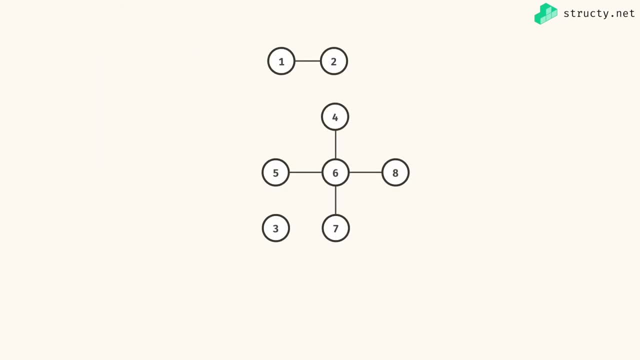 like a graph with this structure. The first thing we should notice about this visual graph is that it has multiple connected components. So, for example, I can look at this component in pink, spanning just this component, And then I can look at this component in pink. 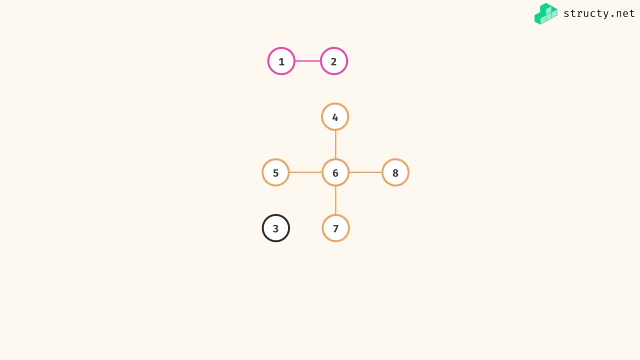 spanning the one and two nodes. I can look at another component spanning the 45678 nodes And finally a third component just covering the three node, And that's why we say that your result for your function here should be three right, because there are three different. 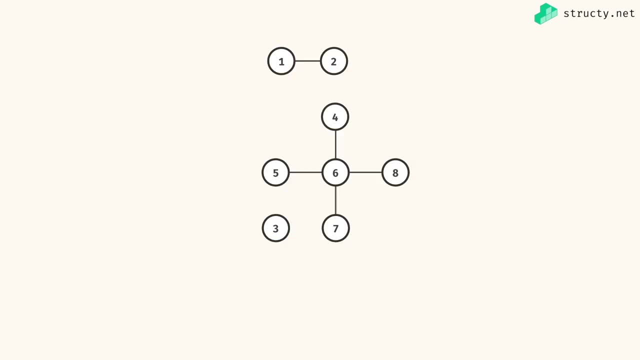 connected components. So let's come up with an algorithm we can use to count the components. we know that a general counting algorithm is going to use some variable and we'll initialize that count variable to zero, And the trick here is to use a combination of both some. 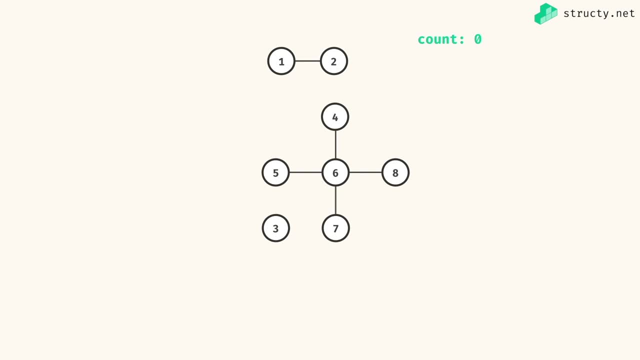 standard graph And, in the end, what we're going to need is sort of an idDe‑percent error. So, instead of a dependency method, what we're going to need is not that tea Muller seed for the function, but something terrified, and we're going to need j, none. 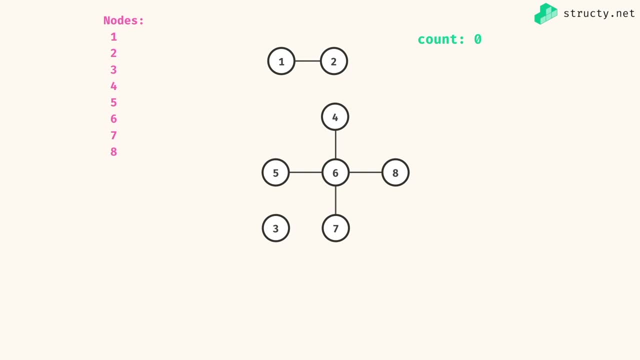 of the parameters within this field now. so I'll pull up. this has a function And I'm going to pay it $22.. And that at this point this function amount will be Federal. It's not gonna happen. Why don't we? Our image is gonna be empty, so I'm gonnaшийand index. 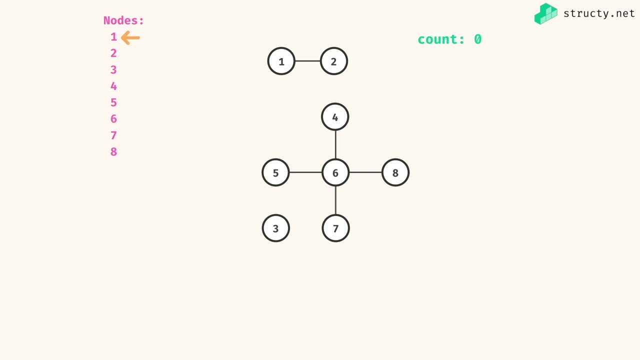 this element. Let me start this fulfilment method For this. let's here I'm going to first. So let's say I start at the one node over here. what I should do now is continue this traversal as far as possible. That's the key to victory here. So from this one node I can move. 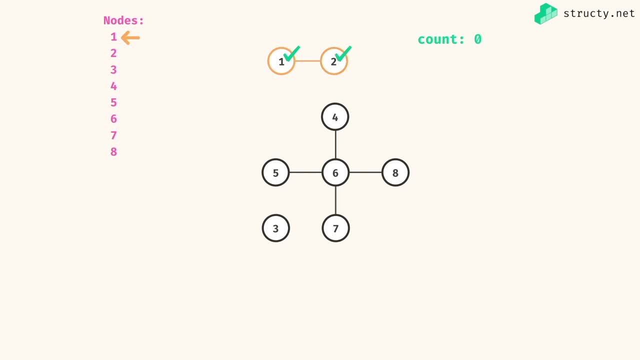 to a neighbor of two. And of course, as I travel through these nodes I want to make sure that I mark things as visited So I can avoid loops. And marking things as visited will also ensure that we don't double count any components here. Once I hit that to note, I've actually completed. 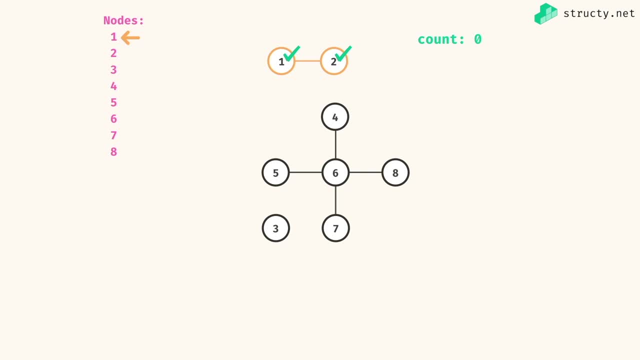 this full component. there's nowhere else I can explore, So at this point I should increment my count by one. So whenever I complete a new traversal on some region of the graph, I need to increment my count At this point. I now fall back to my iterative code on the left hand side. 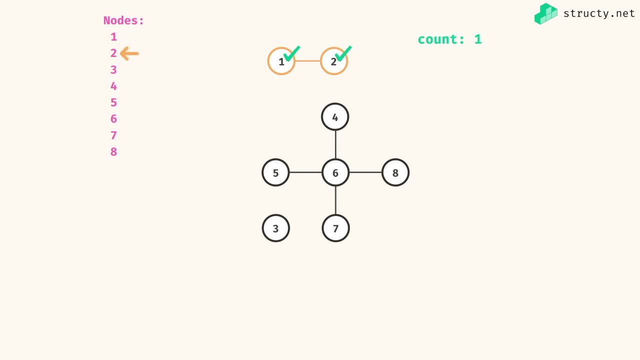 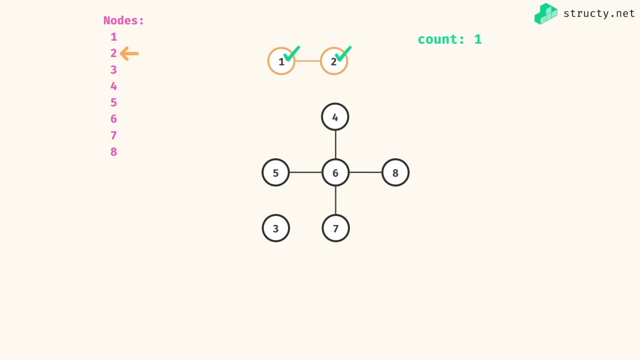 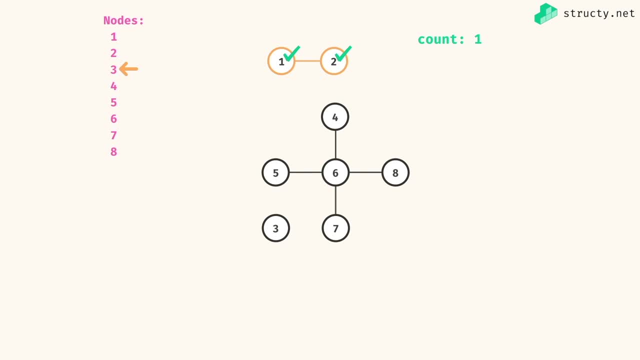 three is unvisited right now. So I should begin a new traversal starting at this three node, which means I just mark it as visited And since this three is a singleton node, right, it's not connected to anyone, I would actually complete the traversal just on this three node. 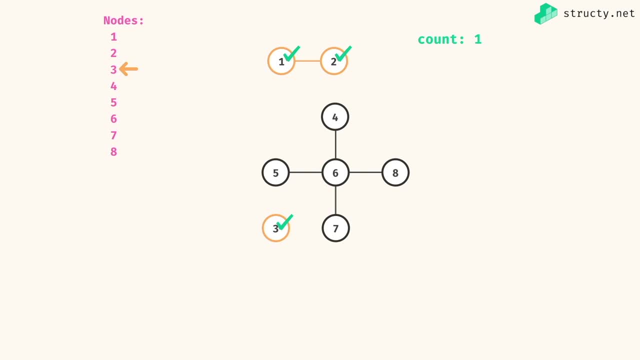 At this point I've completed a traversal. So I increment my count by one, So now I have a total count of two. I fall back to my iterative code, So I move from the three node to the four node and I see that this four node is unvisited, which again means I must begin a traversal from this. 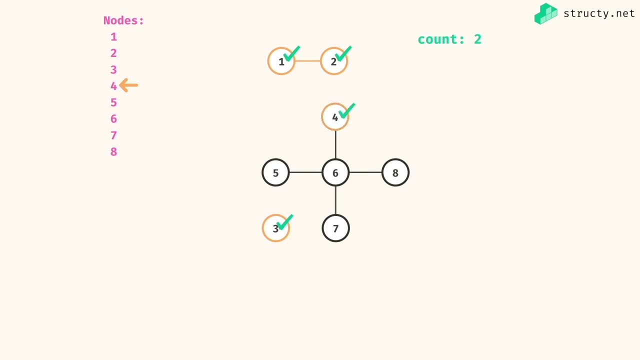 four node And I'm going to expand this traversal, starting at four, as far as I can before I go back to my iterative code. right, so I'm going to explore the six, explore this five, explore the seven and finally explore this eight. At this point I've completed a traversal, so I can. 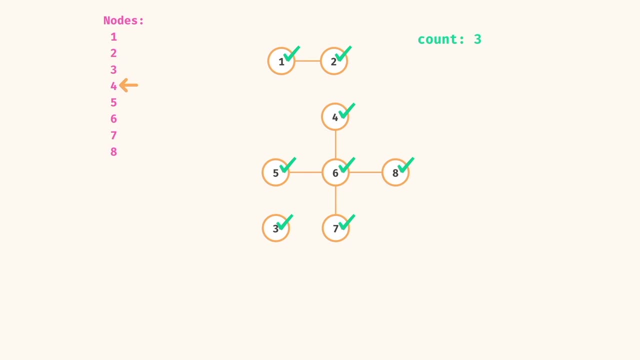 increment my count up to three, And then I have to continue and fall back to my iterative code. So, like at the five node, I see that the five node is already marked as visited, So I don't start a traversal, And I see that the 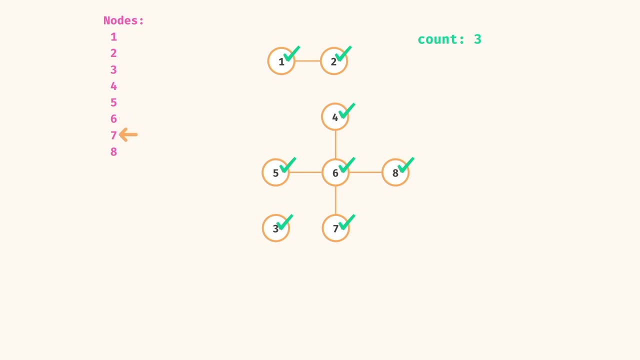 six node, same thing. don't need to start traversal. seven node already visited, eight node already visited. At this point I would be done with the entire algorithm And there's my final count of three. So a few interesting mechanics here. right, you're going to need to definitely. 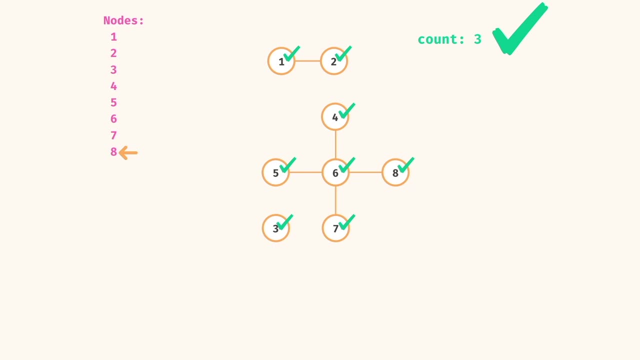 implement some code or some function that does a traversal through some component as far as possible. But then you also need some iterative code just to potentially begin a traversal, And what you want to do is be sure to mark nodes as visited as you traverse them, because only when 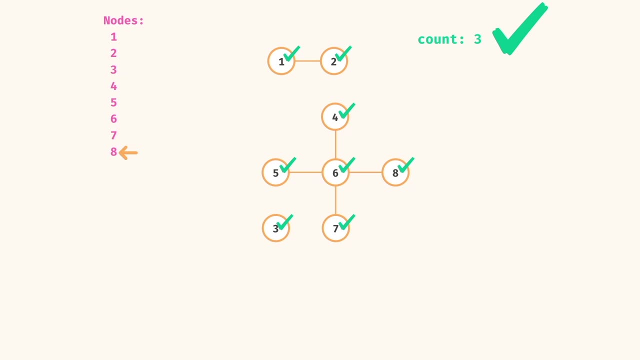 you mark a new node is visited and complete that traversal should you increment your count. you're probably wondering the exact details of how we implement this in some code, But don't worry, you'll realize that it's really just a spin off of our previous graph algorithms in the walkthrough. 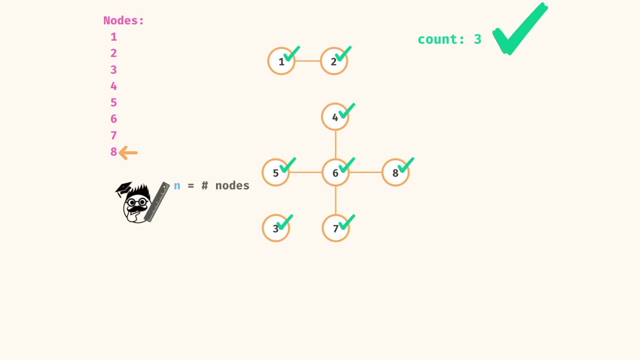 video. But for now, if we say that n is the number of nodes and E is the number of edges, like usual, we know that this is really just traversing through the entire graph. So we can say that the time complexity is just O of E And the space complexity is O of n? right, Depending on whether 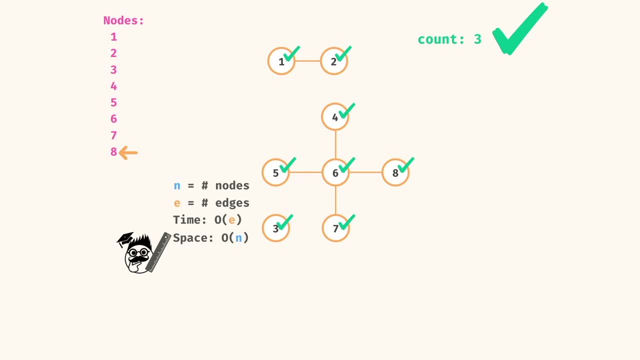 you do a breadth first or depth first, you're going to use that space in terms of your stack or cube, And we can also consider using the space within our set if you use a set to mark your nodes as visited. but overall it still will lead to a linear time and linear space solution, All right. 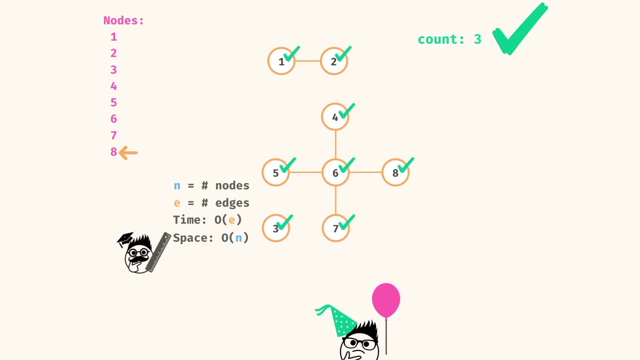 I think I'm ready to code this one up. I'll see you in the walkthrough video. Hey programmers, Alvin, here Right now. let's go over a JavaScript solution for this connected components count problem. Let's go over a JavaScript solution for this connected components count problem. 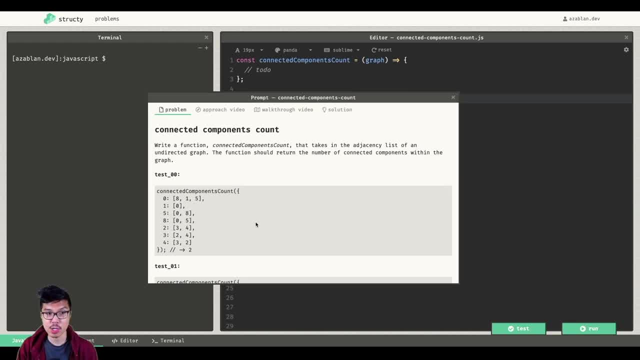 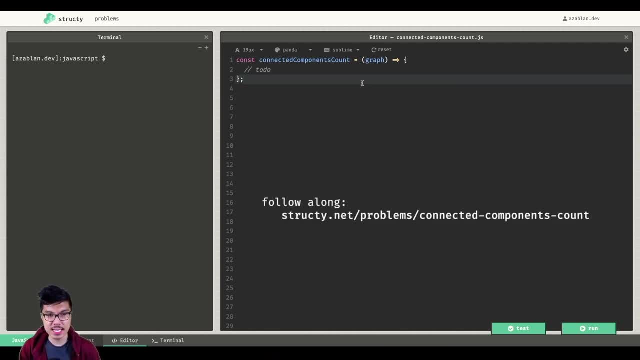 And so we'll implement exactly the strategy we spoke about in the approach video, So make sure you watch that first. We know that this is going to require really two different mechanisms. we're going to need our iterative code just to hop to different connected components, And we also need 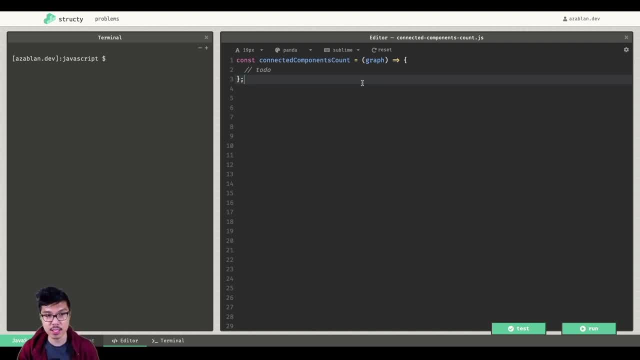 some traversal code to just explore some single component as far as possible, And so what I'll do here is: let me start with the iterative code. So I need to begin a traversal at every potential node So I can start with the iterative code. So I need to begin a traversal at every potential node, So I 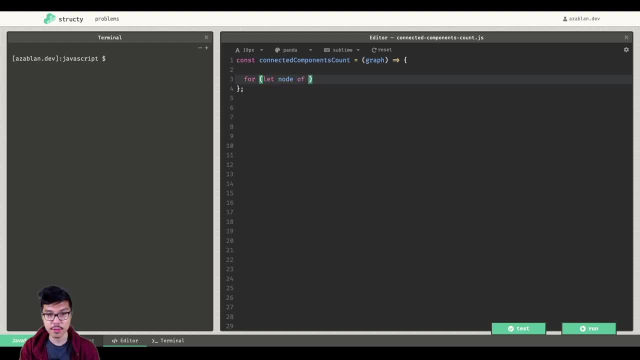 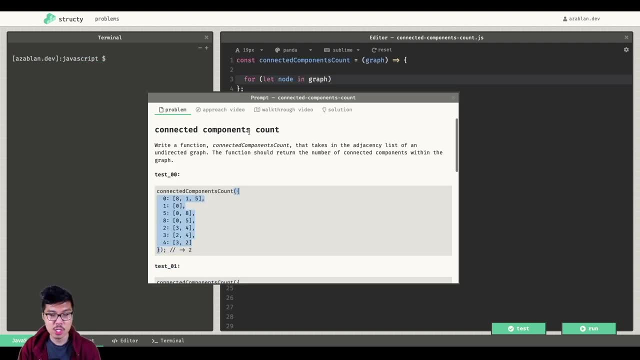 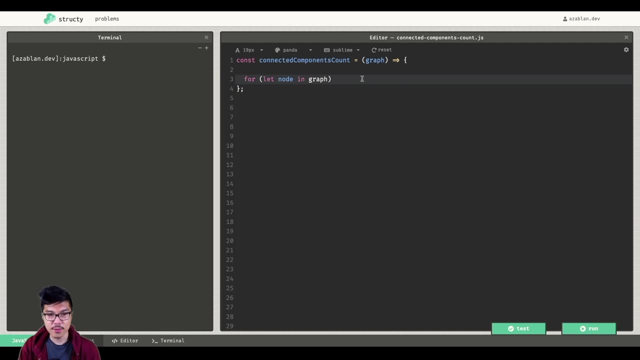 can say for let node of my graph and really essay in my graph here, because for this problem we're given looks like JavaScript objects. So if I say for let node in graph, that would give me each of these keys like 015, and so on, And so for every node of the graph what I want to do is begin a 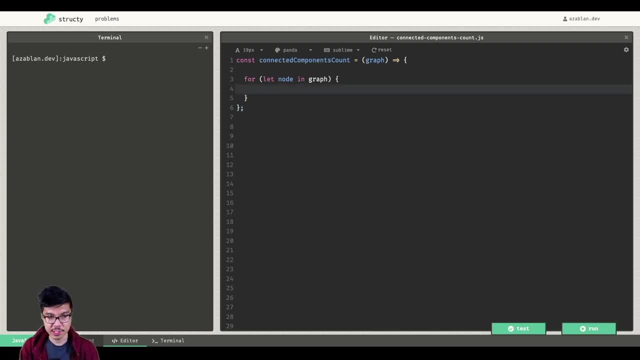 traversal. So I'm going to assume I have a function here. I'll call it explore. I'm going to pass in, of course, the graph as well as that node, And what I want to do is I'm going to pass in a function. 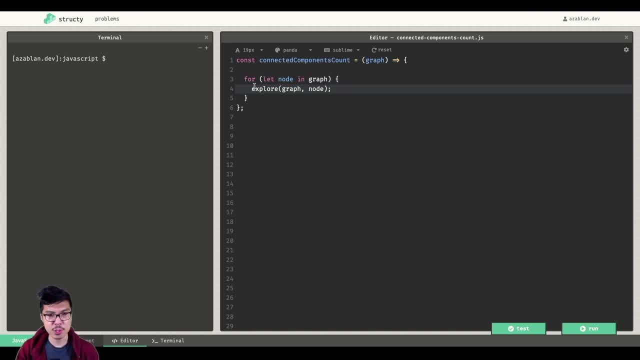 here, And what I want that function to do is do like a- we'll say, adapt first traversal from that node as far as possible, Right? So probably going to need to add more logic into this main function, But for now, I think it's about time to actually flush out explore, So I'll choose to do this. 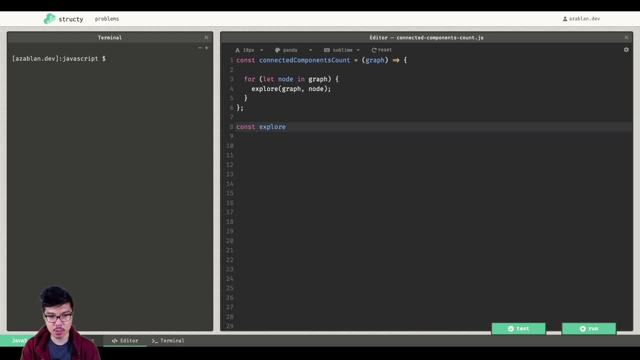 explore method recursively. So we'll define, explore. it's going to take in a graph as well as my current node. I'll just call it current right And then from there I want to solve the recursion of this one using a depth first. So recursion is fine And not much to do here. but 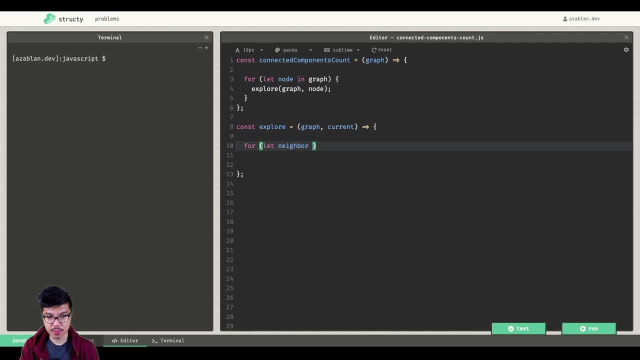 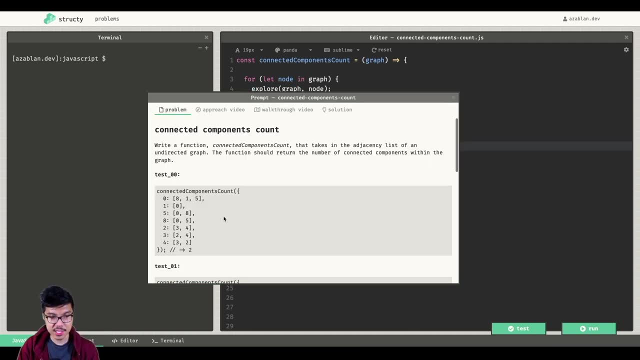 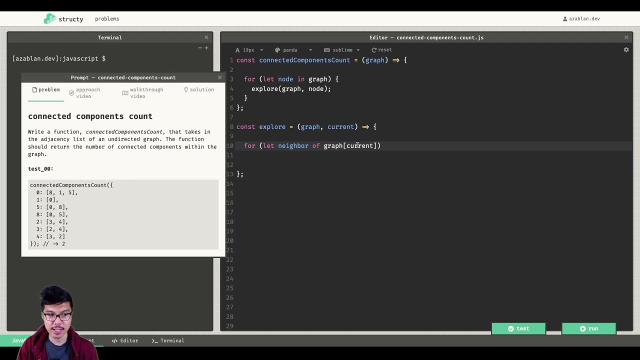 really go through. my neighbors want to iterate through every neighbor of this node. I can say, like neighbor of graph of current Right, recall that graph would be an adjacency list. So if current spread this out, So if current was a node like eight, then on the first iteration neighbor, 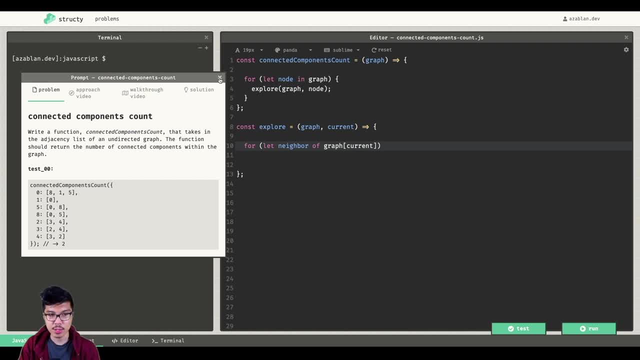 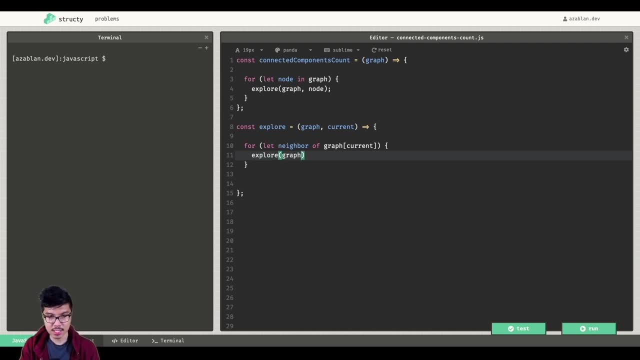 would be zero. next iteration neighbor would be five. So here I'm just going through all the neighbors of my current node. I just need to traverse to them So I can call explore, pass along the same graph. that doesn't change. But now my new current node would be that neighbor. 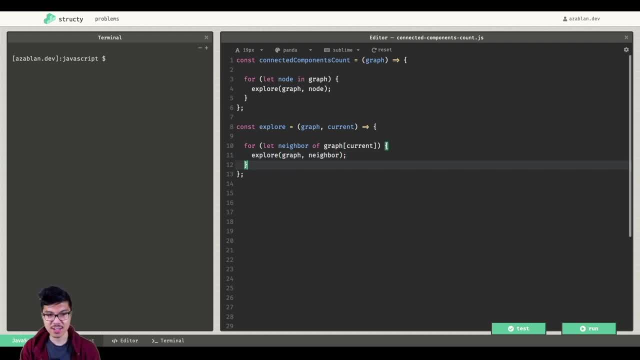 Just like that, And this will perform the baseline of just the kind of depth first traversal. But we need to also mark things as visited, like we said in the approach video. that's a really important a part of the solution And I want this, like visited, set to be global for. 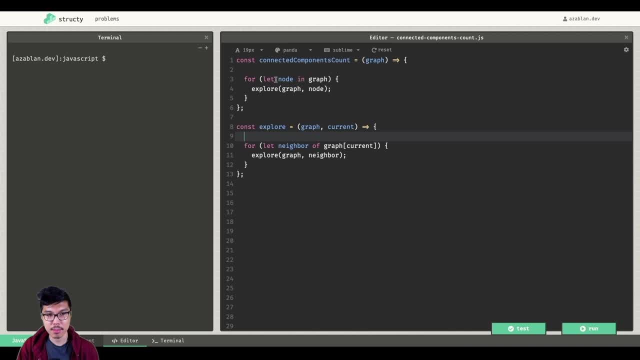 entire traversal. So I'm going to have to create it- maybe my main function over here- so I can create my constant visited, make it a JavaScript set, because JavaScript sets offer me O of one lookup and O of one addition And I can pass this visited set by reference into all of these calls. 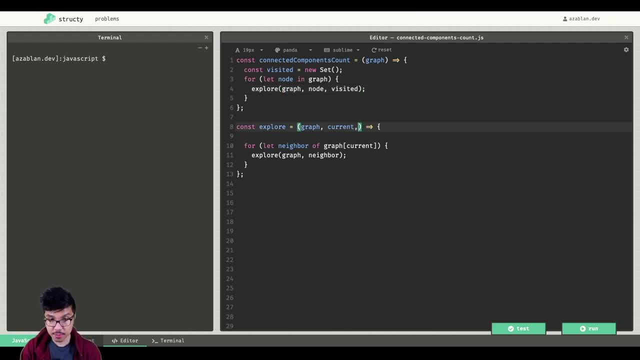 over here. So I know I'm going to receive visited over here now. Now I want to actually start using visited. So a few things to note. right, I definitely want to use visited to prevent cycles, right, That's one of the main reasons that you'll be able to see this. So, for example, for like: 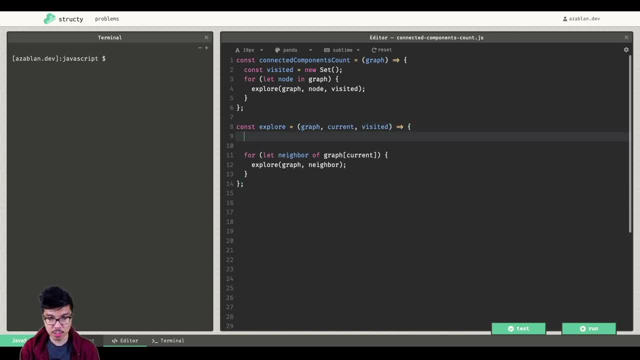 reasons we always add visited to our graph traversals. So some familiar code here if I've already visited this node. so if visited has this current node, then nothing much to do here, maybe just return false. Later on we'll see the really cool trick we use here by returning. 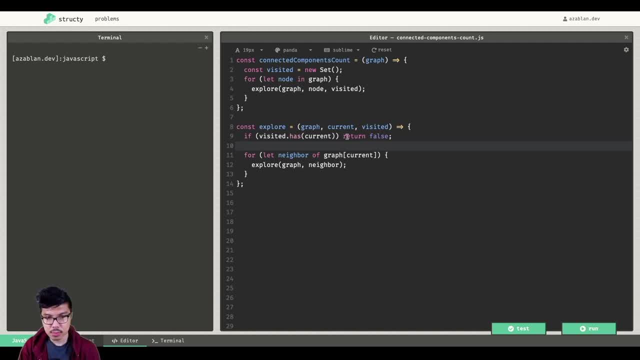 false right actually serves two purposes. So return false because this might be a cycle. And then I need to make sure that I pass this visited set along over here as well, Nice, And let's say that we have a current node that is not visited, So this statement is false. 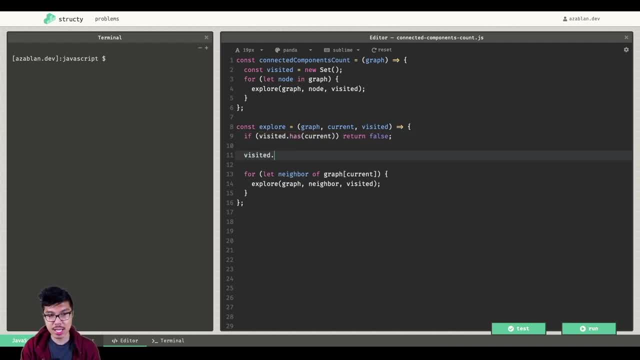 well then, it seems to be that we're visiting this node right now, So now we should add it into the visited set Nice, And then, beyond that, we need to make sure that our explore function is consistent in its type, right? So what I'm going to have my explore function do. 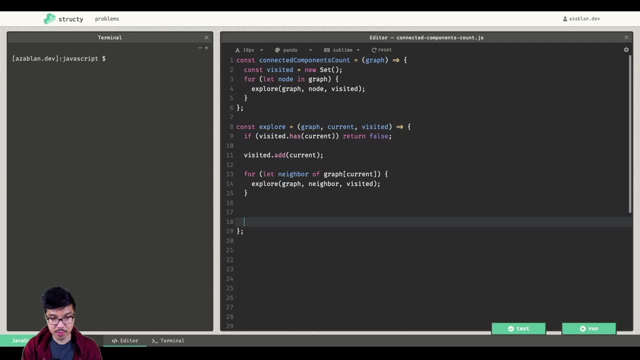 is it's going to return true whenever it explores like a new node. return true. If you take a look at this code for my function to hit this line 17,. return true, then it must be the case that it has already finished exploring all of its neighbors, right? 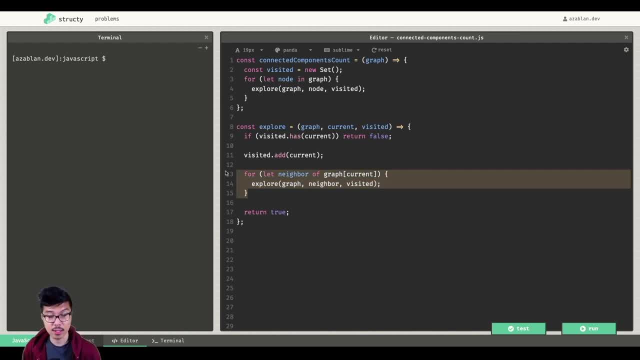 Because I know that this for loop does the job of exploring all of the neighbors, right? So only after all of those neighbor calls return will I return. true, And that must mean that I've explored this component as far as possible, right, And that seems good to go, And what I can do is 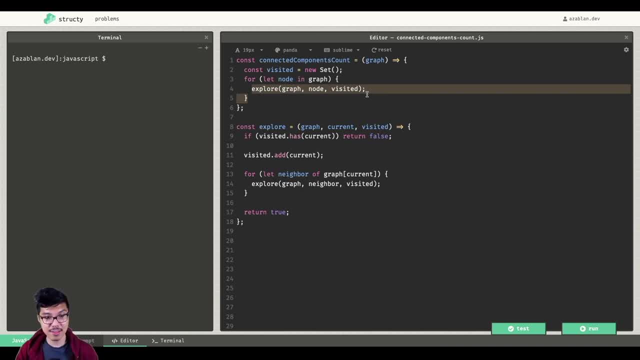 now in my main function, when I call explore it now it's going to give me Boolean data, right? If it's exploring a new island or a new component, it's going to return true, So I can check. Alright, if explore returns true, then that's a new component, So I can probably increment. 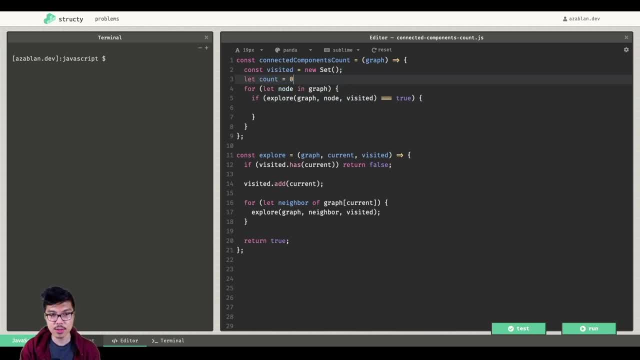 some count here I should have created. So I'll say: let the count equals zero And I'm going to increment that count when I find a new component. plus equals one by the end. I should of course return that count. And what you'll notice is for scenarios where we, let's say, iterate into a node that we already. 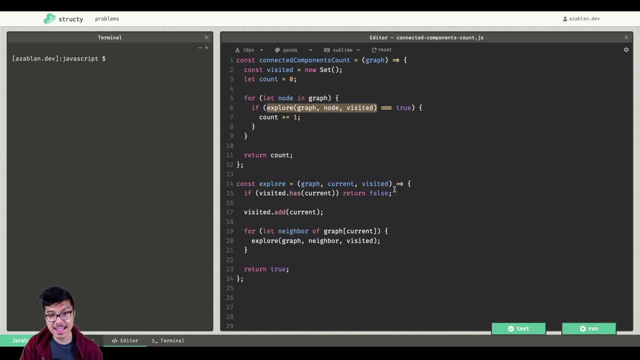 explored. when I make this call, I know that that call is going to return false, because if something's already explored, it would have been added to visited. So that's why I'm using some Boolean return values for this recursive function. So that code is looking pretty good, I think, at 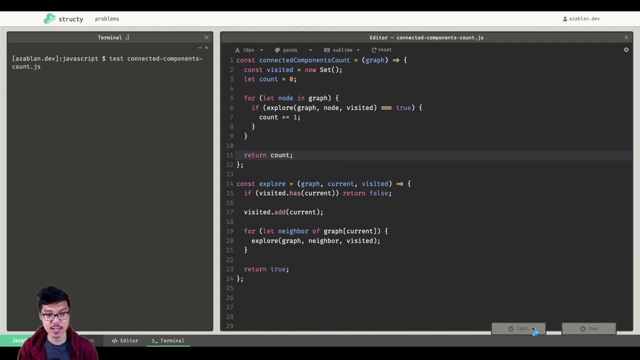 this point, we might be ready to test this one. Let's give it a shot. Let's give it a shot Here. So some pretty tricky code. it's not very long, And this is a really core pattern. here Looks like I'm getting an error. we have something wrong here, So looks like the answer should have. 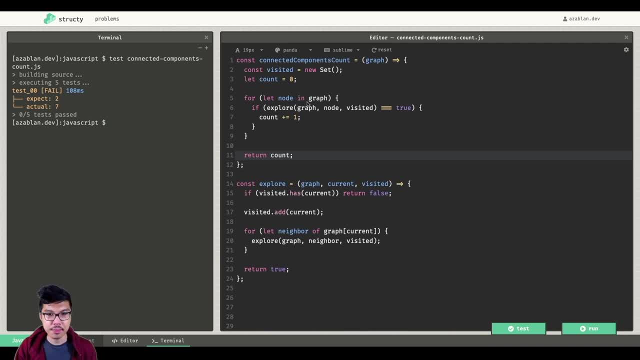 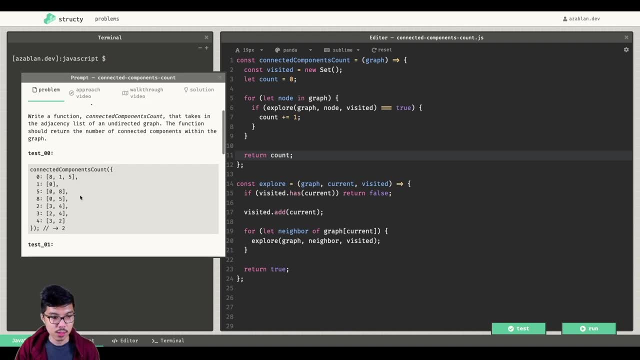 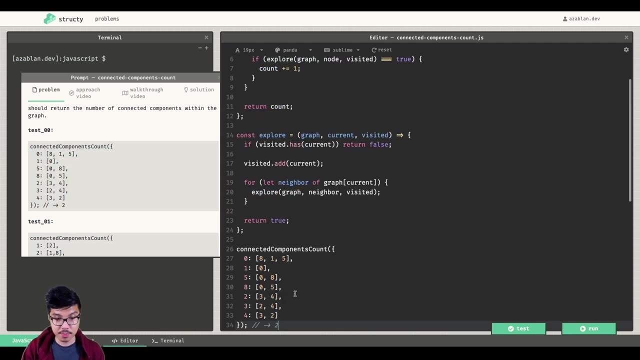 been two, but I gave back seven, So I'm counting way too high. So what I'll do to debug this one is really just maybe print out my visited. So this is a very common mistake in JavaScript. I'm going to bring in, I think, this example- we can test it manually- What I want to be sure to do. 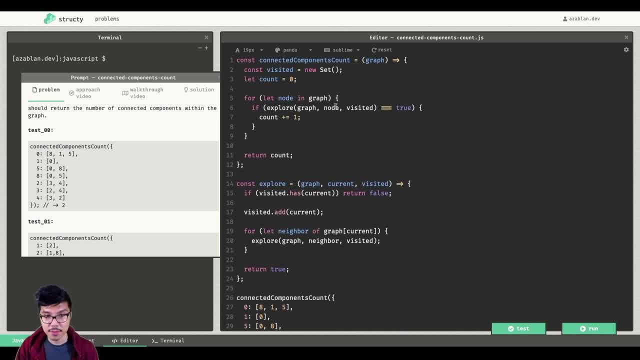 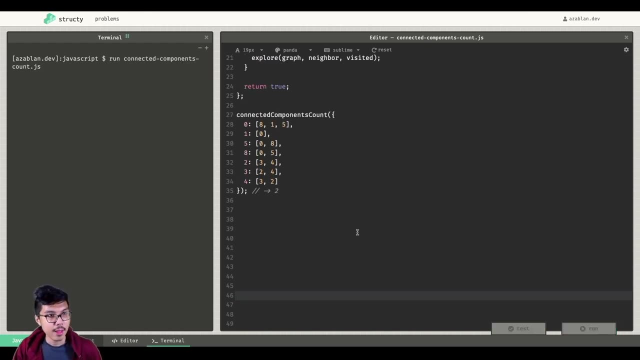 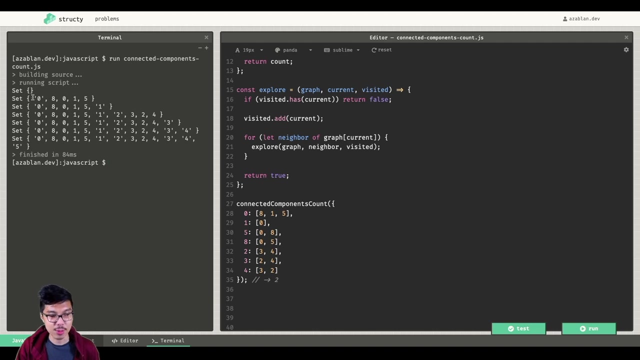 is maybe at every iteration of let's say this this for loop: I console dot log what visited is. we'll see how visited changes every time And I'll run this manually by just hitting run And let's see what we get here. So a few things to note. it looks like some of our keys or some. 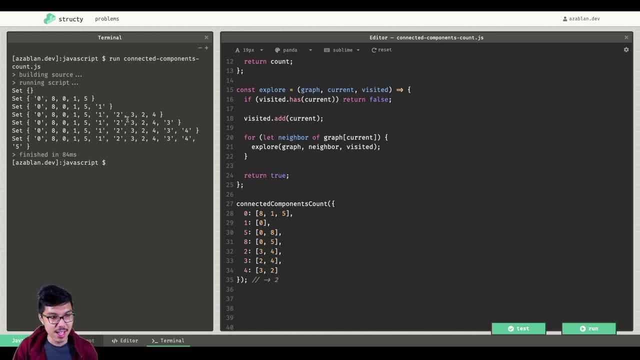 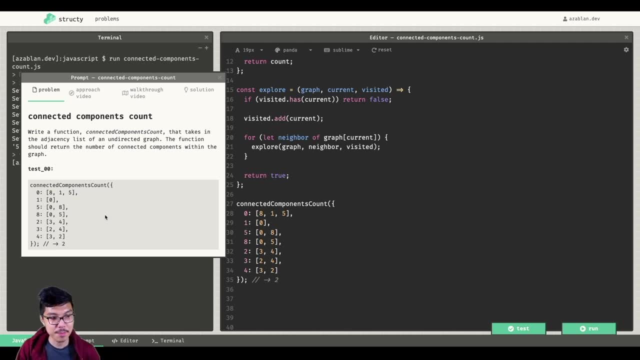 of our items of the set are strings, like zero is a string And other times they're actually numbers. notice that they're missing quotes. that has to do with, you know, kind of just JavaScript objects. technically, keys of a JavaScript object are going to be always converted as strings. 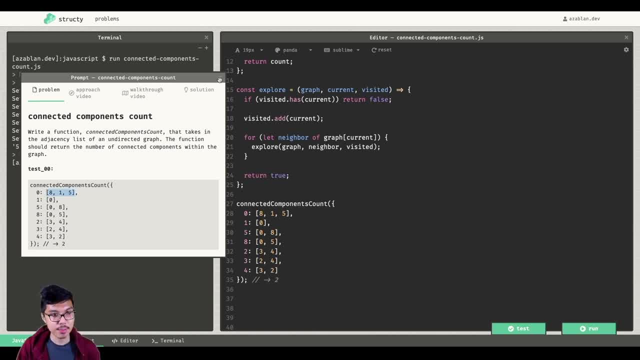 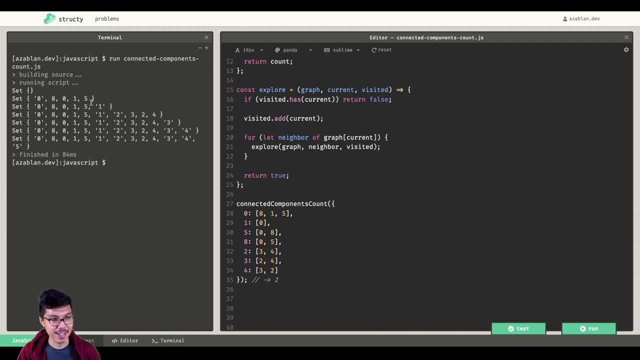 although the data within these arrays over here is going to be number and sets, can actually store both types, And so if you have like two different types, it's not gonna be able to figure out like that those really represent the same node, For example. 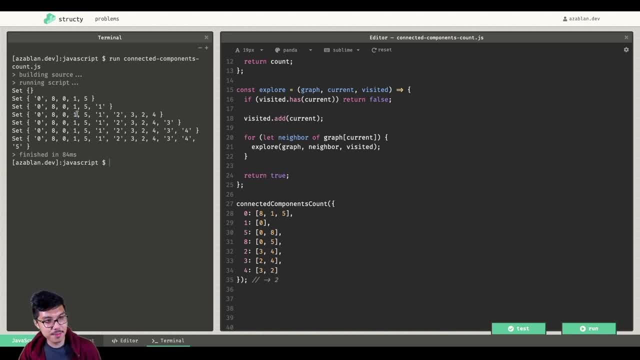 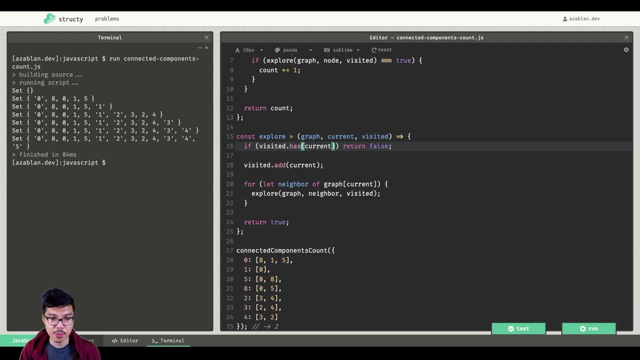 looking at this visited set over here I have, like the number one as well as the string of one, which is no good. So let's just convert them all to maybe strings. So I'll check visited if it has the string version of my current node, So I'll just do the conversion for me And likewise. 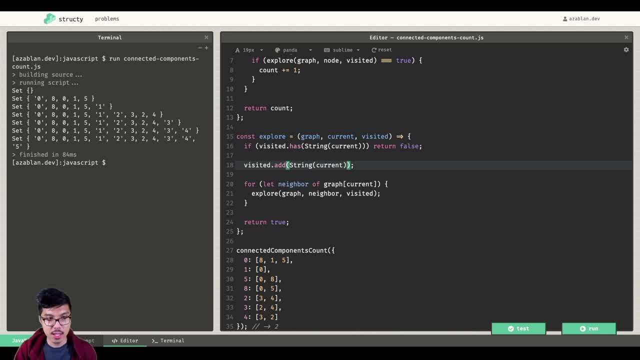 I want to add the string version of the current node over here. that way have very consistent types. So let's run that manually again. should just see all of our strings now. Awesome, And I think we can run all the test cases. So that's a really important thing to know. So let's go ahead. 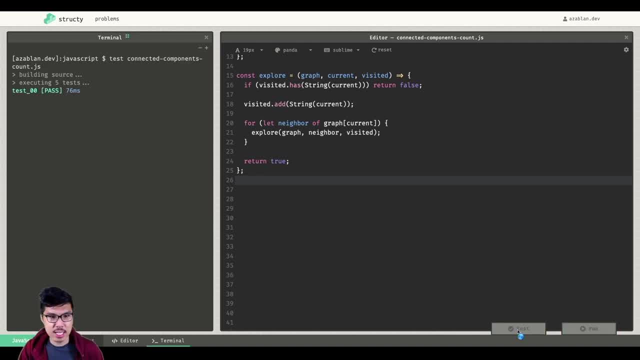 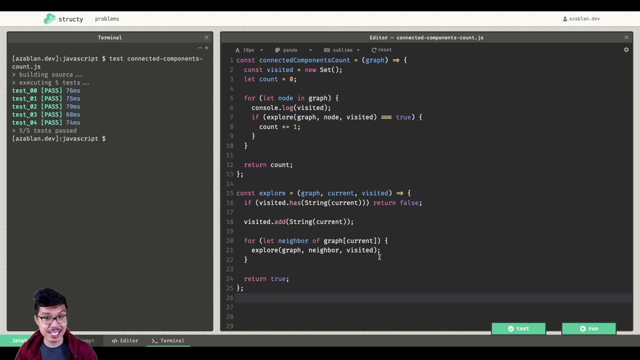 and go ahead and run that. So this is actually an important thing to watch out for in JavaScript- And JavaScript is pretty unique in that regard. I just automatically converts all of your keys into strings. Awesome, All right programmers. that's all I got for this. connected components count. 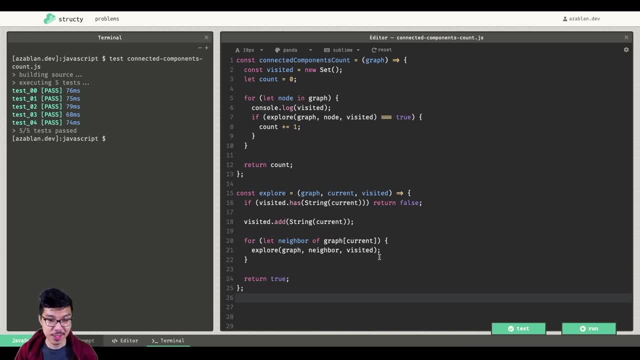 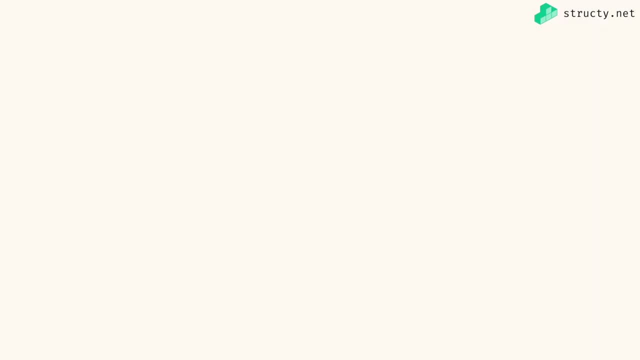 problem which you want to do is really practice this problem. It's actually a very, very common interview question And there are many variations of this problem that we're going to do in the future. Hey, programmers, Alvin here, right now I want to go over an approach we can use for this. 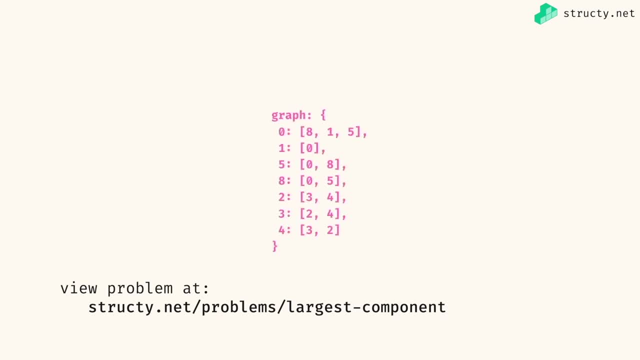 largest component problem. take in a graph, just like we've been doing as of late, And the first thing you should probably do is think of this graph as a picture. So hopefully you drew it out So you can really understand what this is asking. Our graph information is already given as an adjacency. 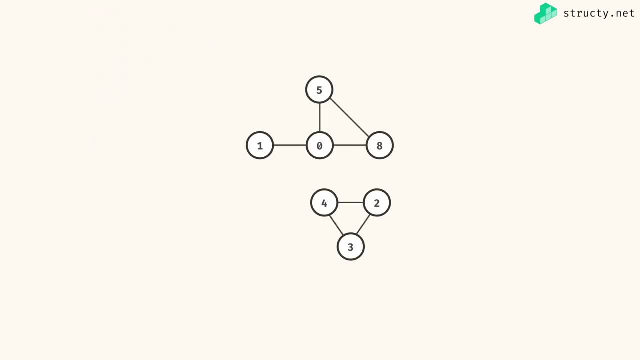 list, So it's pretty easy to draw out. So, since I have a graph like this, the first thing I should notice is it could contain multiple components, right? So here I kind of see two separate islands, two separate components, And I want to consider the sizes. 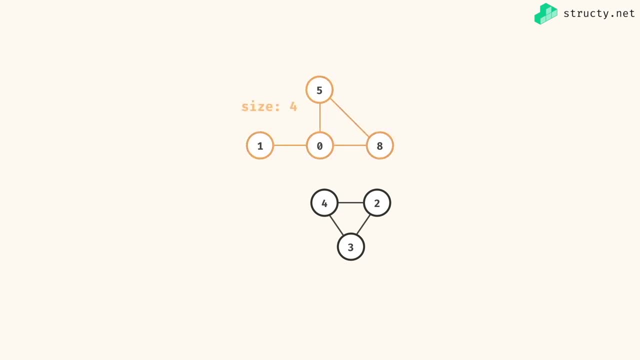 of each respective component. So if I look at my first component spanning the nodes 015 and eight, I know that they have a size of four. they are. the four represents the number of nodes within that component. So I'm really interested in the number of nodes. 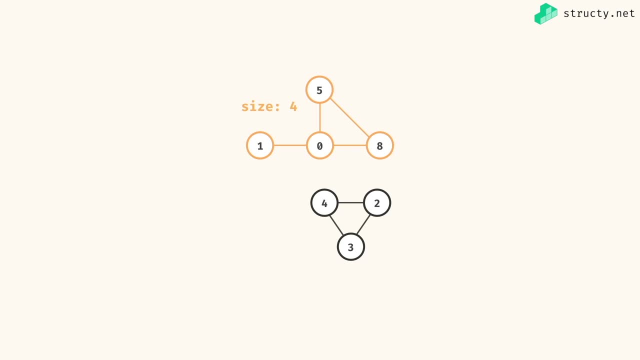 of a component, not necessarily the number of edges. If I look at the other component that spans the nodes two, three and four, that definitely has a node group of three And this problem really cares about the largest component. So I should just return four because 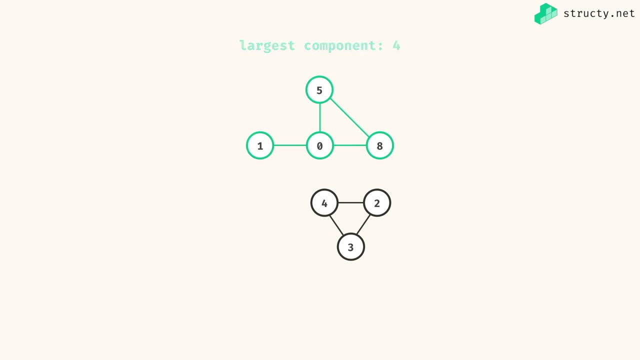 it's the largest component size. So, when it comes to what this question is asking, you do have some familiar patterns if you've been following these problems in order- And, of course, I always recommend that you do these problems in order. So how can we go about solving this one? Well, I know. 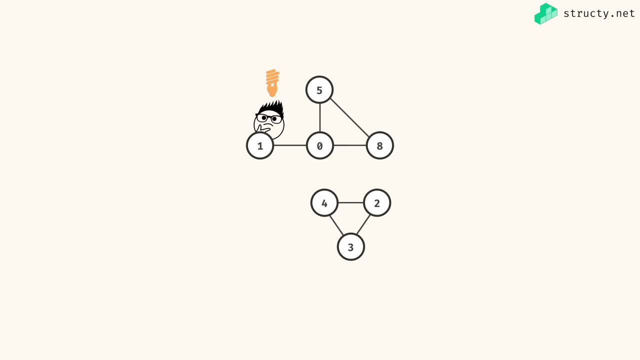 I'm going to need some sort of iterative code. that way I can travel and hop to different components or different islands And I can probably do some depth. first, traversal variation that also finds the size of a connected component. So let's step through how this algorithm might. 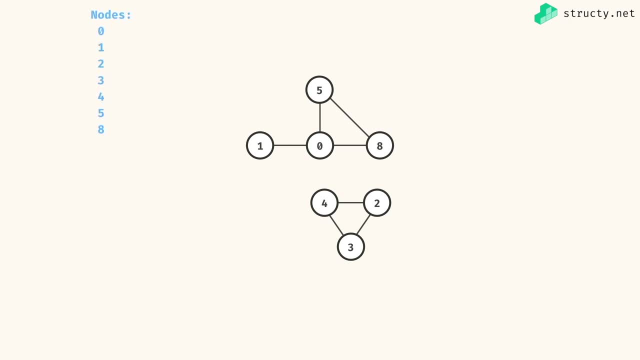 run On the side. I'm going to list out my nodes to represent how I'm going to do my traversal. I'm going to do the iterations to begin a traversal at every node as my starting point. So I'm going to start at node zero And since node zero is unvisited right now, 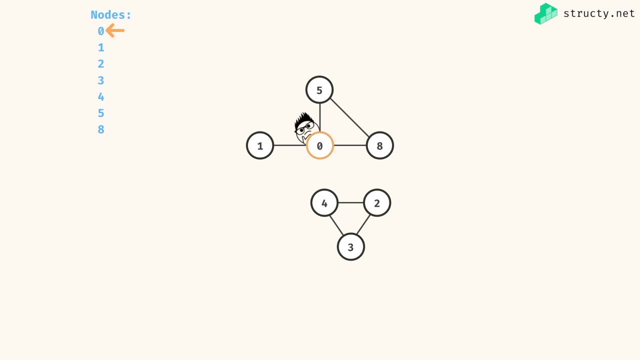 I'm going to begin a brand new traversal, starting at node zero, And I'm going to mark my nodes as visited as I go Because, like usual for our undirected graphs, you want to watch out and prevent any cycles that you may get trapped in, And I know that this depth first traversal- 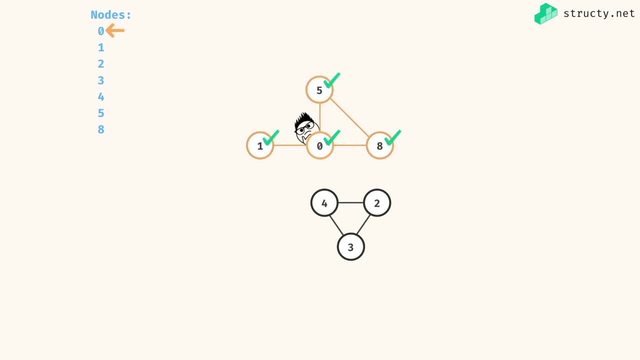 is going to explore this full region as far as possible, And by the power of recursion, it'll be pretty easy to implement some pattern that can count every node as we traverse through it. So I'm going to treat each of these nodes as just being a single node, of course, And 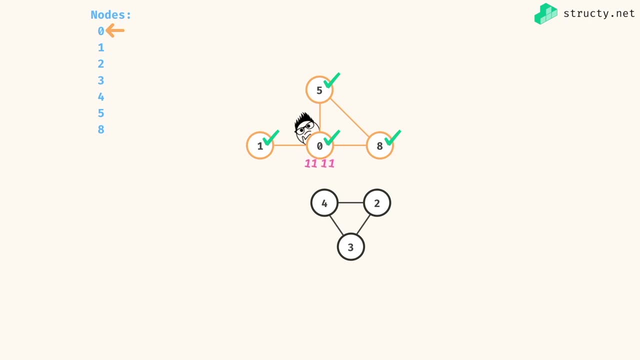 eventually, those ones are going to return to my top level column, in which case I can add them all up, getting me a grand total of four. If this feels very hand wavy and you're wondering, like how the heck are we going to code up that pattern, don't worry. 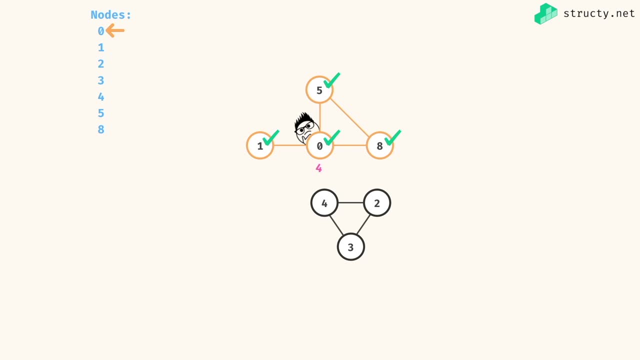 it's actually a pattern we've seen before, And so I'll cover that in detail in the code. Just know, for now it's actually not a big deal to get the count of nodes right, because it's not a big deal right. So now that I know that the size of this component is four, 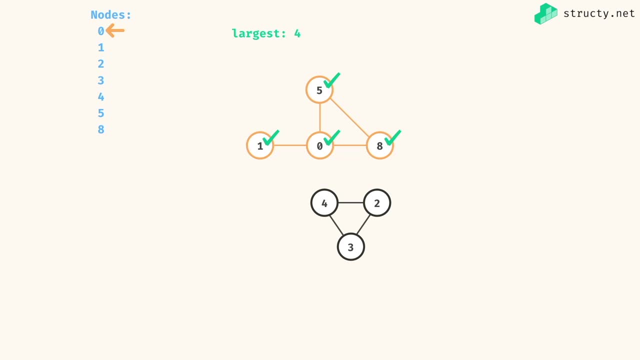 what I should do is, I guess, store it as my current largest island or component I've seen so far, because it's the first component that I've considered. At this point I should fall back to my iterative code, So I look at the node of one. what I should notice is: 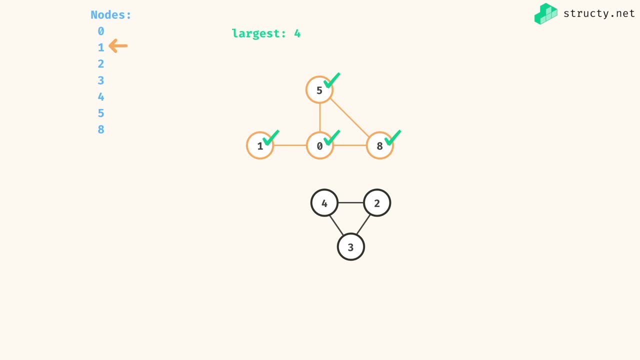 this node one is already checked off, right, it's already visited. So there's no reason to start another traversal from this node, Because if it's visited, that means I have already explored the component that node one One is a member of, so I can basically skip it, go on to node two in my iteration, since 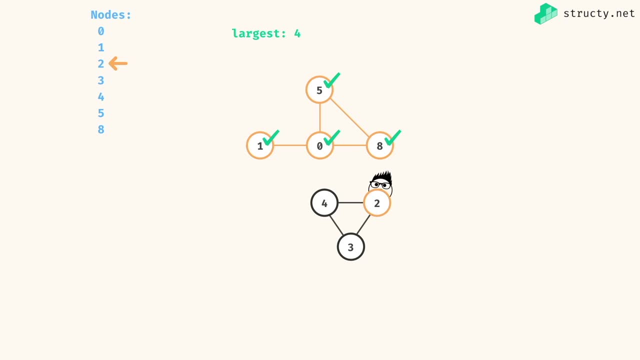 node two is unvisited. I should begin a new traversal over here. I know that this depth first reversal is going to explore that component as far as possible And it's going to go ahead and count all of those nodes as one and eventually sum up those counts together, giving me accounts. 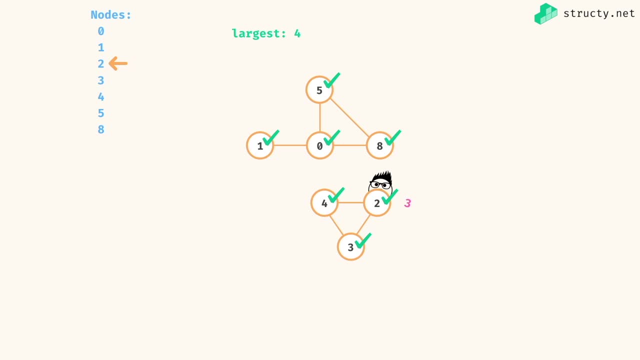 of three, And so this next component has a size of three. I need to compare that three against my current largest of four. obviously the four is bigger, so the four gets to stay as the largest. When I fall back to my iterative code, I get to my node of three. three is: 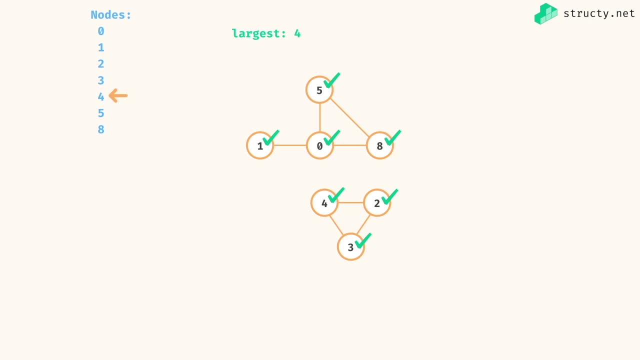 already visited, So no reason to start a new traversal. Four is already visited, So nothing to do. five is visited And of course eight is visited as well. At this point we're done looking at every single node within our graph And we must have explored every single component. 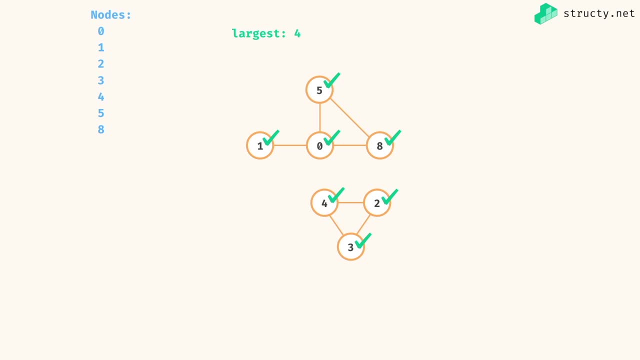 So we can just return the final value that we have stored in that largest variable. Awesome, When it comes to the complexity of this algorithm, it's pretty straightforward And it's pretty easy. It's basically exactly all of the algorithms we've seen so far. we say that n is the number. 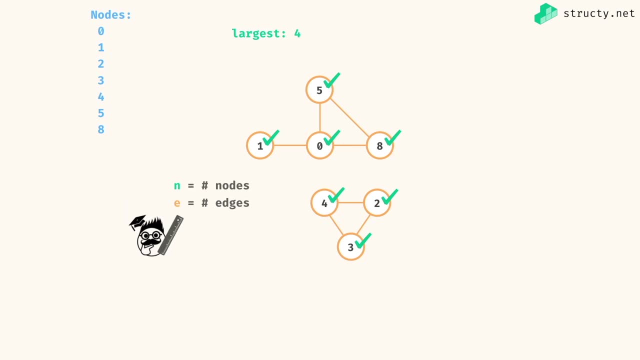 of nodes and ease a number of edges. we know that the time complexity is going to be roughly O of the number of edges. really, just exploring through the entire graph, we can also say that the space complexity is also going to be linear, really just O of n, Because through 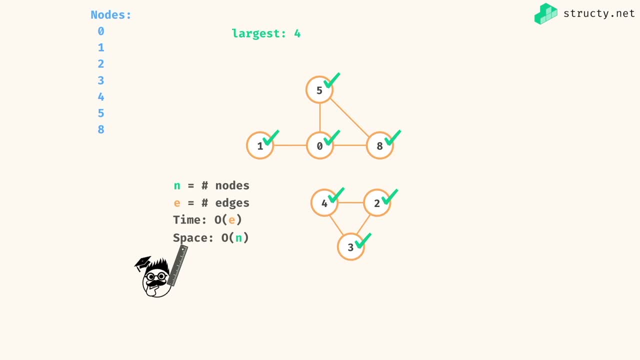 all of this. we're probably going to be storing all of our nodes in a set right to track visited And depending on how you implement your traversal algorithm, whether you use a depth first or breadth first, you're also going to use a linear length first. you're also going to 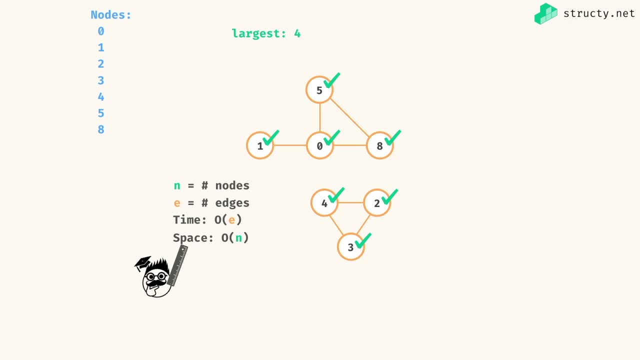 use a linear amount of space through your stack or your queue. So, overall, we're looking at a very efficient linear solution, And so, with that, I think I'm ready to code this one up. What I want you to do, though, first, is possibly give this one a shot on your own. 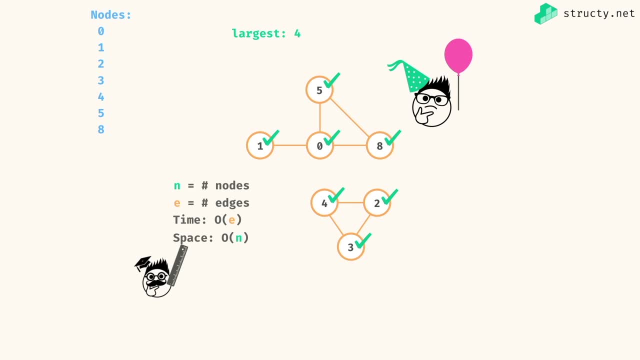 first, because we're really just utilizing some code that we've seen in the past, So give it a go on your own. If you get stuck, you can find me in the walkthrough video. I'll see you there. Hey, programmers, Alvin, here Right now let's go over a JavaScript solution for this largest 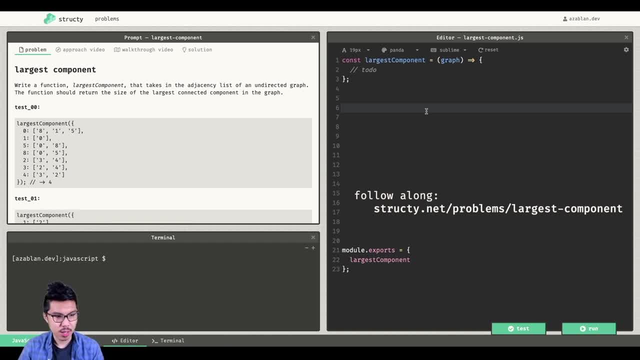 component problem. So this problem is going to be really just a spinoff of our last problem. So we'll hop right into it And, as always, make sure you watch the approach video first, And we'll start by building our code that. 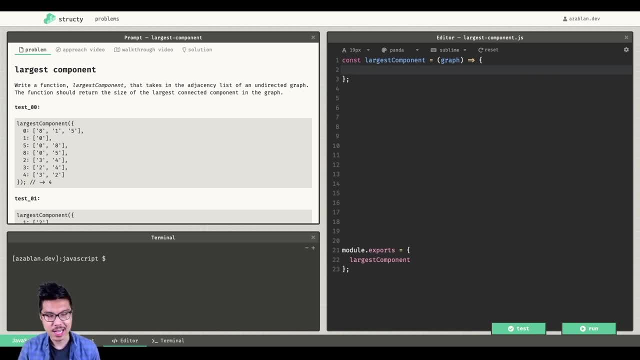 will help us start a traversal on disconnected islands here, right, Disconnected components, we should say. And so I'll start by iterating through every node of the graph. That means I just iterate through the keys of my input. object here, Because, remember, we're given. 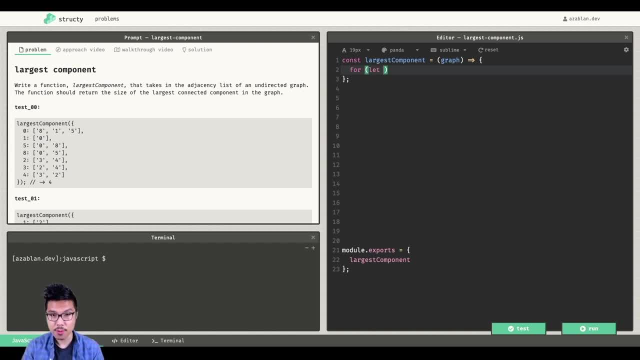 this graph as already an adjacency list. So I can say: for, let node In the graph, so I'll give me the nodes like 015, and so on, And what I'll do is I'm going to start a traversal here, right? So I'm going to pretend I had a function, I'll call it. 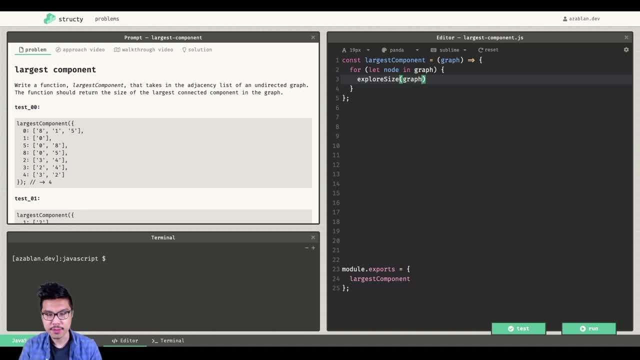 explore size And if I give it the graph information as well as the node that I want to traverse through, hopefully it actually does a traversal through that entire connected component right, And what I'm going to assume is: let me assume that this function actually returns the function. 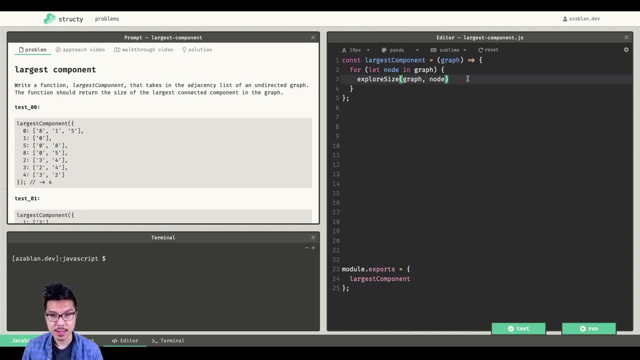 It returns the size of that entire component. So that would be a number right representing the number of nodes in that component. And so if I had that should receive it here. call it size And I know I need some like max value logic for this entire for loop. 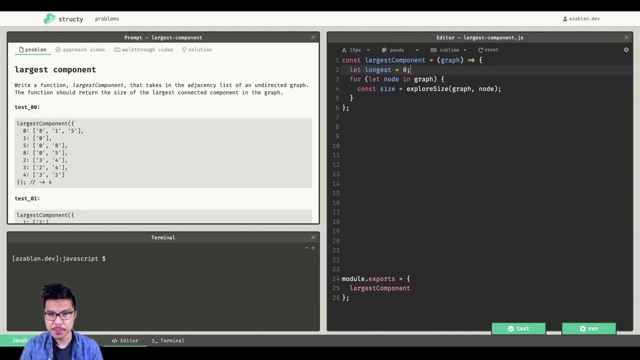 So I'm going to create that longest, initialize it to zero And then from there I can check. all right, if the size of the component I just found, if it's bigger than the longest, then I can replace the longest, simply longest. 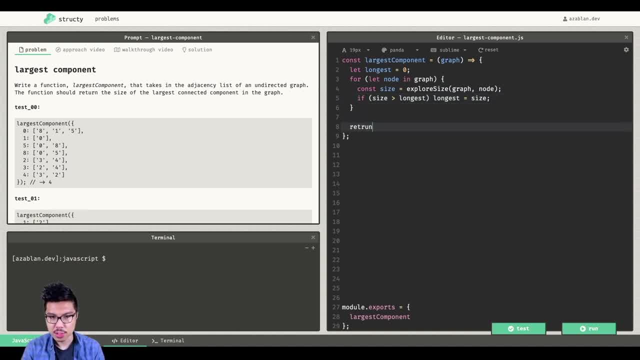 equals size And after the for loop I would just return the longest course. I need to write this explore size function, So I'll implement this as a type of depth first. So I'm going to make it recursive explore size, taking the graph as well as our current node. 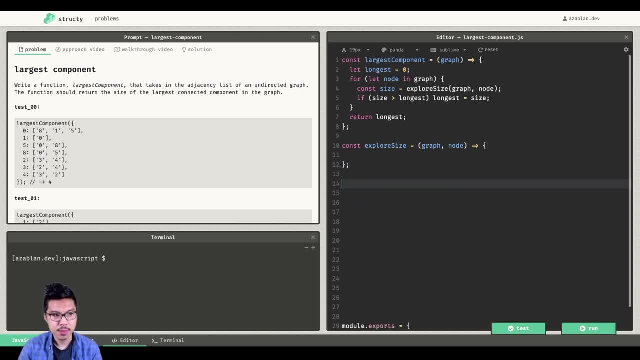 And a few things I should watch out for. here. they tell us that we have an undirected graph, And so we need to make sure that we avoid any cycles. So what I'll also set up here is some classic structure. I'm going to use a visited set. 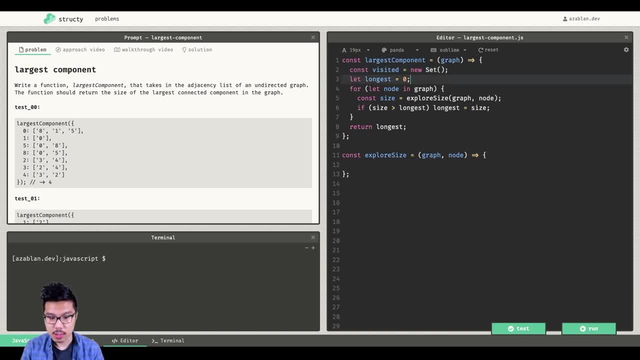 I'm going to use a set because it gives me O of one lookup and O of one insertion. So now that I have my visited set I can pass it along as I start those reversals. And now let's work on a base case. So I'll do to get going. is a check if I visited this node already? 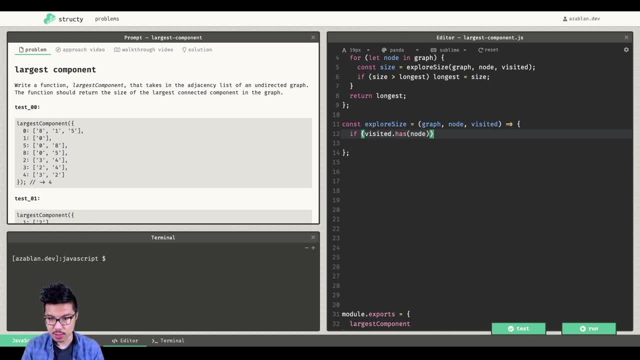 So if the visited set already has this current node, then I need to return, basically avoid a recursive call. But I also want a consistent type here, right? So I'm assuming that this function gives back a number representing the size, at some point in my traversal, if I get to a node that has 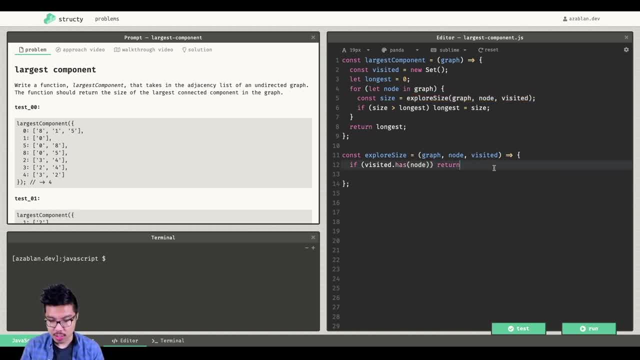 already been visited. that means I counted it already, And so I'll treat it as zero right now, because I don't want to double count my nodes right, Otherwise would be inaccurate here And now. beyond that, what I can do is maybe create a variable here. I'll call it. 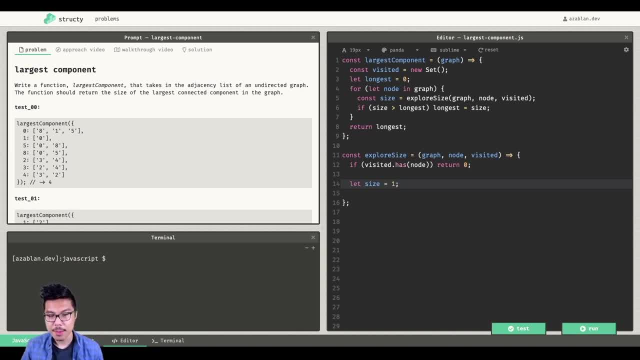 size. I'm going to set that equal to one to represent the current node I'm on right now, right? If this condition is not true, then it's the first time I'm seeing this node, So I need to count it. I will also be sure to do is. 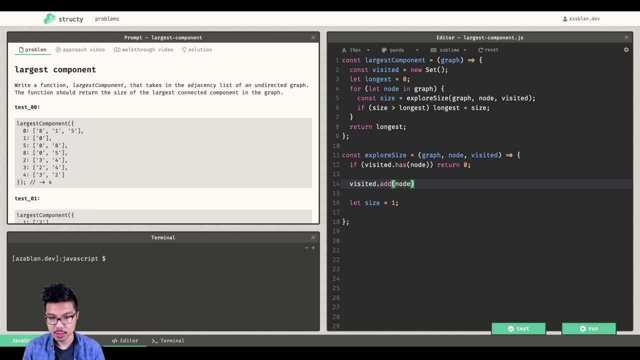 add it to, visited. that way I don't get into a cycle into the node later on Nice. And at this point I need to make my recursive call on the neighbors of the snow. So, like we usually do, we could say, for let neighbor of the graph of node, So remember your shape. 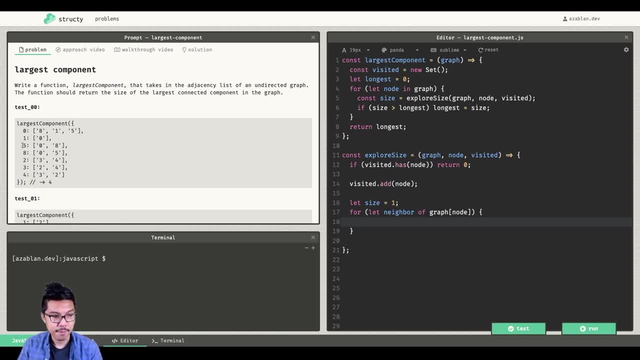 of data here. So if node was a key like five, when I say neighbor of graph of node, that would iterate through the neighbors of five, so zero, and then eight and so on. And so here I make my recursive calls. I'm going to call the same function: explore size pass. 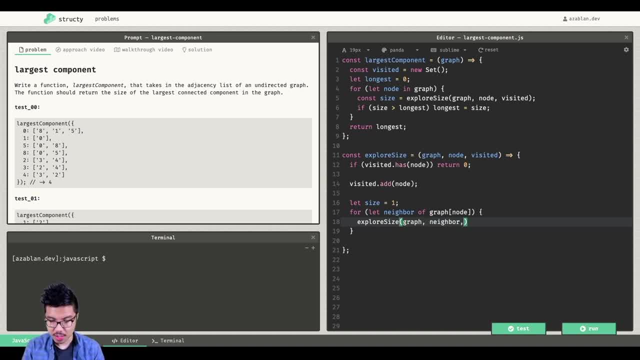 along the same graph, But now you're situated at your neighbor, you can provide the same visited set. And here's where I do my recursively buffet thread. I'm going to assume that this explore size function is working. So if it was working, what would it give back? it would 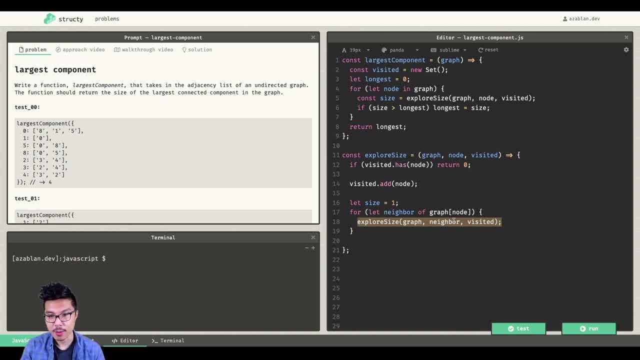 give me back a number representing the size of that graph, right beginning at my neighbor. So whatever number I get back here, I just want to increment my size by that Right And that would accumulate a, basically a count of all the nodes in this fully connected component. 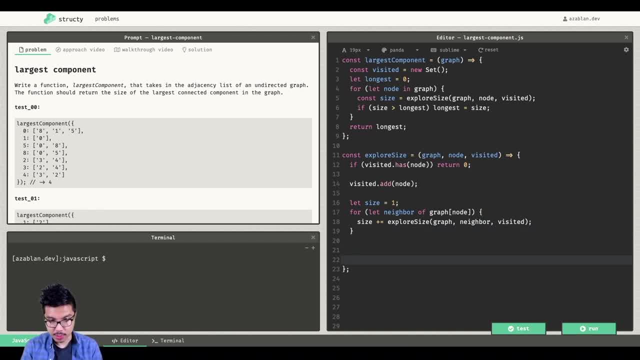 And after I'm done exploring my neighbors, I would have explored the entire component fully, So I can just return my final answer, which would just be the size over here. Really important thing you need to do is make sure, if you follow this kind of strategy, you start. 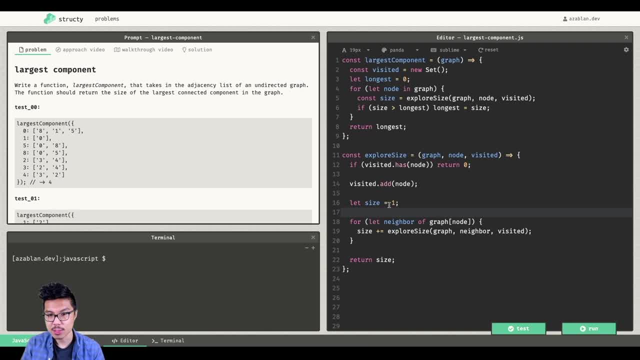 your size equal to one and you add to it over time, Because this one is going to be the size of the node There's going to be. an additional one represents the current node that I'm at. I know that every call is going to count its. 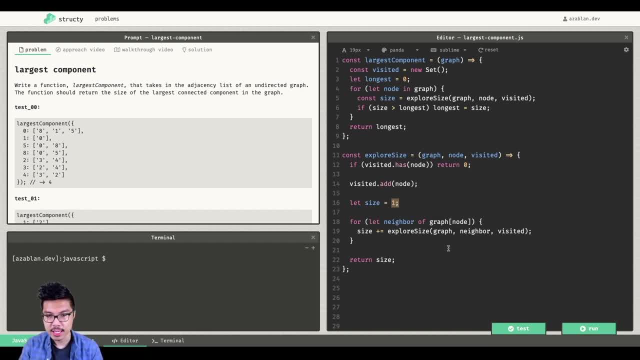 own node. So over time this will actually accumulate everything I need. So that feels pretty good. We have our nice visited logic And we already wrote our main function here. Notice how we're splitting up this code in a nice little helper function here. I think. 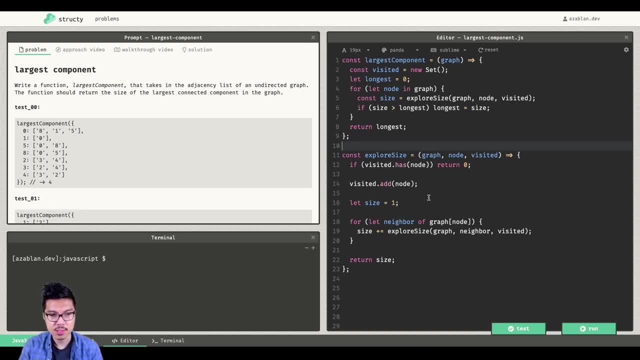 it's the best way to express this, And it's very similar to some previous problems that we've done. I think at this point let's go ahead and give us a shot, See what we get. should be able to put it through a few different test cases. Nice, And there we have the largest. 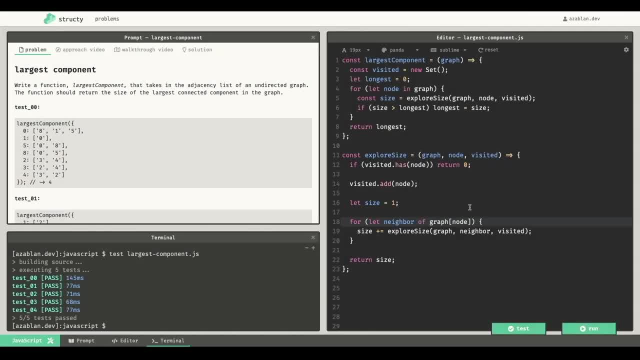 component problem. So a few things. I want to draw your eye to remember that for your graph problems where you have disconnected components, you're going to need not only your traversal code but some just iterative mechanism, usually just a loop, to make sure you can hop to different components right, Because if you only had your regular like. 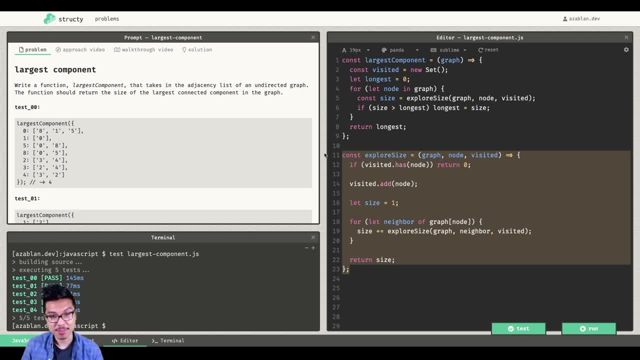 traversal function. by definition, there is no edge between separate components, So you would never be able to Speaker 1, explore the full graph, Otherwise, all right, programmers, practice this and I'll catch you in the next one. Hey, programmers, Alvin, here, Right now, let's go over an approach. 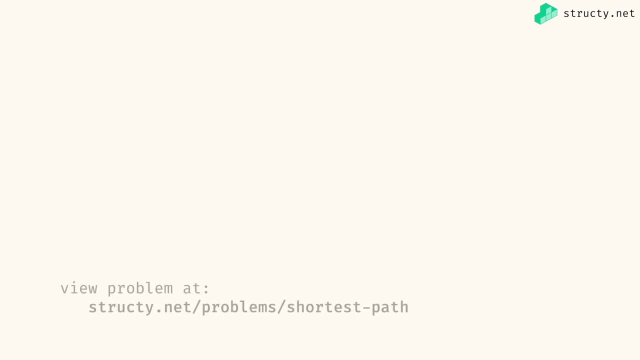 we can use for the shortest path problem. So here we have another graph problem, and your graph is going to be given as an edge list. So the first thing you should probably do is, of course, visualize this graph And in the context of your code it probably would. 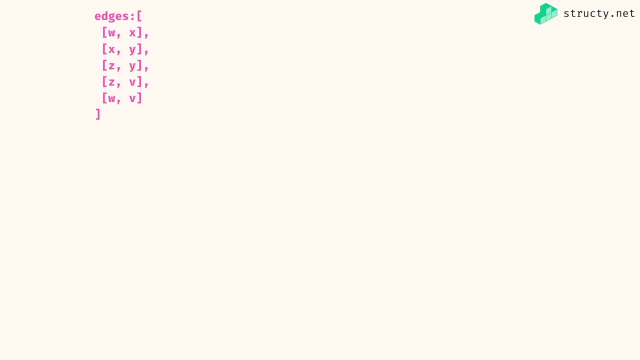 be best if you convert it into an adjacency list. Since we've seen that pattern a few times in some recent problems, I'll leave that part to you. But we're going to end up with a graph that looks like this, And in this problem we're also going to be given a two nodes here, let's say w and z. 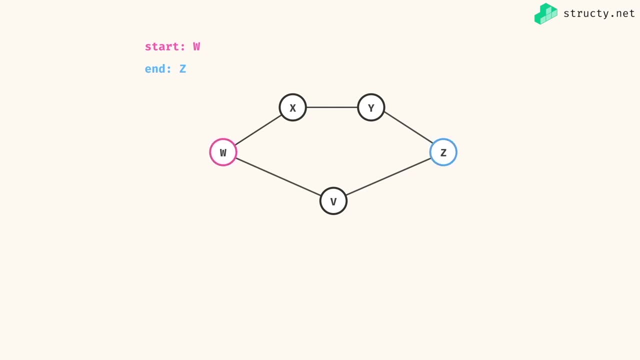 what I want to do is return the smallest path between these two nodes, And here I have two obvious paths right. One way I can get from w to z would be to go through x and y, And there I can see that that path length would be three. do note here that we're going to 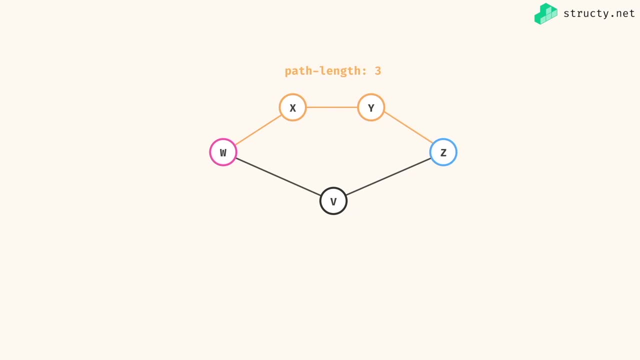 consider the path length as the number of edges within the path, So not the number of nodes, right? So that means how do I calculate three here? what's really just two nodes, three lines right, three edges. that's one way to get from w to z. Another obvious way: 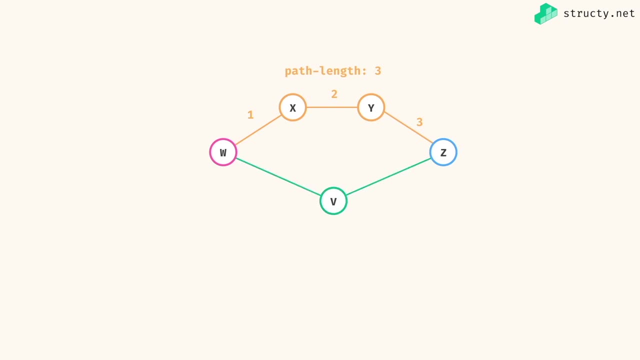 to get from w to z would be to go through v, in which case I would only need to use two edges. So that path length is, of course, two. And this problem. what I want to do is return the smallest possible path length, So I should return the final answer of two. 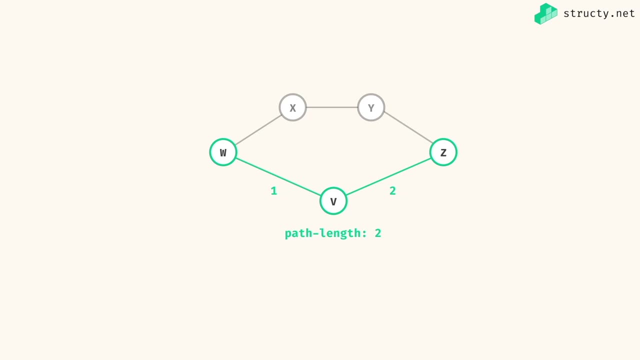 here. So we know that this problem is going to require us to do a graph pathfinding algorithm, And the question is: which one should we take? We either can choose, of course, a depth first reversal or a breadth first reversal. 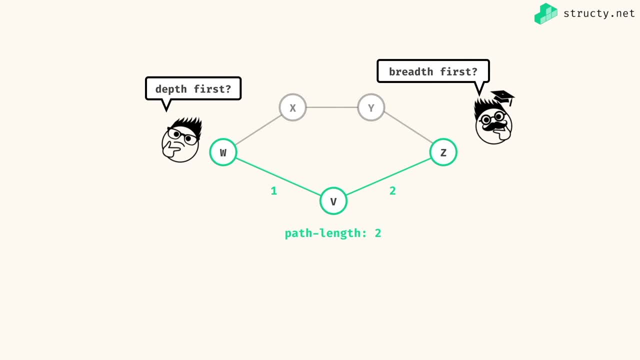 I'll cut to the chase here- And both of them would actually give you a strategy that works, meaning you can solve this with either a depth first or a breadth first strategy, But maybe one of these algorithms would be better than the other. So let's consider the possibilities. 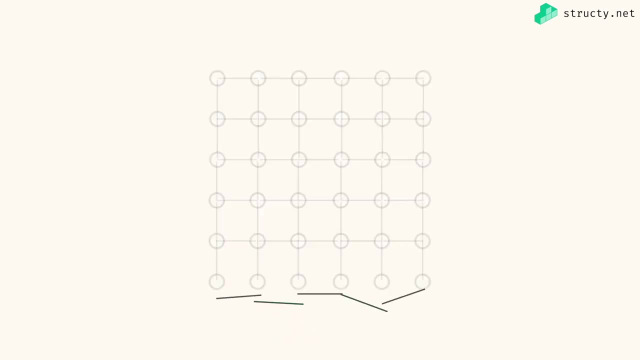 So let's say I had some large graph. we'll think abstractly right now, So kind of just looking at an abstract example. And let's say I was stepping through some depth. first traversal: let me say I have my starting node in yellow and I'll have my target node in 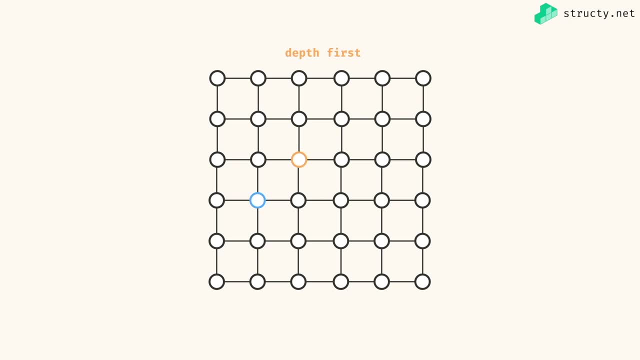 blue. So what I want to do is again figure out what's going to be my starting node And what's the minimum path distance between these two nodes. Obviously, you know, just in the long run, you should get an answer like two here, right, Because two is definitely. 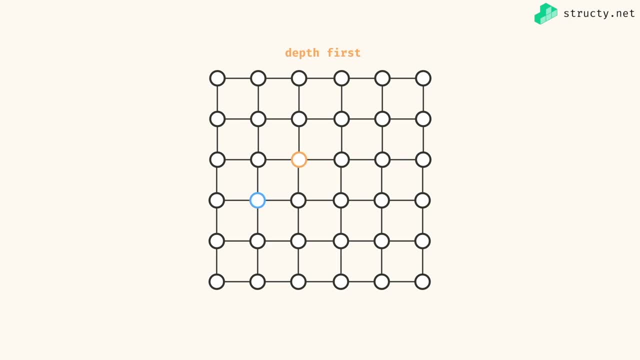 the shortest path between these two nodes. If we did a depth first traversal, I know that depth first would force me to look in one direction as far as possible until I have to switch directions right. So from my starting node in yellow, let's say we move. 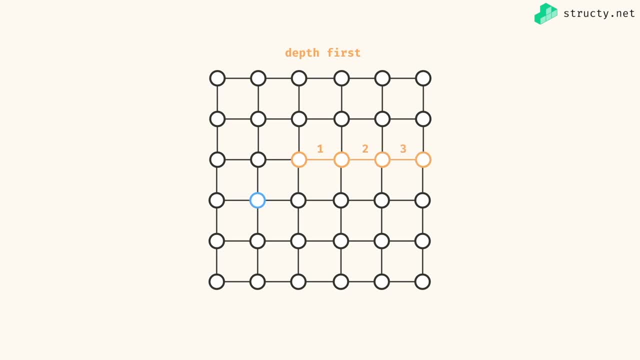 to the right, that'd be one edge- and move to the right, again two edges, move to the right- again three edges. At this point I can't move right anymore. So let's say we move downward- Four, five, six, have to switch directions, again seven, eight, And at this point we 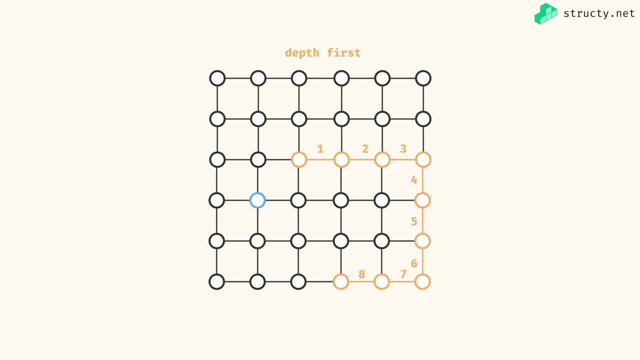 kind of already see that this is going to end up possibly getting to the blue target node, but it wouldn't be the shortest path. Something unfortunate here is, although my start and end nodes are really close together, a depth first traversal could be unlucky in. 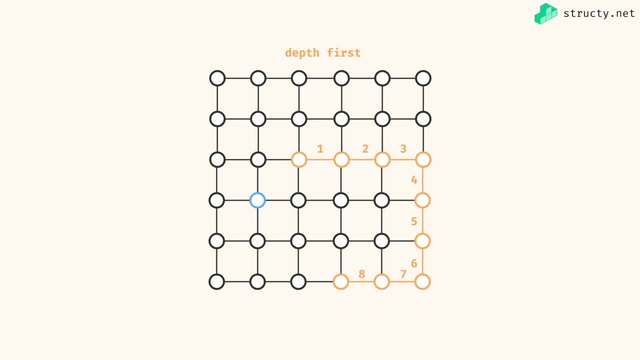 that it may search in a totally wrong direction and snake all the way through the graph until it eventually finds my target node, at which point I definitely don't have the shortest path. So I think a breadth first traversal is going to be more useful here. So let's say I started. 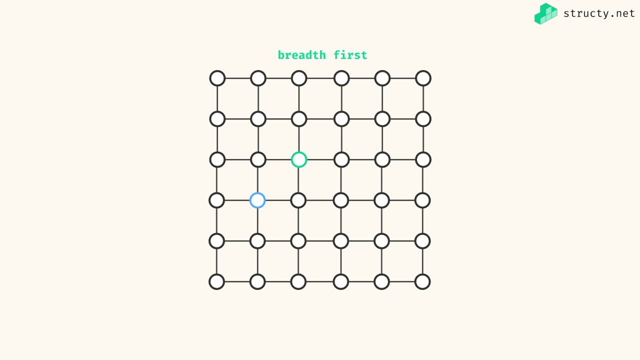 at my green node- still my same starting point- And if I did a breadth first reversal, I know that breadth first means I'm going to explore all the directions very evenly. So it would look like this: So I would explore all nodes one edge away from my starting point And 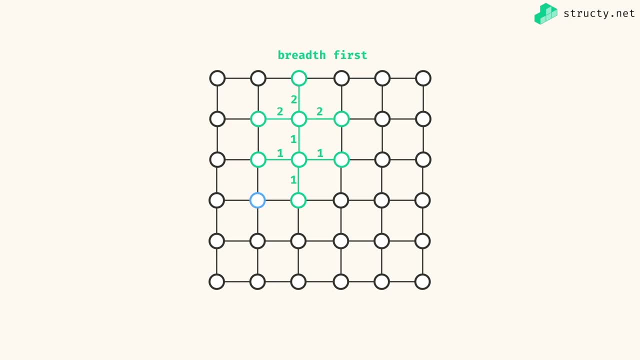 then from there I would begin to explore all nodes, two edges away from my starting point, And at some point I'm going to hit my target node. And if it's the first time I'm seeing my target node, then by definition I must. 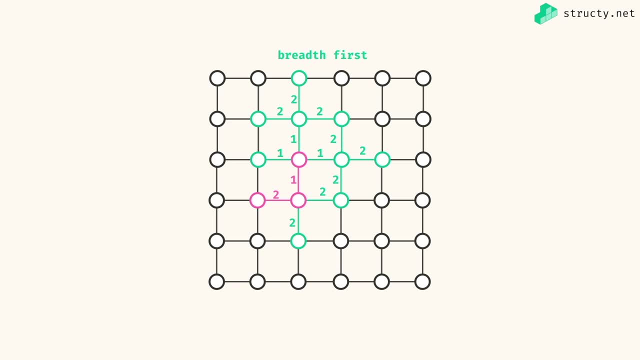 have just found the shortest path. right, the shortest path would just be two. So that's my high level argument for why a breadth first search is going to be more useful, in my opinion, for this problem. Let's step through this process a little more algorithmically, So. 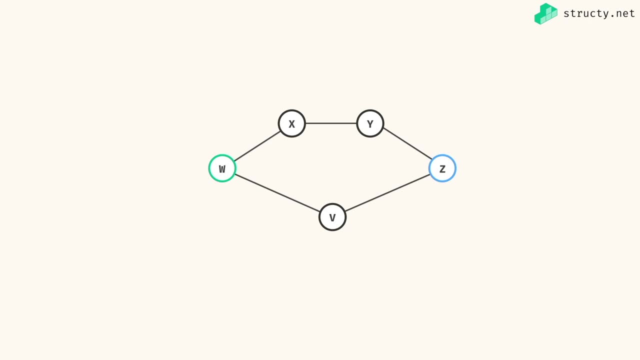 let's say, I had my original graph And if I'm going to do a breadth first traversal, I know that I have to use a queue, right, no matter what a queue is what gives you that breadth first order. And what I'll do is, as I'm going to do, a breadth first traversal. 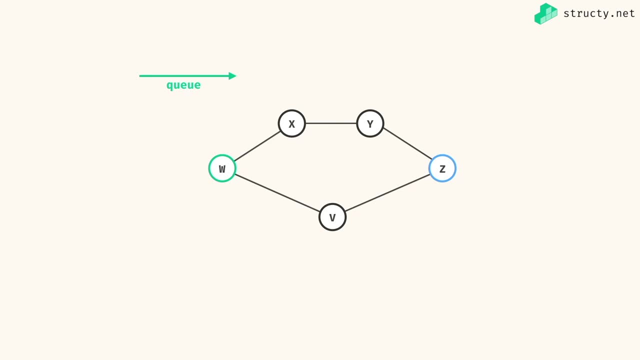 is the items of my queue. I'm going to store not only the nodes but also the distance from my starting point. So that means I'm going to initialize my starting node on the queue along with the distance of zero, And that represents the fact that all right, that 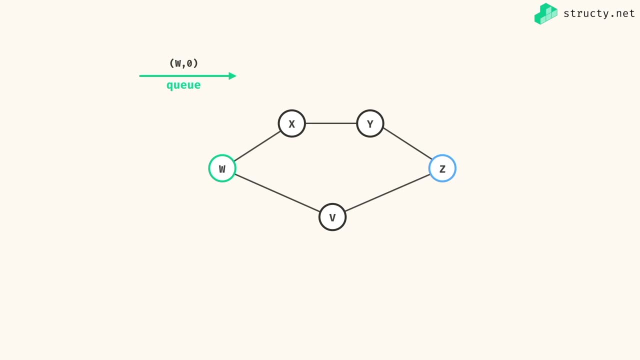 node of W is zero edges away from the starting point because it itself is the starting point. So any point in time, the items of my queue are always going to be pairs right of node comma distance. So now we can begin our general algorithm. I'm going to keep iterating while. 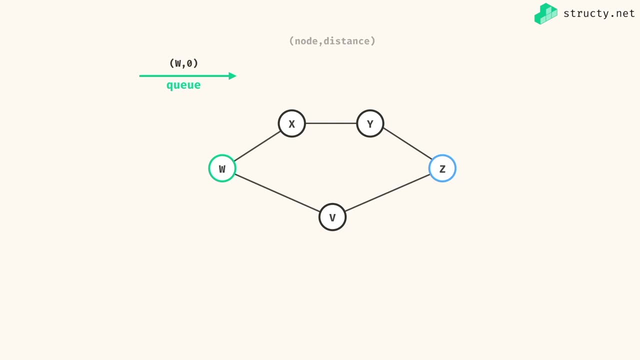 my queue is not empty. A single iteration of breadth first would remove the front item of my queue and I'll label it as my current node. At this point I should check: Alright, is my current node of W the thing I'm looking for? It's not, so I need to explore W's neighbors, So I can. 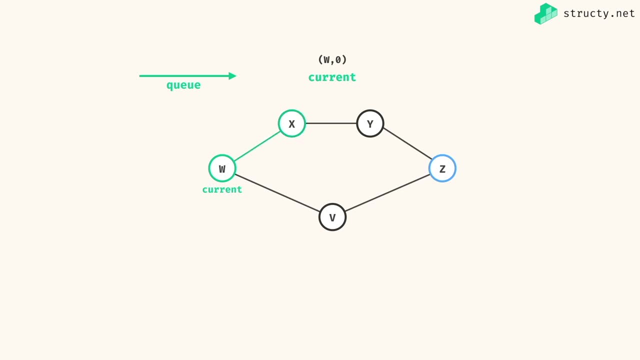 look at the X node And I know I need to add it into my queue. But when I add it into my queue I want to make sure I tag it with a distance. So if my current node has this zero, I know that a neighbor of this node would have distance one. So I just increment. I. 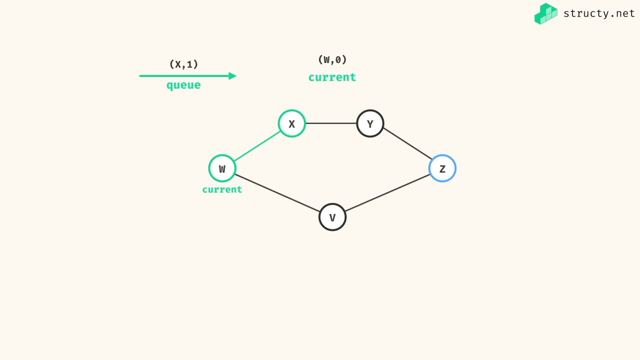 add the current distance by one. So onto my queue I put an item that says x comma one, And I have a similar scenario for this V node. it's also a neighbor of W And so I put V comma one on my queue as well. At this point I can go to my next iteration or move the. 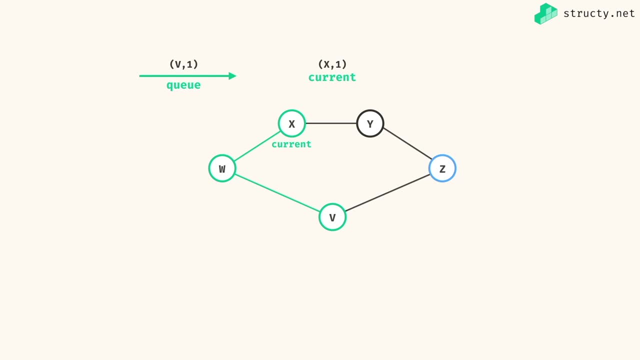 front of my queue, So I look at the X And then I look at X as neighbors. do bear in mind that, because I have an undirected graph here, X really has two neighbors. right, it has W as a neighbor as well as Y. So something you should already know is that if you have 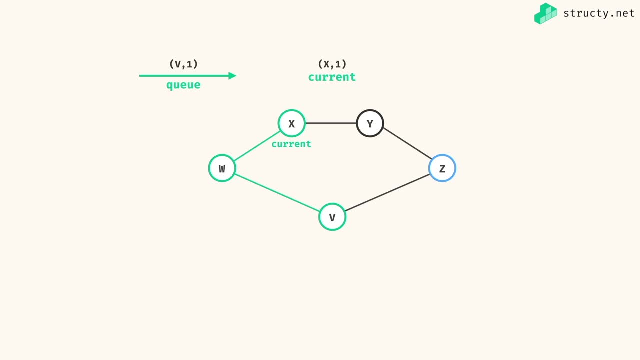 two neighbors you should already know is I need to track visited. In other words, when x is going to consider its neighbors, it should really only care about the y right. I don't want x to put W back on the queue because then I would get an infinite cycle. So I'm 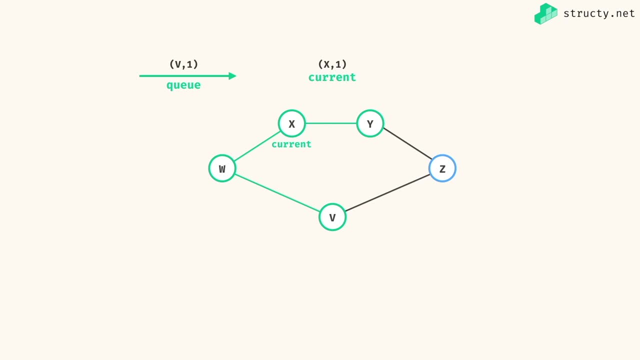 just gonna look at the y over here. I'm going to add it to my queue Because I know my current node of x has a distance of one. y must have a distance of two, always just incrementing the distance by one. Cool, And then I'll carry on with this algorithm. I remove the front. 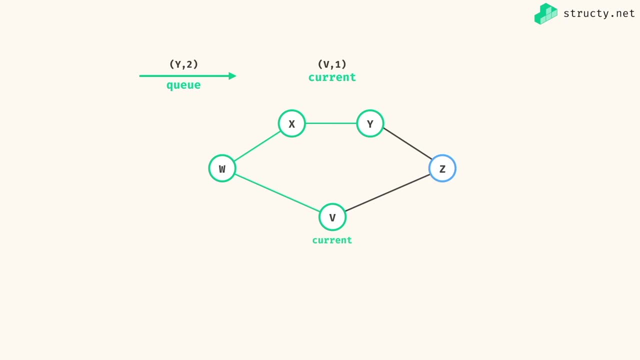 of my queue Now, which would be the V node, And at this point I can consider these neighbors, And I do see that one of its neighbors is actually the Xena. that's the only unvisited neighbor. I'm going to be sure to add z into my queue and tag it with a distance of two right. 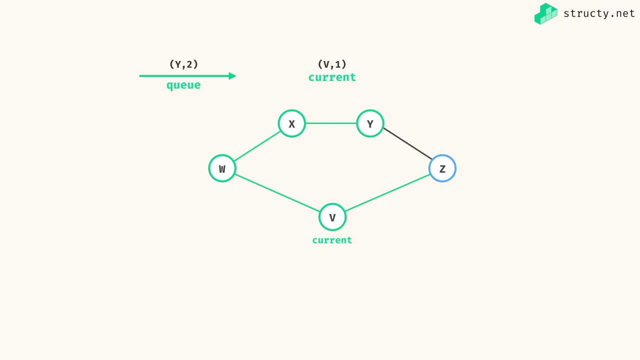 Because if my V has distance one, its neighbor would have a distance of one greater. At this point, you can already see how this algorithm is going to work out. Eventually, this Z node is going to leave the queue, And that would actually be my target node. So since I've 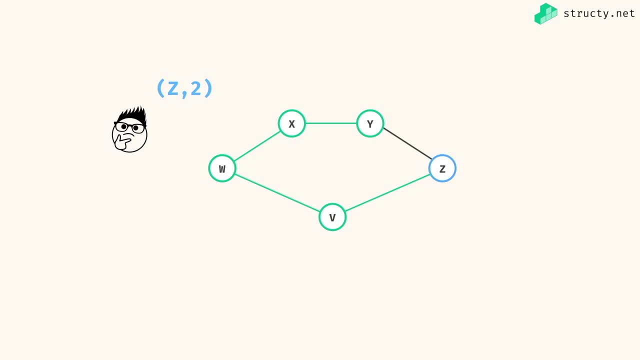 added a node to the queue that matches my target. I know I have my final answer. The two here does represent the number of edges we took in that logical path And I would, of course, just return that to. So for the most part, this algorithm just sounds like. 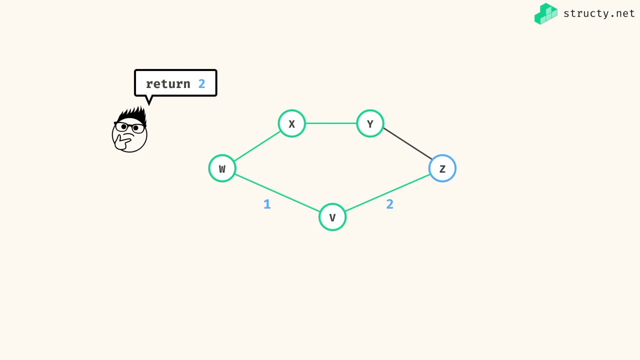 a classic breadth, first traversal using a queue on a graph. The only interesting bit is now we're also going to track the current distance. You know, when it comes to counting the length of a path, you need some counting mechanism, And so if you begin your queue, 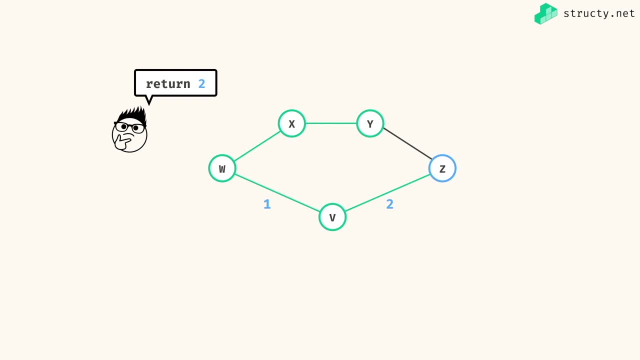 with your starting node with a distance of zero. every time something leaves the queue and adds its neighbors, it should increment that distance by one And, like you already guessed, this algorithm is pretty efficient because we don't have to traverse through the graph. 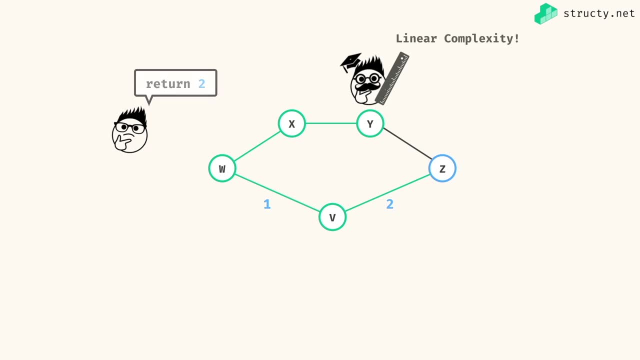 more than one, So we'll see that this has a linear complexity. All right, I think I have everything I need to code up this one. I'm sure you're wondering about these implementation details, So what you want to do is possibly give this implementation a shot on your own And, if you need some help, 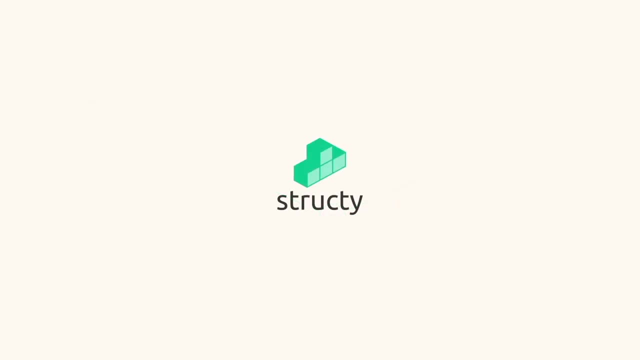 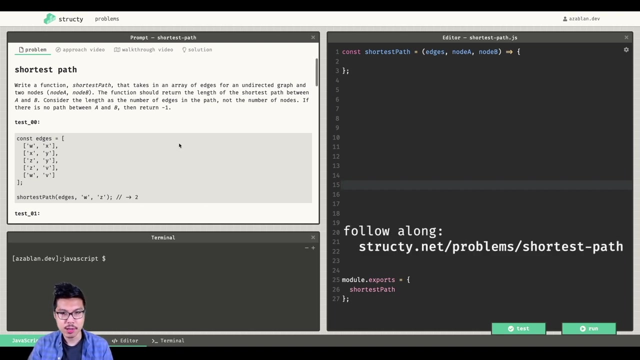 you can find me in those walkthrough videos. See you there. Hey programmers out in here, right now let's go over a JavaScript solution for the shortest path problem. So we'll jump right in, hopefully. watch the approach video. And so we'll start by converting our edge list input into: 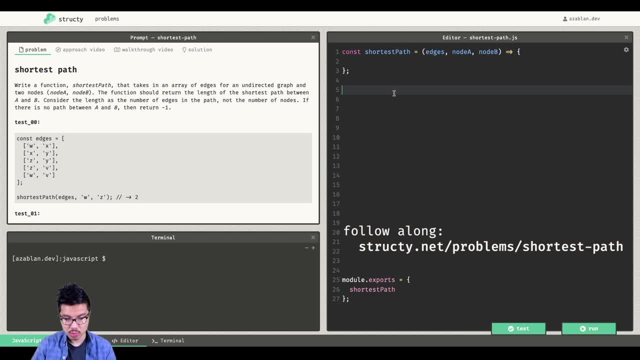 something more useful for a traversal, like an adjacency list. we're going to write a very classic function. we're going to call it build graph. like you expect, it takes in the edges and I want it to return an adjacency list. For me, that means a JavaScript object. I'll call it graph. 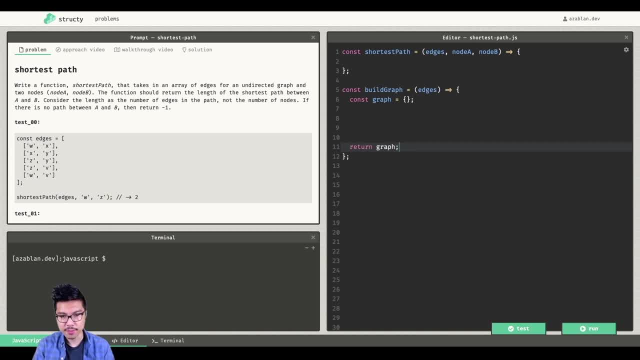 by the end of this function, this little helper, I'm going to return the graph And some common code. I'm going to iterate through every pair right, basically every edge. I'll say: for let edge of edges. And as I'm iterating through every edge, what I want to do is unpack that edge into its. 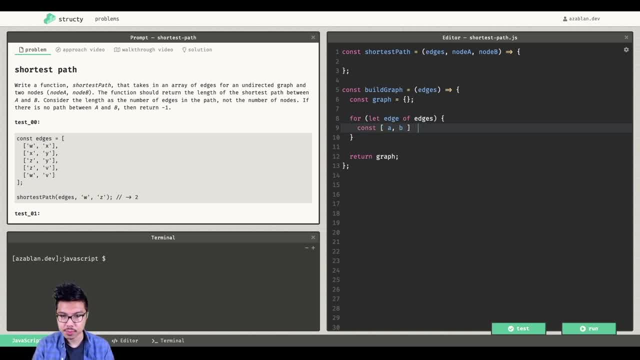 component nodes. I'll call it A and B, And now I can start formatting my adjacency list. So I know I want the keys Of this graph to be obviously the nodes. I want the values to be an array of the neighbors of that. 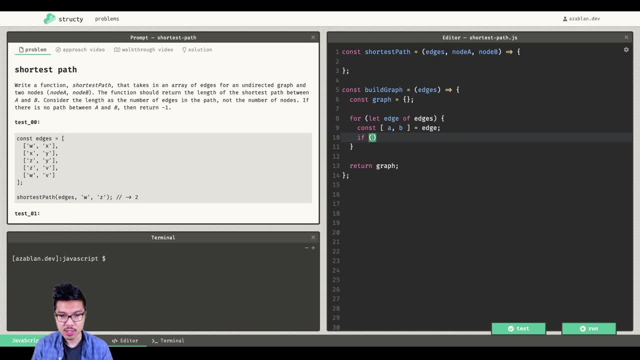 node. So what I'll do is, if it's the first time I'm encountering a node, I'll check. All right, if this a node, if it's not in the graph yet as a key, then I should create it for the first time. 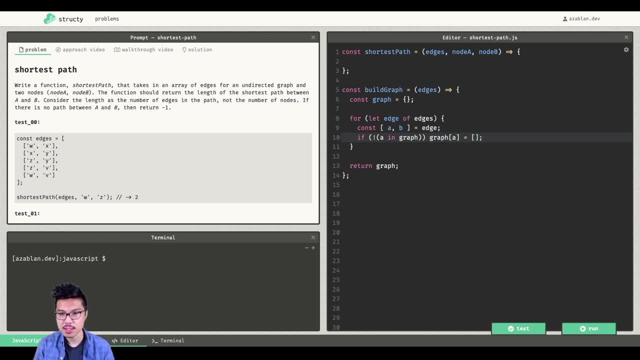 So use it as a key and initialize its value to an empty array. Basically, at the start it's going to have no neighbors. Likewise for B. And then at this point I know that A and B now definitely exist as keys now within the graph. 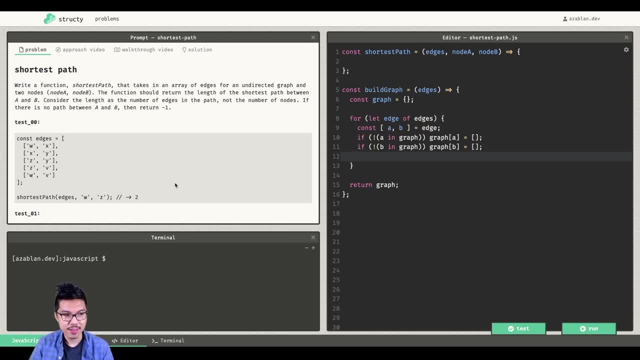 And so I just want to add those neighbors. So if I have an edge like w comma x, I know x is a neighbor of w and w is a neighbor of x. So simply put and say: graph a, dot, push B, And then just the inverse of that should be good to go, Cool. So that should give us our graph. 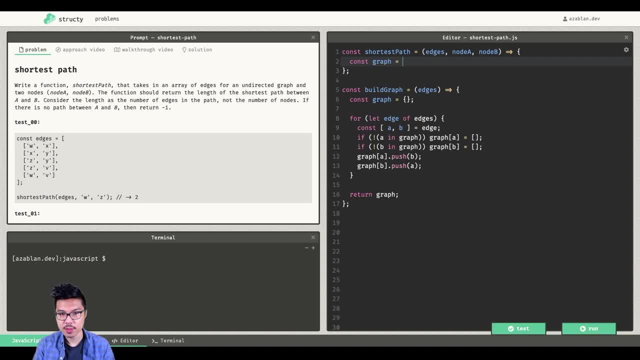 Let's go ahead and use that in our main function now. So we'll just say: graph equals build graph on the edges, And what we want to do now is actually work in our breath. first logic, like we said from the approach video. So a few things I'm going to need. I'm going to definitely 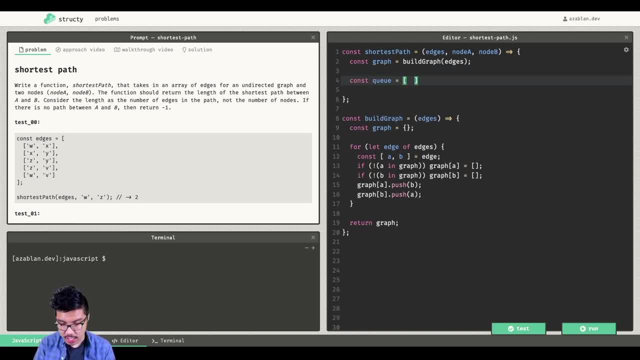 set up my queue, We said that the key to victory here was to not only store the node in your queue, but for every like frame inside of your queue also store its distance from node A. So I'll just use like a pair of things. So the elements of my queue are going to be always a pair And I'll throw on 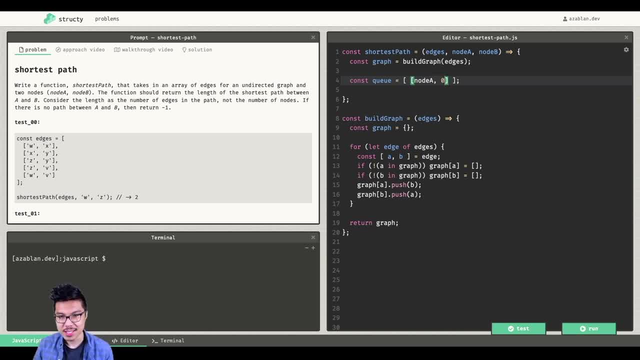 a second key, which is the initial node A and also the number zero, because at the start right this node A is zero edges away from itself. So that's good to go, And over time I'm going to be incrementing this number. it seems nice, And so let's keep on keeping on here. I'll. 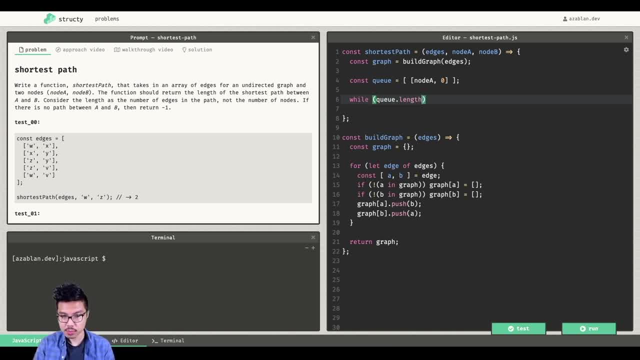 write a while loop. classic condition would be: alright, while your queue is not empty, then I shall remove something from the queue. So always remove from the front if you want to follow a true breadth, first order. so I can do q dot shift And that'll give me back an array right. 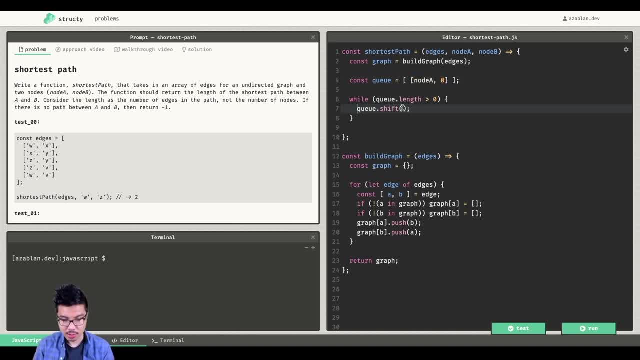 give me back one of these sub arrays here. I know it's always going to be a pair, So I can just unpack And I'll just say, Alright, grab the current node as well as the distance. Nice, I'm gonna check the node here that I just removed from the queue. If that node 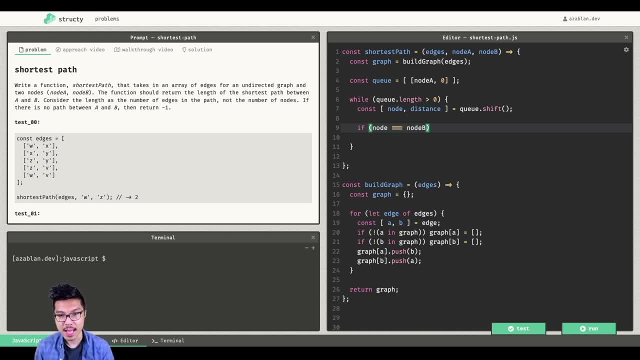 is node B, then I must have just found a path And I know the distance in that path. I can just return it. But if this condition is not true, then I need to keep searching through my graph. So that means I need to add this- nodes neighbors- to the back of the queue. 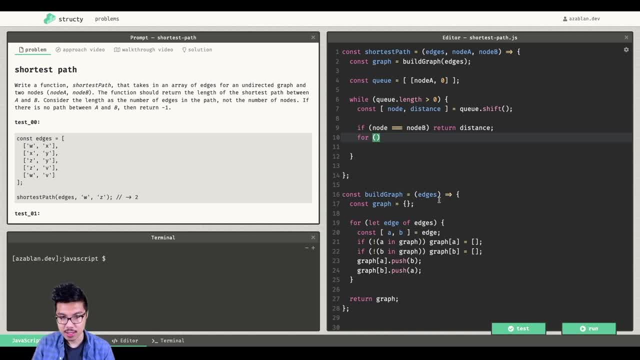 So I'm going to iterate- remember that we have an adjacency list the entire time. So I'm going to say, for let's say, neighbor of graph of node, so get all the neighbors of this node, And what I'll do is just add those neighbors into my queue. So q dot push neighbor. 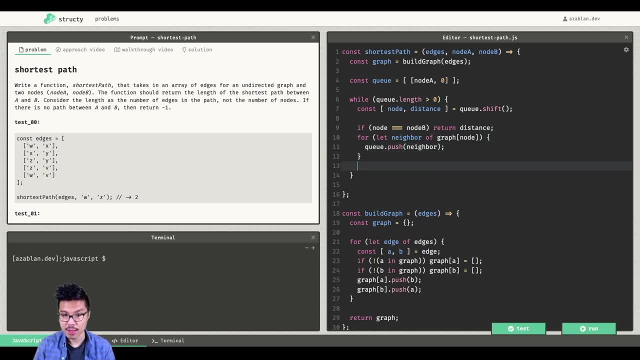 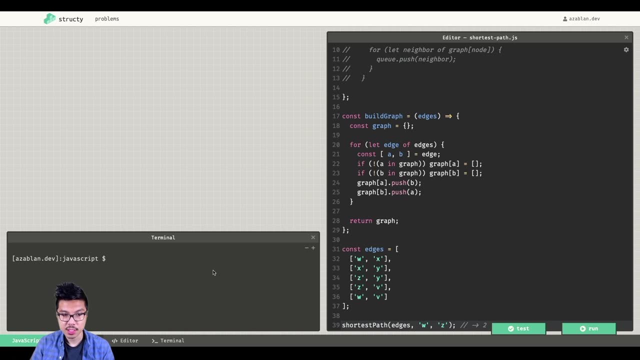 neighbor try to remember what the form of our graph is over here, Maybe as a quick little spot check. make sure, on the same page let me just console dot log the adjacency list. Let's say we took this example manually, just paste it down below And I'll just give it. 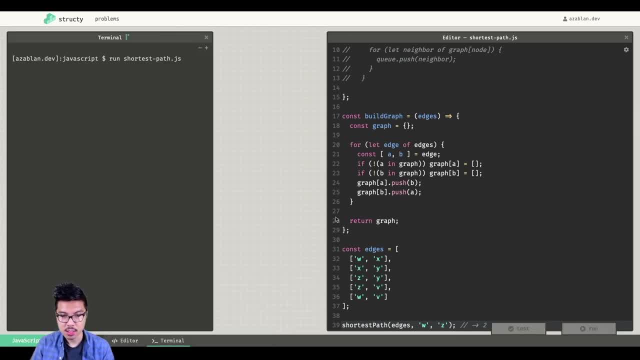 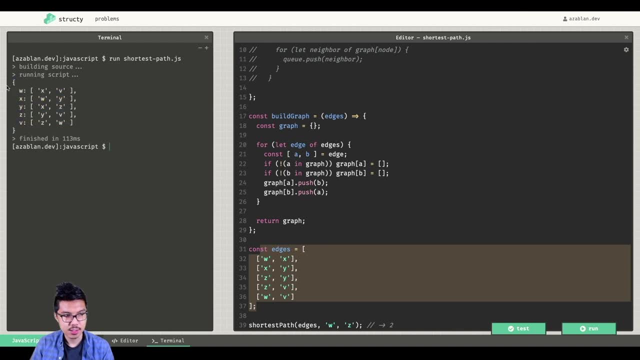 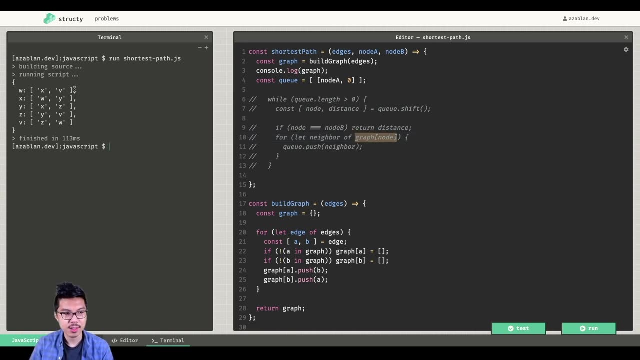 nice little manual run, So I'm not running the test cases quite yet. So we converted this edge list into this adjacency list, right? And when we say node is something like w. when we say graph, square, bracket, node, that would give us this array Cool. So just iterating through all the neighbors of this node and adding. 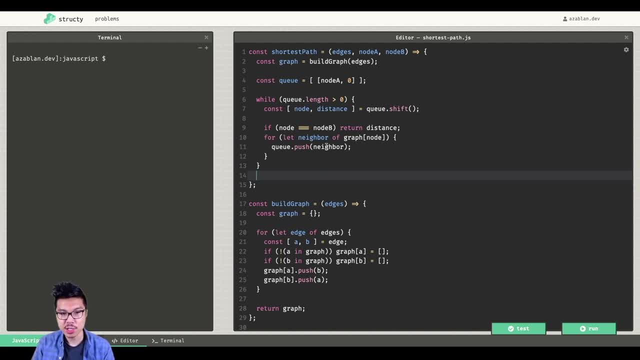 them to the queue. One thing we should watch out for is when we push things back onto the queue. we want to maintain the same format, So I actually still want to maintain pairs, So I'll make the first element of the pair the neighboring node, And the second element 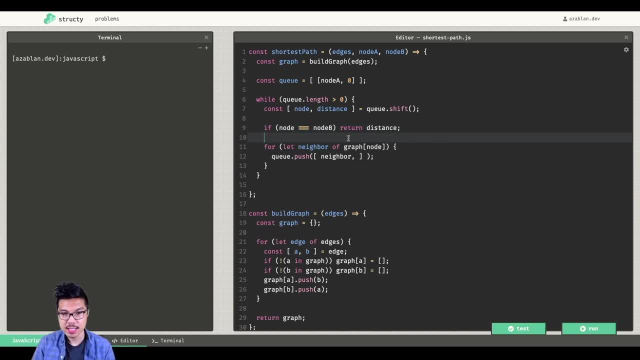 needs to be the distance, And since it's a neighbor, it's distance would be plus one over here. So that's how I'm growing and counting the distance. So let's give this a test run. There are a few things we need to work on still. 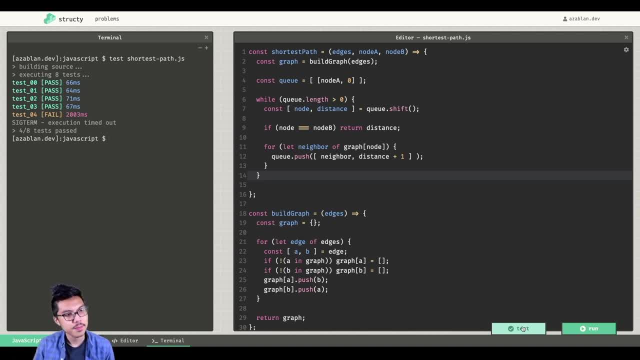 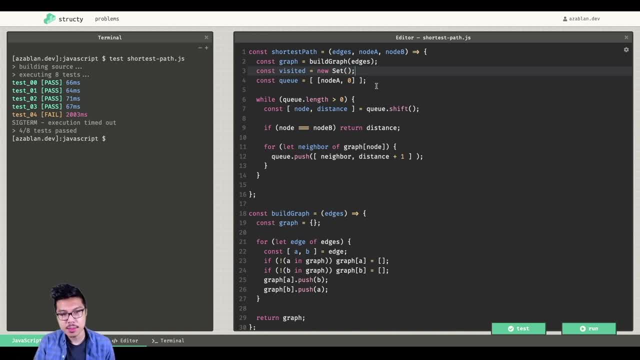 iteratively. the move would be to make sure that if something is added to the queue queue it should also be marked as visited. So if I initialize my queue with node A, then I also want to initialize my visited set with node A, just like so. So if you're unfamiliar, 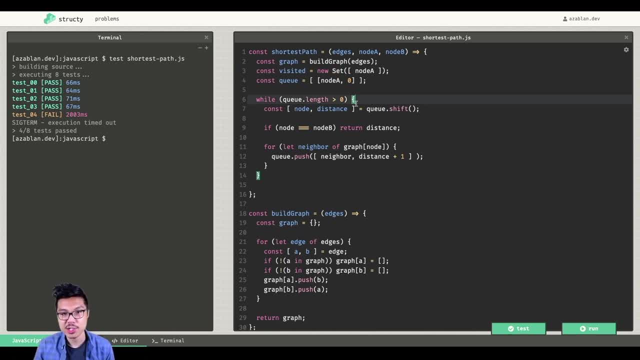 with the set constructor in JavaScript. if you want to initialize it with some values, you actually have to pass in an array containing those values. So the values of my visited set are just going to be the nodes, right, the node IDs, Cool. And then I want to work. 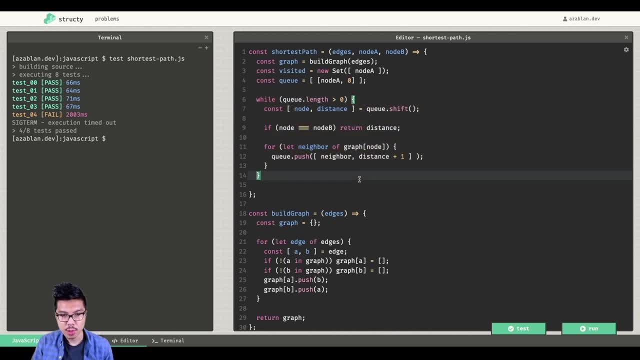 that logic into my while loop, And so whenever I'm about to add something into the queue- that is where I'm going to add a neighbor into the queue- first check if that neighbor is not visited yet. So only if not visited has neighbor Right. so only if this neighbor. 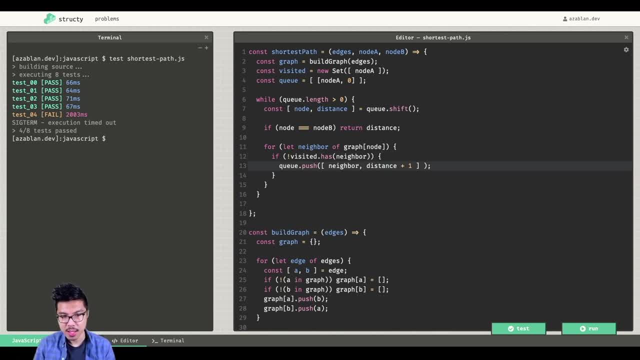 has not yet been visited, then I should add it to my queue. And if I'm about to add it to the queue, like we just said, anything that enters the queue should immediately be marked as visited. So here I'll say visited. add the neighbor. that should avoid adding any particular node. 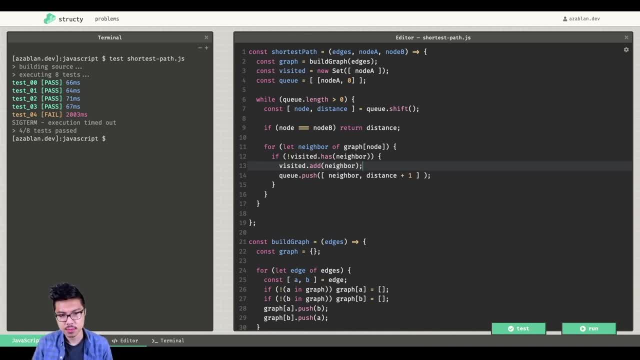 more than once into the queue, avoiding any cycles- Awesome, So that feels pretty good. Let's give that a test run now, So we hope to not time out at least On that same example. we're actually returning undefined where we expect negative one. So if you look at the 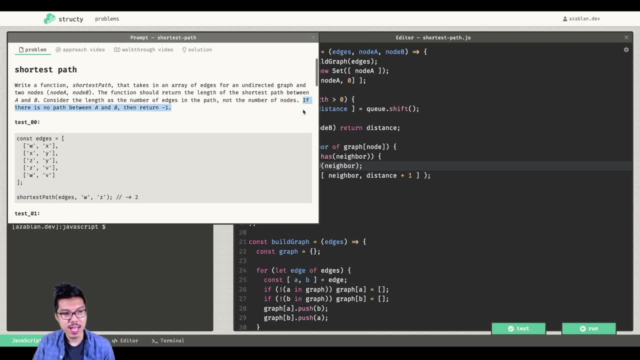 actual prompt. they tell us that all right, if you can't find a path between A and B, then you should return negative one. So if you look at example or test 04, and you kind of drew it out, you would see that there would be no such path. that connects B to G. The reason: 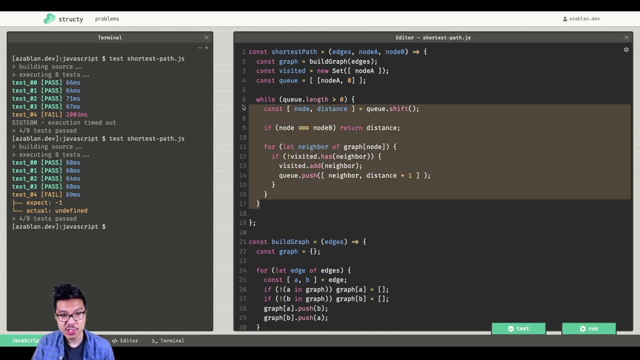 we're returning undefined right now is we're going to finish our traversal, mean meaning our queue is going to empty out, And then we're just going to hit the end of this function. And if I don't hit a return line by default in JavaScript, I'm going to get undefined. 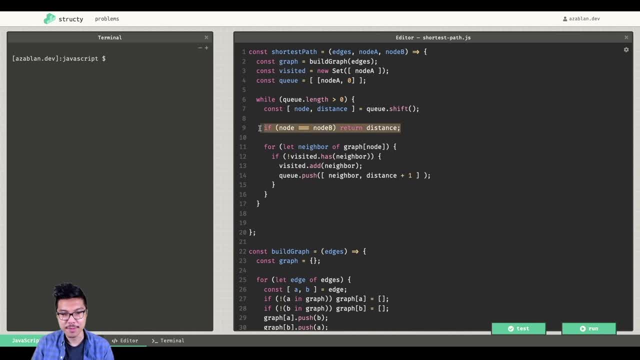 So we know, if we finish the while loop and we never found node B, Then we can just return negative one. that must mean that there is no such path that connects A to B. So let's give this a test run now, And this should be our final version. 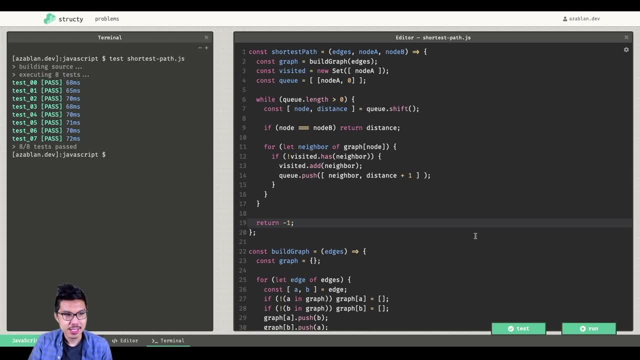 of our shortest path algorithm Awesome. So be sure to practice this algorithm before you move on And do make sure why you understand the choice of breadth first here, over depth first for most of your basic just graph problems that require you to calculate a shortest path. 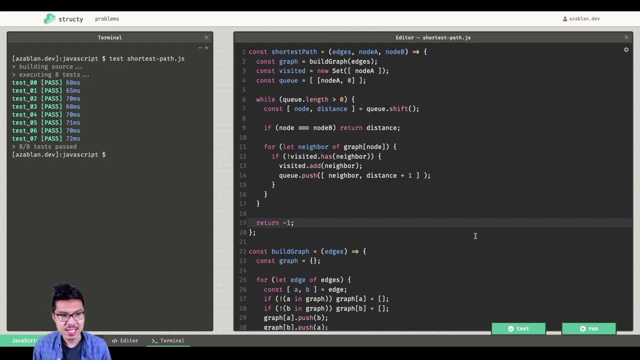 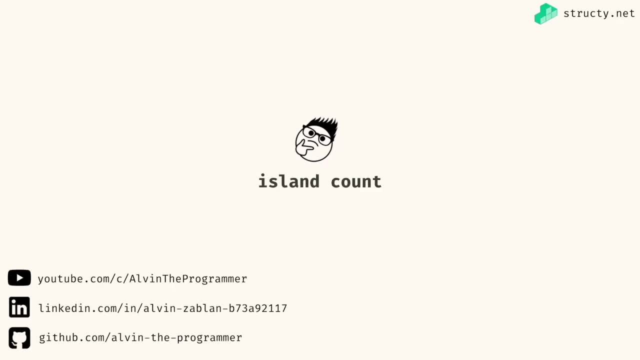 path, meaning just the number of edges. Typically you'll find breadth first, the easiest way to calculate that. Hey programmers, Alvin, here, right now let's go over to the approach for this island count problem. So in this problem we're going to be given a 2d array. 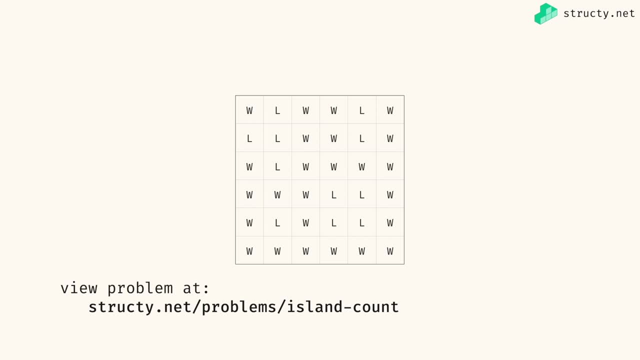 representing a grid of land and water. So here we have L characters representing land and W characters representing water. Let's try to visualize this In this problem. what we want to do is return a number representing the number of islands on the grid. we're going. 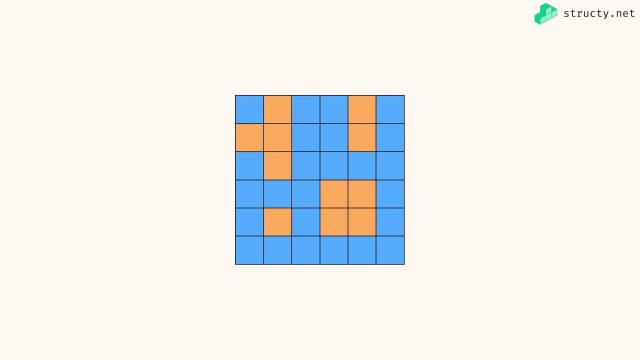 to consider an island as a vertical or horizontal connected region of land. So in this particular example, we should return four, because there are four different islands, we can label them as such. this is going to be a new type of problem for us And we should. 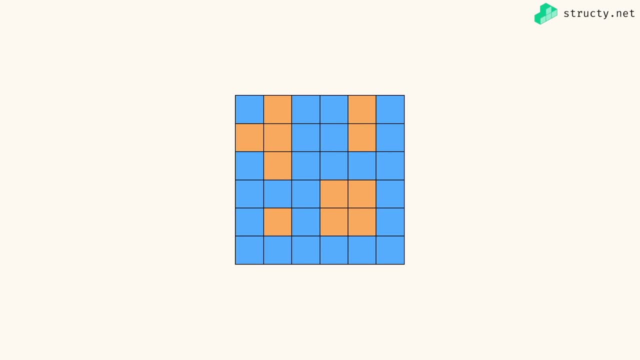 really think about it as if we have a graph- I'm going to refer to these style problems as a grid graph- And so, although we're not given any explicit like nodes and edges, I can still think about positions of this graph as nodes. So, for example, let's consider the 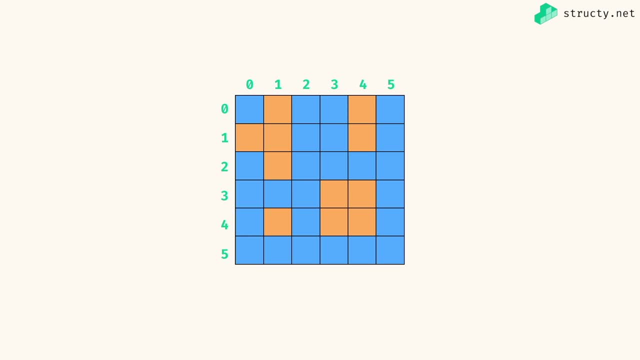 indices here. So I have my row indices along the left hand side and my column indices along the top. Now I can designate any position Of this grid using a pair of row and column. So, for example, if I looked at position three, 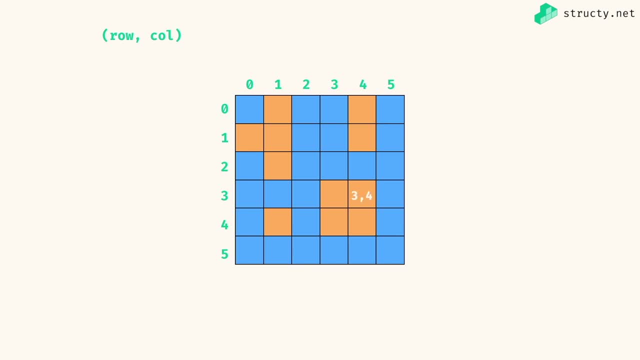 comma four. that would be this position over here, And what I should do is mentally think about a position as if it's a node. And if I'm at some node I do have some potential neighbors, Given any position of the script. I have at most four neighbors in the up down. 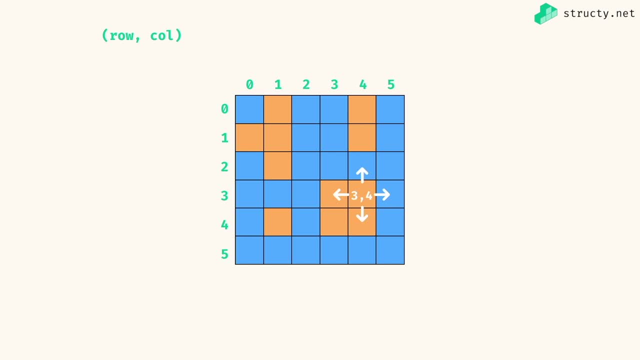 left and right directions. Given any position of the grid, it's really easy to determine what our potential neighbors are. It's really just a matter of adding or subtracting one from either the row or the column. Let's generalize this formula. So let's say I was at some position. we'll call it RC If I wanted. 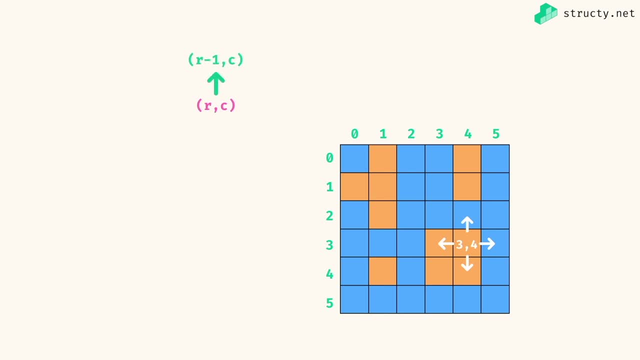 to go upward, that would mean you decrement the row by one. keep the column the same. If you went down, that would mean increasing the row by one. if you went to the right, that would be increasing the column by one. And if you want to go left, then you should. 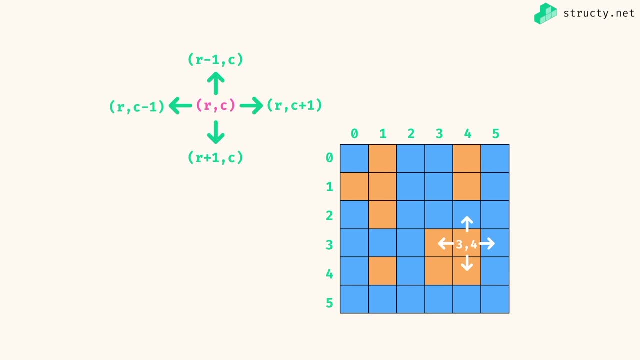 just decrease the column by one. do bear in mind that the top left position of our grid is going to be 00. And that's why we have this type of arithmetic rule. So now that we're starting to frame this grid problem as if it's a graph we can use, 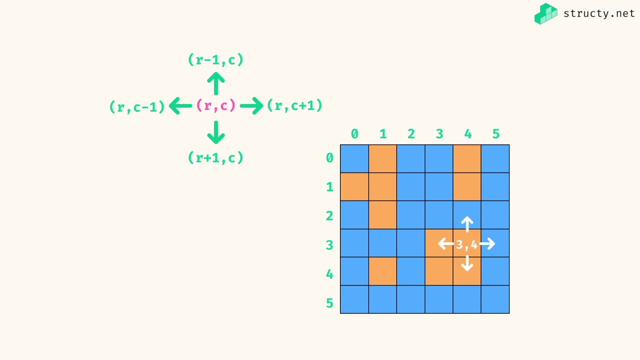 some common patterns. I know that this problem is really asked me to count the number of connected components or the number of islands on this grid, So I'm going to need some iterative code, probably some nested loops, to just iterate through every potential island and start some. 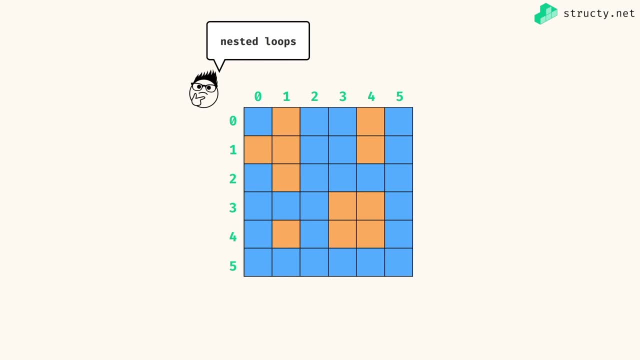 traversal at that island. So when it comes to our iterative code, we just want nested loops iterate through every row column. That means the iterations should look something like this: Just moving left to right And tell me finish, So in which case we can go to the next row. But let's actually iron out the main logic. 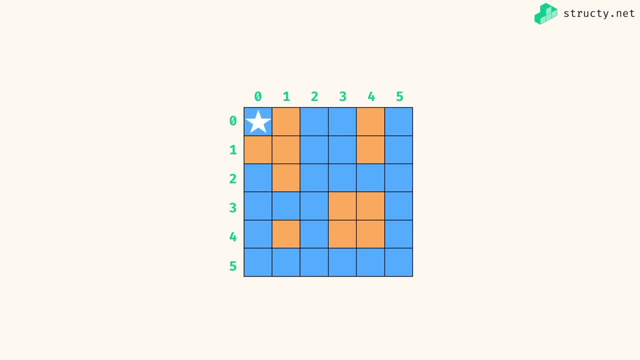 that we need in our algorithm. So let's say, we start our nested loops from the very beginning. what I do is check my current position. what I want to do is check if my current position is land. right now it's water, so I can just continue on the next iteration. I do have 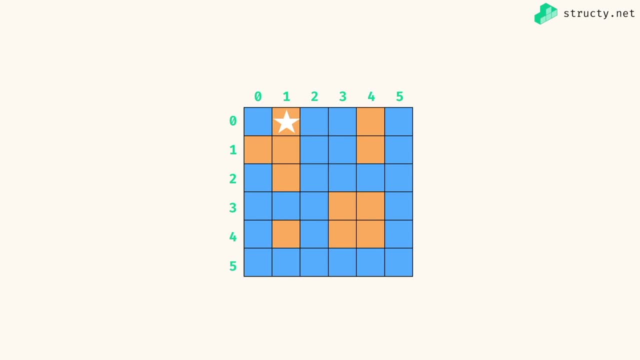 some land position And since I'm on a piece of land right now, what I want to do is explore this land region as far as possible, probably using some depth first traversal, And do bear in mind, like most of our undirected graph problems, we're not going to be able to do. 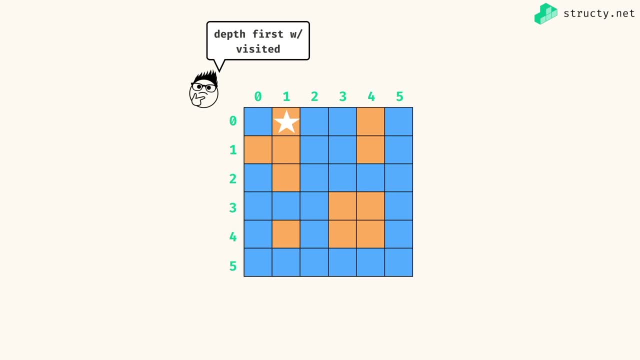 that. So what we're going to do is we're going to go to our nested loop and we're going to do our first graph problem. we're going to need to be sure to mark things as visited So we don't get trapped in any infinite cycles. So, for example, if I start a traversal at 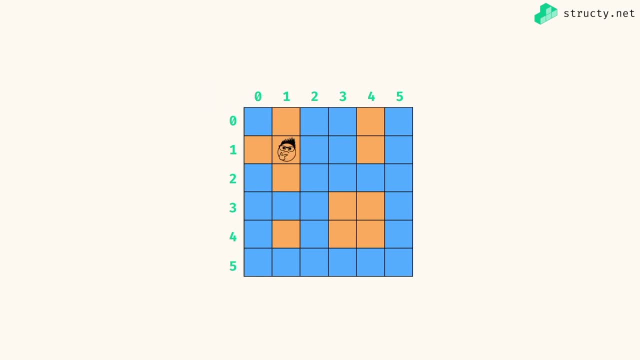 this position. I can go downward, but I can also go upward from here And I can bounce back between the two going up and down, giving me an infinite cycle. So we know how to fix this using all of our graph mechanics. right, just use a visited set. So if I do a depth, 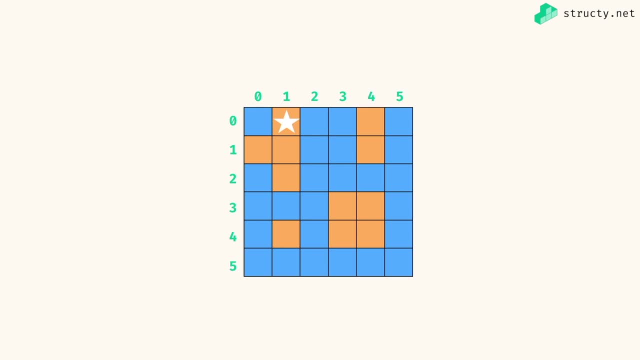 first traversal, starting at this position, I know I'm going to mark off all of these land pieces as visited, And what I also want to do is make sure that I increment accounts representing the fact that I've just explored some new island fully. So right now my count zero, since I just finished exploring something. 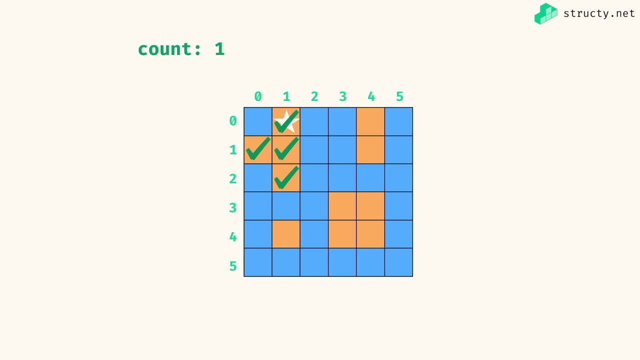 now my count is one, And at this point I can fall back to my iterative code to scan for another island. So I move to the right. it's water, So continue, water, continue. Now I have another island And again I just do some depth first traversal through it And 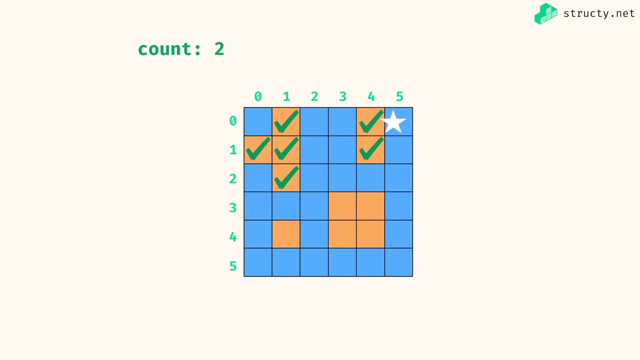 of course I increment my count. This pattern will follow right. eventually, when I hit the new row, I could be at a land position, But I should also make sure that this land position is unexplored, right. So, since I'm at position 1 comma zero and this land has, 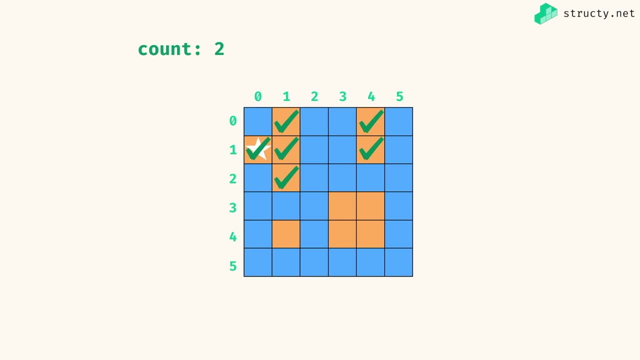 already been explored. I don't need to begin a depth first reversal, And I also don't need to begin a traversal here. This continues avoiding starting a traversal wherever I have a visited piece of land. We know eventually we're going to hit a new island like this: one where I have a piece of land that is unvisited, Because in this case, this is a hidden piece of land, But what we have to do is we have to hit this data. this is just a random piece of land, And what I did here is I'm going to hit this data, And if I hit this, 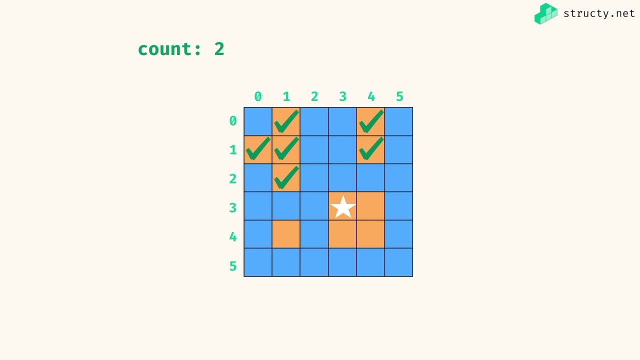 So at that point- that's my criteria for starting a new depth first reversal- I explore this region, increment my counts and continue business as usual until I hit this final island that is unvisited. So I visit it and increment my counts And by the end of my iterations, 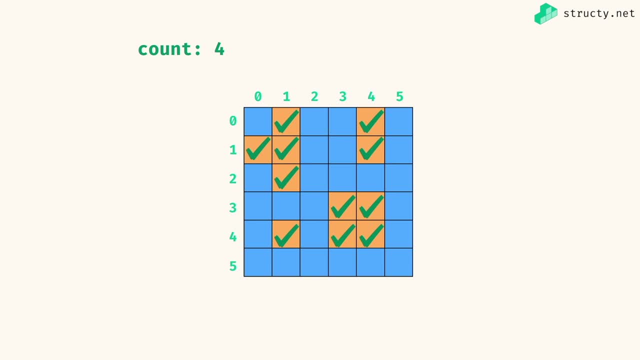 I should have my final count of four. So that logic is actually pretty straightforward. just a variation of our classic connected component counting logic, except now we're adjusting the criteria we use for looking at neighbors. right, our neighbors are actually going to just be either above, downward to the left or to the right of our current position. 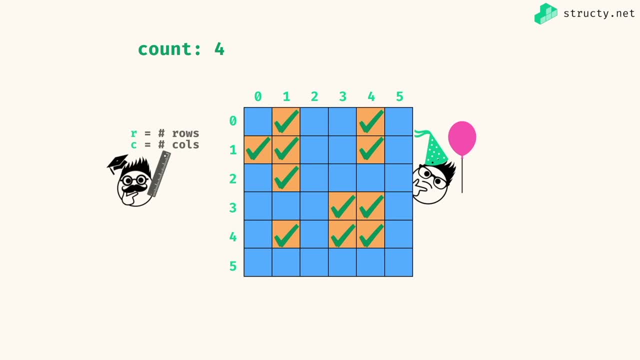 we talked about the complexity of this algorithm. we should consider the size of the input and the fact that it has two dimensions, right? So if I say that R is a number of rows and C is a number of columns will land, the iterative code is pretty straightforward. I know that's. 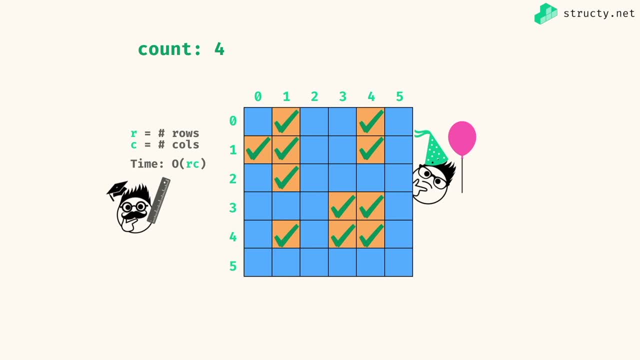 going to give me our time C iterations. And if I also consider any potential, indeed depth, first reversal I do, starting at some land, in the worst case I could have one giant island, which is also going to be our time C. So the overall complexity is just. 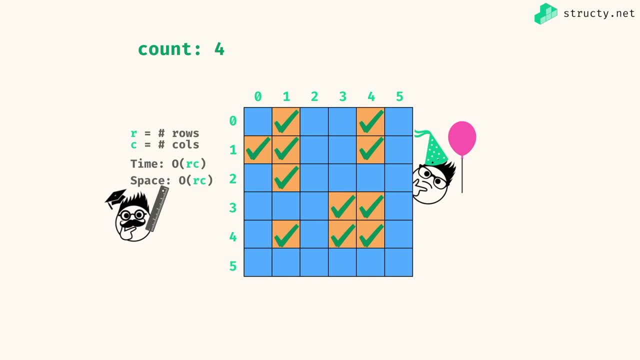 going to be our time C. the space complexity, for very similar reason, is our time C, because imagine that we mark all of these positions as visited. that probably means we'd have to add them to some set right. so I have our time C: different positions, And by the 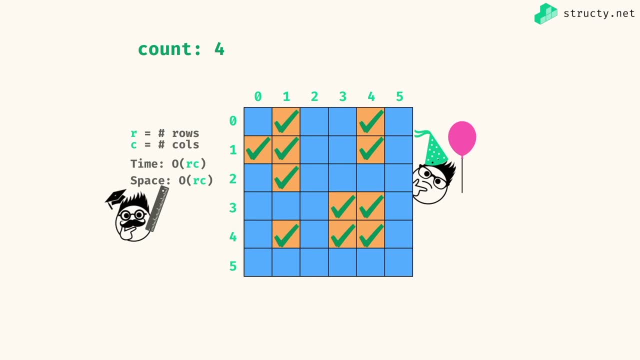 end, I could add each and every one of them into my set. this space complexity of our time C also includes any traversal A related data structures like stacks or queues, depending on how you implement this one. So, overall, this is going to be a very efficient solution to solve this one. what you should. 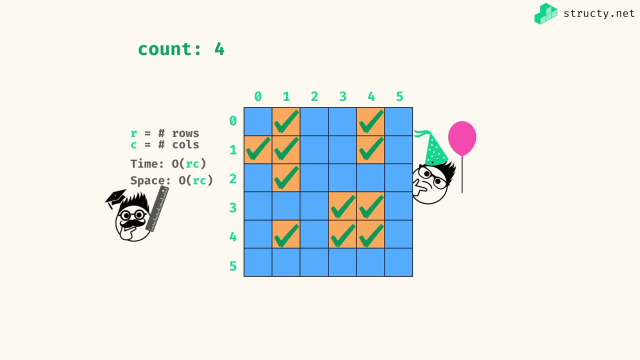 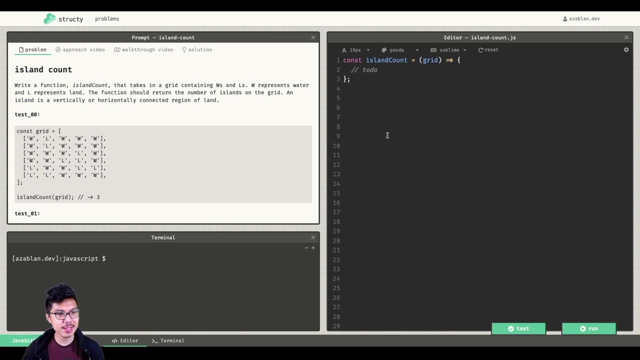 do is probably give it a shot on your own first. if you get stuck, you can find me in the walkthrough videos. I'll see you there. Hey, programmers, Alvin, here Right now. let's go over a JavaScript walkthrough for this. 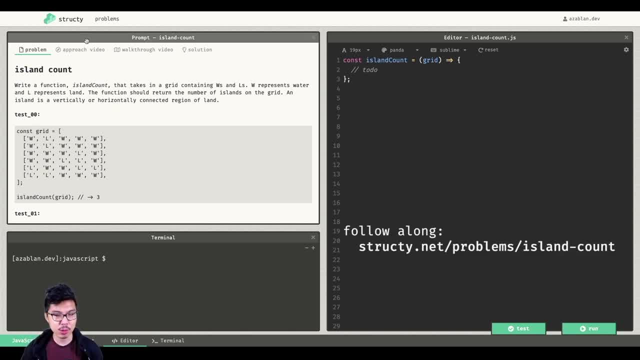 island count problem. So, as always, make sure you watch the approach video first And we'll jump right in. So we know that this is really just a spinoff of our kind of graph connected components problems, Except now we have a grid graph right, And I can still think about like this grid as 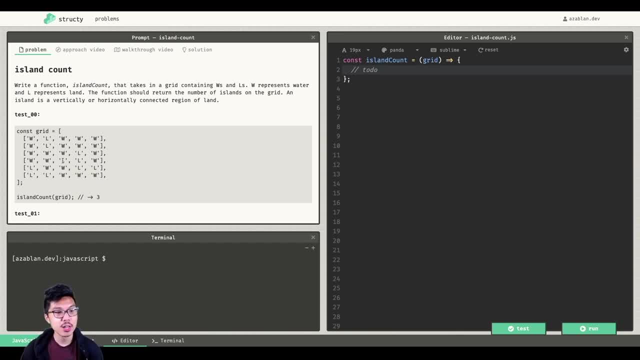 if it's a graph, Because if I think about any particular position of this grid, I know I have some neighboring positions that I can travel through, mainly my four neighbors up down left and right for me. Let me start by laying down some iterative code that can begin. 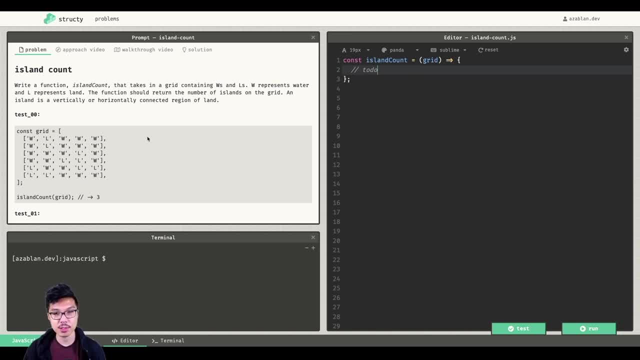 a traversal at every node or every position of this grid. That way I can start considering different islands, right? So I'm going to use just a for loop for this. I'm going to iterate through every possible row, column combination, So every position. so I'll say, like r equals zero, iterate up. 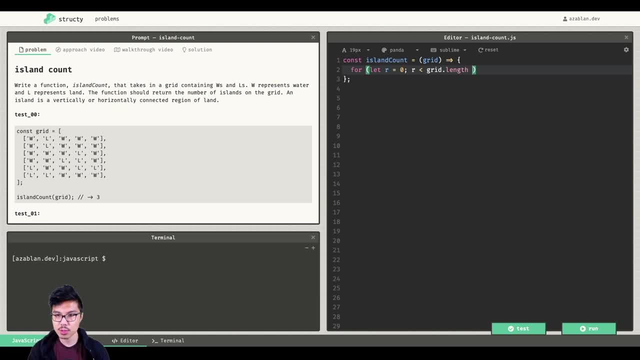 to the length of the grid. So grid dot length to are plus equals one, and do something very similar for my columns nested inside right. Watch out for some details here, though. looking at the examples we can't actually assume that we're always get a square shaped grid. 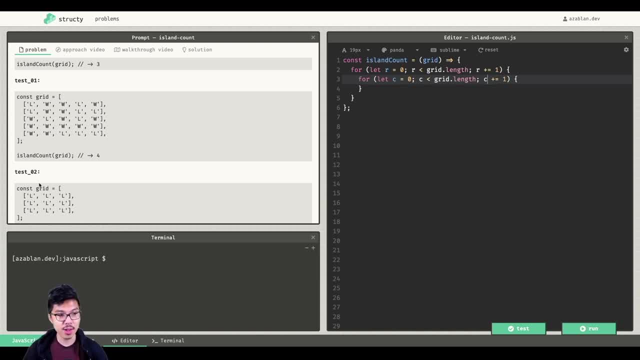 square, meaning like as if the number of rows was the same as the number of columns, because sometimes they'll have like an asymmetric And let's take and say, okay, here's a grid. let's say, I want the melt, And then, if I do, 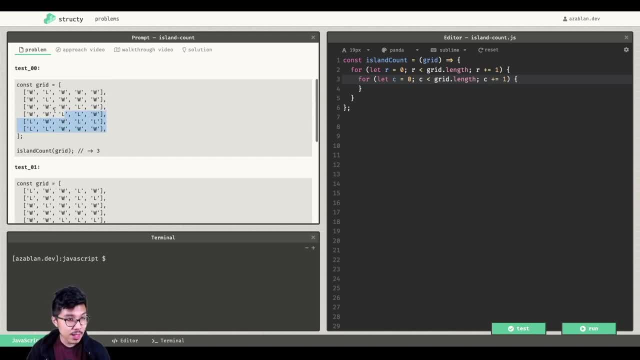 a grid occasionally right. If I look at this very first one, it looks like the width is going to be five here, but the height is six. So separately for the columns I want to reference the column length over here, So I can say: grid zero length, Nice. And so at this point 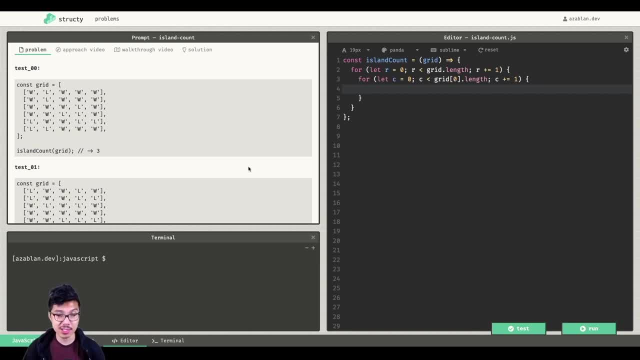 I have some row column position. I want to begin a traversal, let's say a depth first traversal, at that position. So here's where I invoke some like helper function that will make a little bit. I'll call it explore And what's going to do is, of course, taking 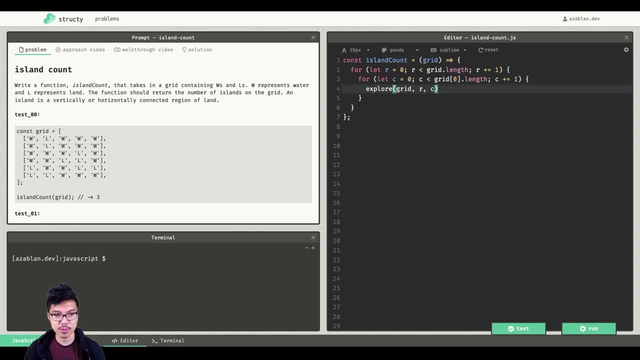 the grid information as well as the row column. I want to traverse through Nice And at this point I think we'll actually hop to building this, this helper function. then we probably need to fill out some more logic within our main driver function here, So let's bake this. 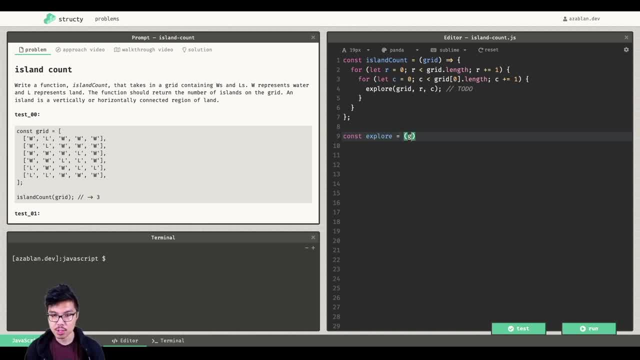 explore helper function. So taking the grid and your row column. and something I should all also consider is because I know that this is really a type of graph problem, right, I want to prevent infinite cycles, right? So consider this. let's say I was somewhere in. 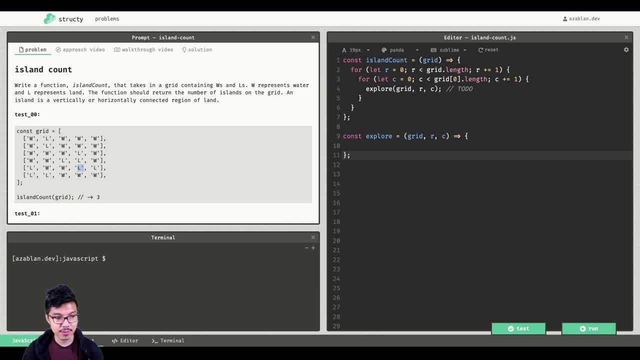 the middle of my traversal, Let's say I was at this piece of land. I know that this piece of land is going to travel through its right neighbor And it could be the case that this piece of land now travels to its left neighbor. So I go left and then right and then left. 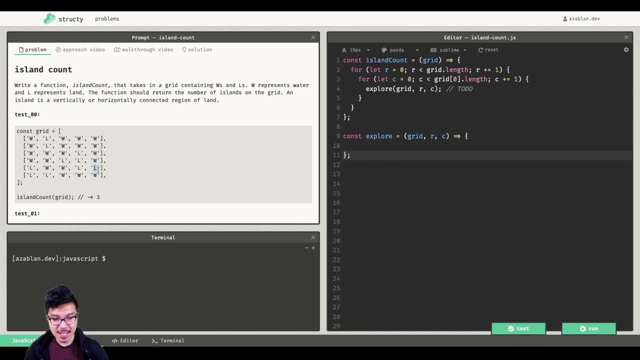 and then right, that would give me an infinite loop, right? So whenever you have this notion of like undirected graph or undirected connections, then always guard With a visited set. we've seen this pattern before, So maybe up top globally for the. 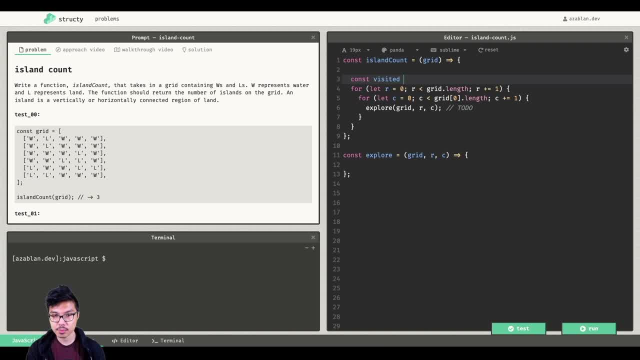 entire traversal. I'll create a visited set. So, in JavaScript, just a new set. you're probably wondering. you know what am I going to make the, the members of the set? Well, I need to designate positions. right, Think about it as if positions are like the nodes in this. 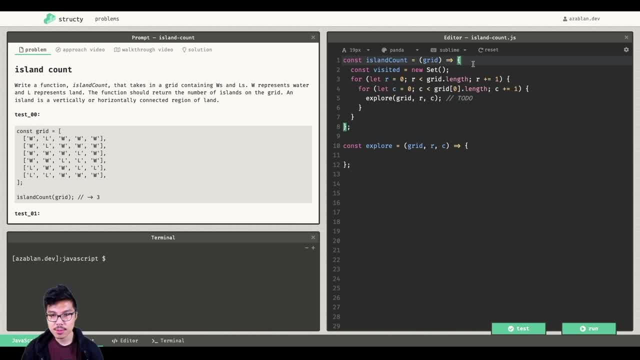 grid in this graph right, And so what I'll do is pass along this visit set so I can accept it as an org over here. And when it comes to using your visited set, what you want to do is make sure you combine your row and column, because together they designate your actual position, And I 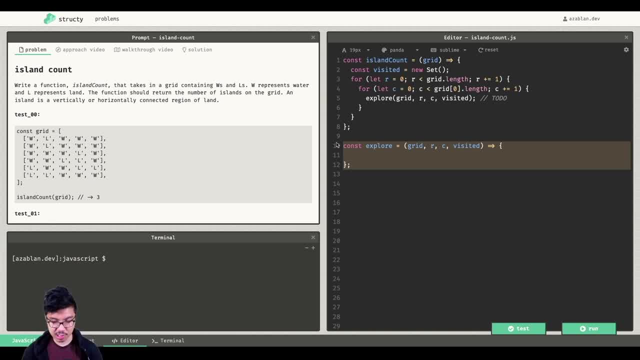 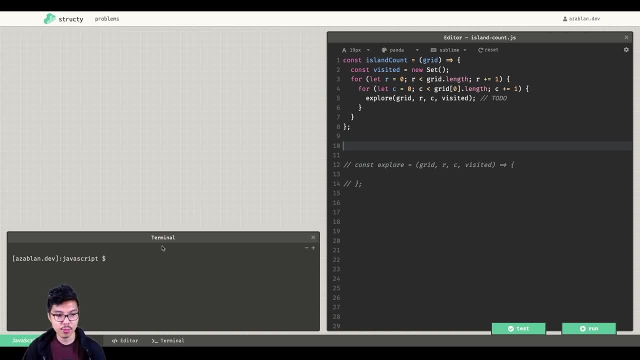 think this is actually worth going through, specifically more of like a language thing in JavaScript compared to other programming languages. So quick aside over here, let me give myself some more room. might be a while, Because if you're unfamiliar with sets and you don't kind of know their nuances, 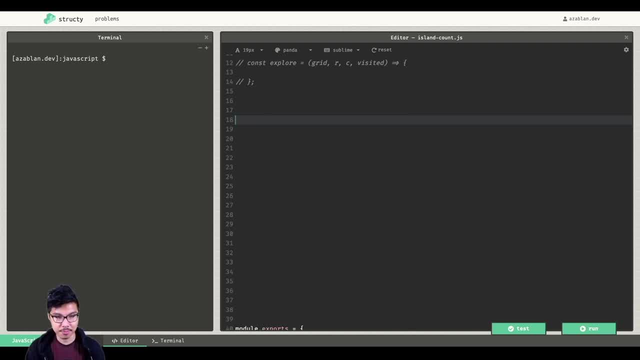 you might actually hit you in the butt later on. So let's say I had a set, So I'll create an offset s can you set? And let's say I added I don't know, like an array containing a row, column, position. So I'm going to say: is alright, maybe I had position, I don't know- one comma. 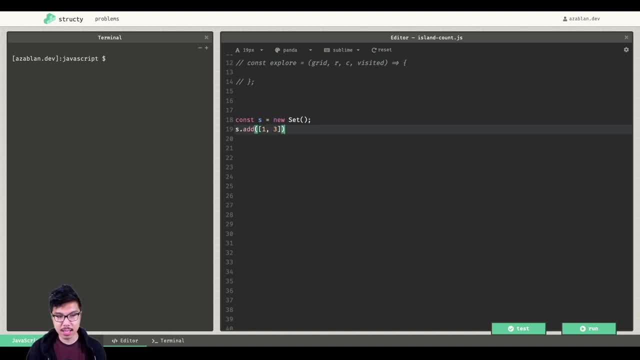 three and I added that into my set, So I do s dot add that position. This is actually a common gotcha in JavaScript. If you put any like reference type, so like an array or like an object, into your set, it's actually going to check for reference equality when you check for. 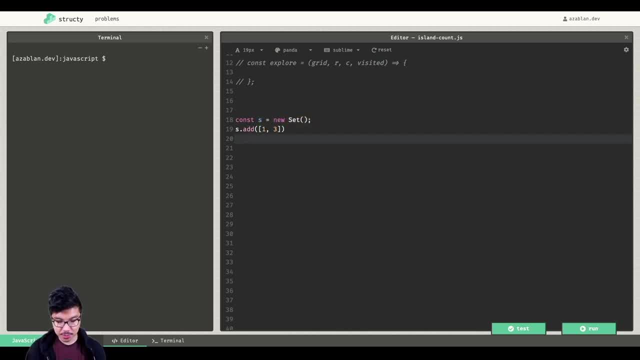 existence later on. In other words, now I can't really do console dot log s dot has 13.. Because this array literal is technically a different array in memory. So I wish I could get like true back in this scenario. but I'm not going to get a true, So we'll just run. 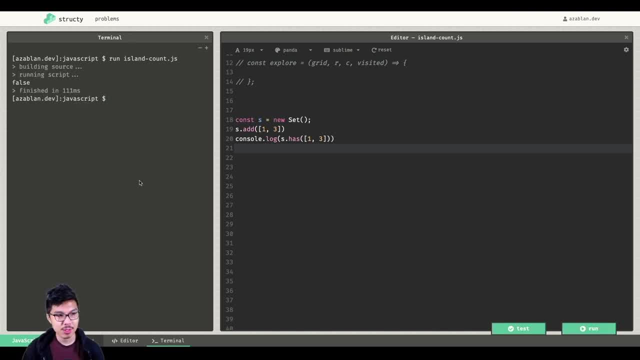 that manually. See what we get. So, like we say, we're going to get a false here, which is not so good. So instead your fix would be to actually convert this into some string data. So instead maybe write as if you had one comma three, because strings are primitive types. 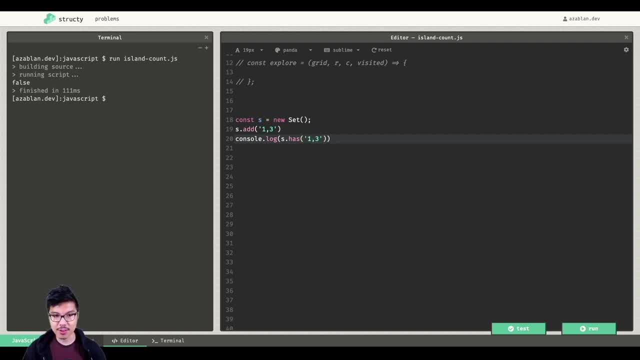 and I would actually be able to store that string. So whenever I say the string literal, this would actually give me a match now, So I should get a nice true here, Awesome. So we'll want to use that pattern to our advantage, And so maybe I'll start by creating some position. 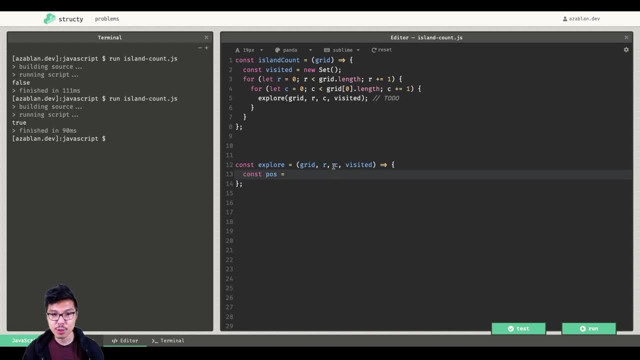 variable. that's going to be like the stringified version of our position. So just take my row, maybe, add a comma And then also put the column here. Nice. And the reason I want to comma separate is I need to have different bounds for my row and column. In other words, imagine I had 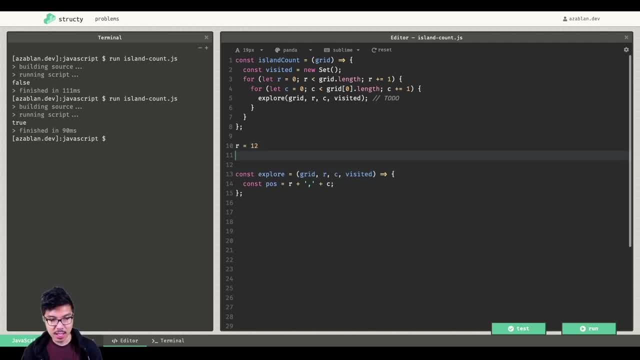 row of, let's say, 12. And I had a column of four. If I turn that into a key or position, that would give me position As it looks like 12 comma. for another scenario, let's say I had row one and then column 24.. 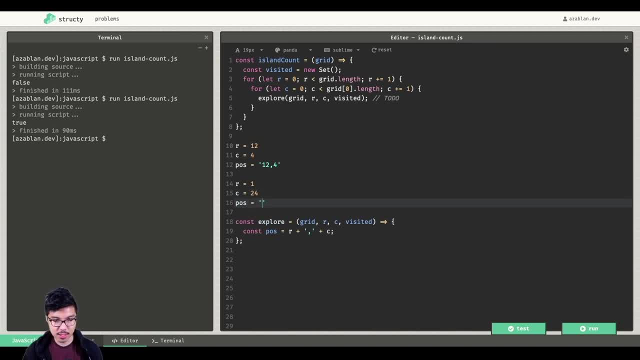 That would give me a position of this. right one comma 24.. Right, it's really important that you put a comma to separate your row and column positions because imagine I didn't put the comma, then it would have a collision. here I have two totally distinct positions: right 12, four. 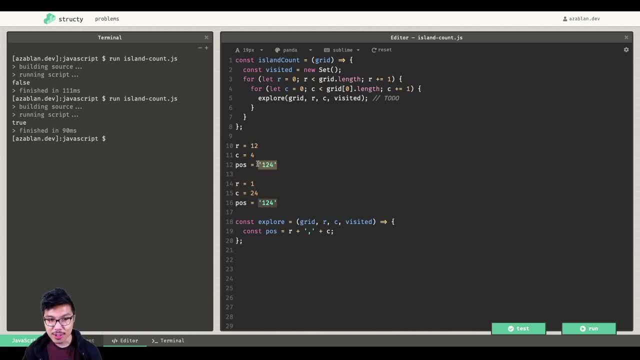 and 124.. If I don't put a comma, they look like they don't have a comma. they look like they don't have a position key. So that's why I need to comma separate them. Common gotcha there. But now 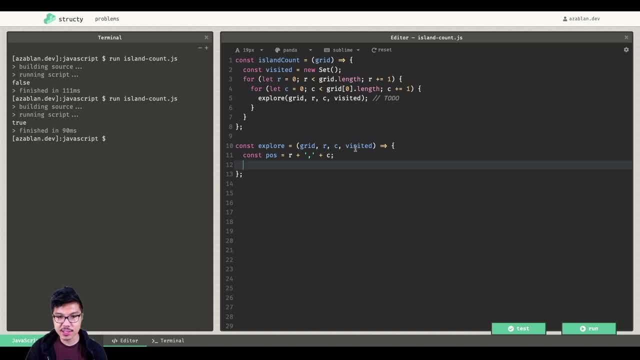 that I have this position. I can use it to my advantage in this visited set. So if I've already visited this position, so if my visited has this position, then I should exit right. I need to return something And I want this explore function to do something similar like. 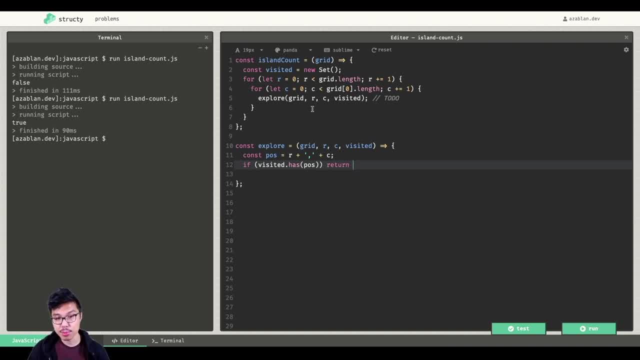 we've done in our old component problems. I wanted to return a Boolean indicating whether or not this island that I'm exploring. So if it's visited already, that's definitely not new, right? So just return false meaning. it's not a new island If I make it passes if statement. 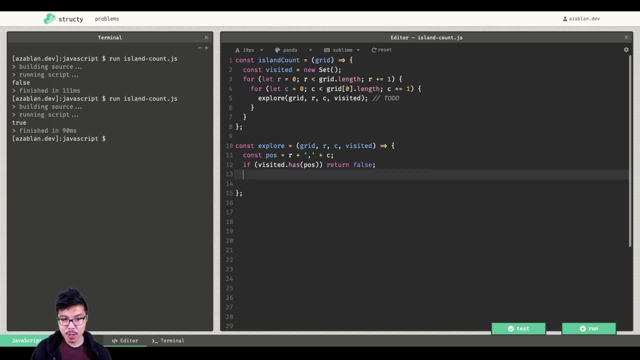 in other words, if position is not in visited, then I need to mark it as visited right now So I can do visited dot add this position. So now I have my core, like cycle prevention logic. Beyond that I have a few other scenarios. we know that in our traversal we're going. 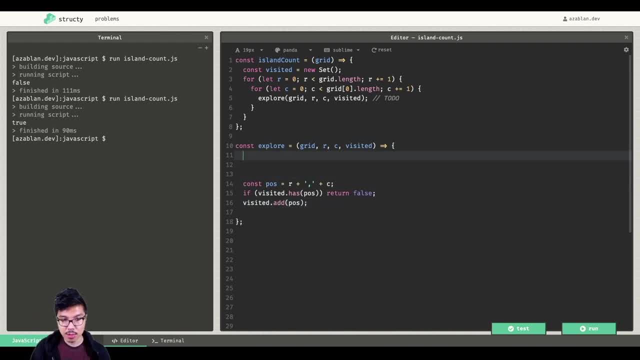 to look at our different like neighbors, And so what I want to do is make sure that I'm in bounds here. So I'm going to check. like to split this up into variables, I'll say one, a Boolean variable called row in bounds, And what I'll do is just check if zero is. 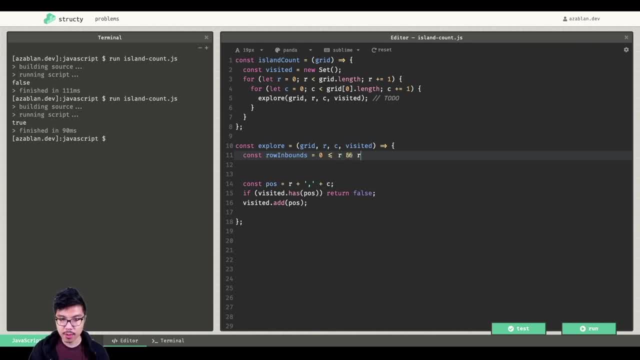 less than or equal to the row, And that row is strictly less than, we'll say, the length of my grid. So I'm just checking to see if my position is in bounds here. If I do a quick check, I need to be inclusive with zero, because zero is a totally valid index, right? 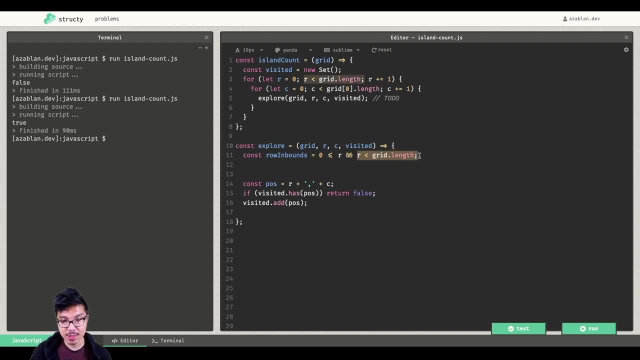 I need to be exclusive with the length, because imagine I had a grid with length five. its last valid index is four. So I need to be strictly less than here, And I'll write a similar variable for my column in bounds, just like this, And at this point I can write: 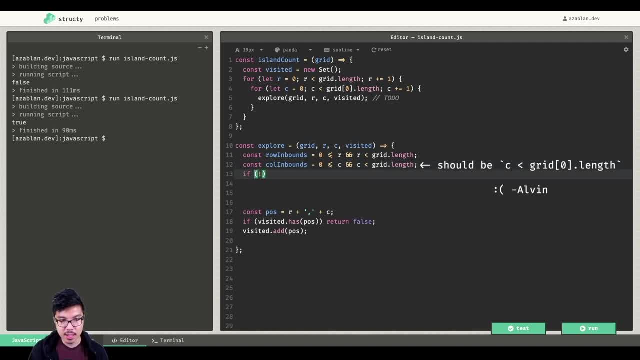 a nice semantic: if statement and check, All right, if your row is not in bounds or your column is not in bounds, then exit, right, So return like before I can return. I can return false right Because I should not consider like an invalid position and out. 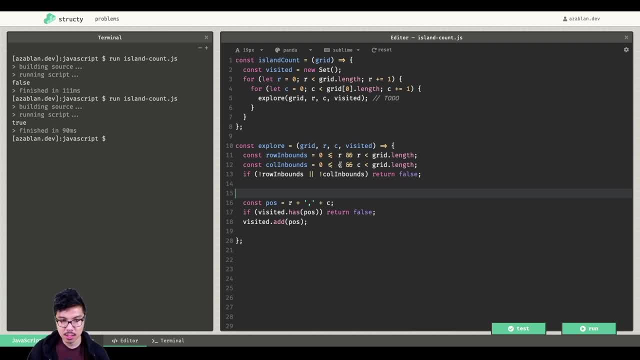 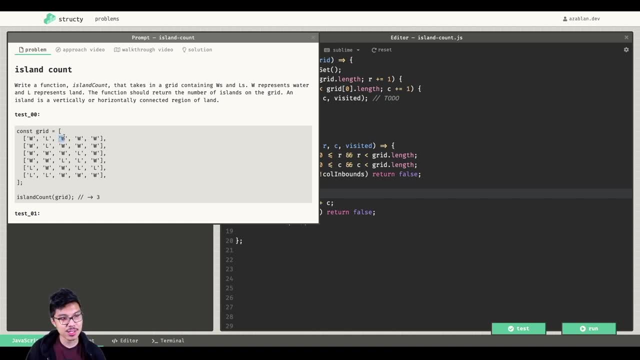 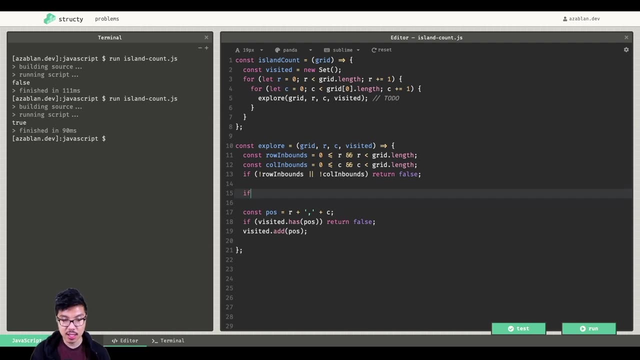 of bounds position as an island right, So that's looking good. Final base case I need, though, is what? if my current position is water right, I only want to do my traversal through land, And so I'll add another statement for that. So up here I can check, All right. 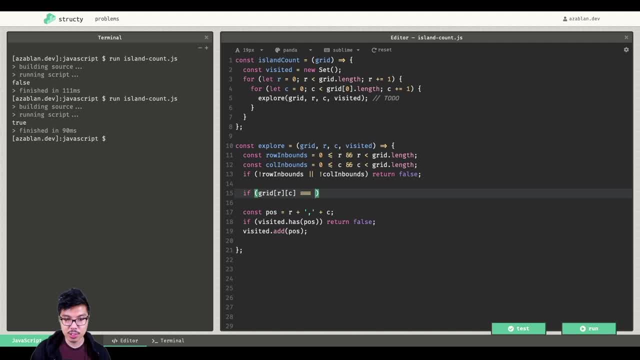 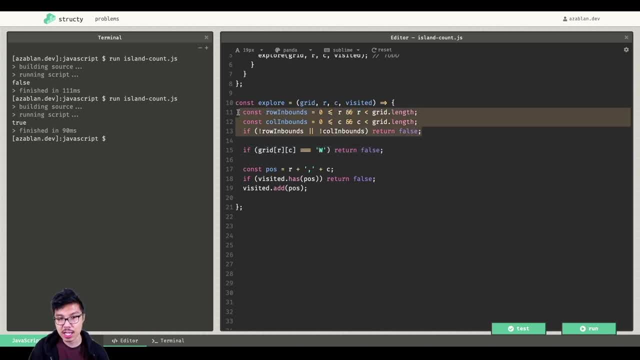 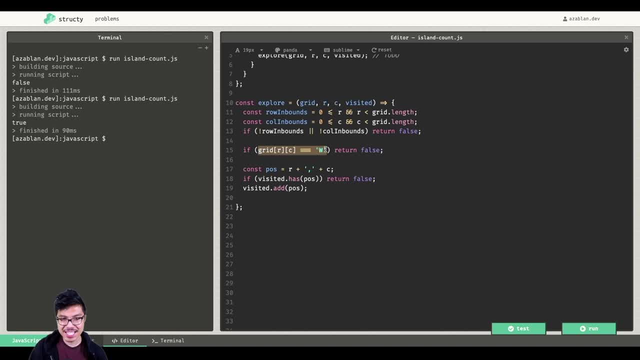 you index into your grid right, Because imagine that your row and column were out of bounds. If you write line 15, like this, immediately you're going to get an out of bounds error. So start with your guard to check if you're in bounds, If you want it to, because most 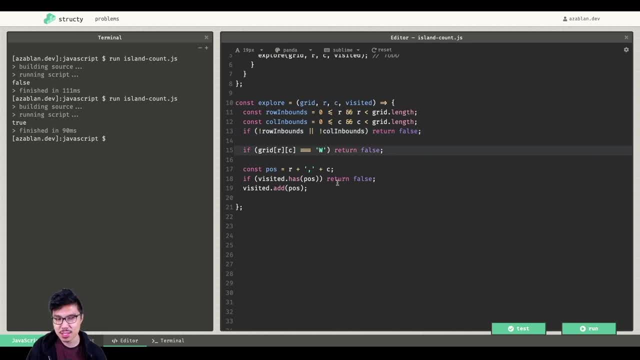 of these conditionals. they all return false, have the same consequence. you can probably or them together. Typically I like to keep them separate. that way I always remember to write them, typically for your- like your- grid graph problems problems. this is very canonical code, Alright, so if I make it past all of these base cases, 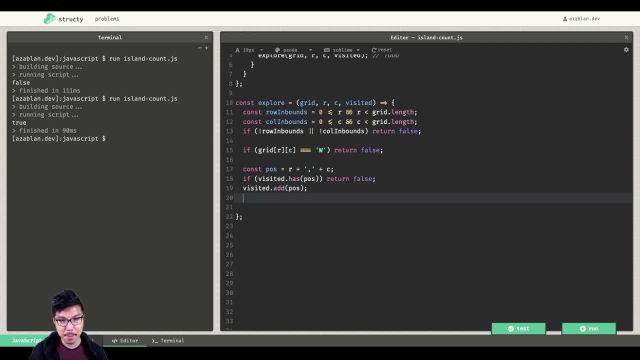 and I have the recursive case. so I must be at an unvisited piece of land And what I want to do is do my depth first traversal right. So here's where I explore my neighbors, and I have four neighbors. If I want to go above, then I decrement my row by one keep. 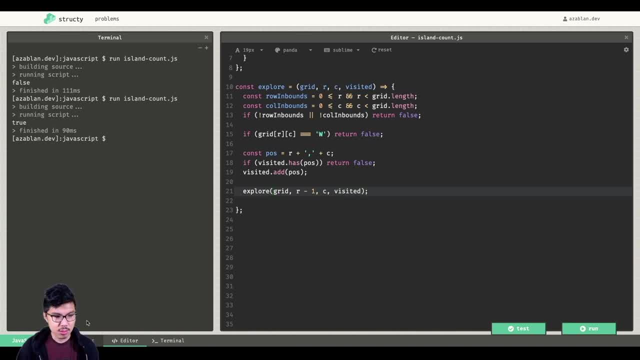 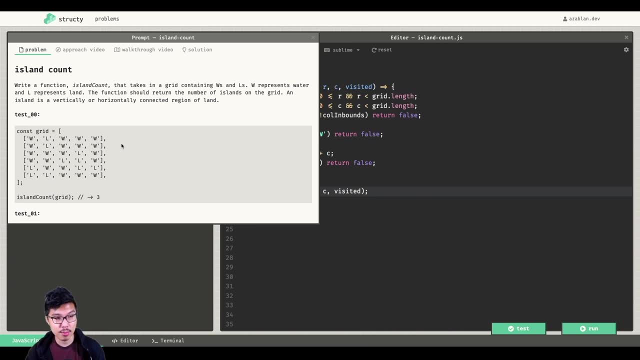 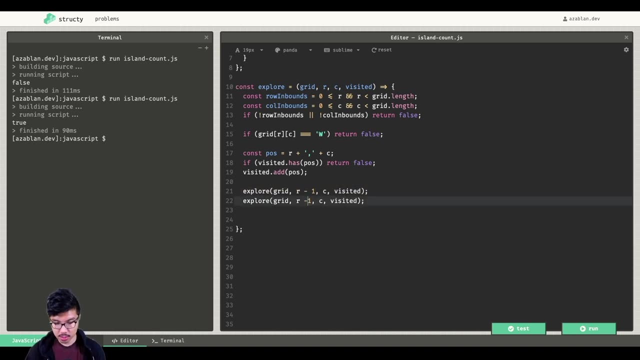 the column, the same pass along, the same visited, because, remember, we have, like, the array indices here. So this is row zero, this is row one, So lower row numbers mean upward, in the same way lower column numbers mean to the left. So this is up, This is down, If I do just. 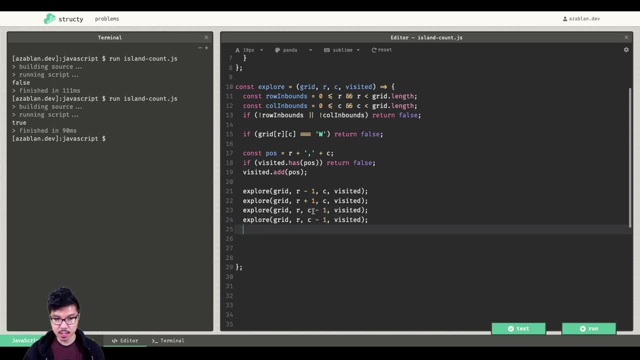 minus one over here, that would be to the left, then plus one on the column would be to the right. Cool, And I can keep this code very flat, as it is something that I'm a huge proponent of. When you write recursion, for the most part it's going to be a recursive. 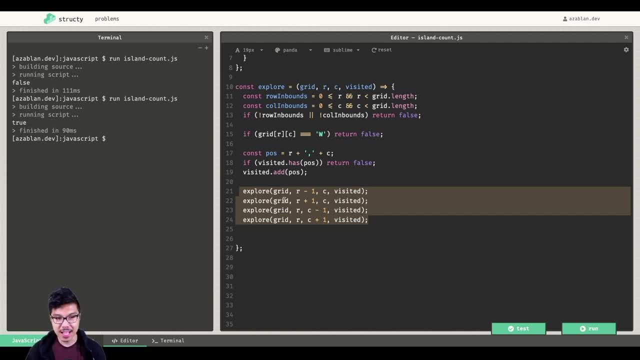 case, But for the most part I always try to make sure that I don't look before I leap. In other words, just from this logic alone, it could be the case that row minus one is out of bounds. But that's okay, Because if it's out of bounds, when I evaluate this call, 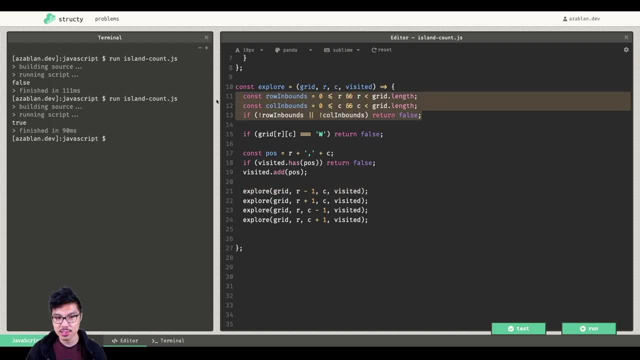 it's going to immediately be caught by this base case. Right, And if I express my logic like this, if I don't look before I leave, if I just leap and then catch myself with the base case, you don't have to write repetitive code. In other words, some people you know, 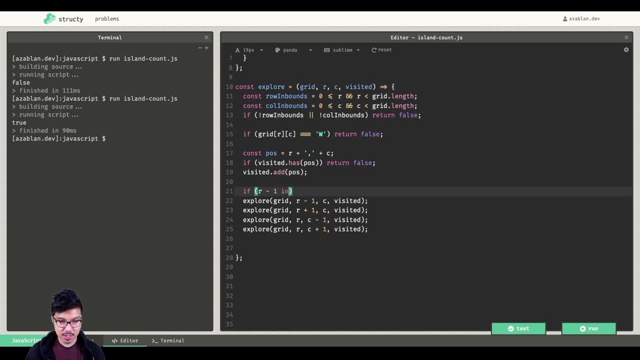 write code like this, where it's like: alright, if we're minus one in bounds, kind of using pseudocode. here they would have to write row plus one in bounds And you would have to write a guarding if statement around every recursive call. Instead, just write one base. 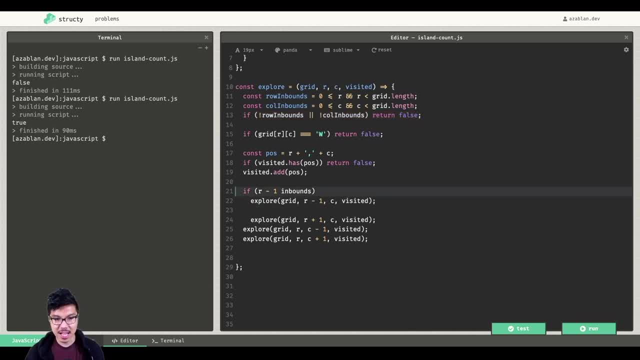 case, And you can catch all of these different out of bounds, right. So that's why I prefer it this way. And so I know that by the time I return out of these recursive calls, I'm back at this segment of my code And what I can do is return true, because I must be finished with that traversal. 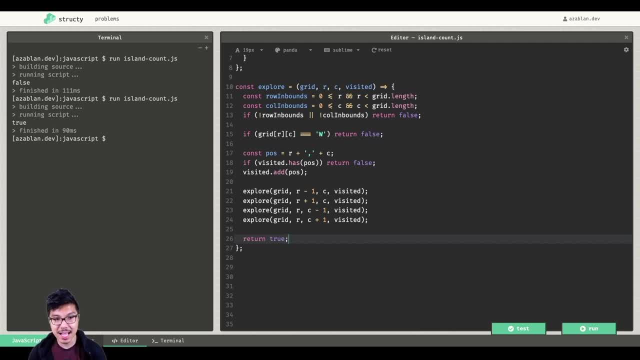 And the reason I'm returning true is true symbolizes that I've just finished exploring a brand new island, So I need to count it Nice. It's also consistent with the data type. I have Boolean for this explore function, So for the most part, this looks like really. 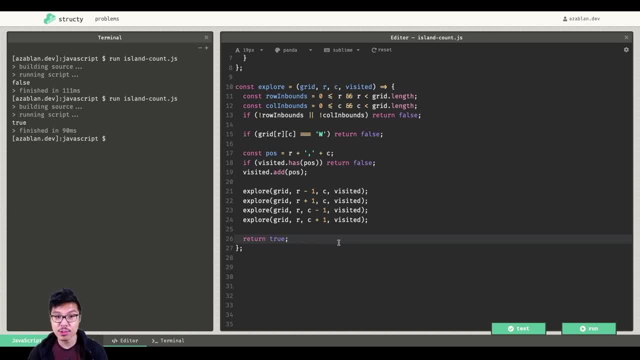 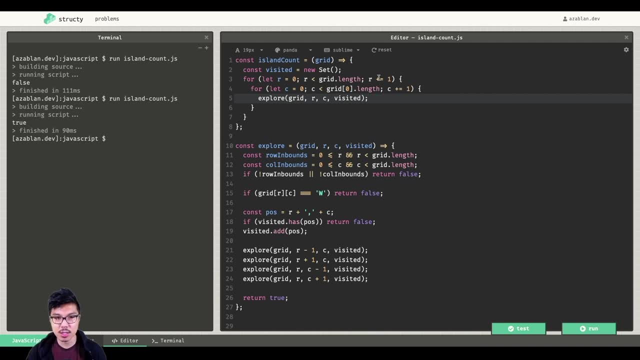 just a spin off of our previous like graph depth first code And now I want to use that Boolean data in my main function here. So here's where I can actually count my islands. So I guess I really need some logic here that says: initialize some counts equal to zero And whenever you find a new island, increment. 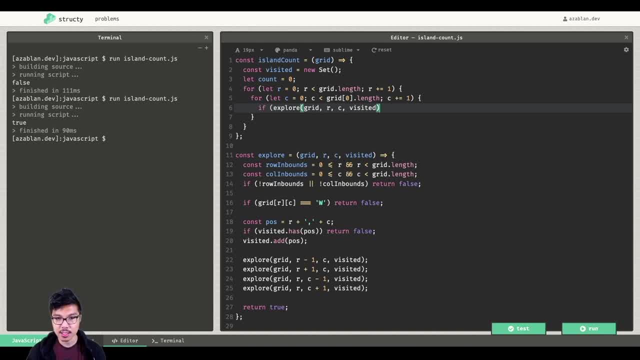 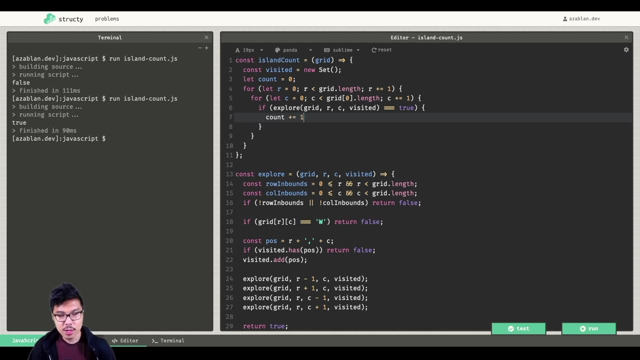 that count. So if I just have found a new island, I'm going to get back true from this. this call right, Because remember that I'm beginning a traversal starting at this row column position. So if it gives me back true, then I can totally increment my count by one. 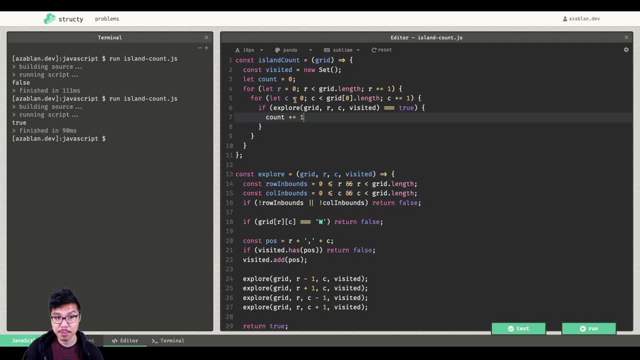 Notice that whenever I begin a traversal on a position I've seen before, it would have been added to visited before. So I would return via this if statement on line 21, I return false. If I return false then I don't double count that island. So I do need a combination of both iterative. 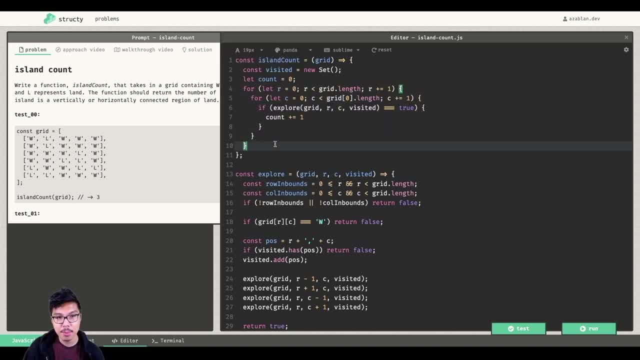 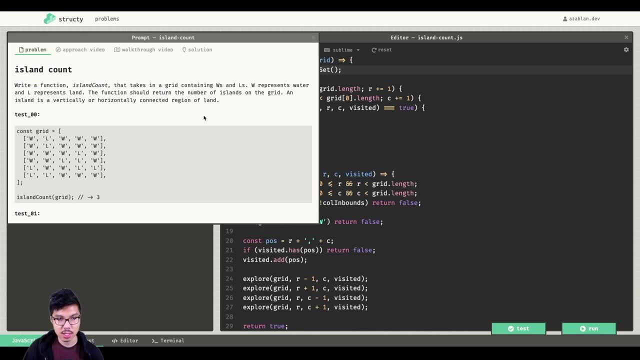 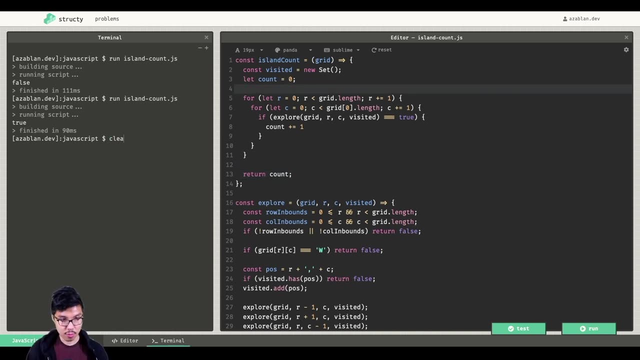 code to potentially leap to different islands, But I can use a visited set to prevent myself from double counting any particular island, So this is looking pretty good. Let's not forget to, of course, return our counts at the end. Let's give this a run. This will. 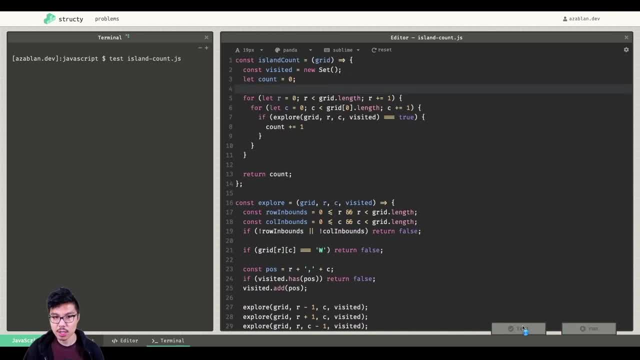 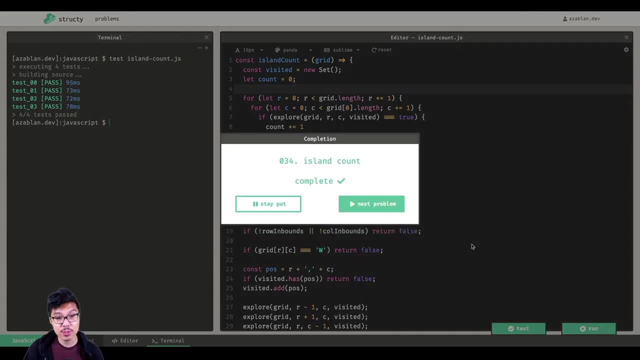 probably be the first in a series of these like grid graph problems. Really try to understand how we can think about still a grid as if it's a graph. right, We just have different rules for how we look at our neighbors. right Now, a node is really a position and its 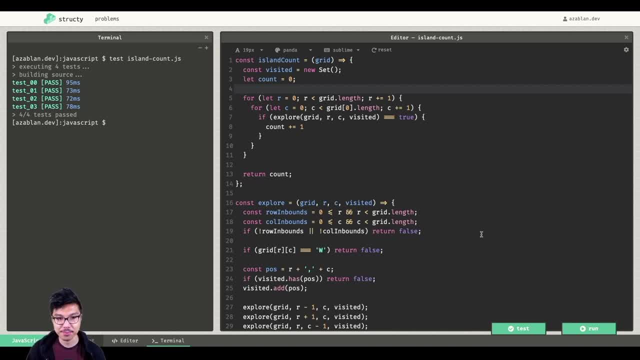 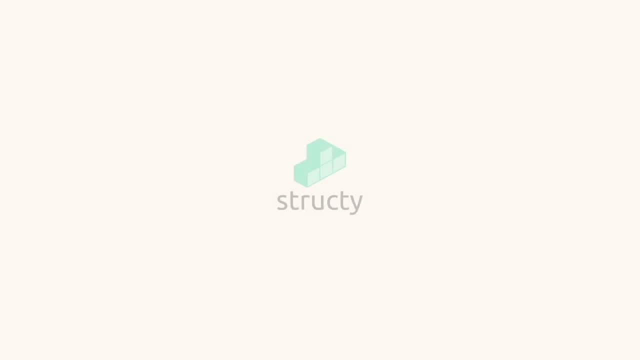 neighbors are its four neighbors up down, left and right. All right, programmers, I want you to practice this pattern because we're going to see it in the next few problems. I'll leave it to you. See you in the next one. Hey, programmers, out in here right now. 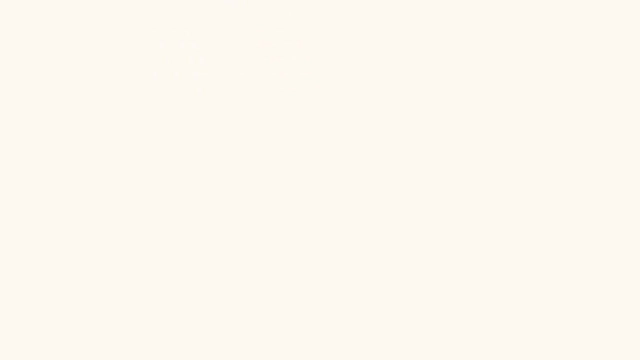 let's go over an approach for this minimum island problem. So we're going to be given here a grid containing a water and land, really just some characters inside of our grid. So, of course, as always, let's visualize this And what I want to do in this problem is return. 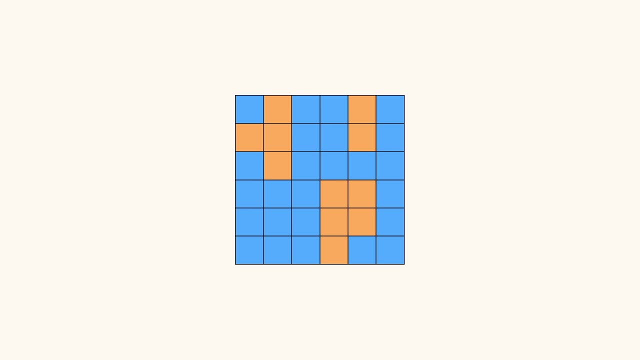 a number representing the minimum island size. we're going to consider an island a connected region of vertical or horizontally connected pieces of land. For this particular input, our answer should be to looking at our grid. I have three separate islands and they all have different sizes. right sizes of 42 and five. I just choose. 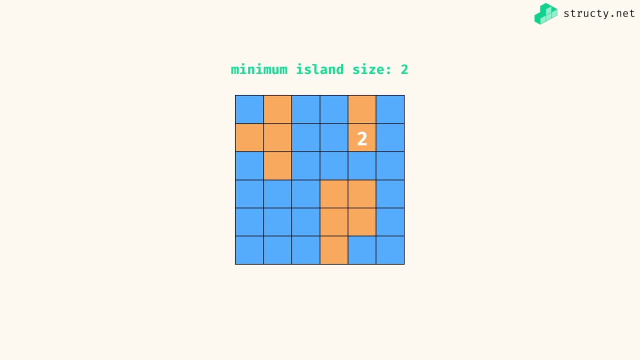 the smallest of the islands, So that would be the two over here. So how can I actually come up with a strategy for this one? you should already know that this is just a spin off of our previous a grid graph problem, where, instead of doing just a count of the 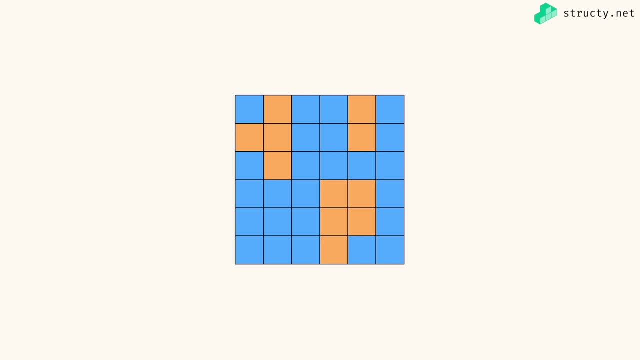 number of islands. now I want to find the sizes of islands. I know to actually look at different islands I'm going to need some nested code, but I'm also going to need some depth first reversal code to explore a single island. So overall, this should be a pretty classic strategy for us. So let's say we started. 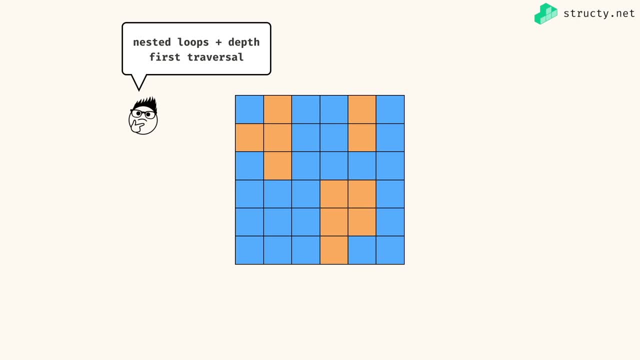 attacking this. we know we're going to begin our nested loops in the top left corner And if our current position is water, then we actually don't need to do anything. Next iteration: I have some land At this point. I could begin on my depth, first reversal, And I know that. 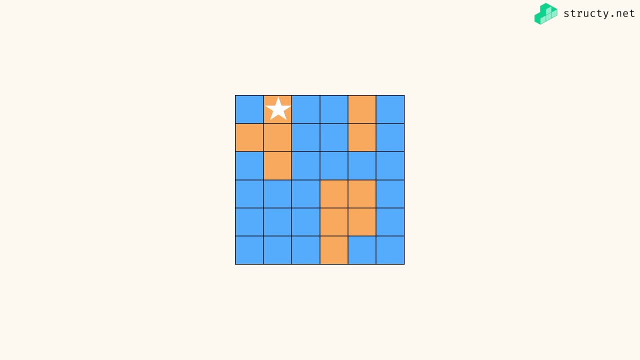 I should be marking things as visited to avoid any infinite loops, right? So, by the way, by the time this traversal completes, I'm going to mark all of these guys as visited, But I also want to determine the size of this entire island region. So every time I get, 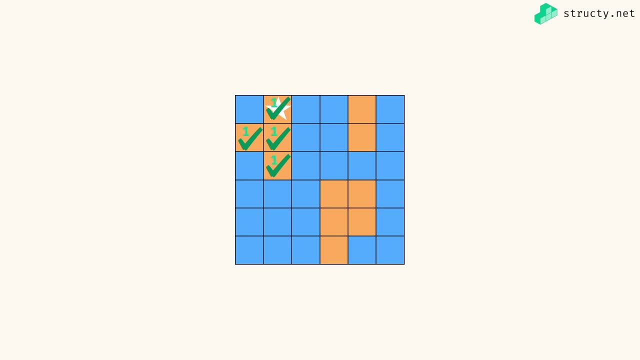 a position that is land, I should treat it as one. And then, when it comes to how I implement my traversal, I can just gather up these ones, right, just add them all up, So that would look something like this: And for my top level call for that traversal I should get an island. 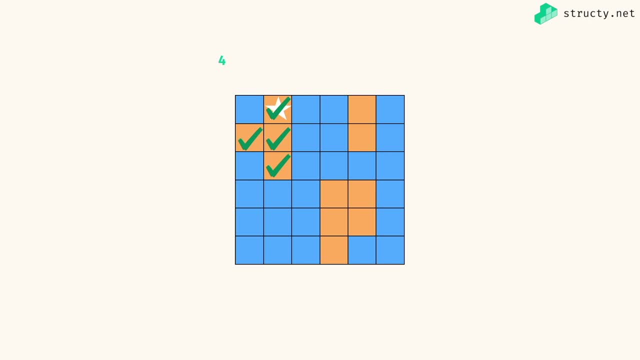 size of four, And so if that kind of traversal algorithm, especially how we compute the size of the island, is pretty hand wavy, don't worry. Now, when we actually go through the code walkthrough, it's just a matter of some recursion, And some recursion we've actually seen before. 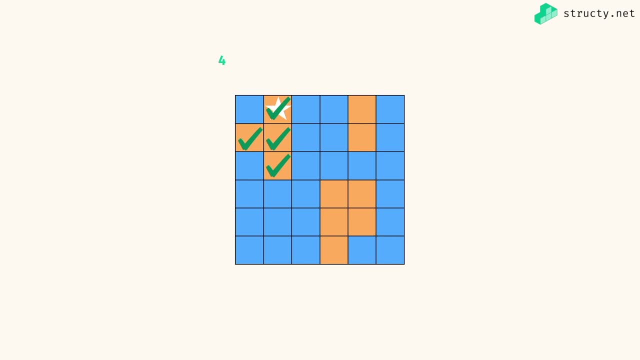 in past problems, of the course, But any case, now that I have this island size of four- it's actually the first island that I've seen, And so I'm going to consider it the min size so far, But I need to keep looking in case something is smaller. So move to the right. 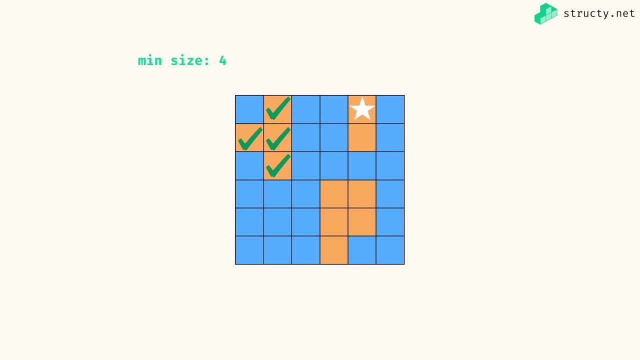 So if it's water, I do nothing. Water again, do nothing. Now I have another island And so I begin my traversal, mark these as visited, And when I find the size of this island, of course it's going to give me two. I compare that to to my current min size. two is smaller. 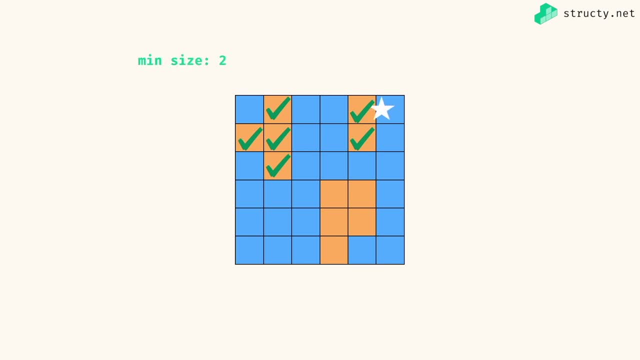 So I store two as the min size so far And we just continue business as usual. Note that when we get to a piece of land, we really want to make sure that it's land but also a piece of unvisited land. So right now that piece of land, but it's visited. so I should 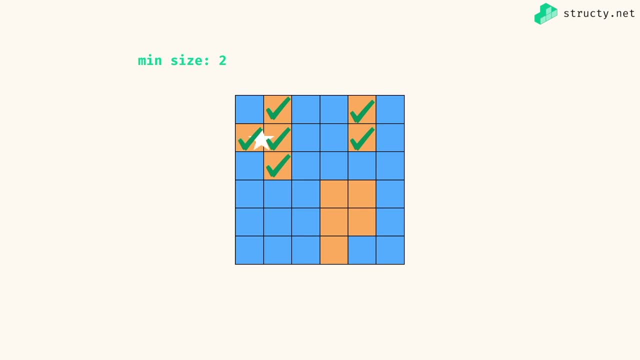 not where I don't need to start traversal here. Likewise for this position. Eventually, though, I'm going to hit some new unvisited land, in which case I should begin my traversal. I'd explore this region And I want to count. 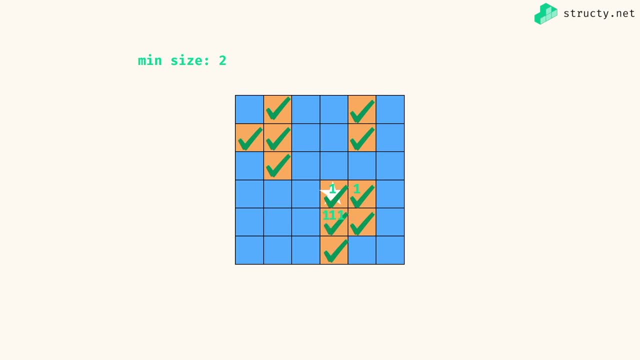 up all of these pieces of land And I should realize that the final size of this island would be five. I can compare that five against my current min. five is bigger, So the size of two gets to stay And I can just end up returning the minimum size by the end of this. 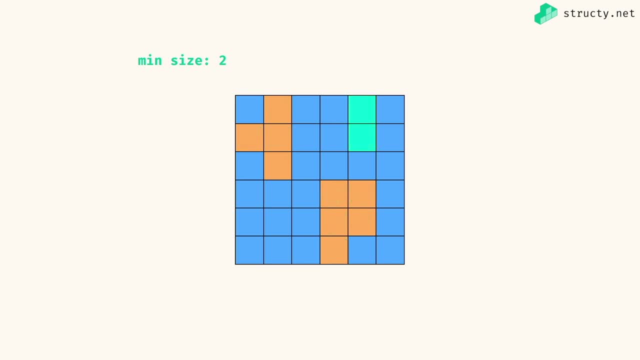 algorithm basically representing this island of size two. The complexity of this algorithm is straightforward. we should say that the size of our input is r times C, because we have r rows and C columns, in which case the time complexity is simply r times C. right, we have to iterate through every row, column within the grid, And even 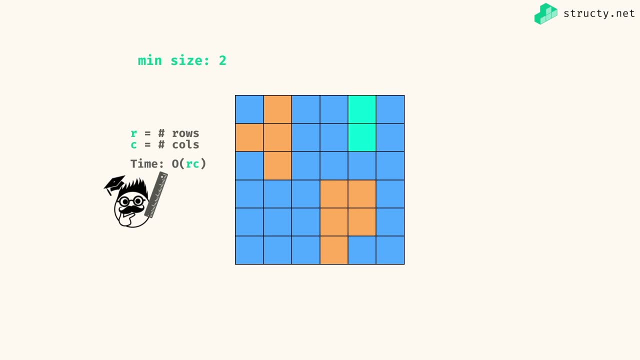 when we begin a traversal. in the worst case, we could have an island that spans the entire grid, in which case it would also be r C right. So, overall, our full complexity is our time C, space complexity is our time C, and we'd have to integrate that into our 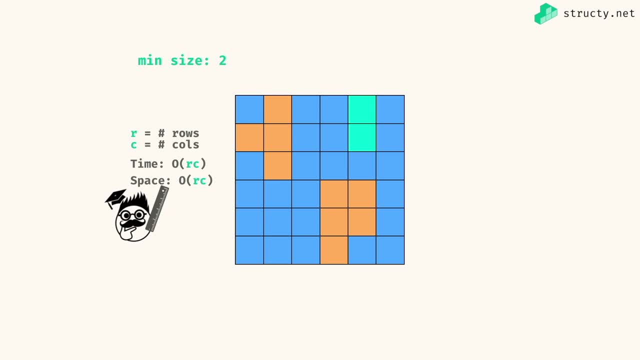 times C as well. And do know that this is technically a linear solution in the size of the grid right, Because the grid itself is exactly our time C positions. So with that I think we're ready to code this one up and try it on your own first, And if you get stuck, 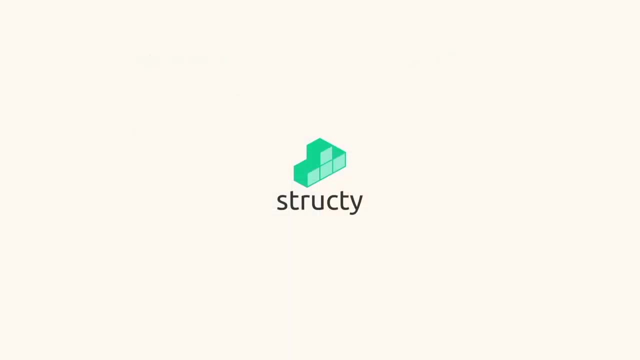 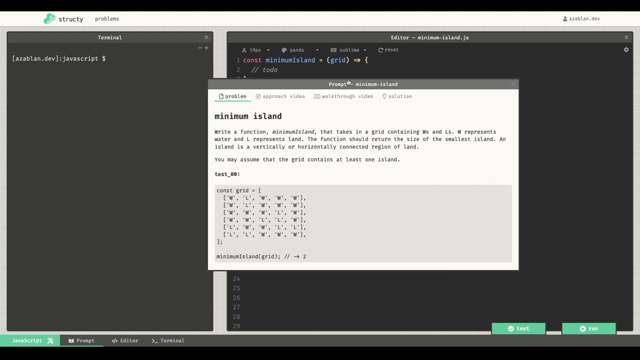 I'll catch you in the walkthrough videos. See you there. Hey programmers, Alvin here right now let's go over a JavaScript walkthrough for this minimum island problem. So I'll jump right in. make sure you watch the approach video. as always, this is just a nice spin. 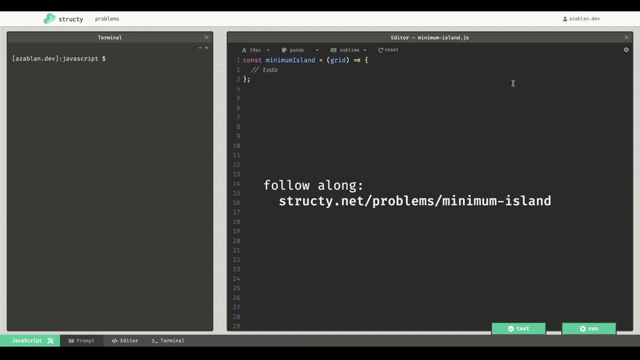 off of our classic island hopping logic, but for a grid graph, right. And so let's start with the iterative code that can help us begin a traversal starting at every different position of our grid. So that just means some nested loops. So we'll start by iterating. 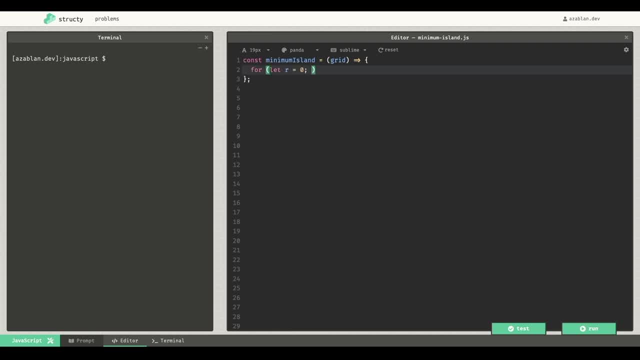 through all of the rows and columns. So r equals zero. go up to while r is less than length of the grid. also, do r plus equals one and very similar loop for my column, But do make sure that you you reference your inner column length, because we could have like a rectangular shaped grid. 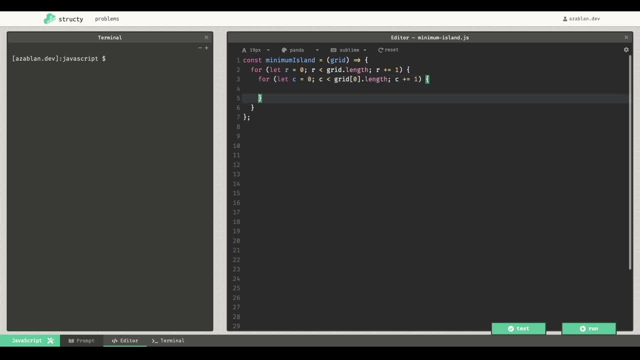 over here And what I want to do now is begin a traversal, starting at every row column. So I'm going to assume I have a helper function here that does that traversal. I'm going to call it explore size. That's because in the long run I'm interested in the size of that. 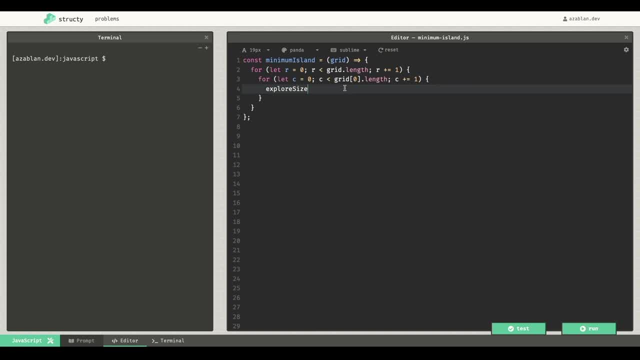 island, right? So like a number representing how big or how many positions that island spans. So I'm going to pass along the grid information as well as the position. So I'm going to pass along the grid information as well as the position, And I know when it. 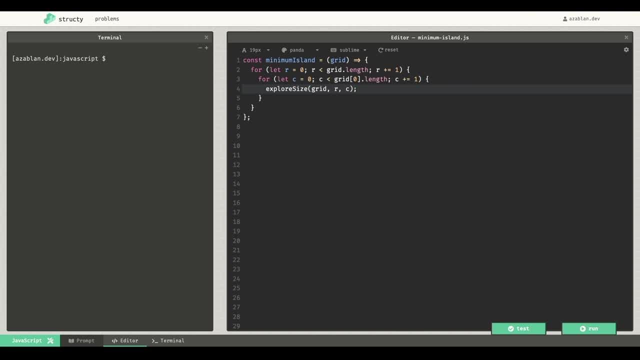 comes to all of these, like undirected graph traversals, should probably guard against your loops, And I have some foresight here. So I'm going to pass along a nice visited set which I can maintain globally for the entire traversal, because there's only a good reason. 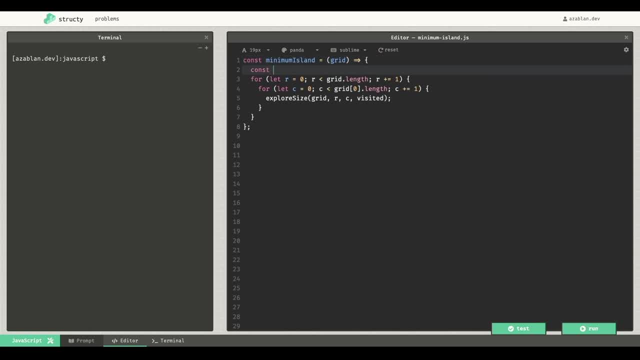 to explore a position once right. So I'll create const visited. I'm going to make it my nice JavaScript set, And a few reasons for that. Well, for one JavaScript set gives me all of one lookup but also all of one insertion, So it's going to be a really good. 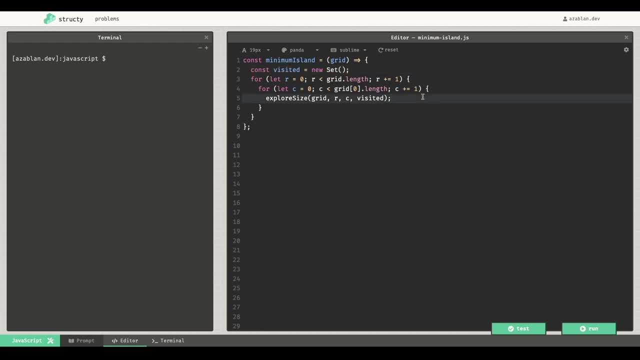 a really quick data structure to use And from there you probably have to add some more logic over here to actually do something with the size. But for now I think I'm going to switch gears and actually take a look at building this helper function right, So I? 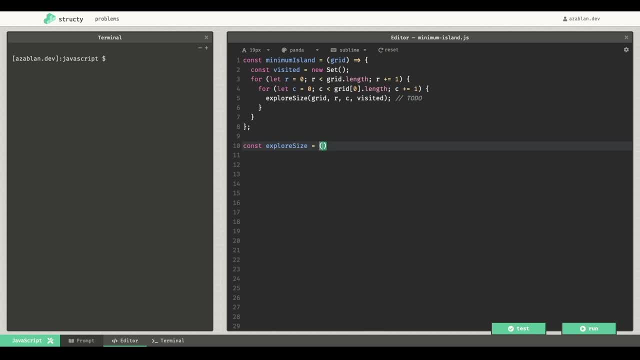 think the best way to build this traversal is to use a depth first. typically just my go to for a problem like this. it's going to take in. I know the grid, the row and the column and also visited. I need some base cases, very classic base cases. I'm going 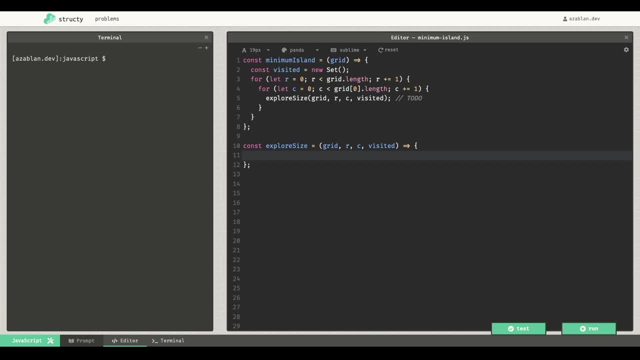 to start by checking If this row column position is in bounds. So my favorite pattern for that is to split up in some variables. just makes it easier to read and debug. So I'm going to say, is my row in bounds? and just make that like a Boolean variable. So I'll check if let's. 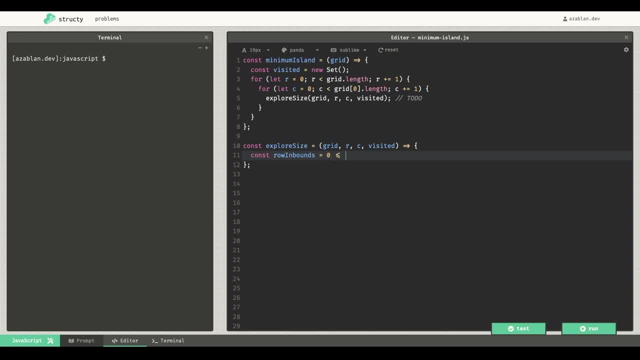 say zero is less than or equal to the row needs to say and write and that row should be strictly less than the grid length. So this Boolean would only be true if it's in bounds right, And something very similar for my call in bounds should. 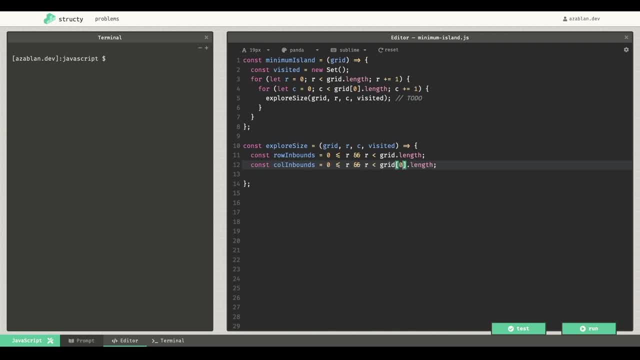 be between zero and grid, zero length. Nice, just like this, I believe. And then I can write a nice if statement using both clauses. So I can say: all right, if let's say your row is not in bounds or your column is not in bounds, then you're definitely out of bounds. 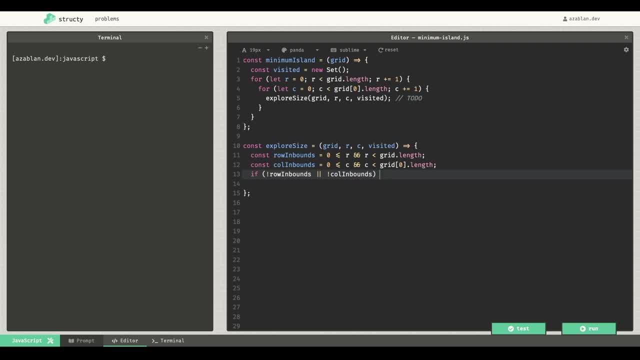 So you should probably use some base case here, right? So I'll choose to return here is zero, because I want to keep a consistent number right, Consistent return type, that is. I know that this function has a kind of goal of returning the size of the export island size as a number. 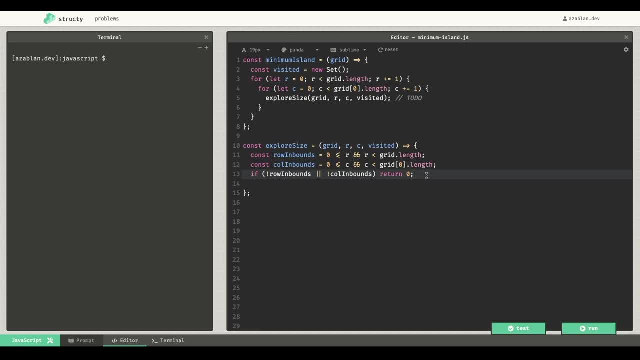 So even in my base case, I need to make sure I return some type of number, returning zero, to represent that, hey, this is out of bounds, it's not going to contribute anything into the count of the size, right, which is good to go. I need some other base case here. what? 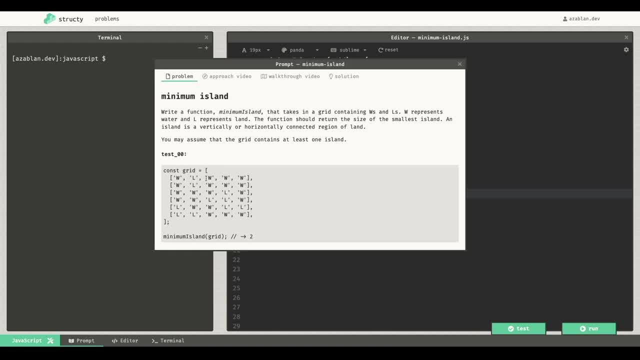 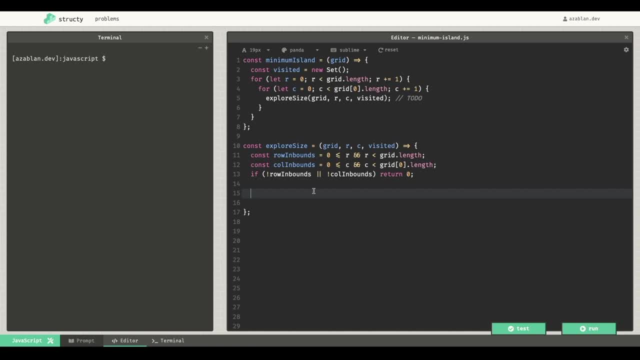 if my position is in bounds. but what if it's actually water? I don't want to count that as well. I only want to count islands. so land right. And so quick fix, what I'll do is add a new base case. I can check if my 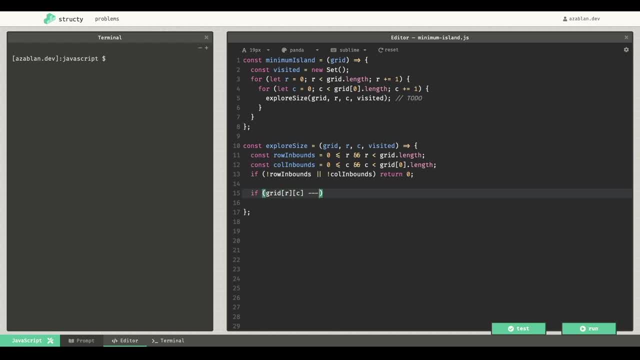 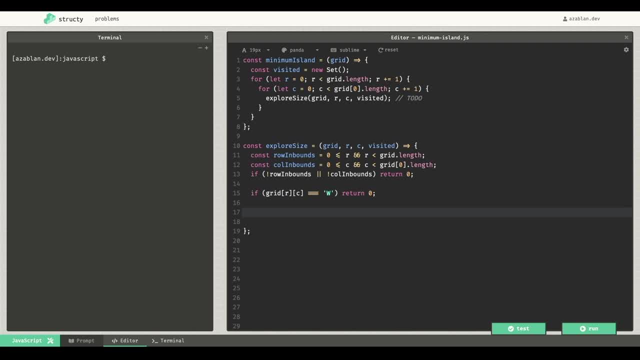 and do that, And I'm going to go ahead and do that. And I'm going to go ahead and do that. I'm going to go ahead and do that And I'm going to go ahead and do that. I'll go ahead and do that. I'm a final condition I'll have here is alright if I make it past both. 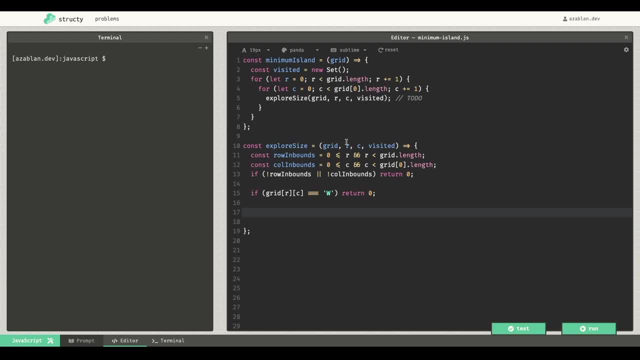 of these base cases. it might be the case that this position is land, but it's land I've already visited. So here's why I work in my visited logic. I'm going to represent a position, like we said in the last episode, as really just a string, So I can put it as: 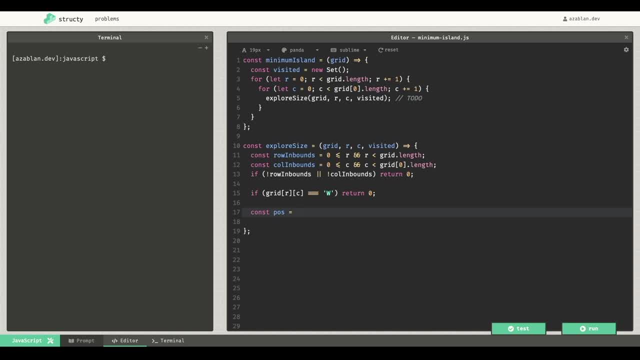 the members of my visited set. So I'm going to say position, so going to be the row plus a comma, plus the column, So just representing Dan Mc�ar, такие position. And that's because I can't add like an array into a visited set and then look. 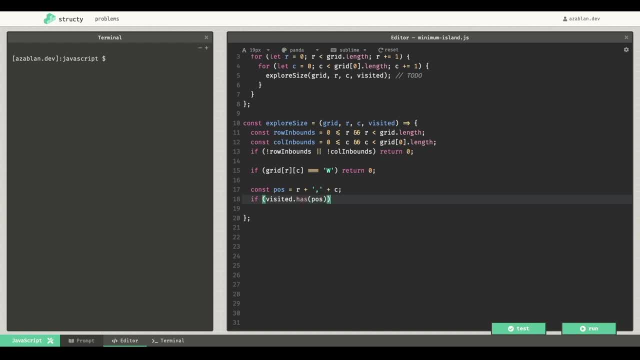 it up later, And so if visited has the position, then it's a duplicate position that I've explored, So return zero. Otherwise it's not been visited yet, So I must be visiting it right now So I can add it. Nice, So I have my base cases laid down. Now I'll need my actual recursive. 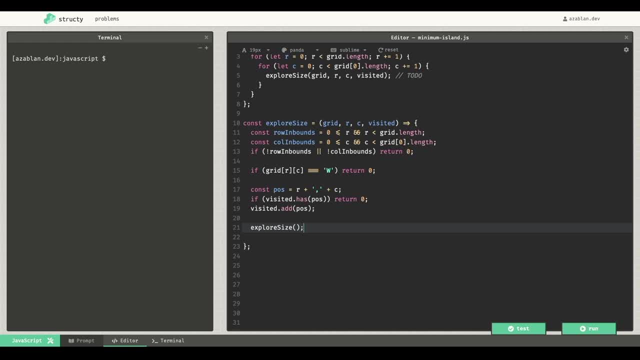 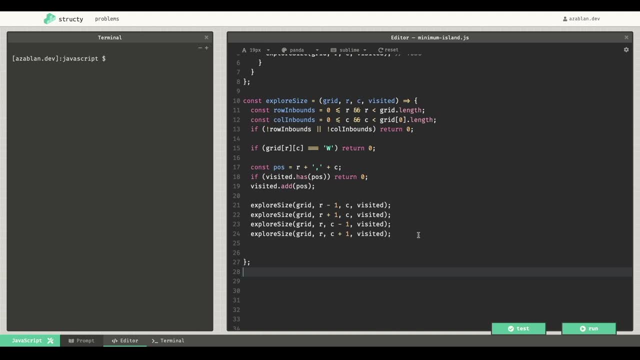 code, So I'll explore my four neighbors. By now you should be familiar with this pattern. So go upwards. a row minus one column passed on the same visited. So I'm going to explore my up down, left, right neighbors respectively, And I do my recursively buffet here right. 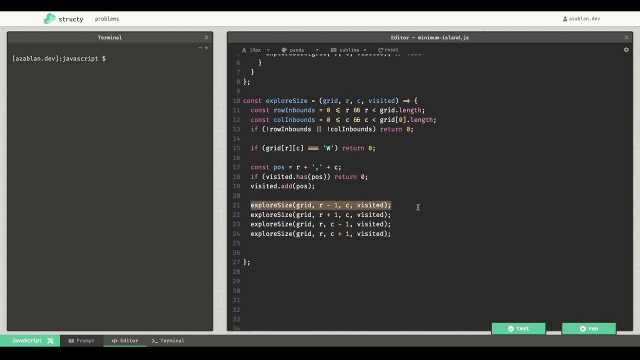 So what type do I expect back from these calls? they're going to give me back a number representing the size of the island that my neighbor is a part of. But if my neighbor is part of some larger island, then I am too, because we're connected right to our neighbors And so I 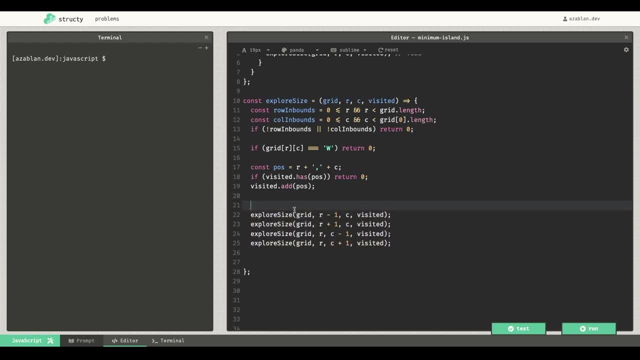 want to create the grand total of all of these return values. So I'm going to create some size variable. Let's say let size. I'm going to initialize it to one over here. it's going to be one and not zero, because the one represents my current position, my row, column And whatever. 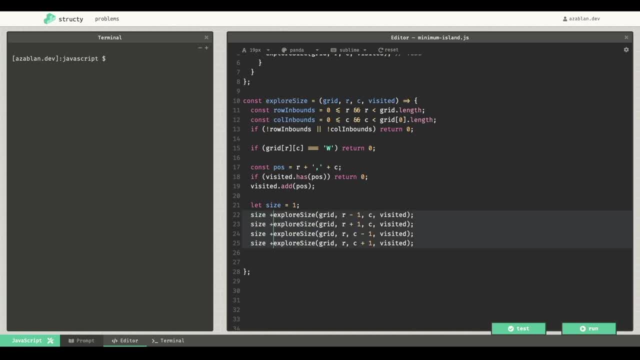 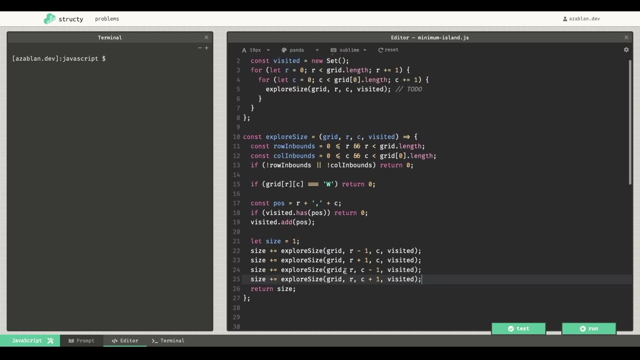 these calls return whatever number. I'm just going to increment my size by that number, like so, And finally I can return our total size over here. So that will do my depth first reversal because it's recursive, But it will also tally up the nice size of this island. 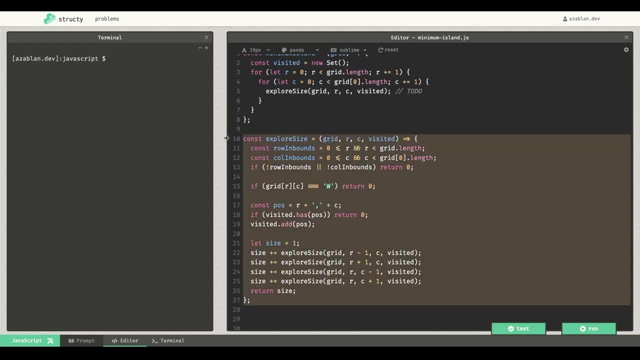 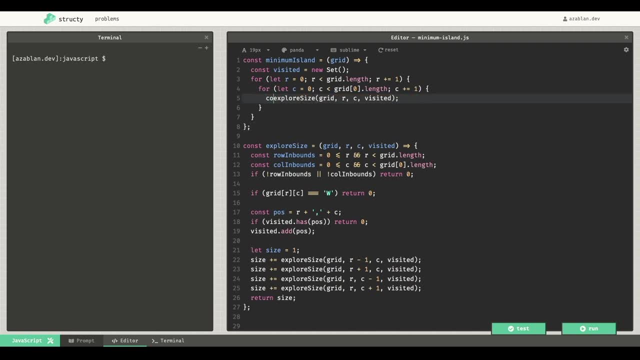 region, Cool. So now that I have a working explore size helper, let's use it in our main function here. So I'm going to get back a number from this call. I'll call it my respective size. And what's great about this logic is, if I have a island or position that I've already 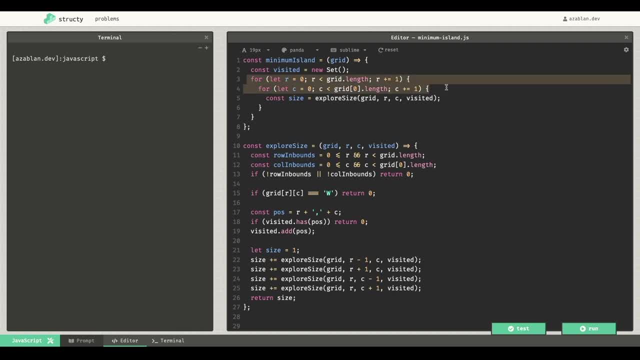 seen before and I encounter it again in this, this for loop. then I would just return early because I would hit this base case, right: if something has already been visited, just automatically return zero because I've already considered it, No reason to consider it again. But now I need my minimization logic, right? I want 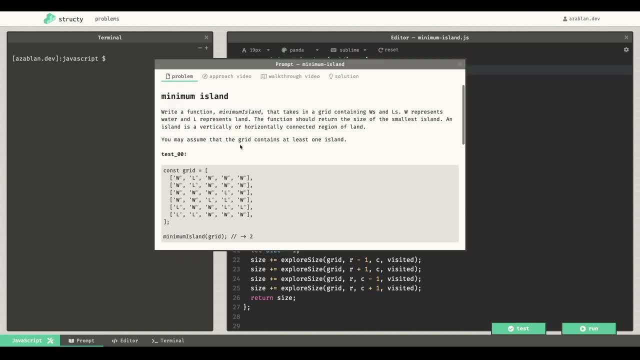 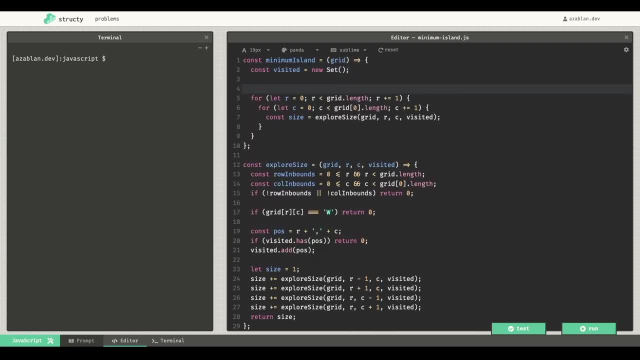 the size of the smallest island And they tell us in the problem that we can totally assume that your grid contains at least one island. So I think a great default value here is to use positive infinity So I can set- some will say- min size variable to be positive. 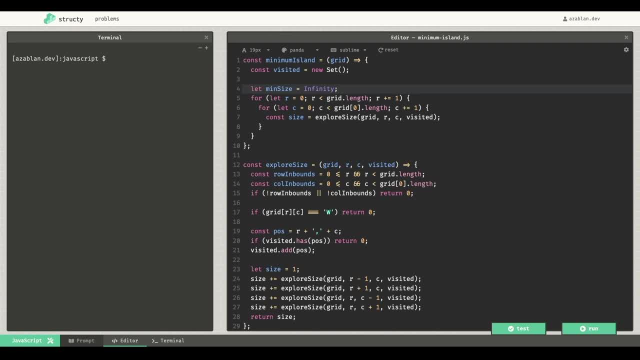 infinity JavaScript. If I make it positive infinity, I know when I encounter any like valid the island size, it's going to be less than infinity and it should replace it. So now I can do some min logic here and check, all right, if the size of this island is less. 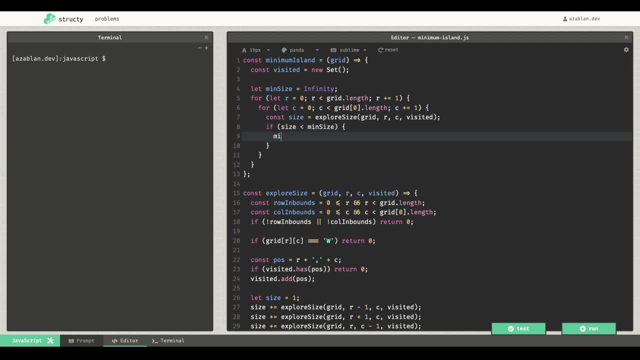 than the minimum size I have seen so far. then just replace that min size with that island And after I'm done with all of these traversals- potential traversals- I'll return my min size. So some classic patterns here. There's one nuance that we're not considering. 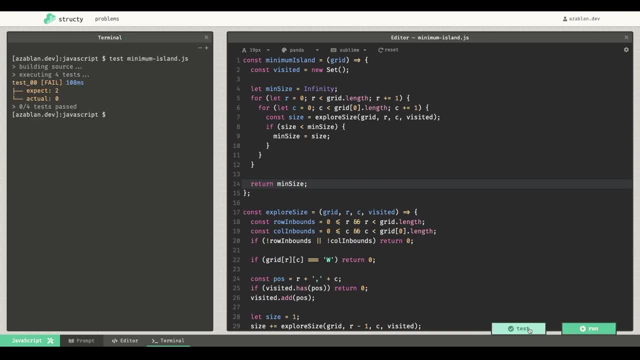 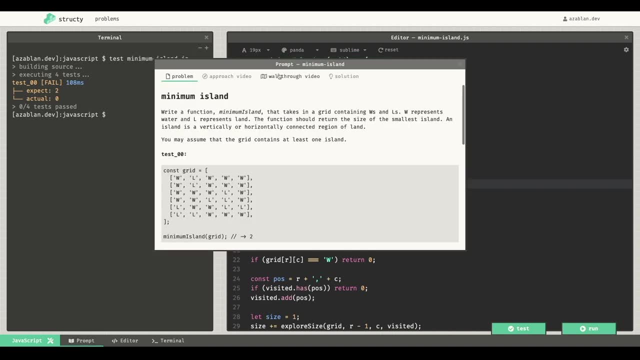 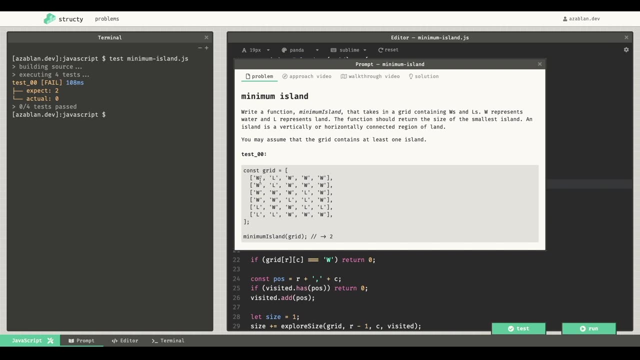 Let's run the code and we can debug it together. So it looks like we failed example 00.. So the very first example: we accidentally gave back zero. if you look at that first example, it's pretty obvious that, yeah, the minimum size is two, representing this island over here. The reason we're giving 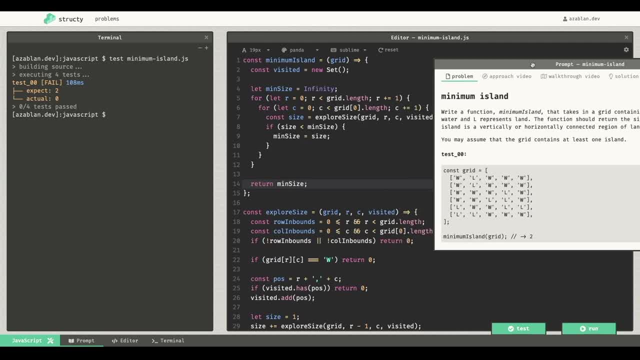 back. zero is according to our code. Let's say we're on like the very first iteration. we can already spot it. I know that rows going to be zero, columns going to be zero. that means my position would be this: W over here When I make the recursive call and I pass. 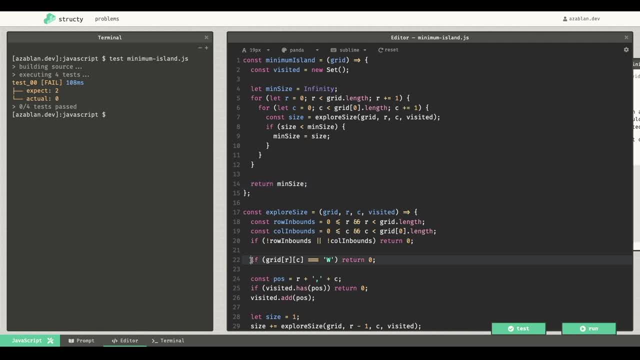 along position 00,. I know that it's going to immediately return zero, because that position is water, And I'm going to check. all right, is that zero less than infinity? it is, So I'm going to replace min size with zero. But if I think about it, zero doesn't even represent. 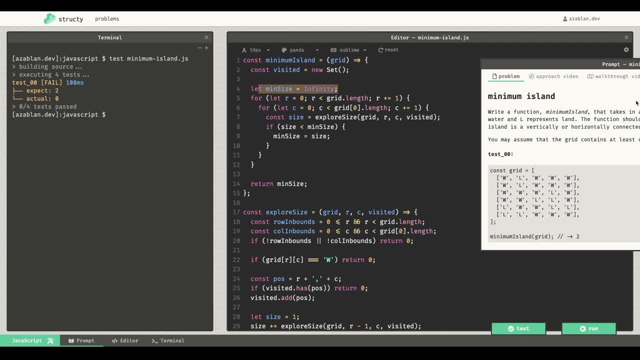 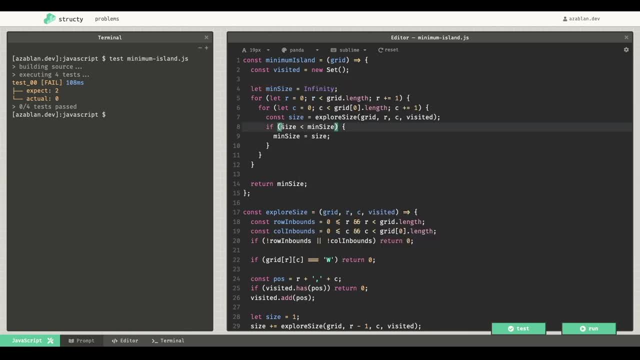 a real island. If an island has a size of zero, then it's not an island at all. it was a piece of water, right? And so I want to add some additional logic here: to only actually look at nonzero quantities, So only do the comparison if that size is also valid. So 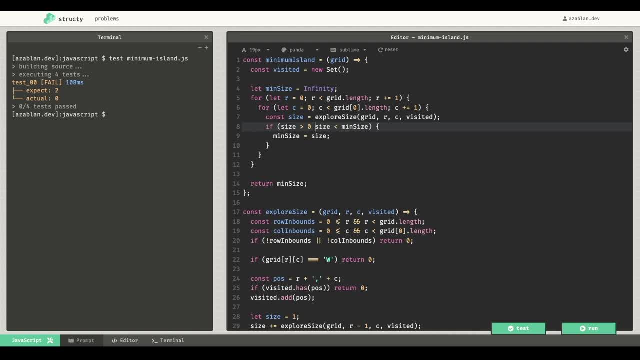 size should be greater than zero, of course, And we'll want to end these together, So let's try that again. Just a little little detail over there that we need: Awesome, And there we have a solution for this minimum island problem. So we've seen this pattern a few.